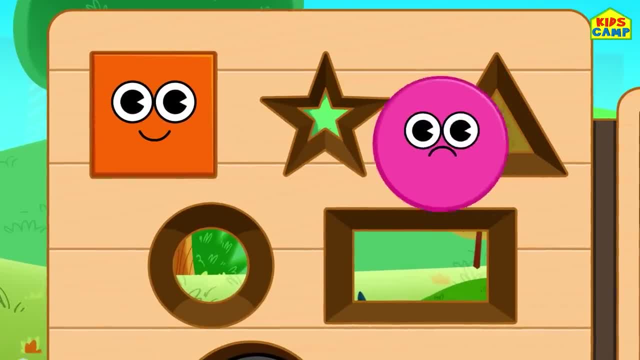 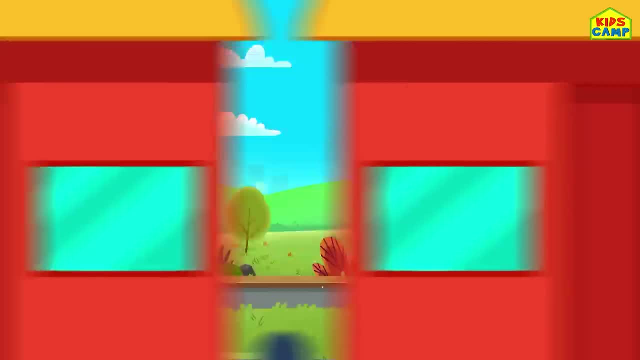 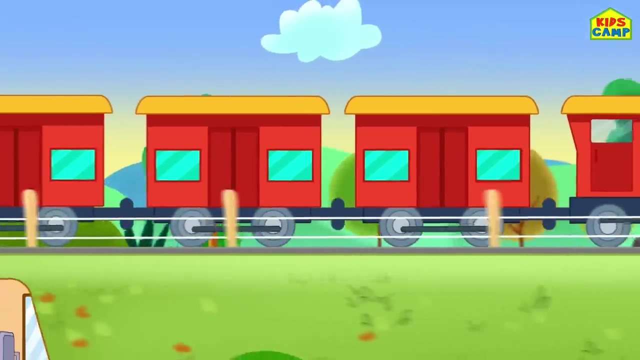 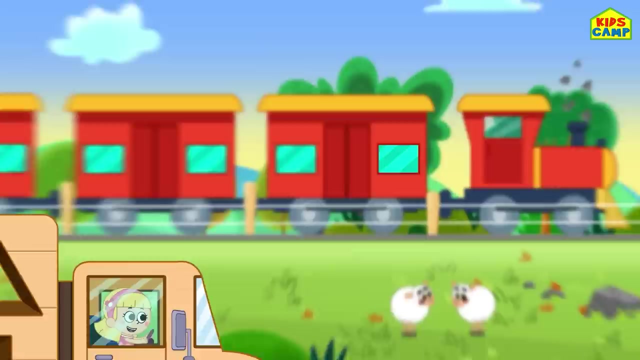 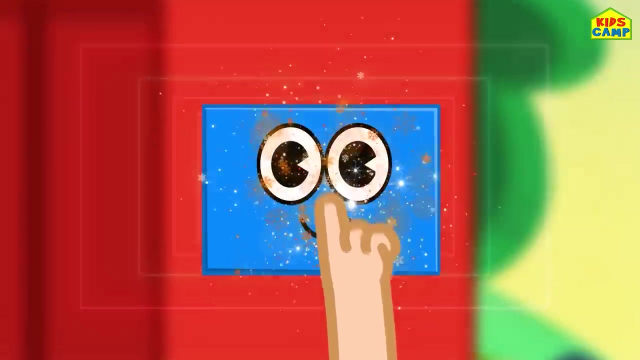 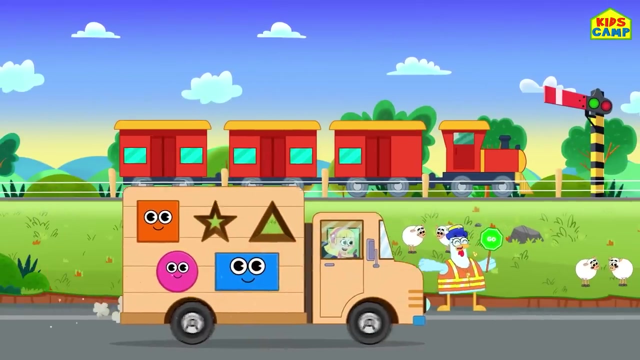 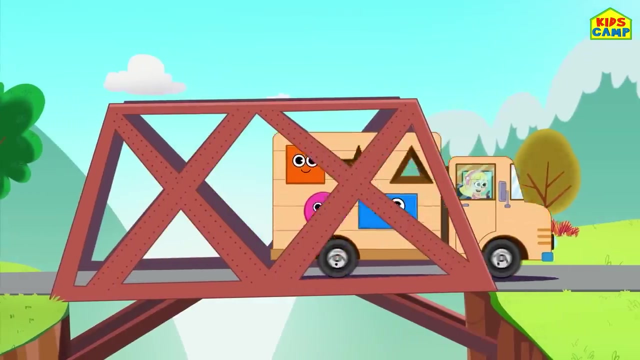 Uh-oh, Not there. No, Aha, It fits correctly, Let's go ahead. Wow, A train. Aha, Do you see what I see Our next shape: Rectangle. Amazing, It fits correctly. Woohoo, Over the bridge, Here I go. Honk, honk, honk, Here I go. 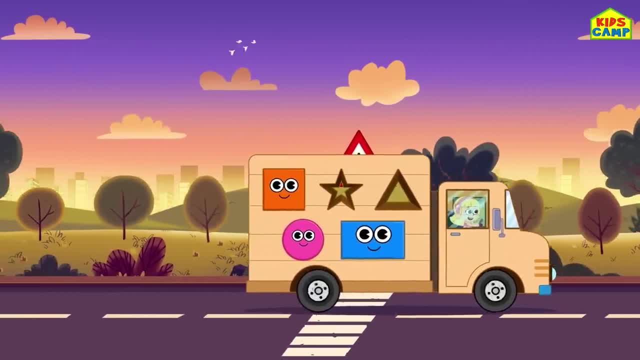 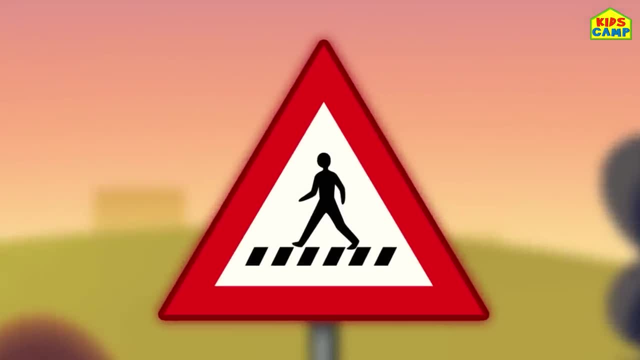 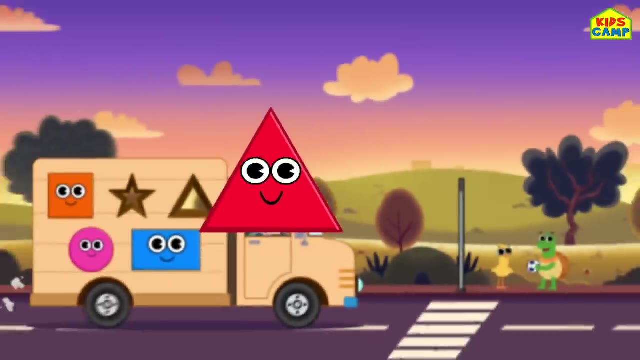 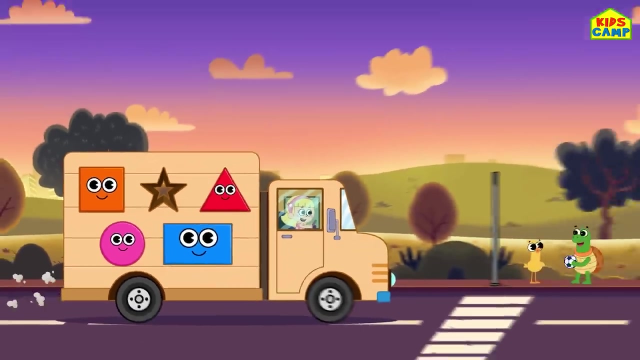 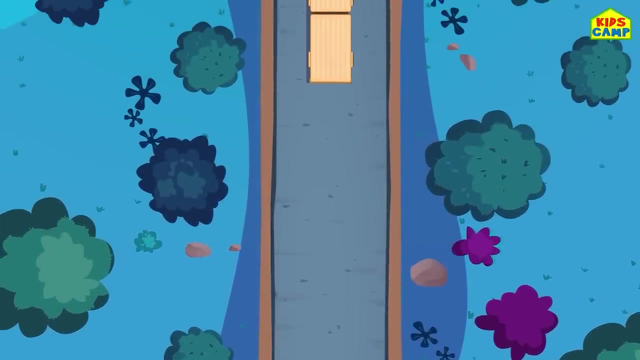 Oh, we almost missed that. Hmm, Is that a triangle? Yes, it is. Wow, Let's place it on my wooden truck. No, Aha, It fits. Let's look for another shape. Where could it be? Wow. 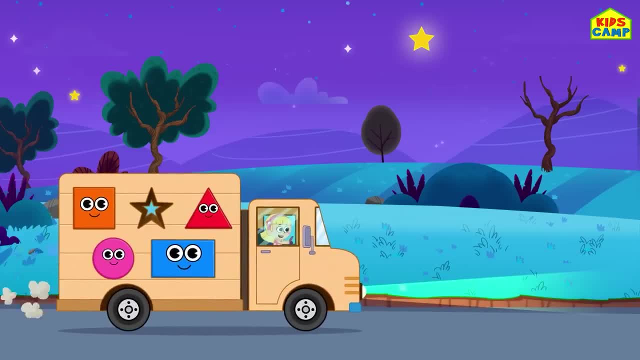 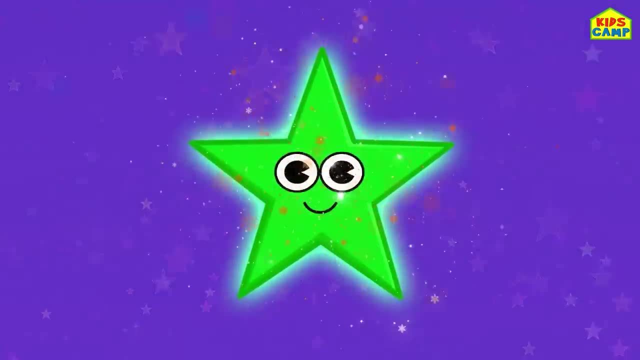 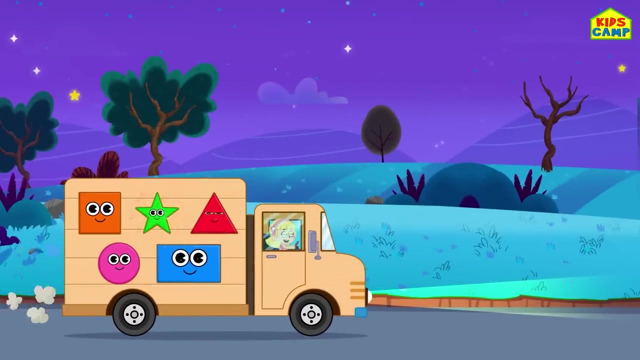 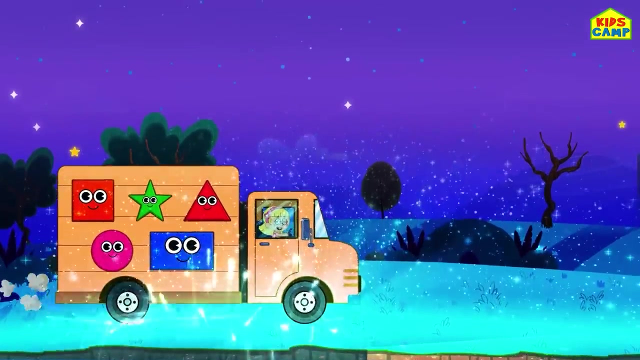 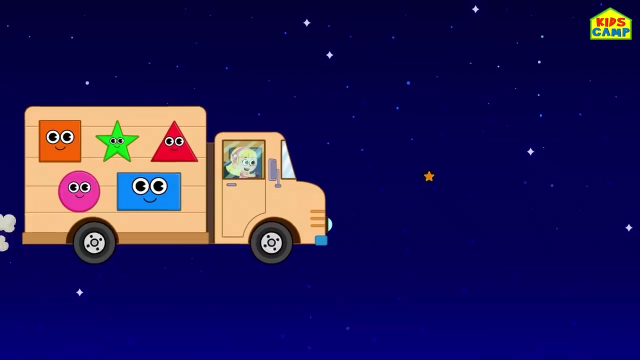 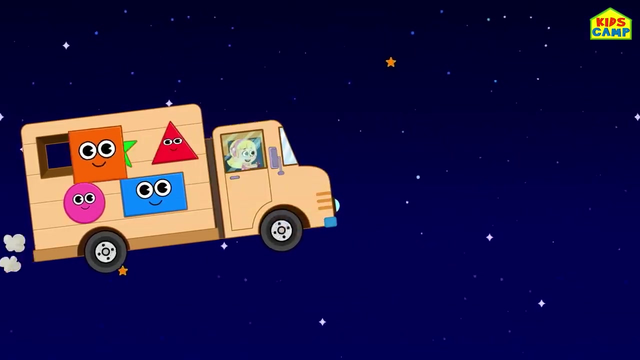 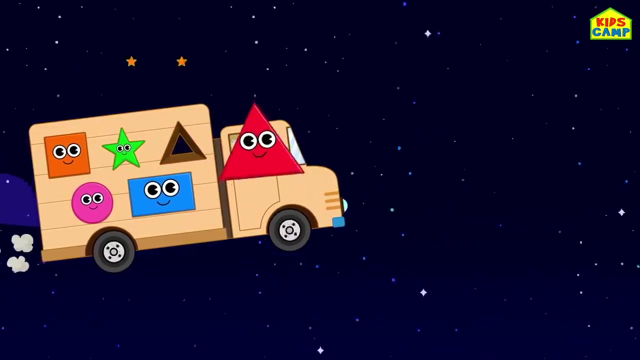 I see it, It's a star Wonderful. Let's place the star on my wooden truck. We've done it. We've collected all the shapes. Oh magic, Wow, Wow, Here I go. Square Star Triangle. 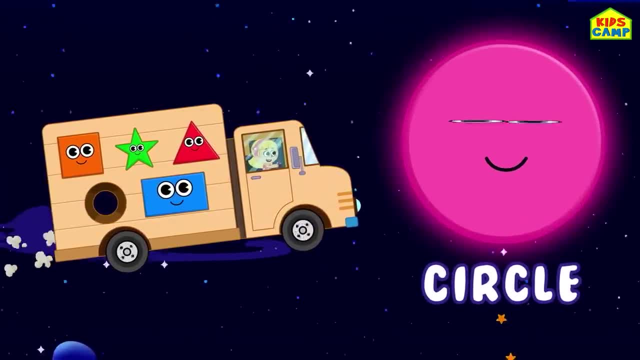 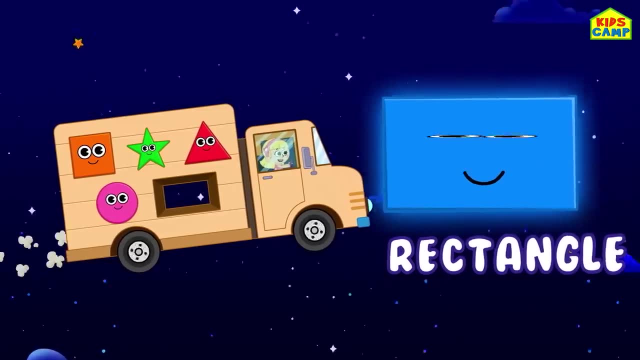 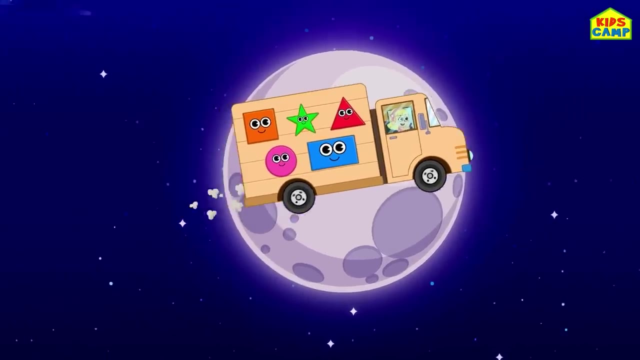 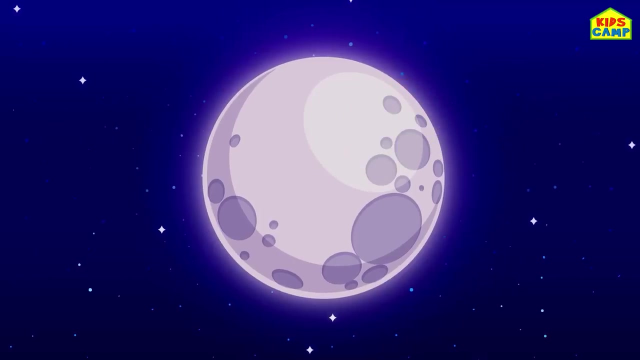 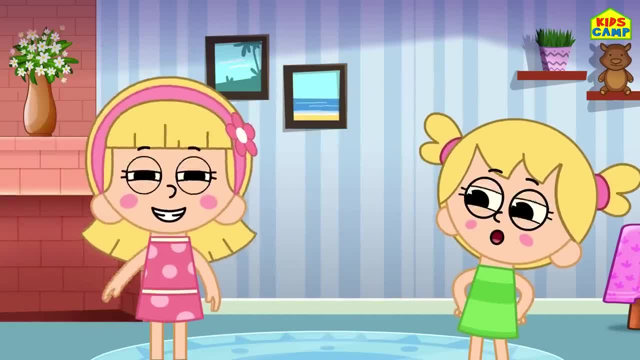 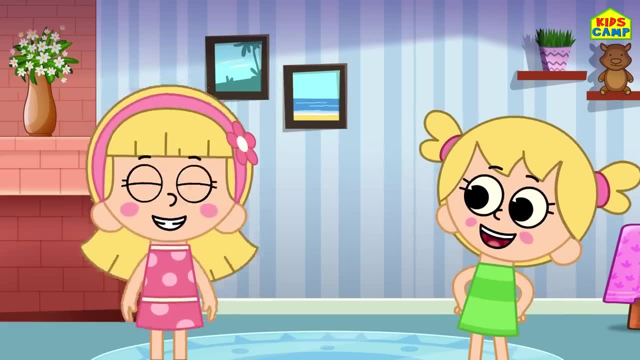 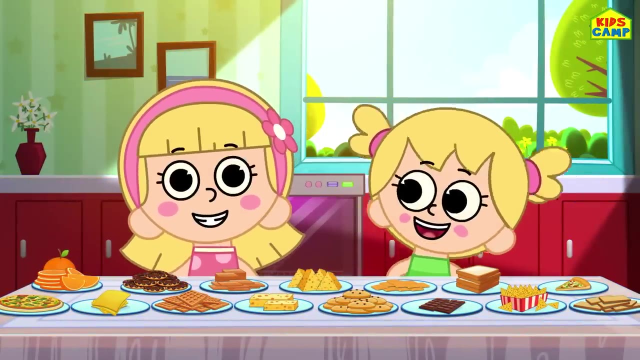 I'm Lily. I'm Lily, Hi kids, I'm Ellie, And this is Eva, And today we're going to have a party. Yay, Yay, Ooh. Look at all this food- So delicious. We're also going to learn our shapes. 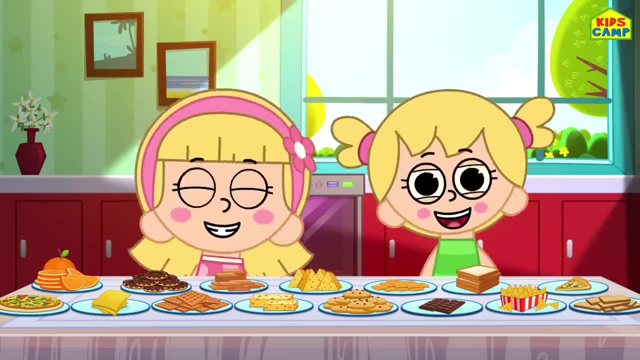 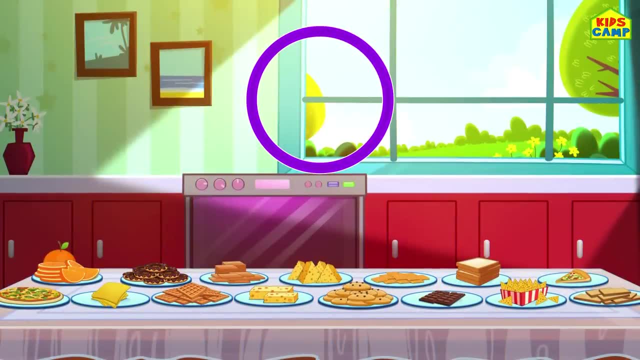 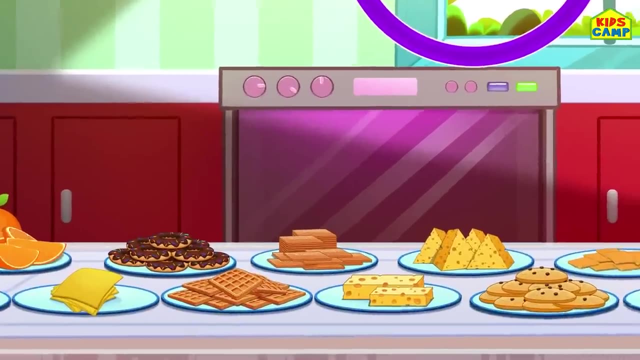 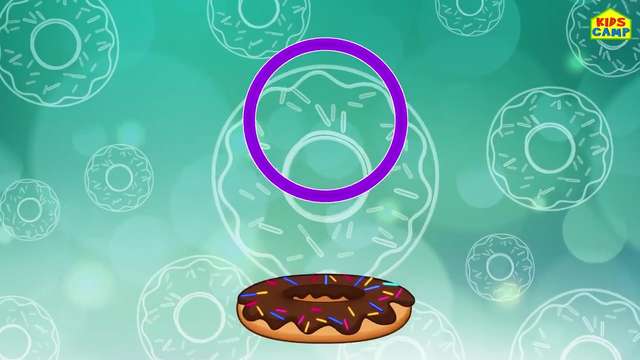 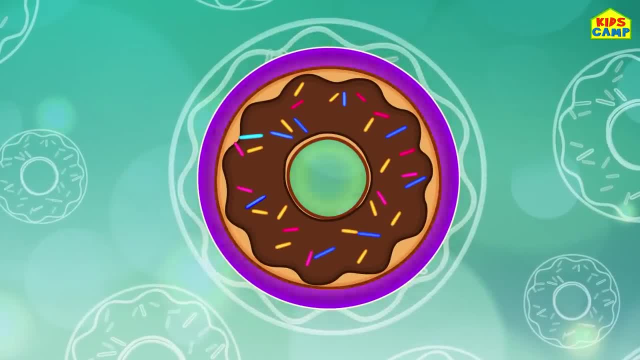 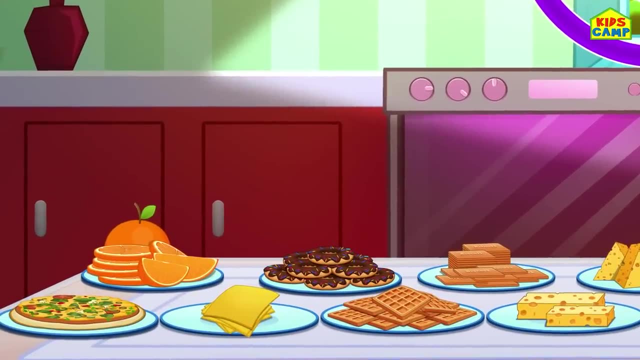 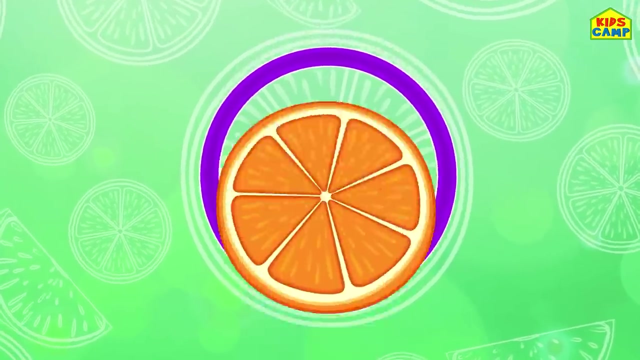 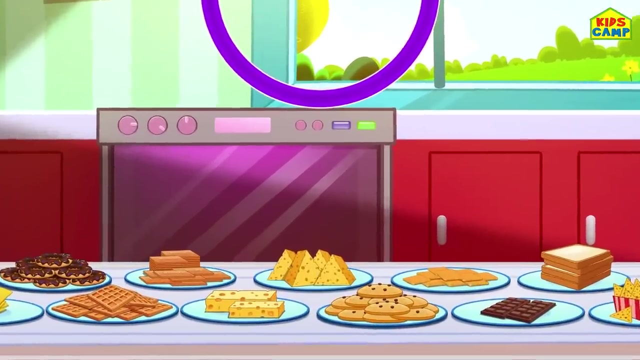 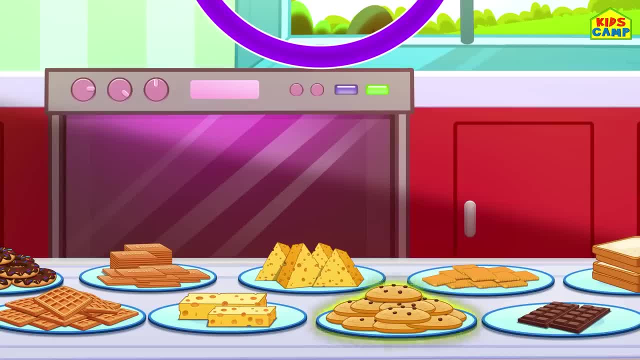 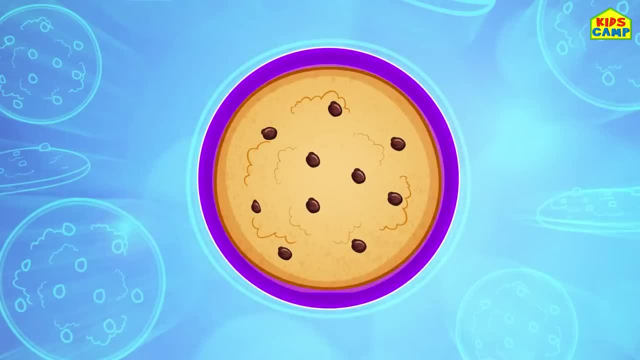 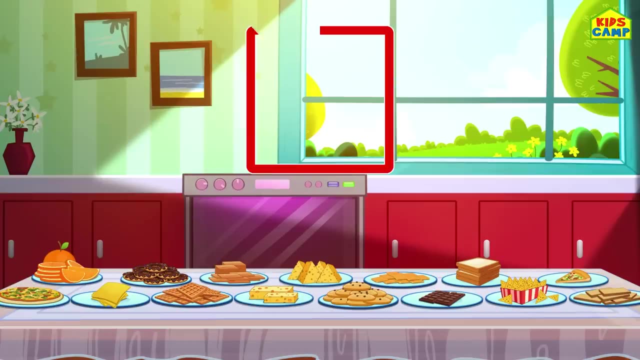 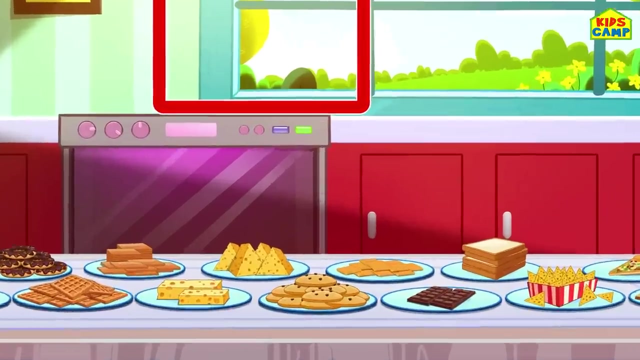 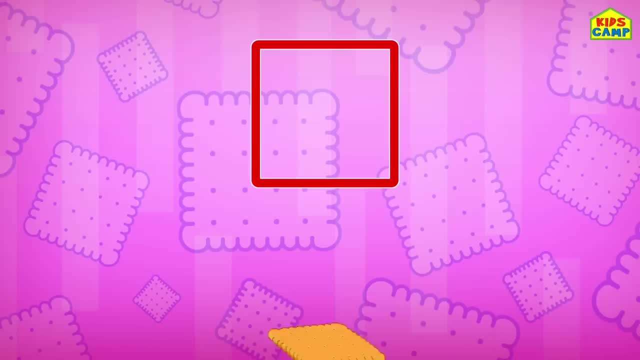 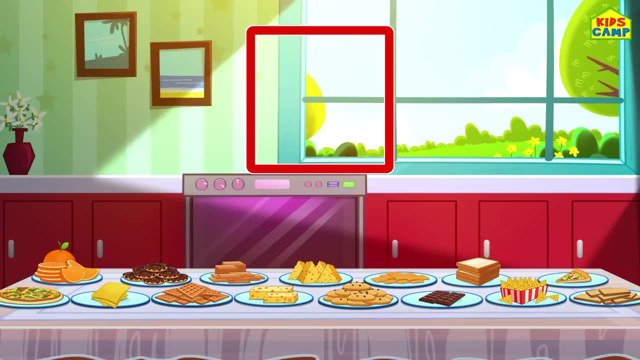 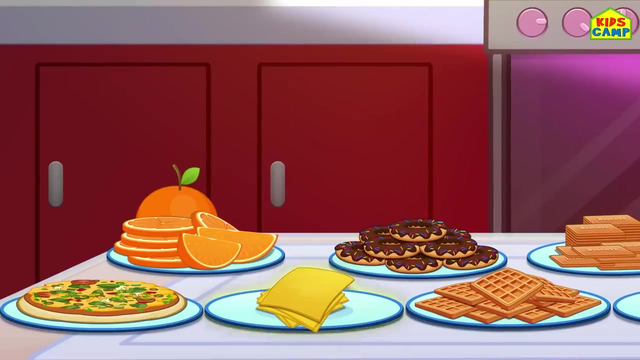 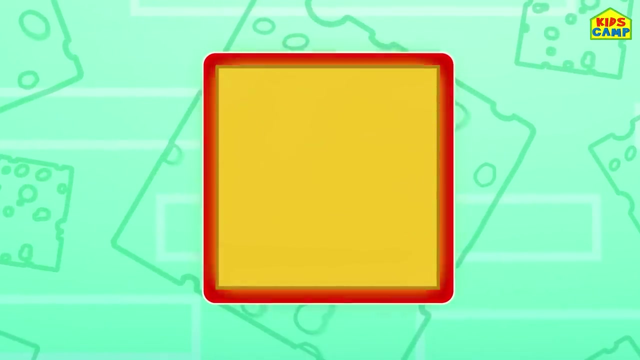 Hmmm, that's right, a craggle, Yummy, that's the shape of a square. What else can we find? that's a square? Aha, a slice of cheese. That's right, a slice of cheese is also a square. 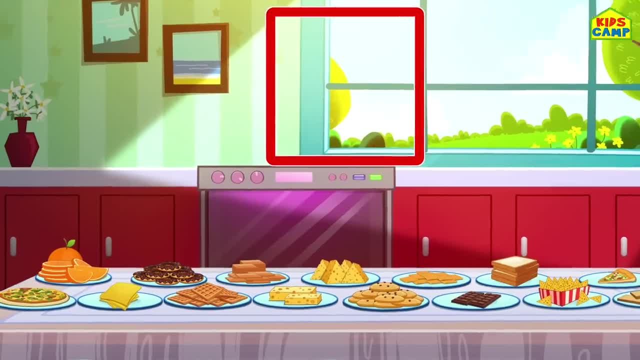 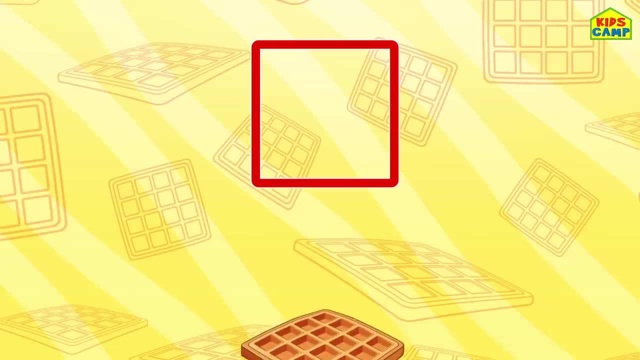 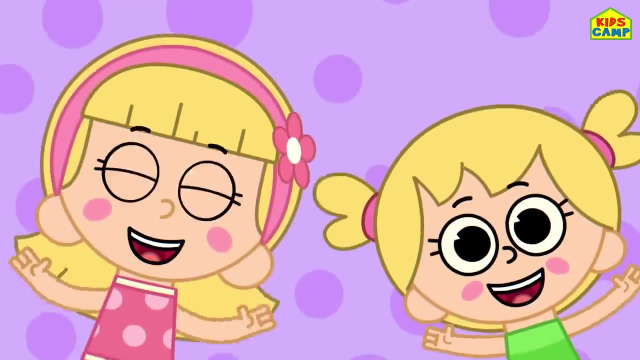 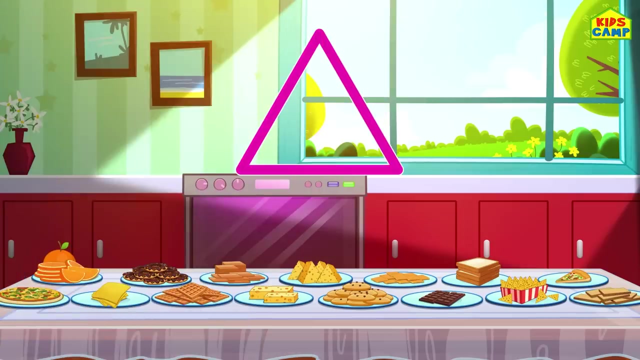 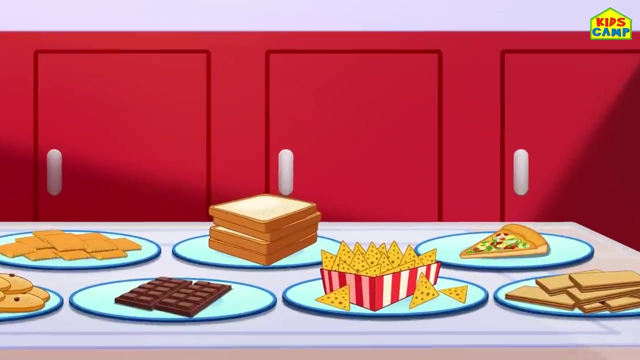 What else is a square? Aha, I see it: a waffle. A waffle is in the shape of a square. Yay, What's the next shape? A triangle. Can you find a triangle? Hmmm, do you see it? 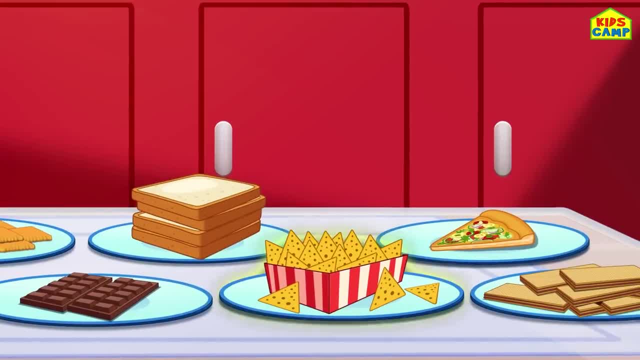 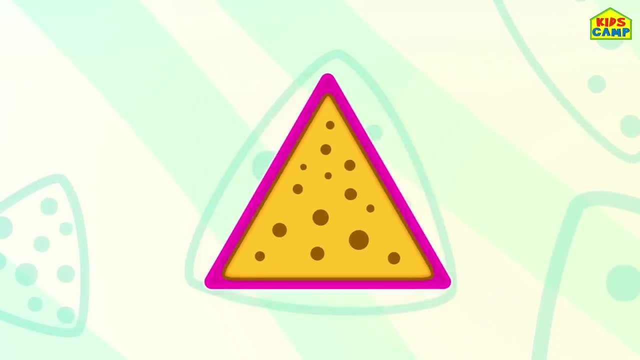 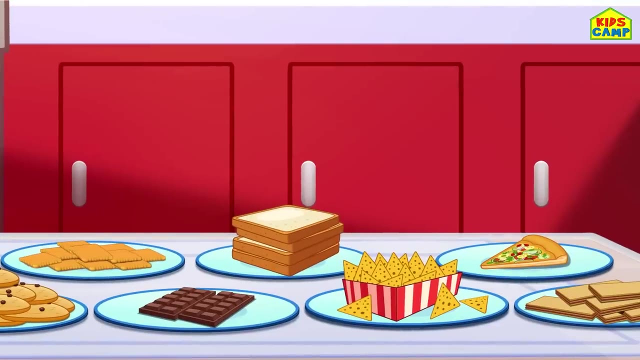 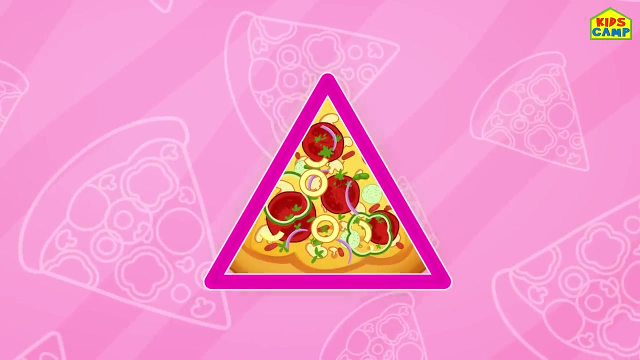 I see it too. nachos- Yay, A nacho is in the shape of a triangle. What else That's right? everyone's favourite, A slice of pizza- Yay, Woohoo, that sure is a triangle. 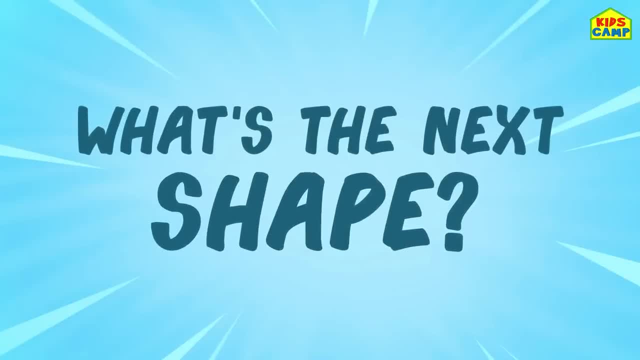 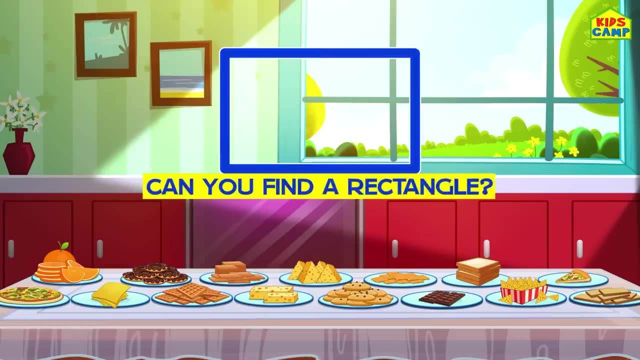 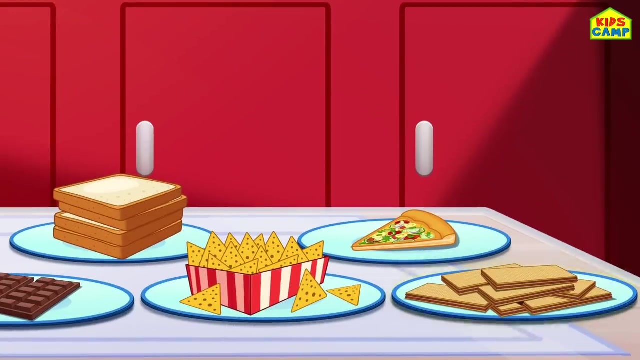 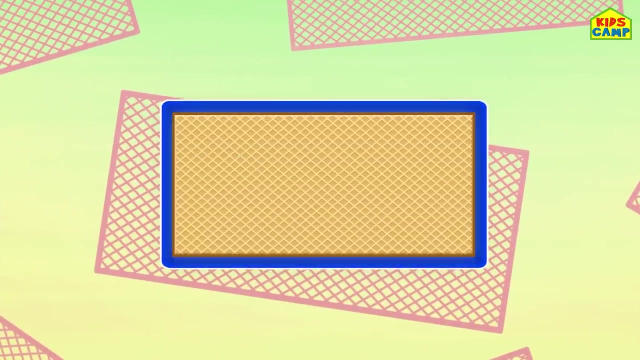 Yay, What's the next shape? A rectangle. Can you find a rectangle, kids? Hmmm, ah, I see it too. a chocolate wafer, That also is a rectangle. Yay, What else? Hmmm, what's that? 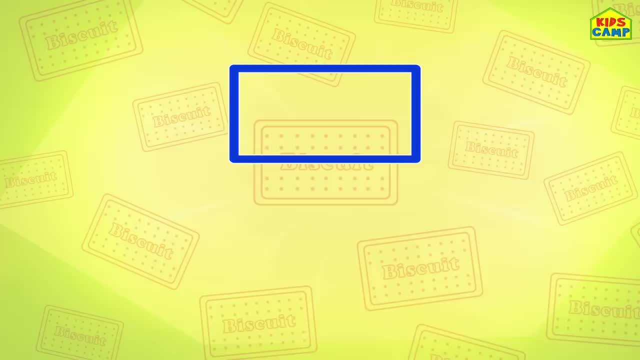 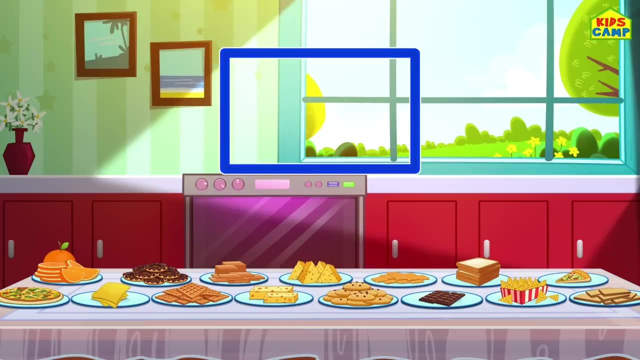 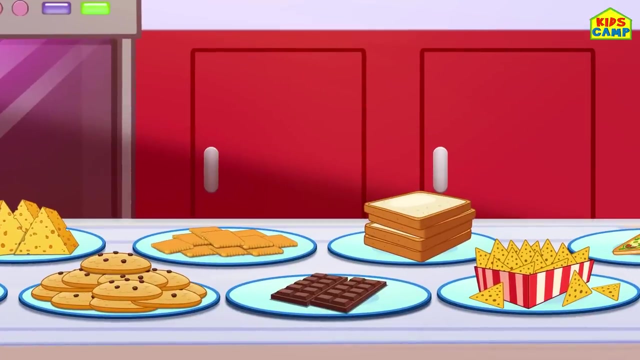 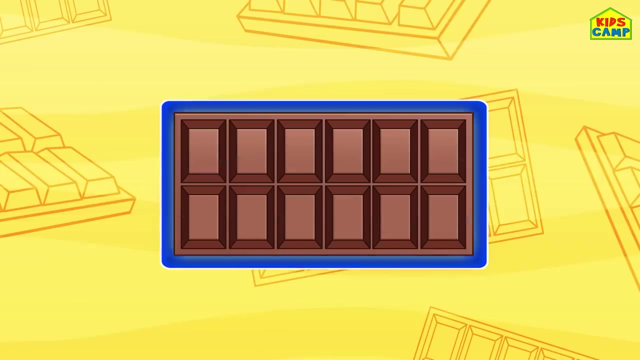 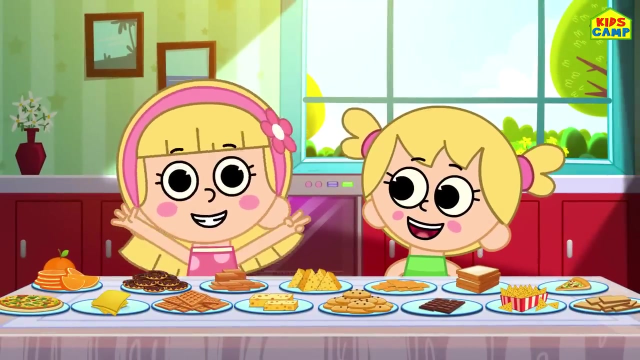 Yummy biscuit. That sure is the shape of a rectangle. Anything else? Aha, chocolate, Woohoo, A bar of chocolate. That's right, kids, We did it. This all looks so good and we found all the shapes. 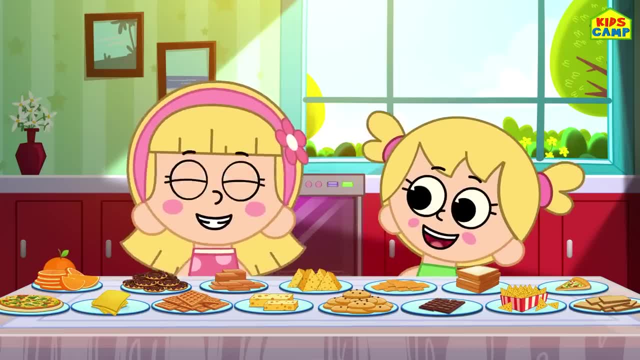 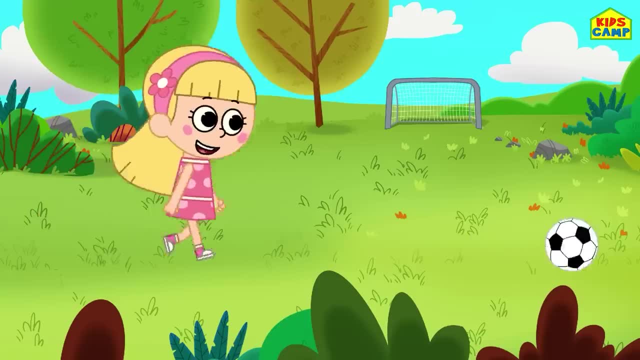 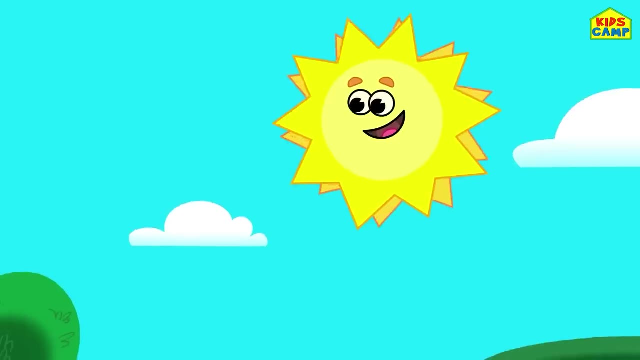 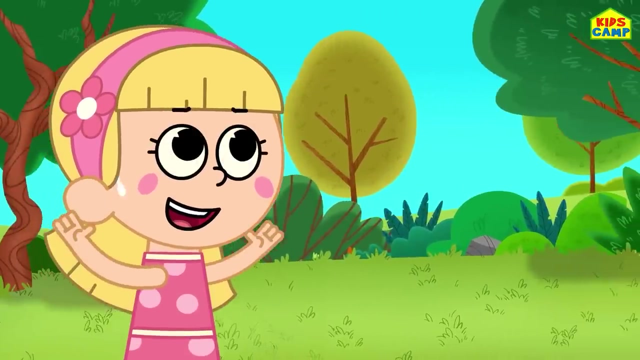 Good job Eva, Good job kids. Bye, bye. What a perfect sunny day to play outside, Oh yay. What should we do to beat this heat? I know let's make summer coolers. Hey friends, what fruit should we pick first? 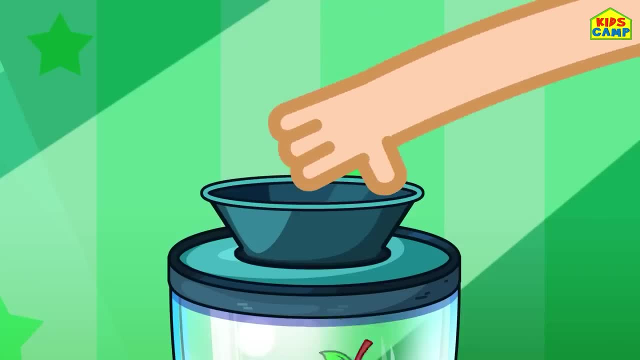 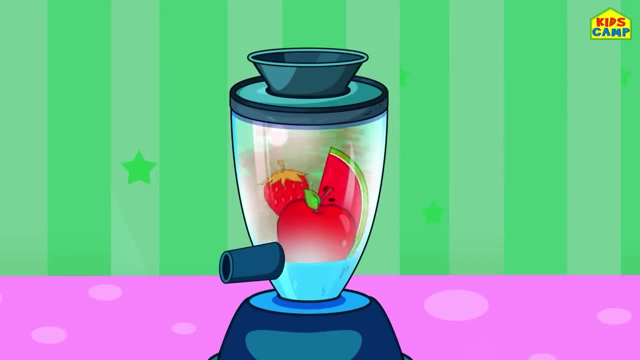 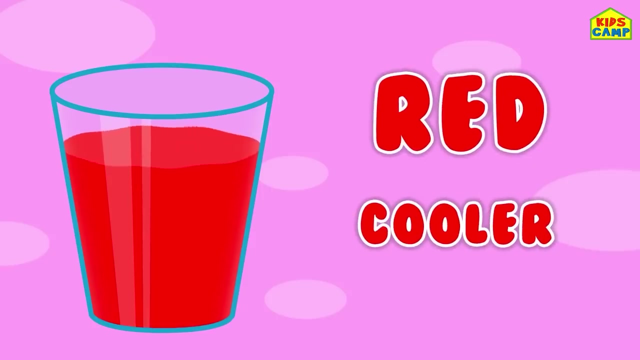 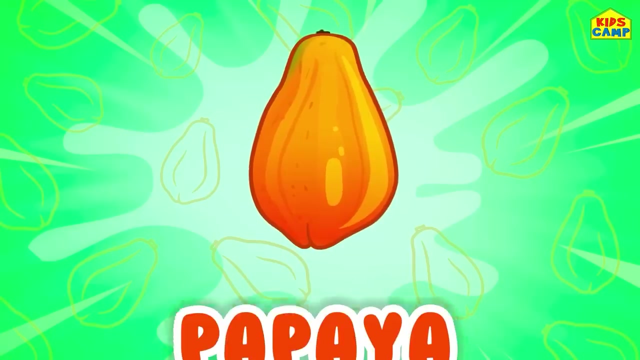 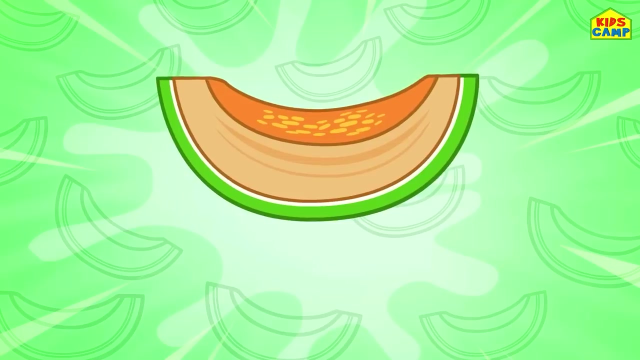 A scrumptious apple, a yummy strawberry and a juicy watermelon. Let's blend them up. Yay, A red cooler. Let us give them another go. I'm going to take a yummy papaya, an orange and a juicy melon. 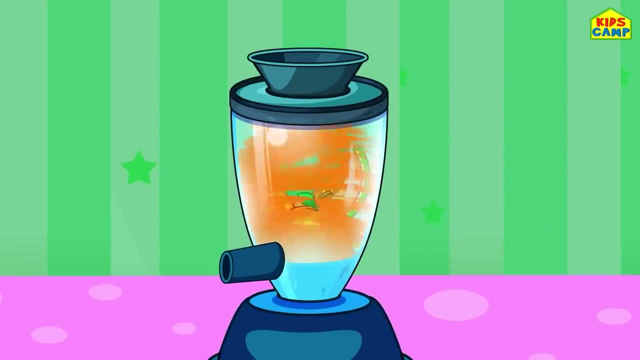 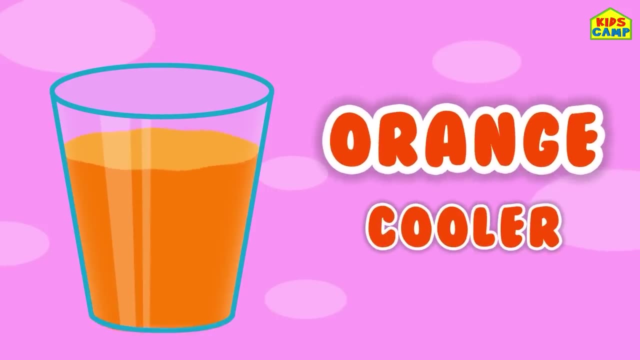 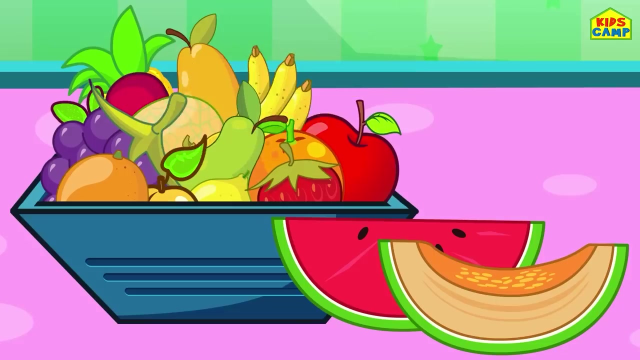 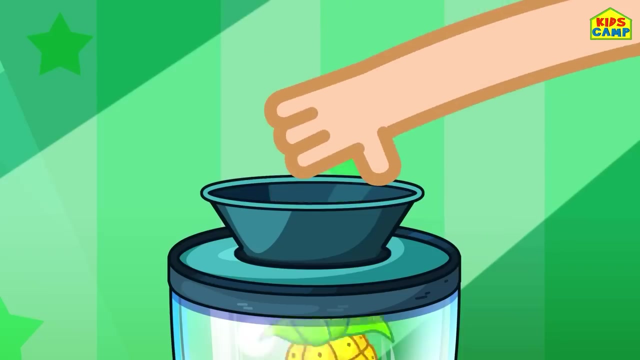 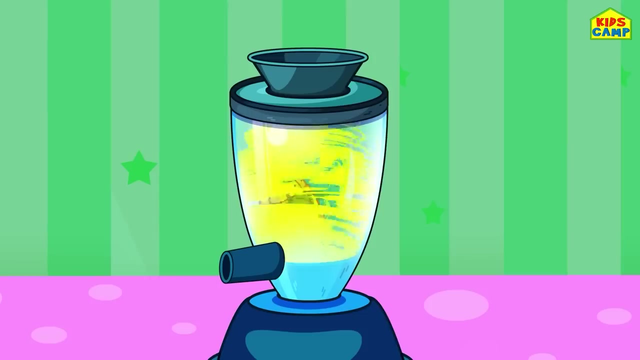 In they go, Let's mix them up. Woohoo, An orange. cooler, Let's try another one. This time I'm going to take a banana and a pineapple and a yummy mango. Woohoo, In they go, Let's mix them up. 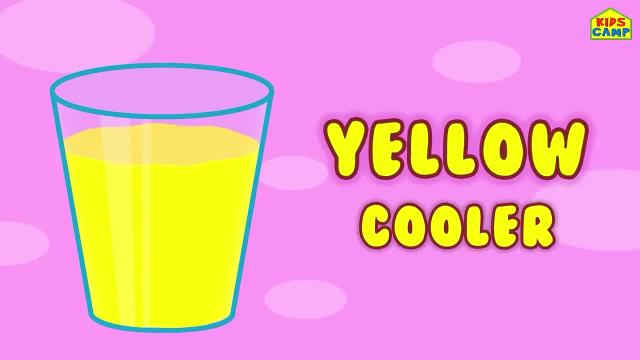 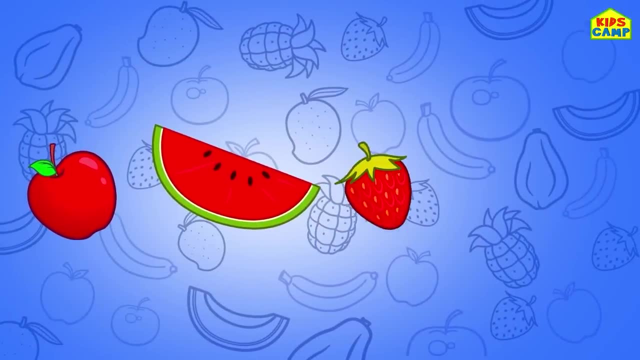 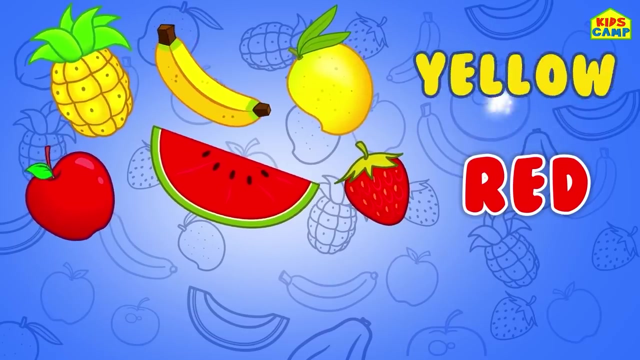 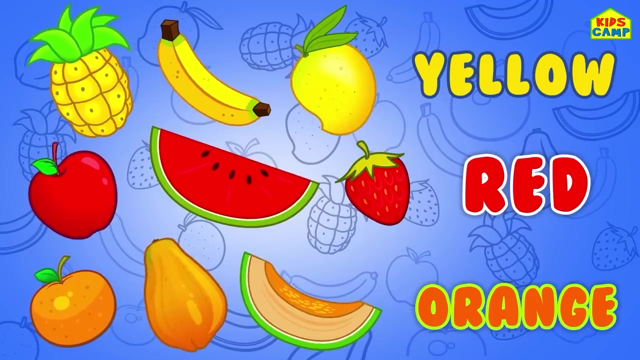 A yellow cooler. Wow, Today we learned that apples, watermelons and strawberries are red Mangoes, bananas and pineapples are yellow Oranges, papayas and melons are orange in color. Yay, We had a fun learning day. 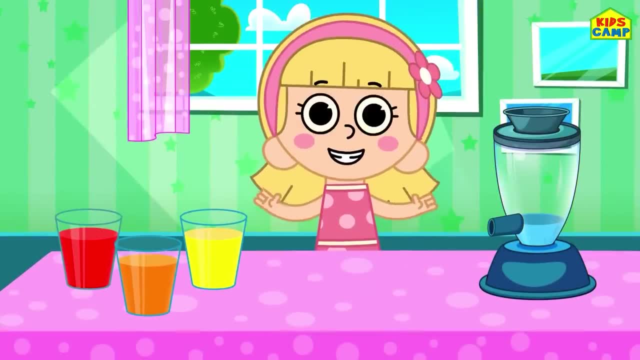 And delicious summer Coolers to drink. Yay, Hi, I'm Ellie, And today we are going to play a fun game with colors. That's right, we all love colors, Don't we? We have to find all the different types of colors as mentioned on the buckets. 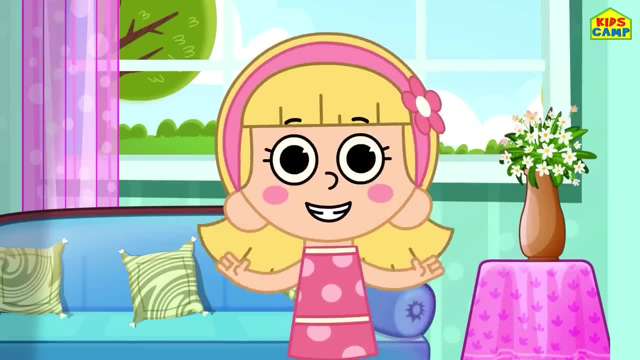 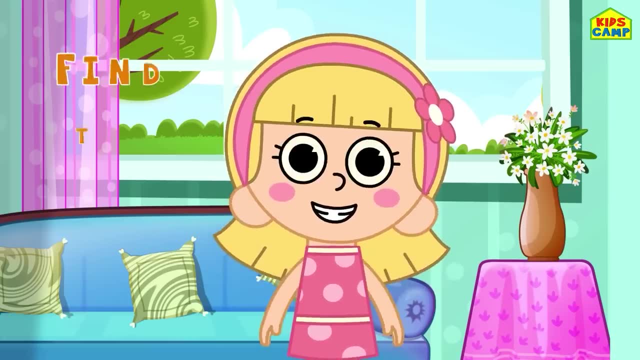 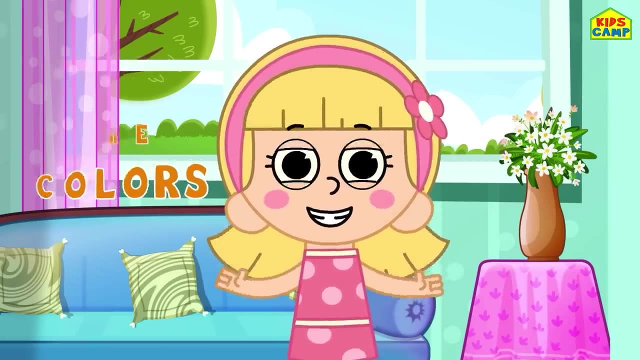 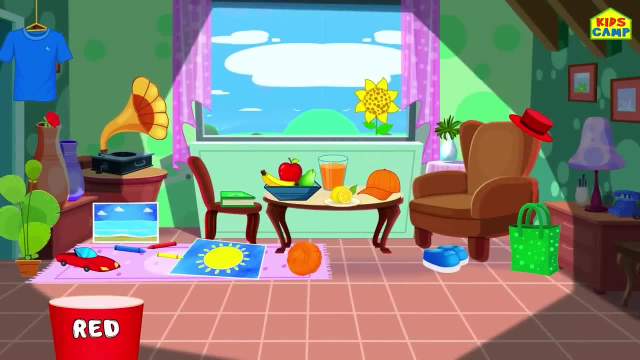 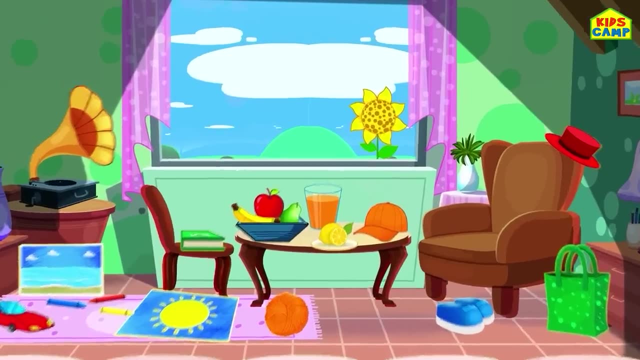 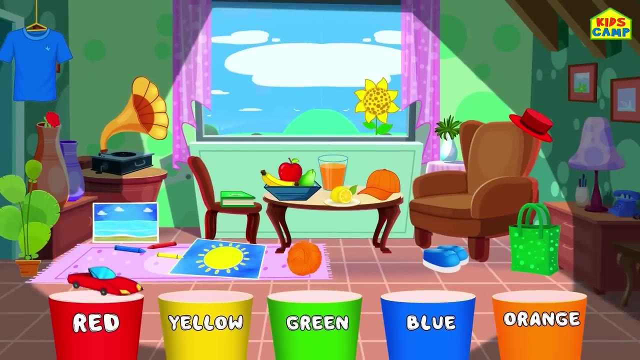 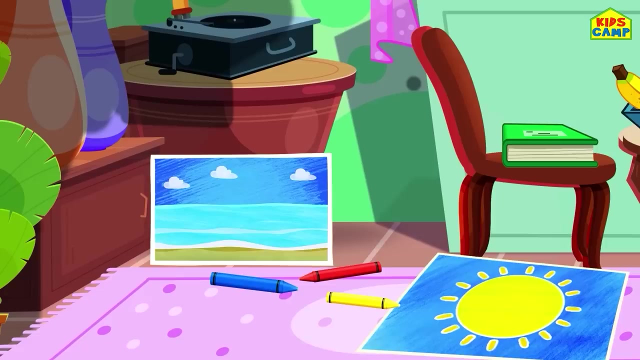 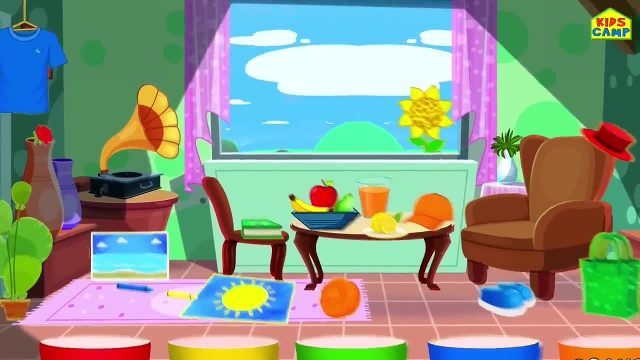 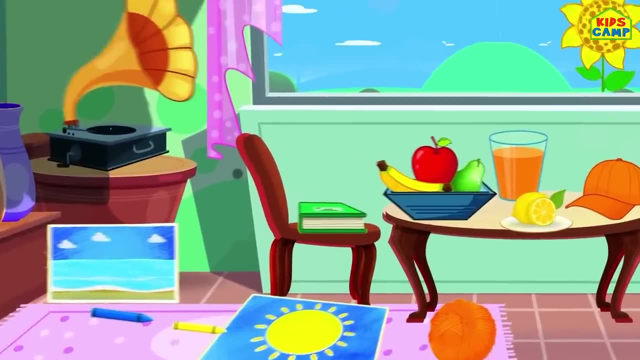 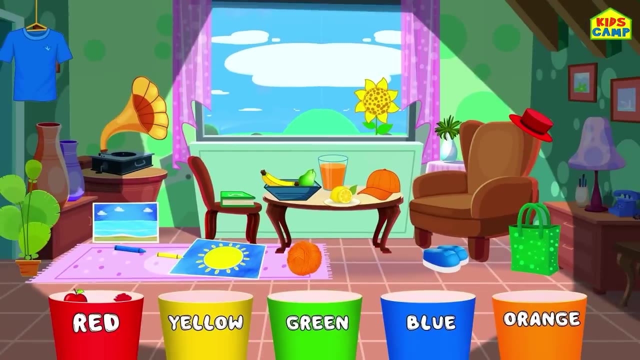 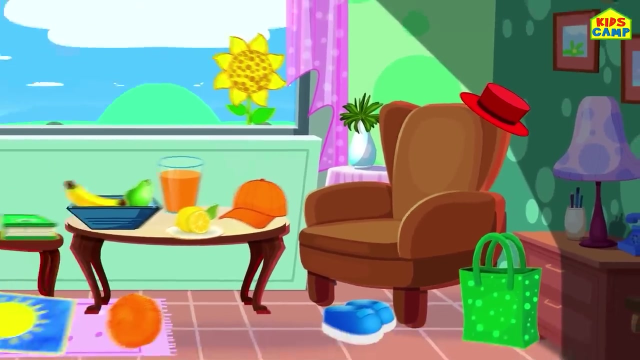 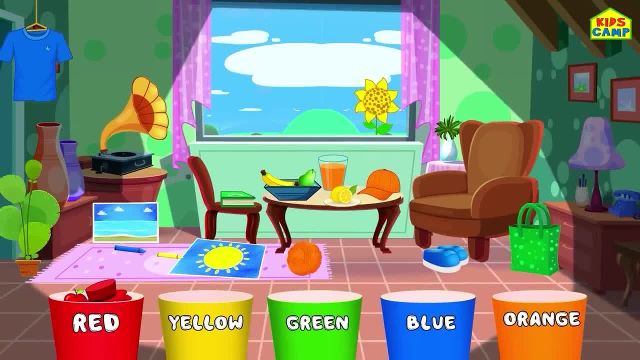 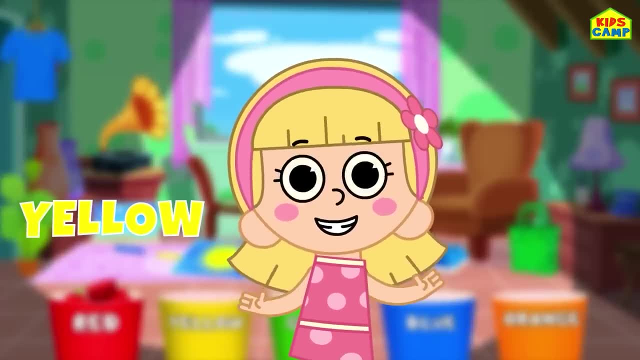 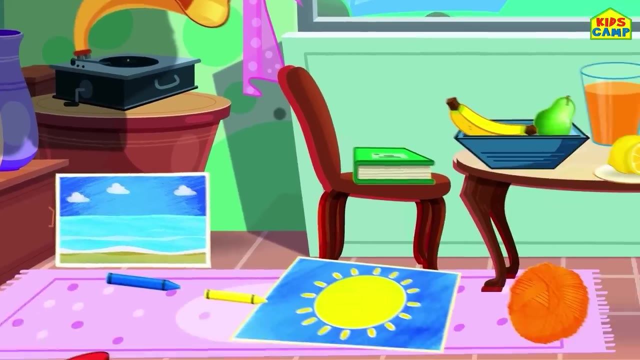 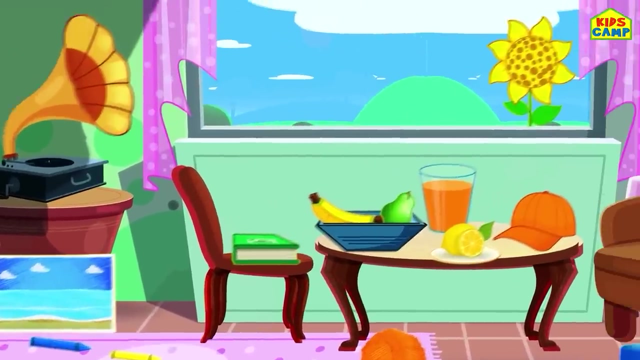 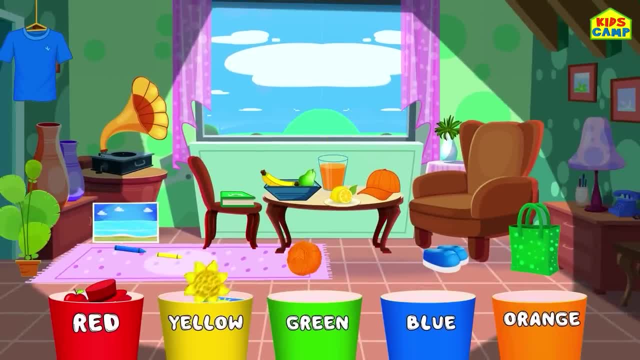 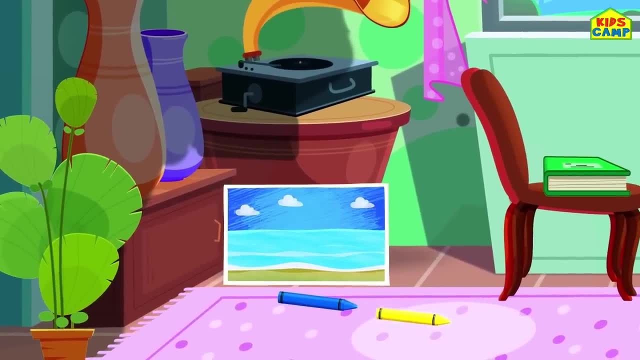 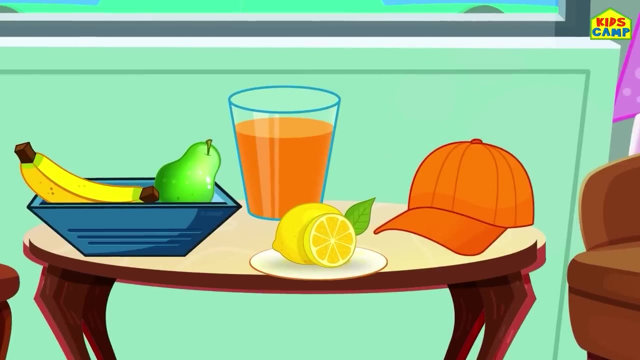 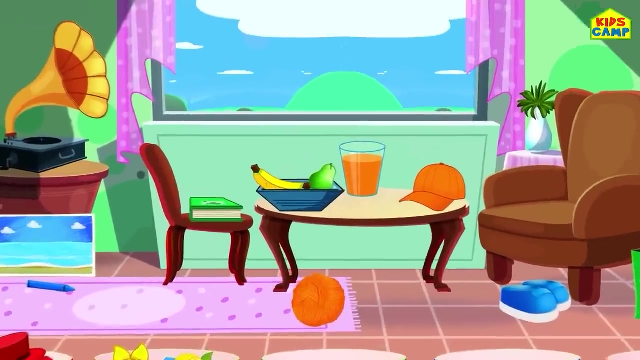 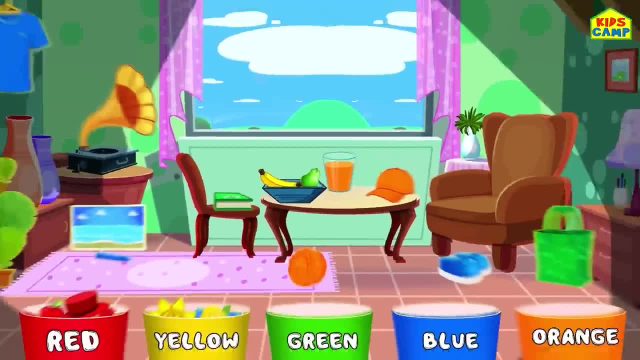 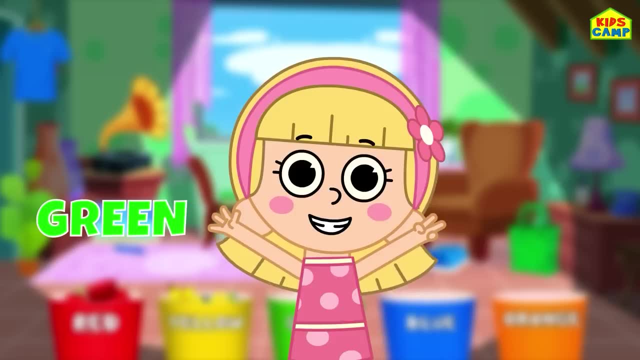 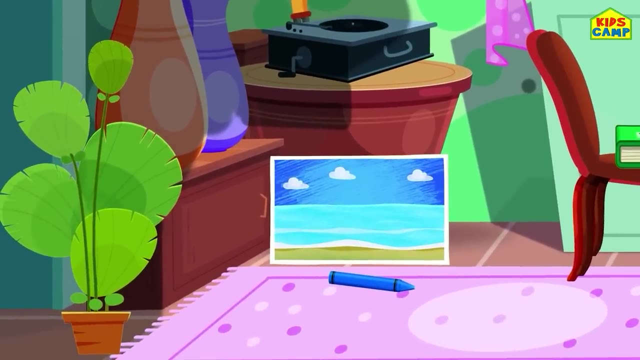 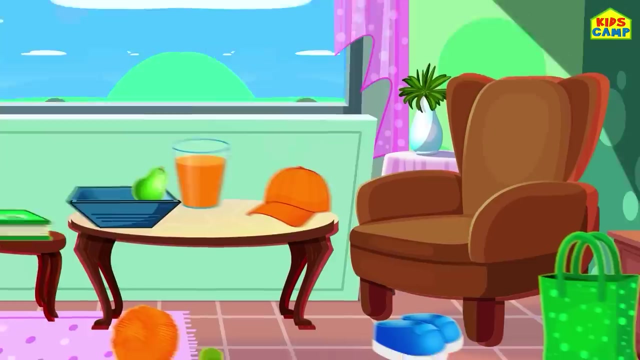 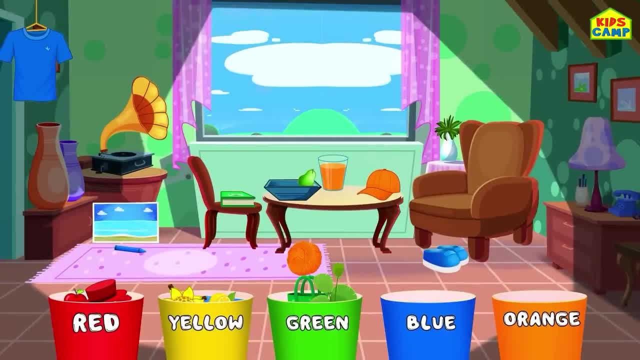 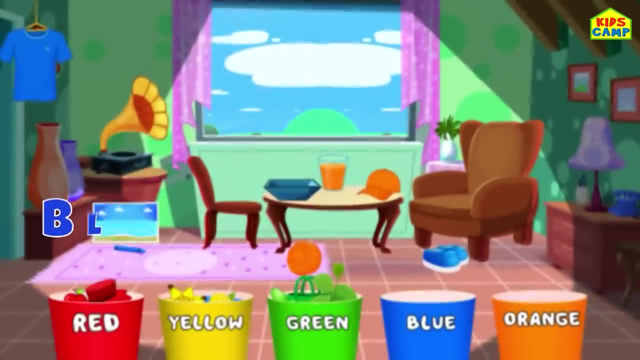 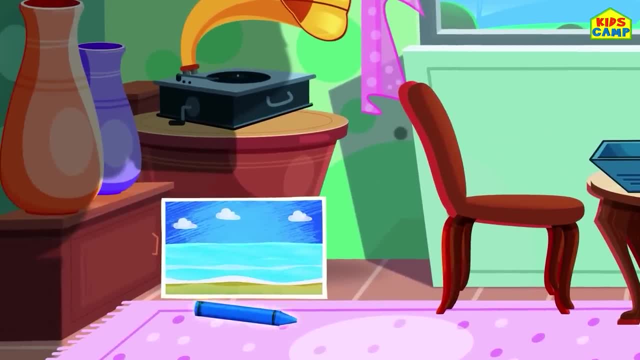 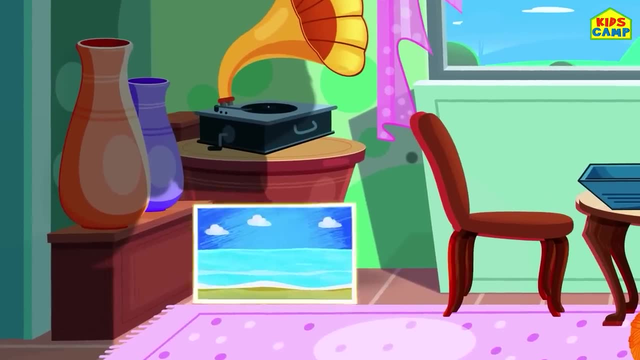 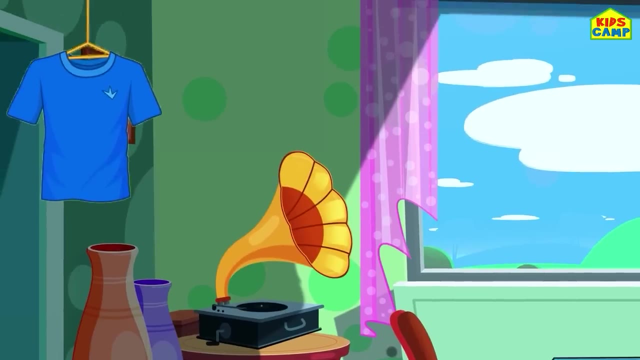 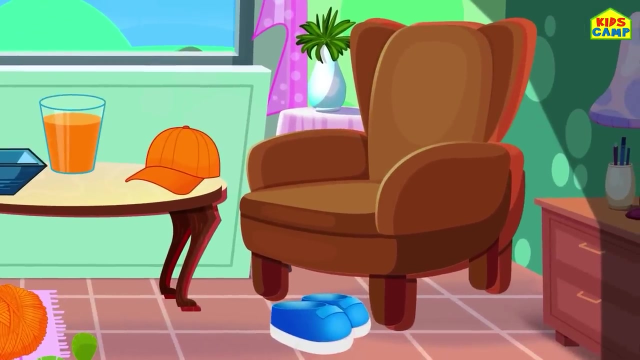 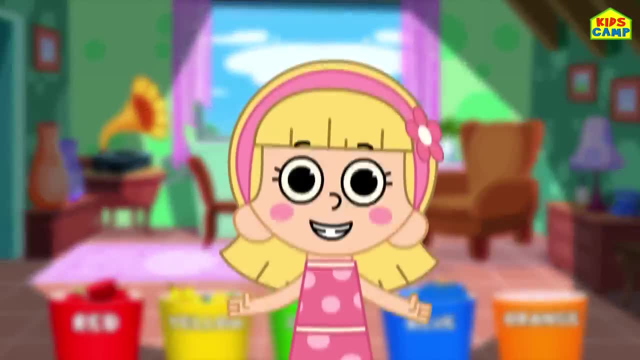 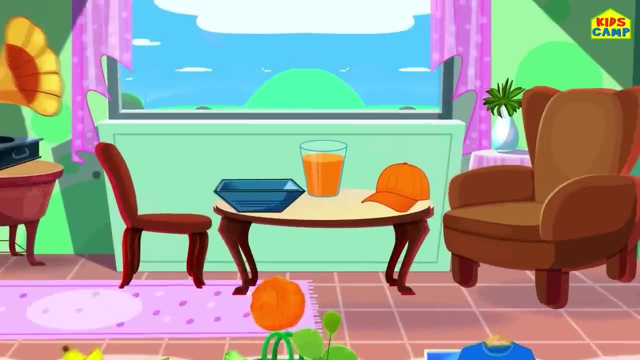 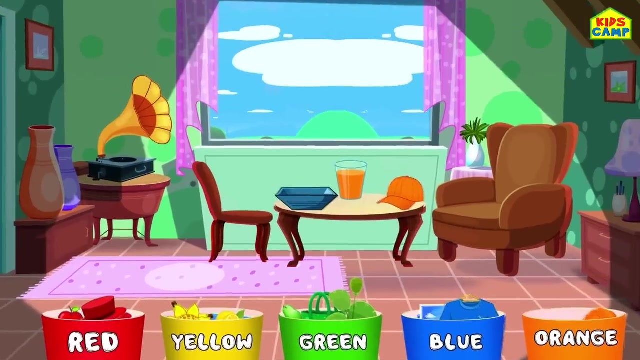 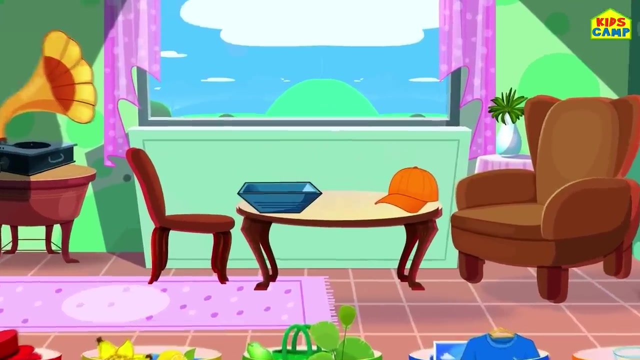 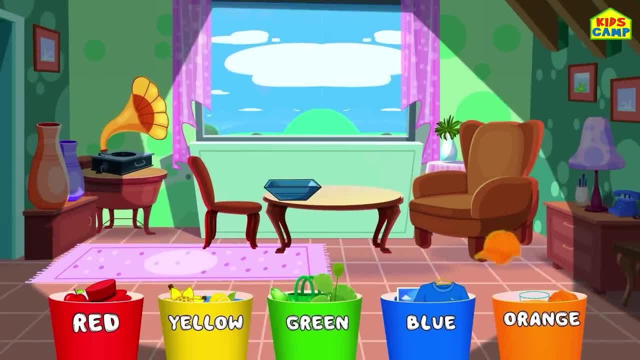 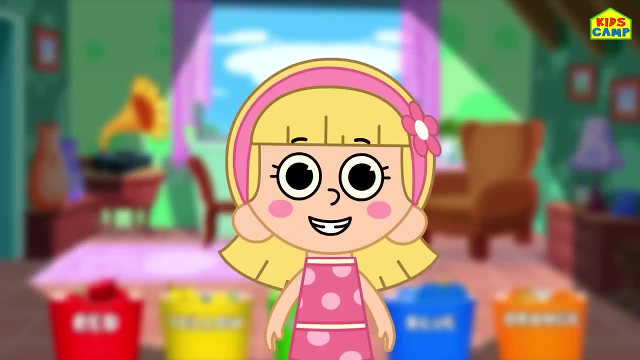 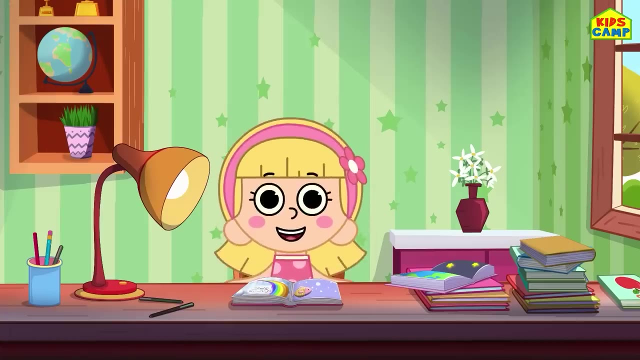 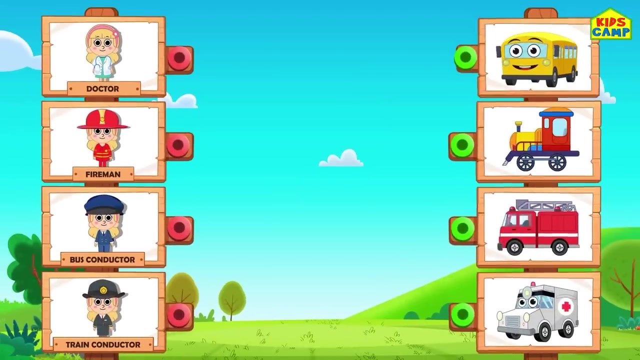 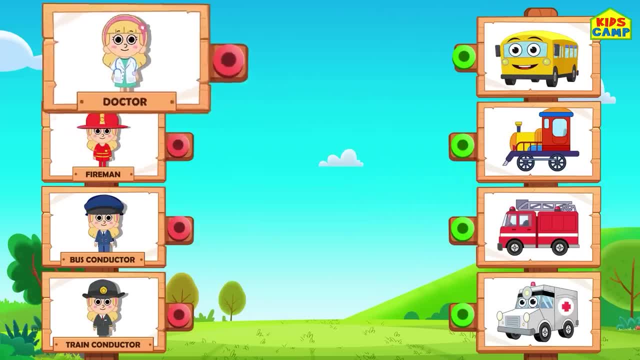 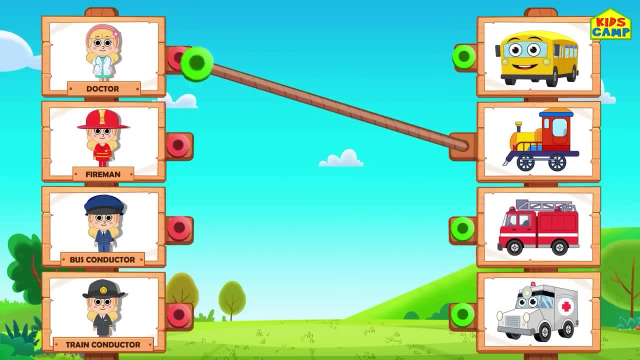 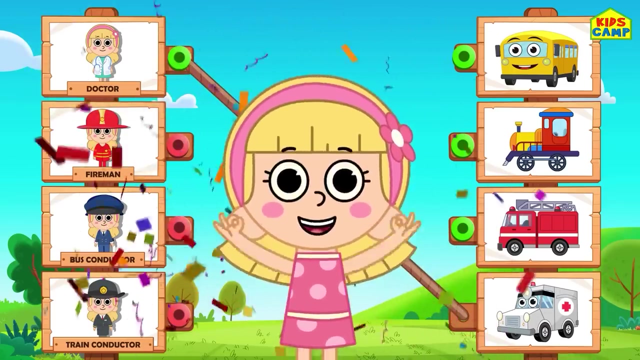 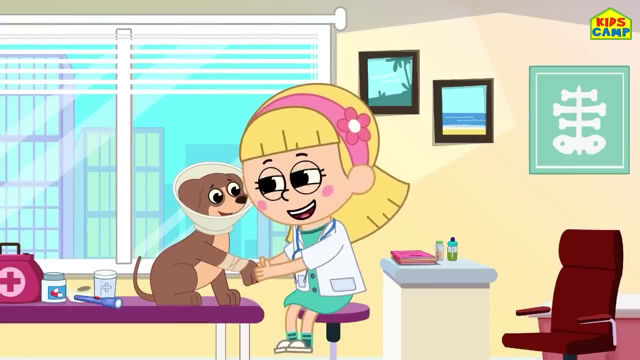 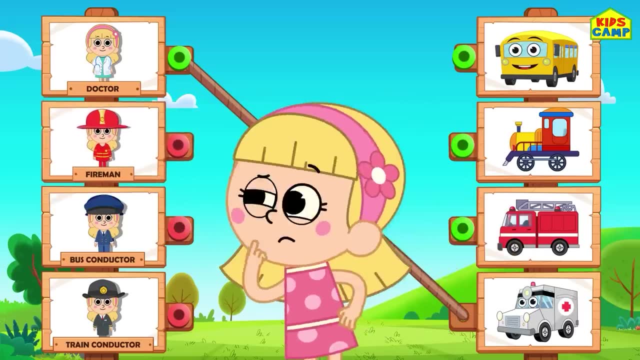 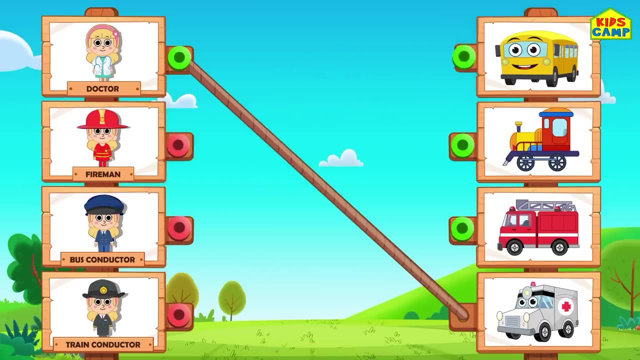 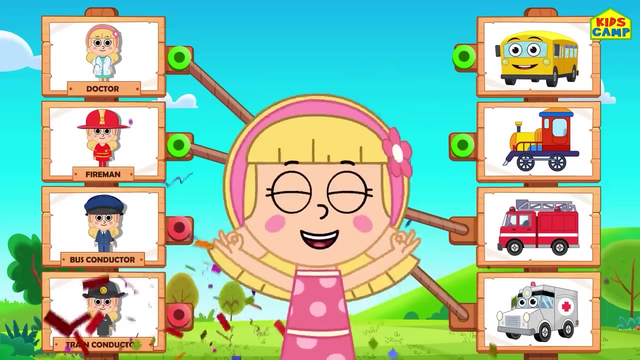 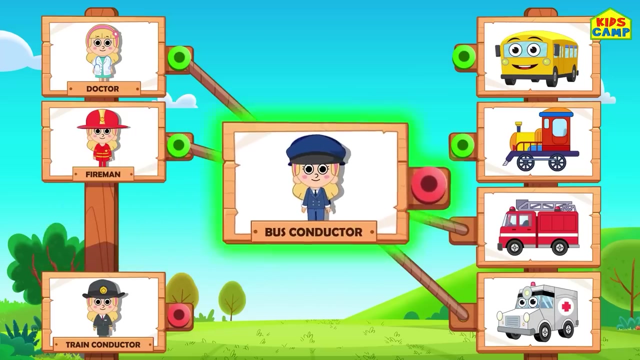 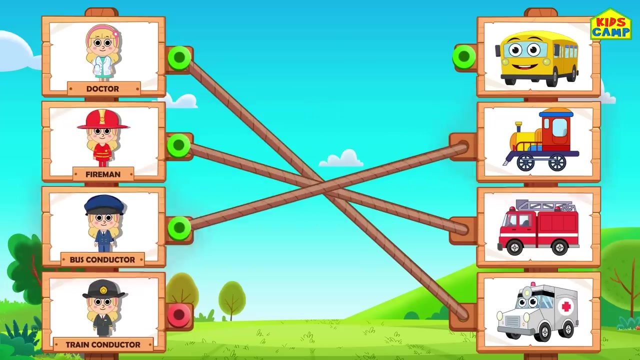 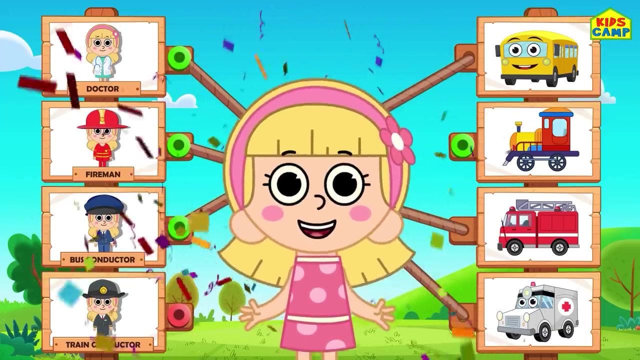 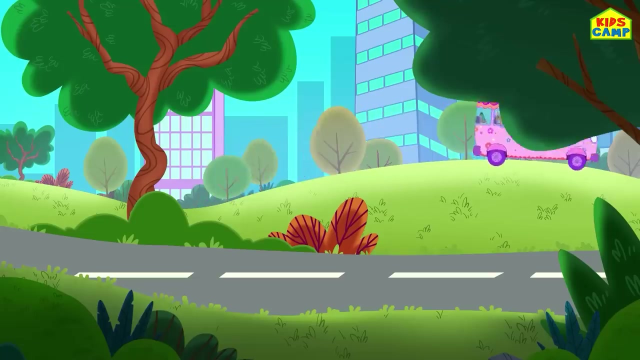 Red Red. A Firefighter will use which vehicle? a bus? no, no, a firetruck, that's right. A bus driver will use a train, no a bus, that's right. Good job, friends, Yay. 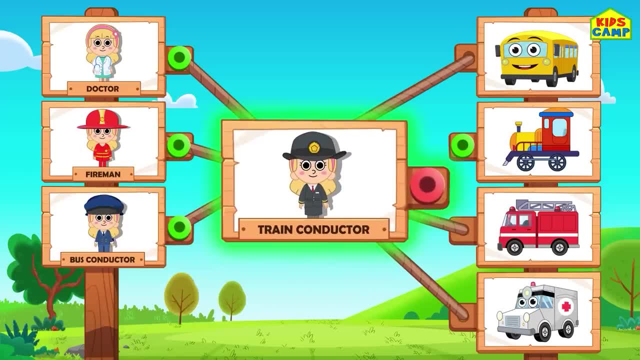 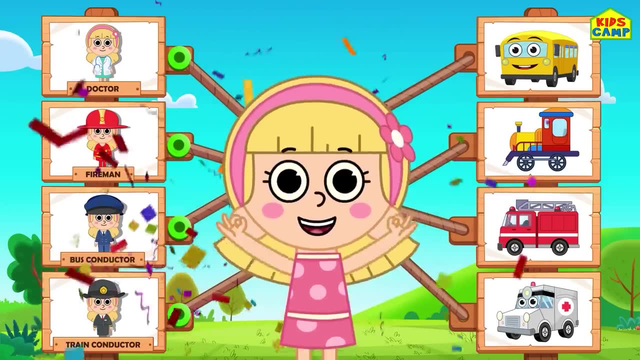 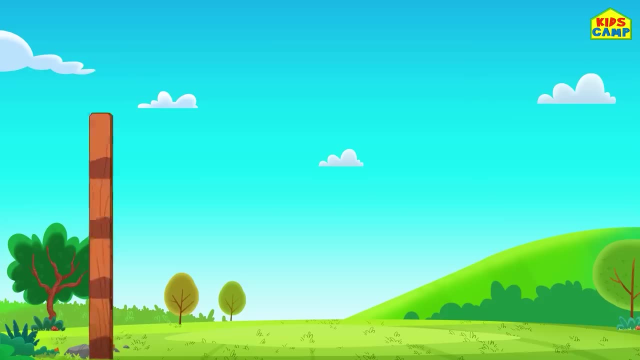 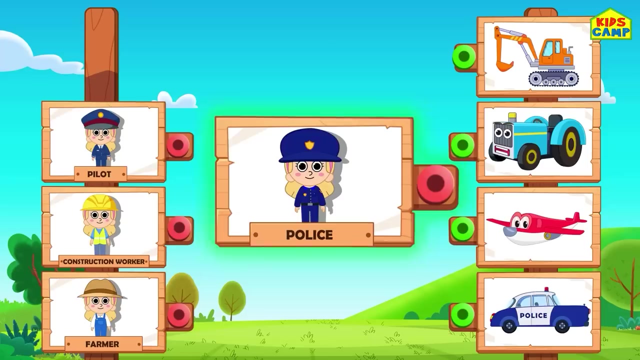 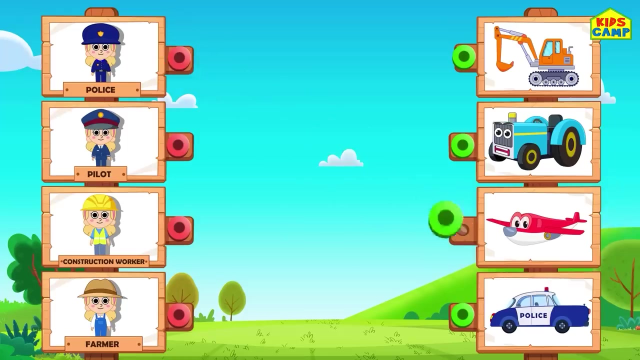 What's next? A train conductor? Which vehicle will he use? The train? That's right, All aboard? Ooh, Which vehicle will the police use? An airplane? No, A tractor? No way. Hmm, I know A police car. 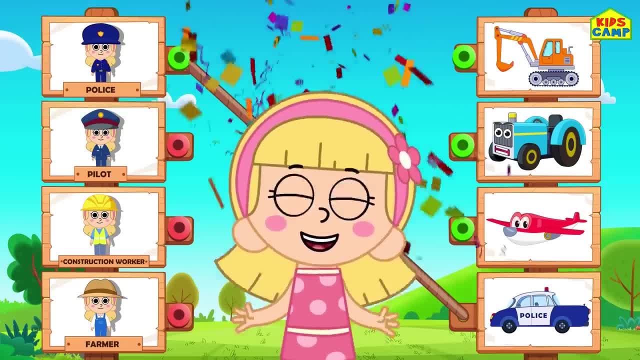 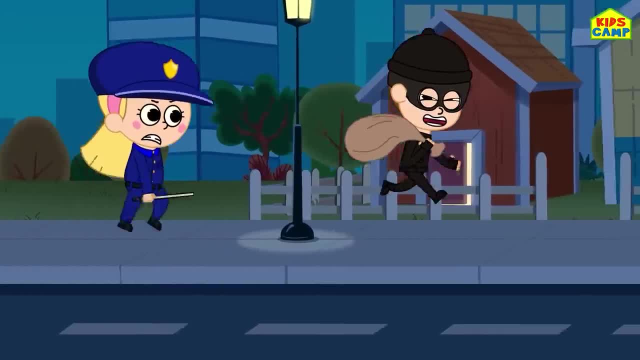 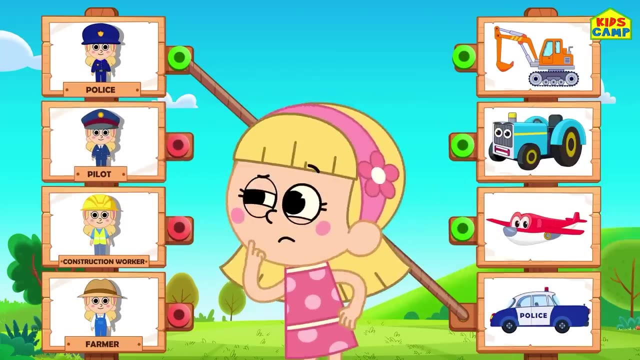 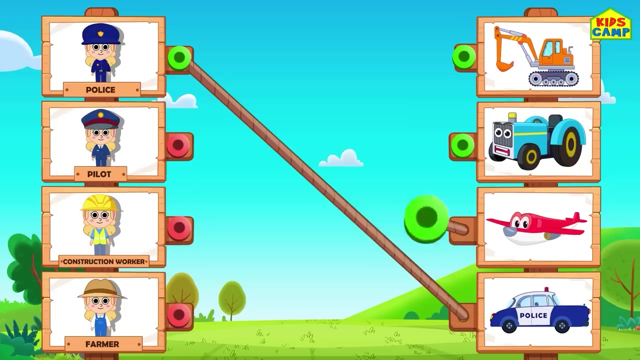 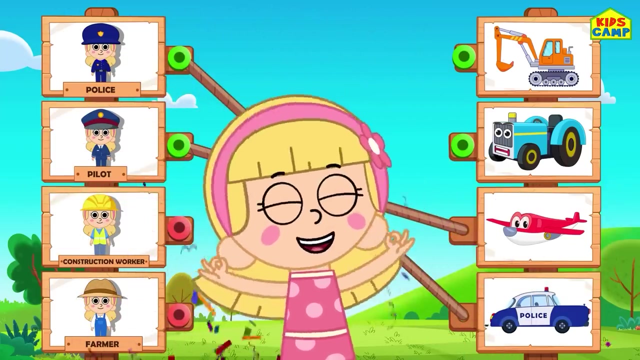 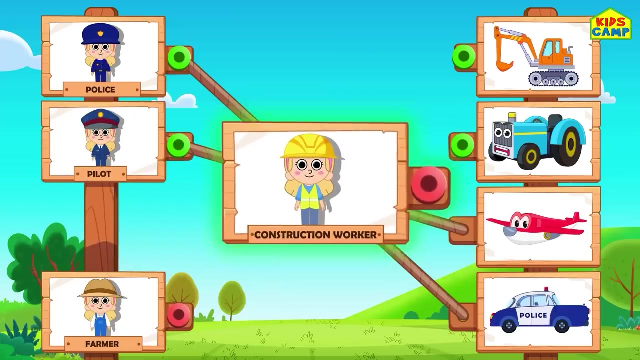 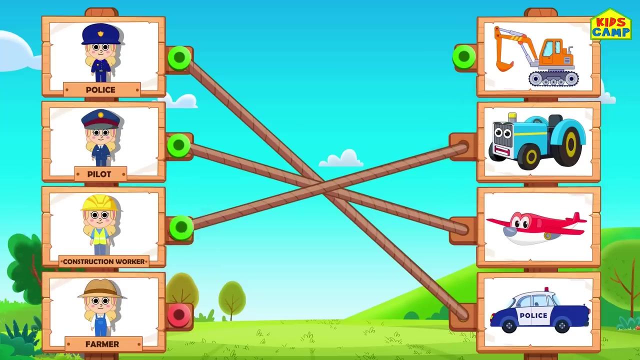 That's right. Yay, A pilot will use which vehicle? Hmm, A digger- No, An airplane. Yes, Fly away. Yay, A construction worker will use which vehicle? A tractor- No, A digger. 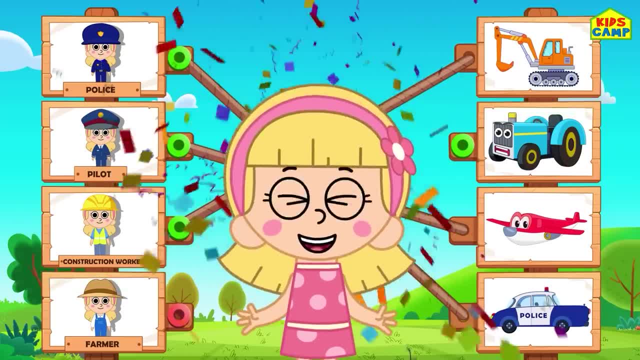 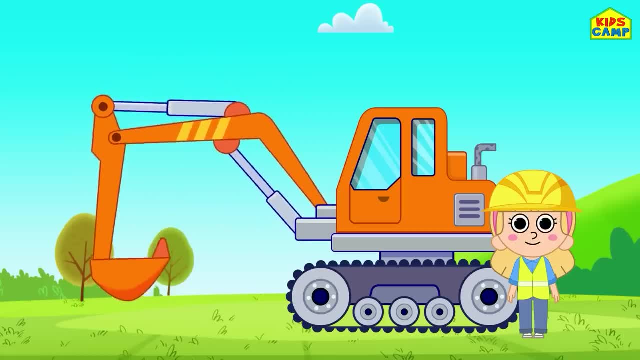 That's right, Yay. What vehicle will a farmer use? A tractor, That's right, Yay, Super. A tractor, That's right, Yay, Super, Yay, Yay, Yay, Yay Yay. 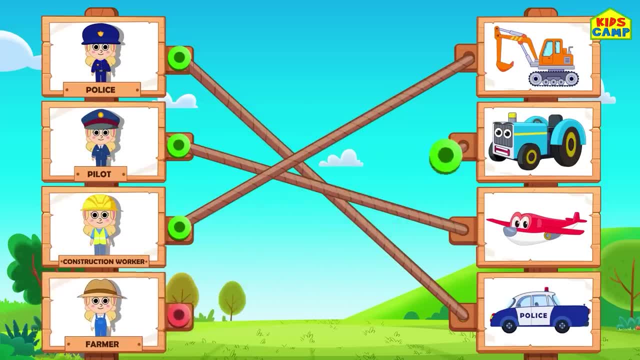 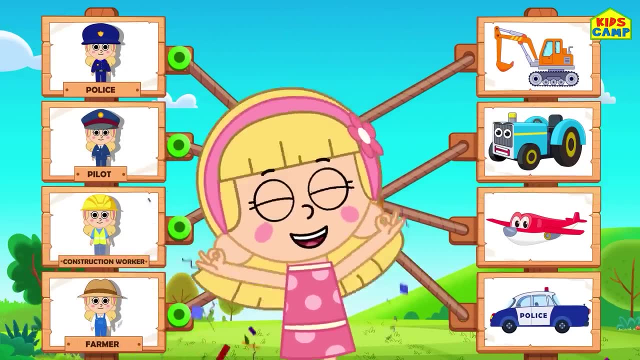 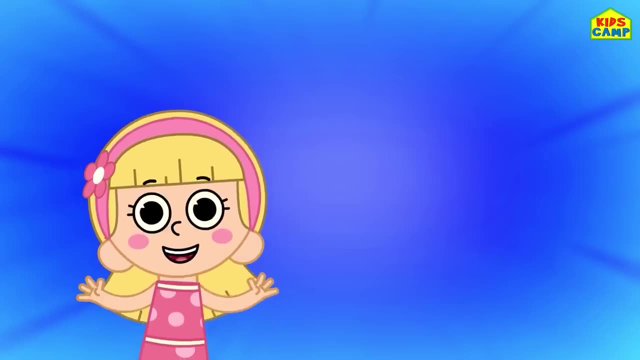 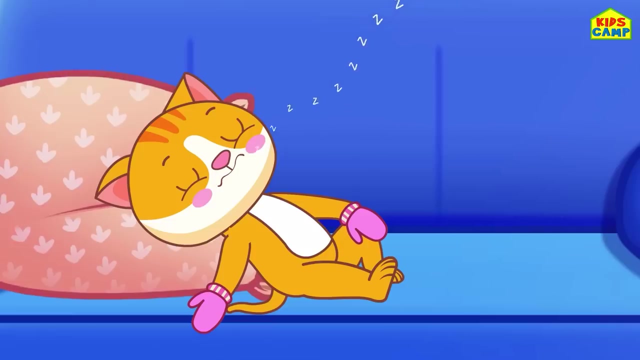 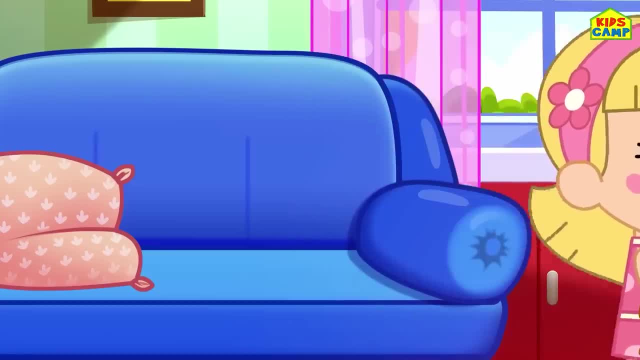 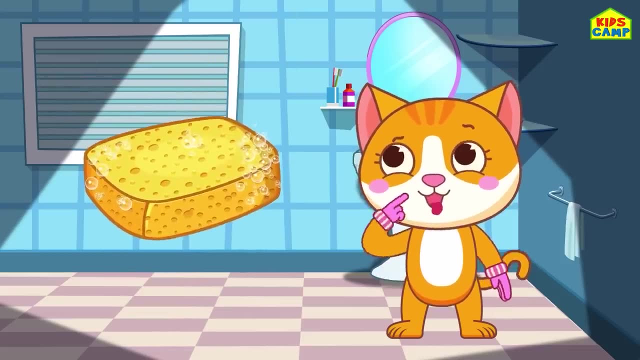 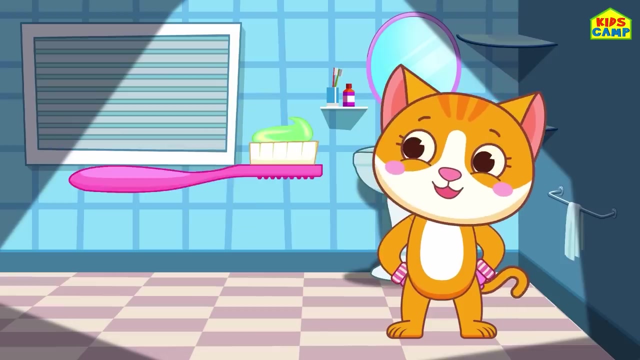 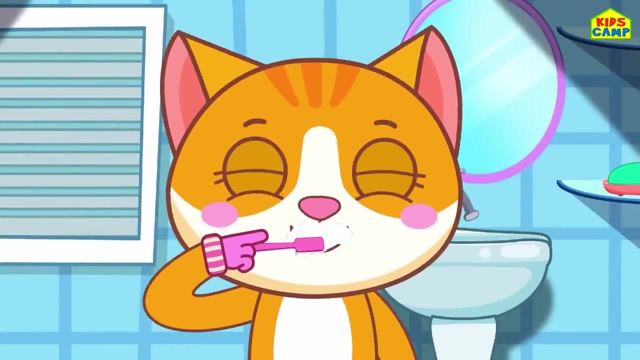 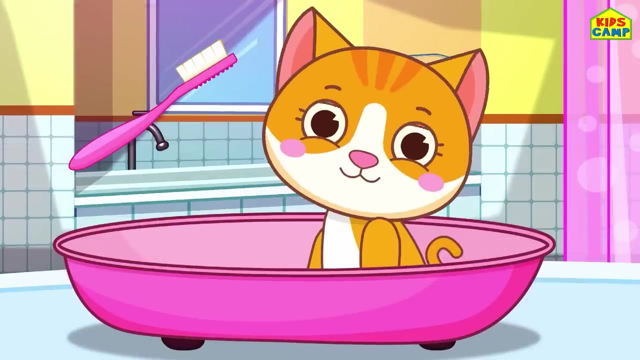 Let's brush your teeth Ready. What do we brush your teeth with? is this a toothbrush? no, is this a toothbrush? no, no. is this a toothbrush? yes, it is. Wow, your teeth are sparkling white. now let's have a bath. what do we have a bath with this one? no, this one definitely. 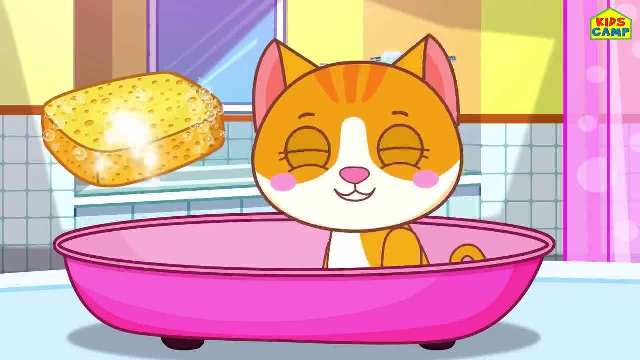 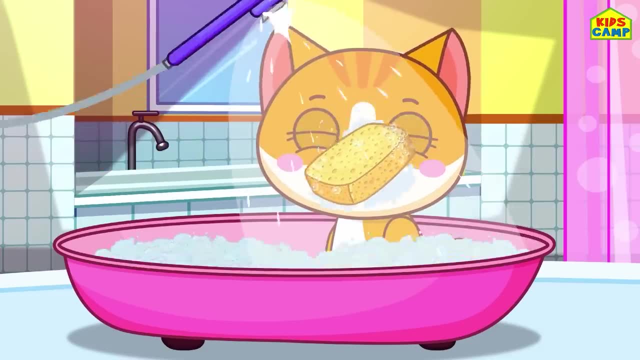 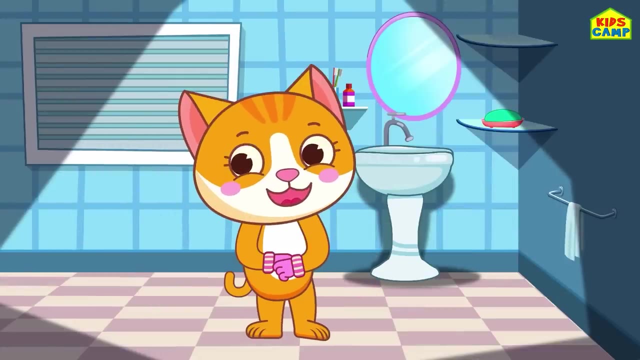 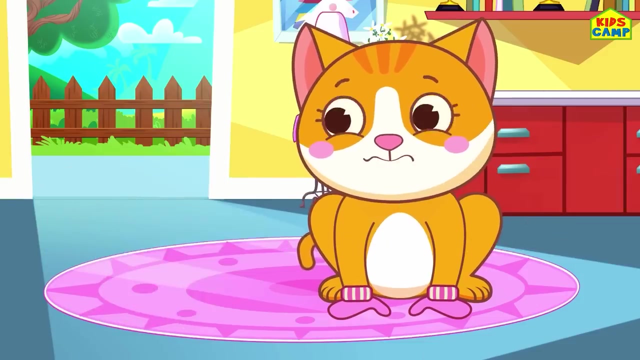 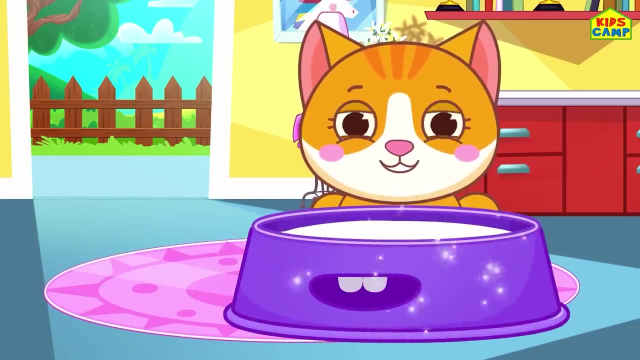 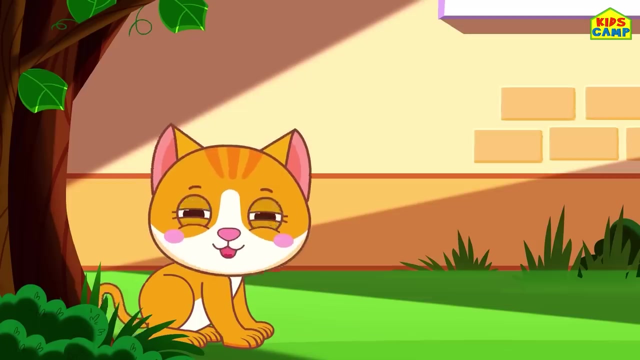 not. don't you love taking a bath? Wow, you're neat and clean kitty. now let's have breakfast. what do we have for breakfast? this one, no. this one, no, no. then let's have milk. yes, milk is good. don't you love drinking milk? now let's play. what do we play with this? no, it's a broccoli. 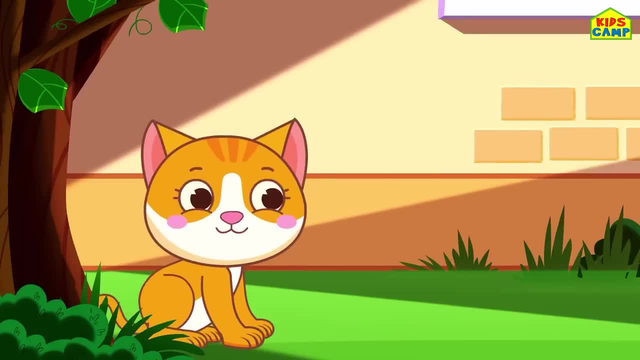 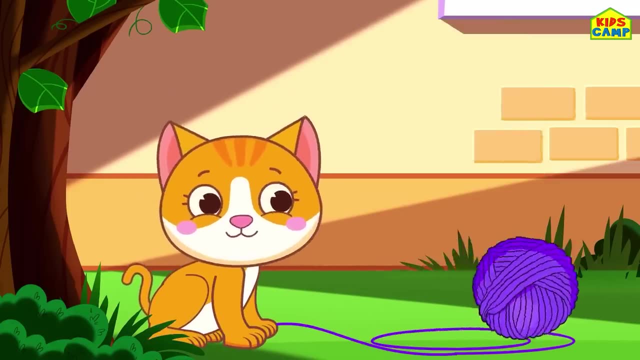 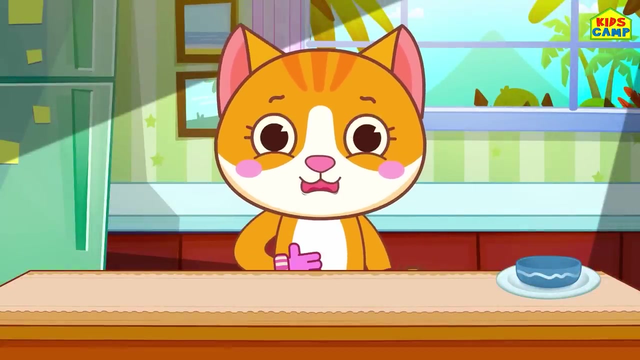 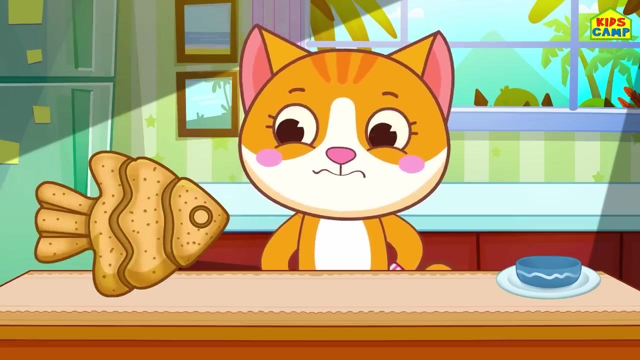 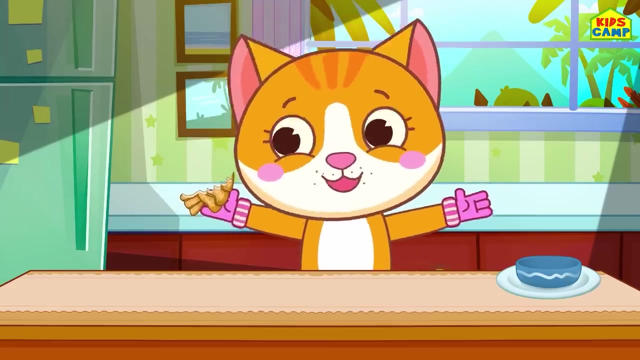 no, we can't play with this. it's a candy. yes, we can play with this, it's a ball of string. wow, so much fun. now let's eat something. are you hungry? can you eat this? no, can you eat this, no, no. yes, you can eat this. don't you love the fish biscuit- yummy. 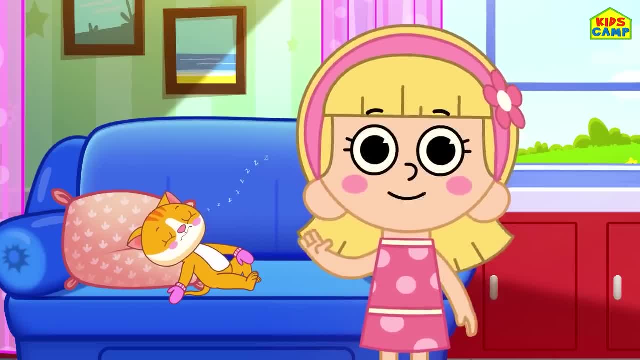 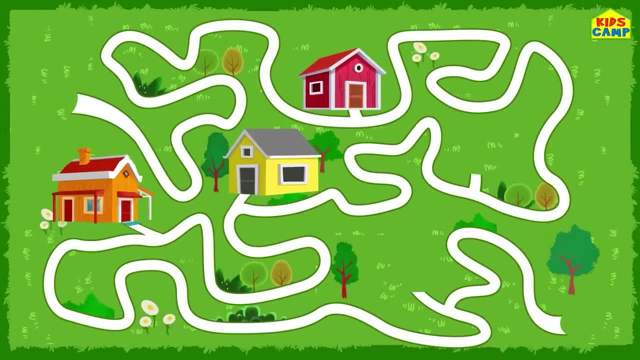 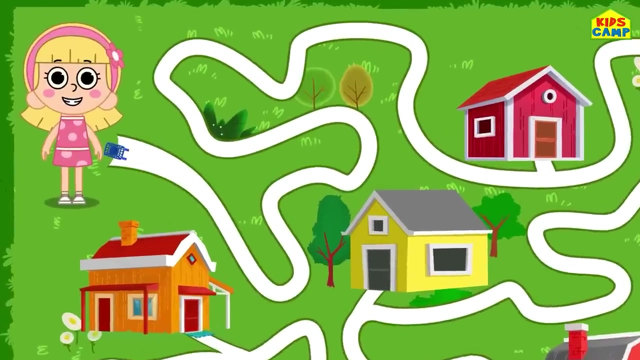 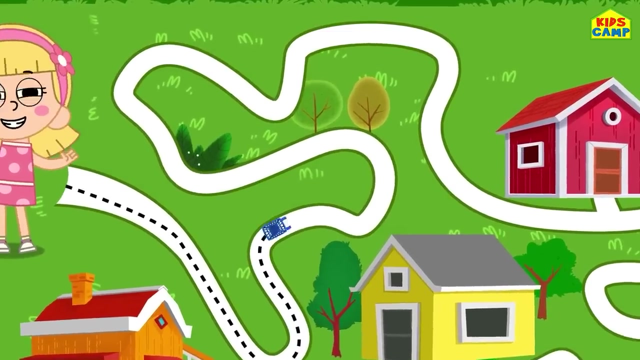 wasn't it a fun day with my kitten. see you soon. bye, bye, hi. I'm Ellie and I have to collect all the fruits into the basket. that's right. here goes my card, let's collect fruits. here goes my card, let's collect fruits. here goes my card, let's collect fruits. 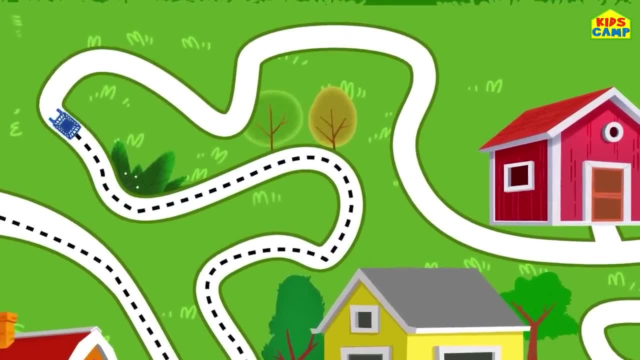 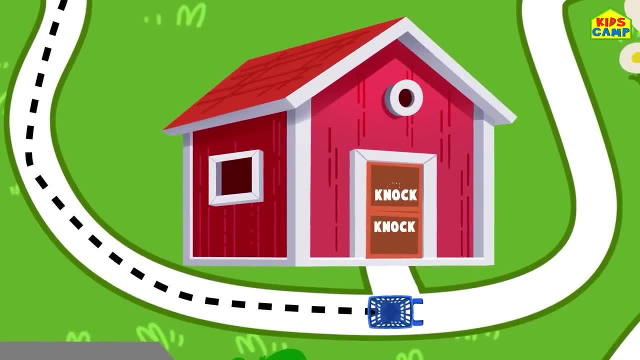 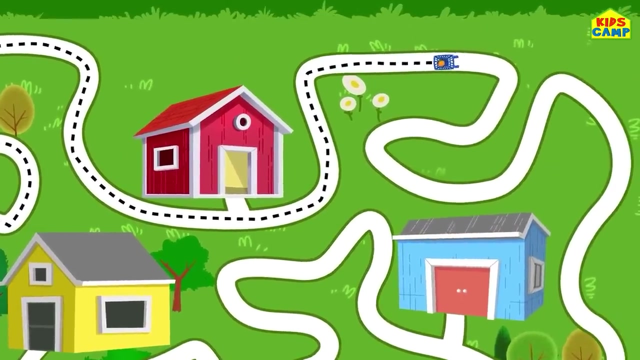 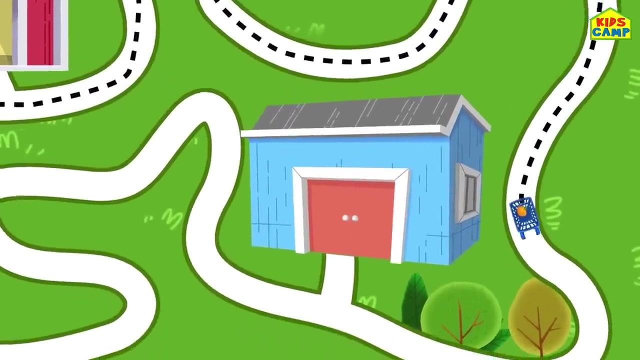 let's collect fruits. let's collect fruits. let's collect fish. hi, do you have any fruit? park into my kart, let's keep going. ooh, let's keep going. oops, oops, oops, oh wow, oh wow. let's see some of the fruits in the forklift ride. let's collect all the fruits. 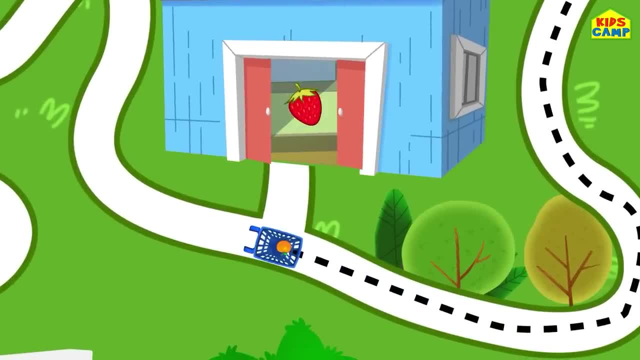 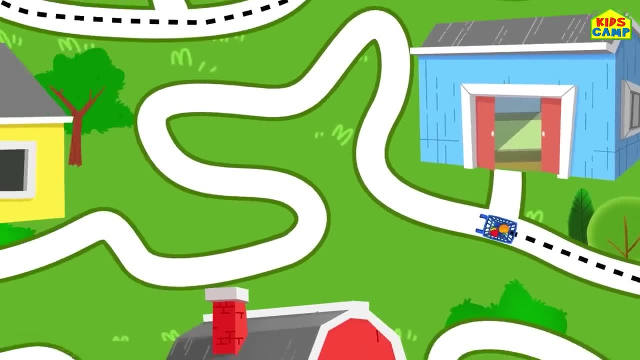 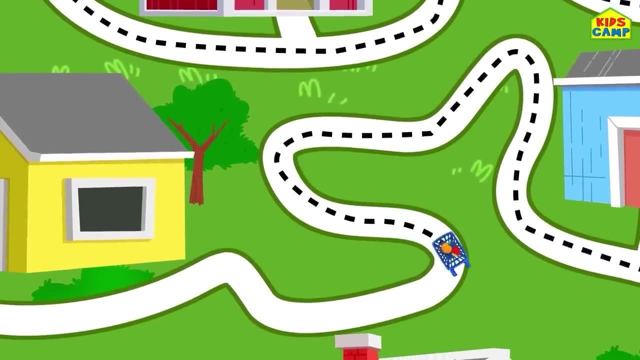 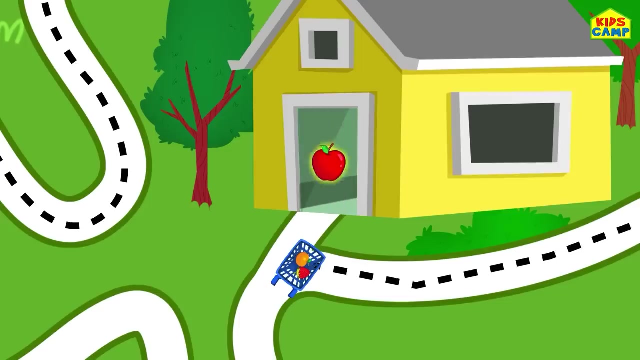 hi, hi, Knock knock. Do you have any fruit? Aha, A strawberry Into the cart. Wonderful, Let's get going. Knock knock, Hi, Do you have a fruit? Oh, My favorite, An apple, Oh, Into the cart. 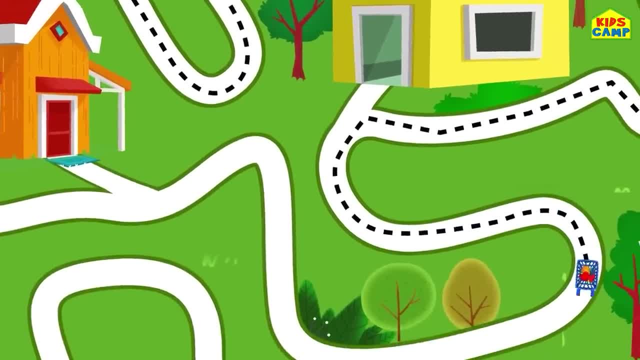 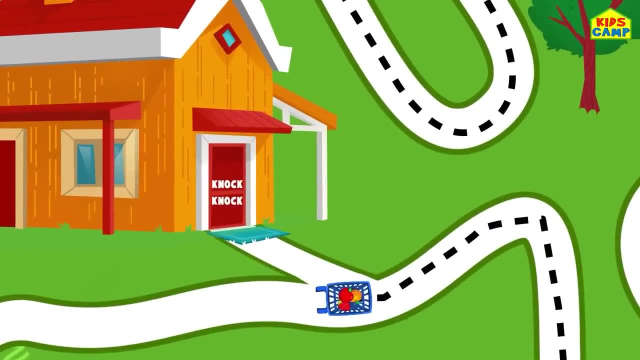 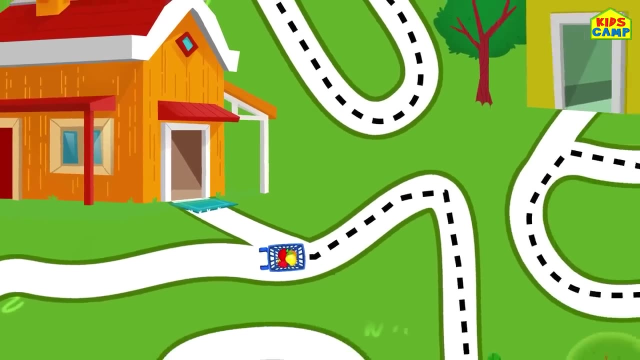 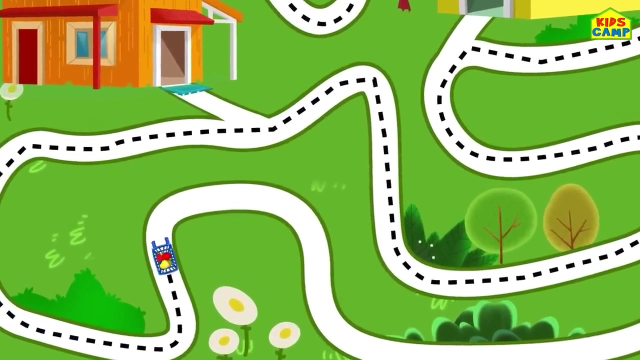 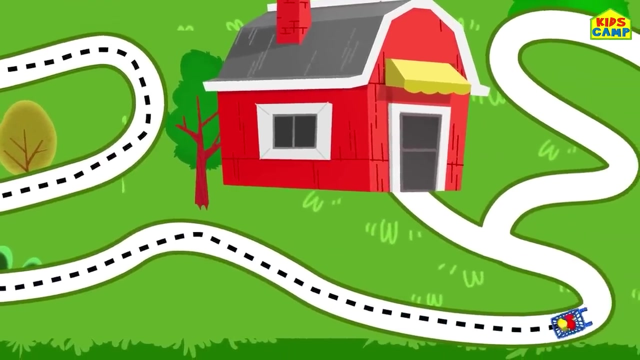 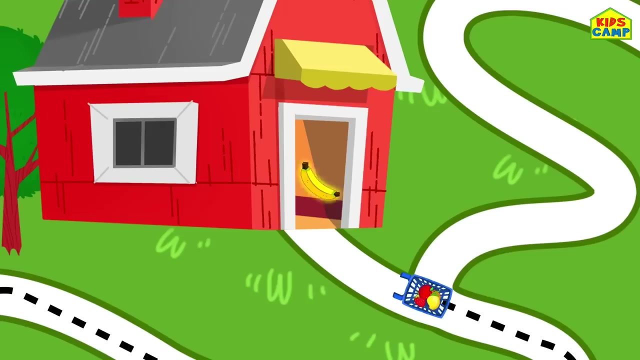 Yay, Let's keep going. Knock knock. Do you have some fruit? Oh, A mango Into the cart, Let's get some more. Keep going, Knock knock. Hi, Do you have some fruit? A banana, Yay, Into the cart. 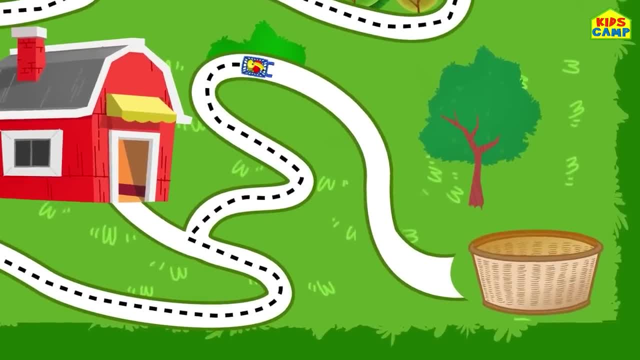 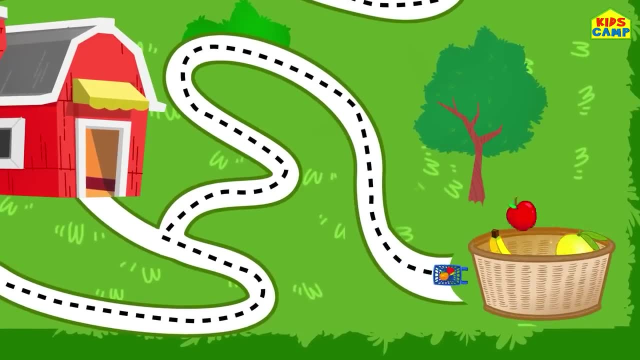 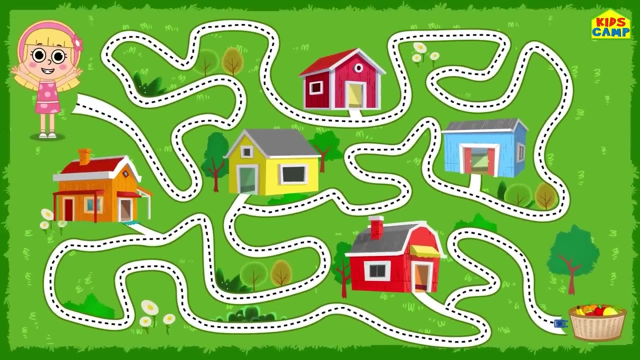 Let's keep going. Yay, We've collected all our fruits. What did we get? A banana, a mango, an apple, a strawberry and an orange. Good job, Thank you so much for helping me find my fruits and collecting them in my basket. 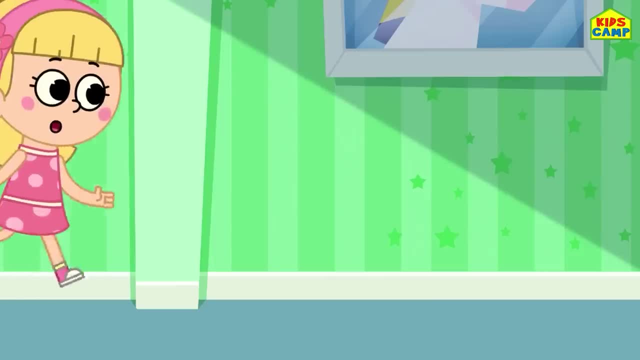 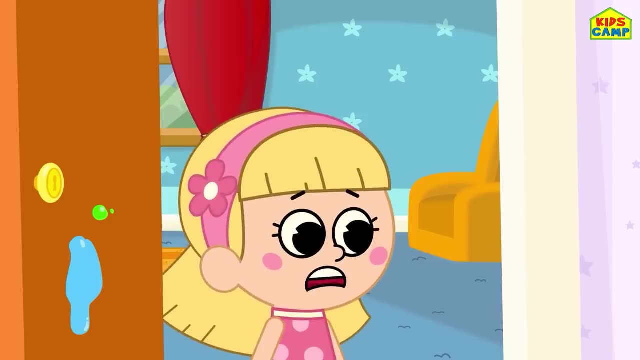 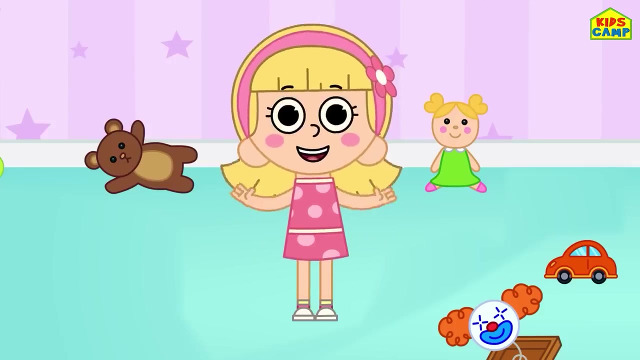 Thank you. Hi friends, I'm Ellie and this is Eva. Eva, Look at your room. You have to clean the room now. Wow, I know a fun way to clean our room. Let's find the objects and put them where they belong. 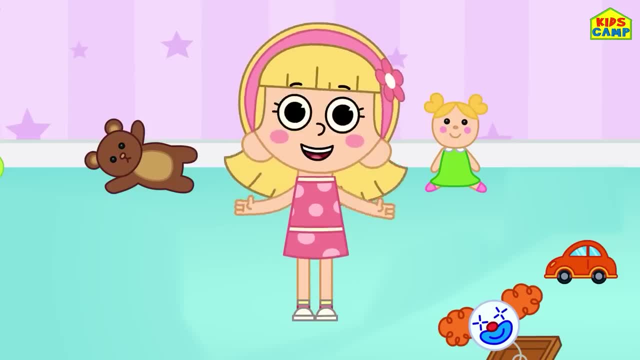 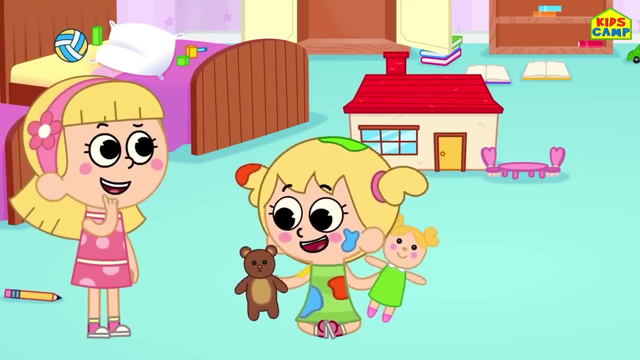 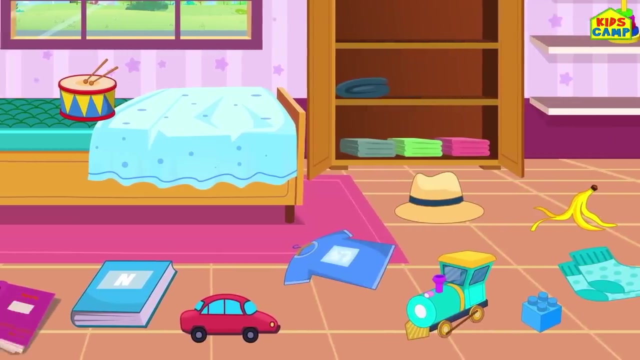 Eva, Let's clean our room. Let's do this. friends Ready, Let's get started. Yay, Come on, Eva. Eva, you know what you have to do. That's right. Yay, Yay, Yay. 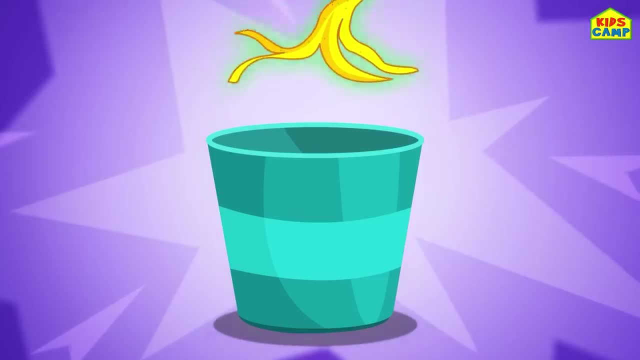 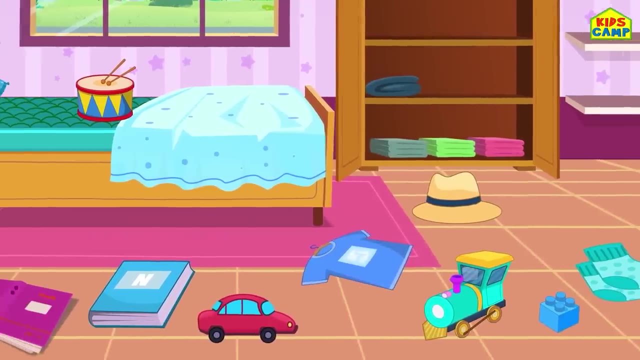 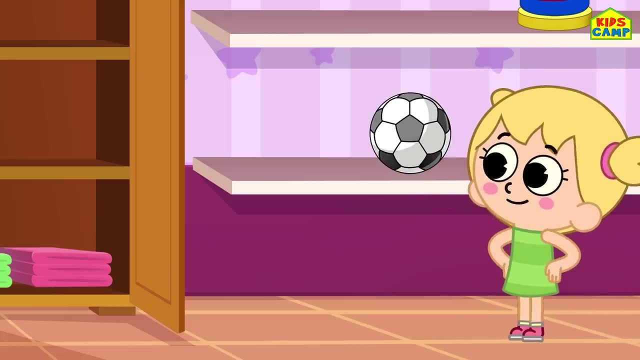 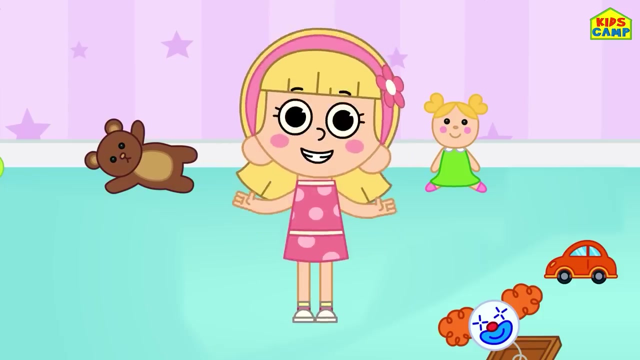 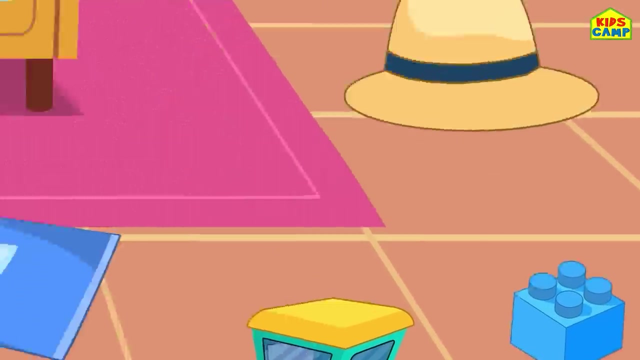 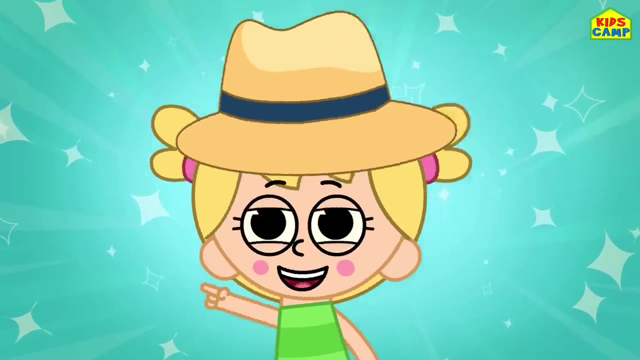 Yay, Yay, Yay, Yay. Very good, Let's clean some more. Let's look for the hat. Where is it? No, That's not a hat. No, That's a hat, That's right. 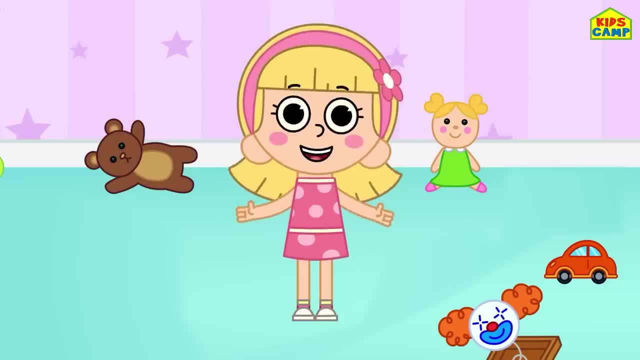 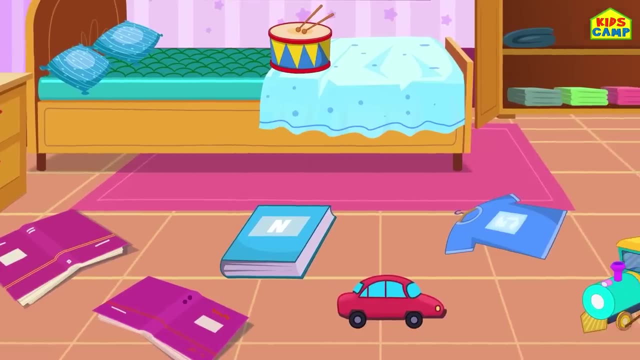 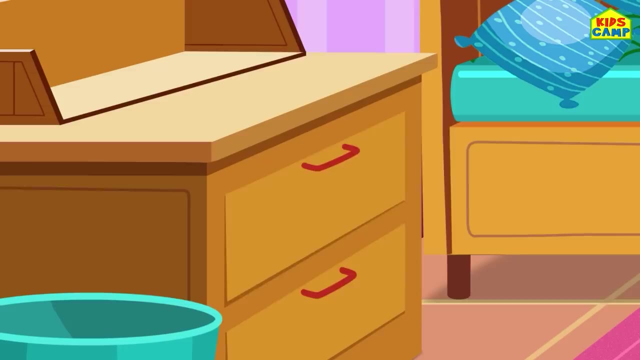 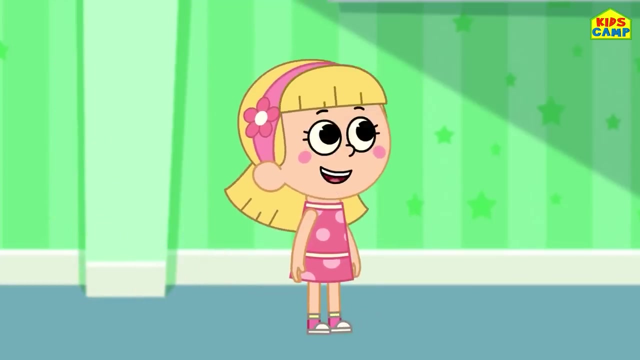 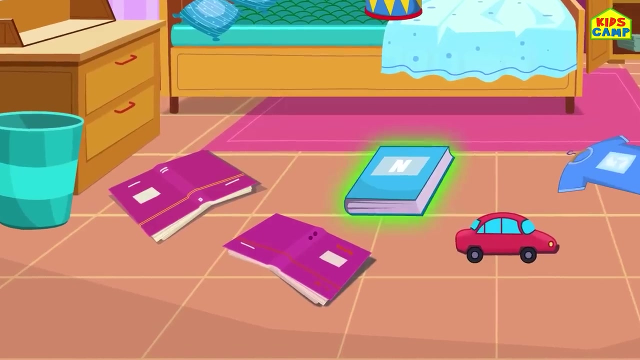 On to the shelves. Good job, Let's clean some more. Now. let's look for The socks. That's right Into the drawer. Wonderful, Very good. Eva. where are your books? Look for them, That's right. 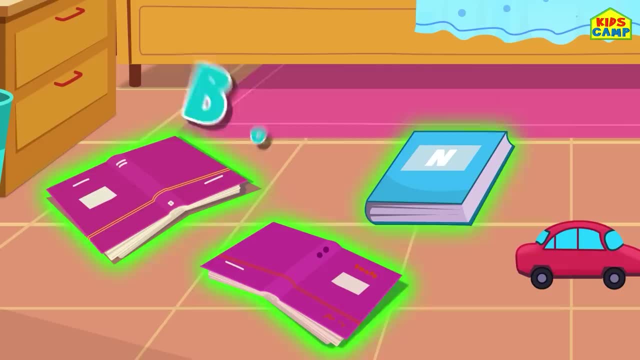 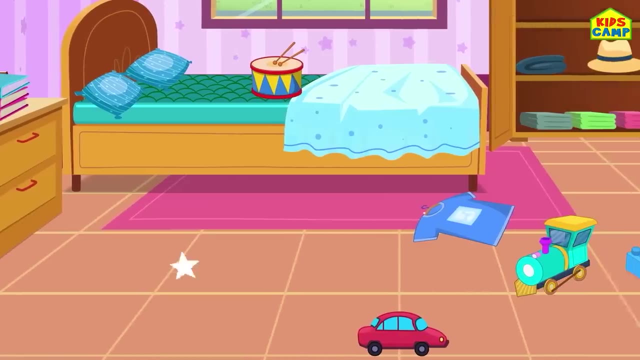 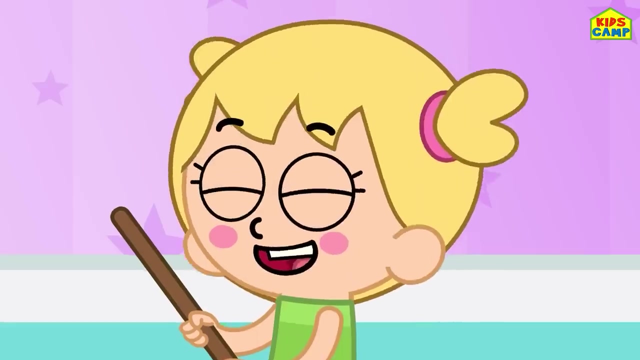 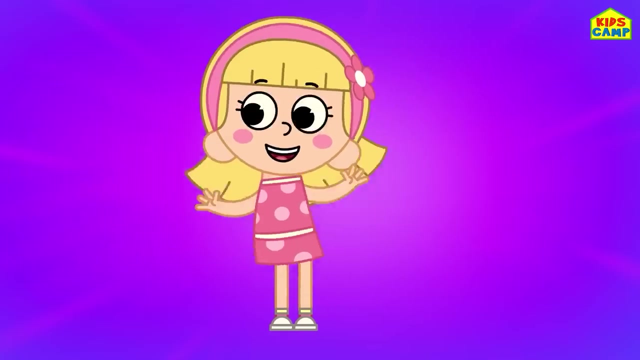 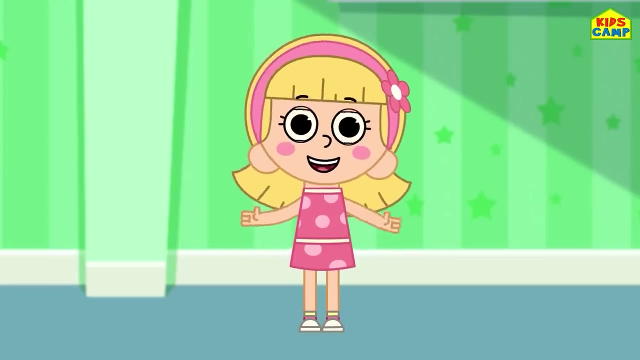 Here are the books. Let's pick them up. Yay, Very good. Stack them together. The room already looks clean, Wonderful. Now let's look for the toy car. That's right, Amazing. On to the shelf. Good job, Eva. 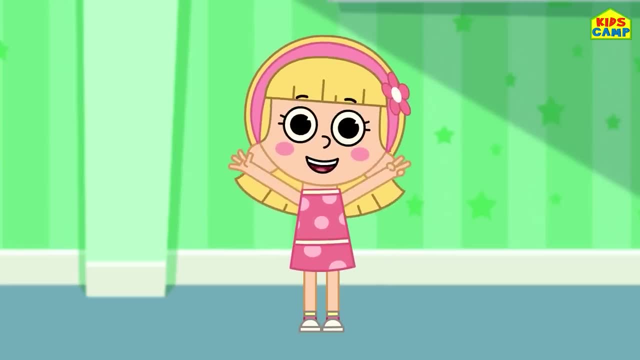 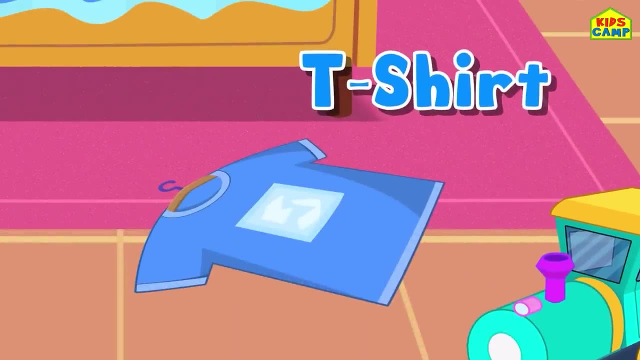 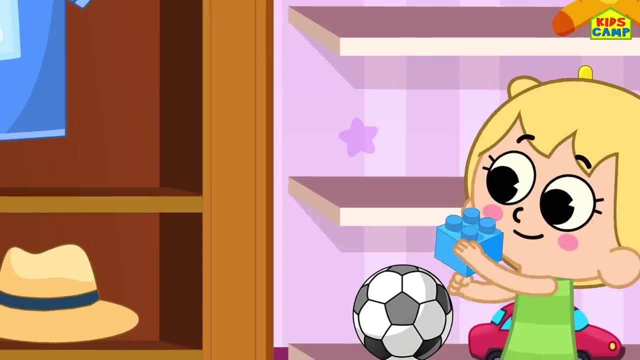 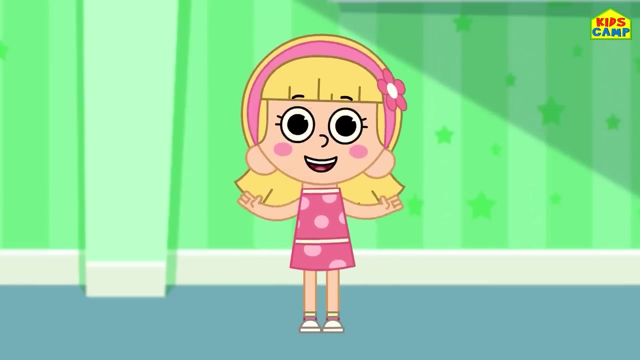 Eva, Let's clean some more The block And the t-shirt. Eva, let's pick them up Into the cupboard And on the shelf. Good girl, Wonderful, Let's clean some more The juju drain On to the shelf. 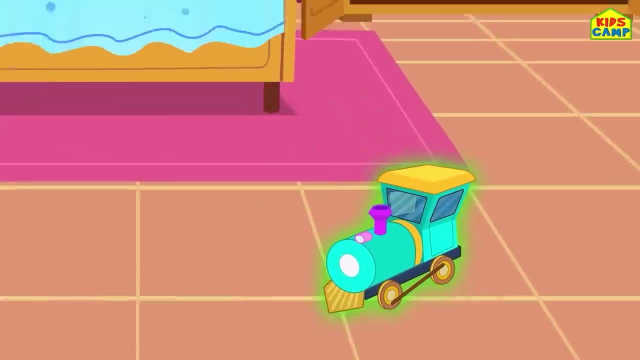 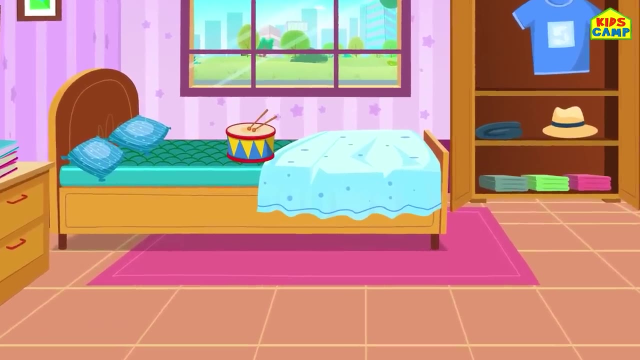 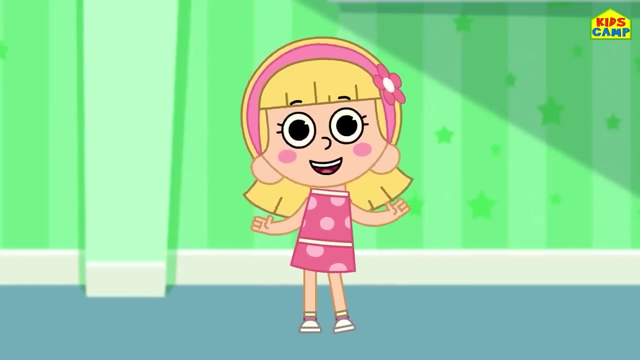 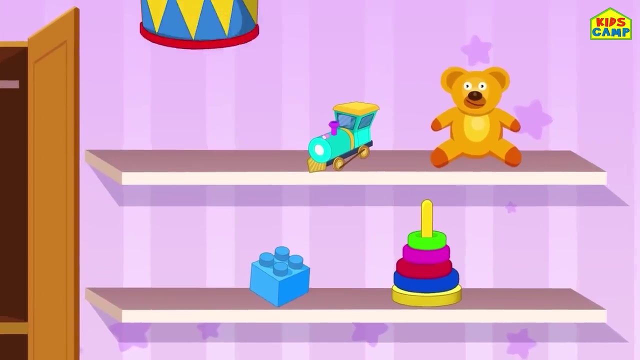 Wee, Let's clean some more. The juju drain On to the shelf. Wee, Yaaayyyyy, Hooray, We did it, We're almost there. Good job, friends. Wonderful The toy drum, Let's pick it up. 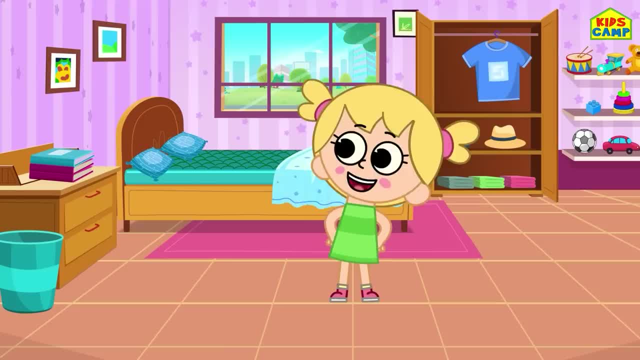 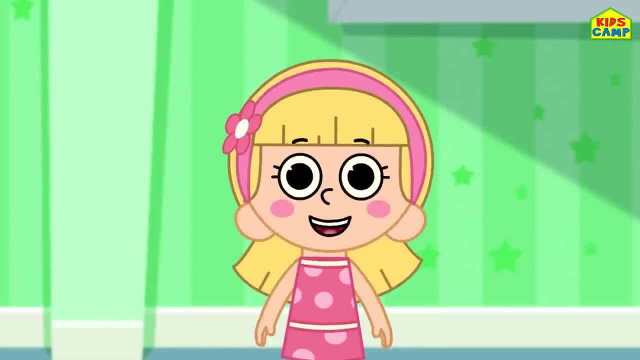 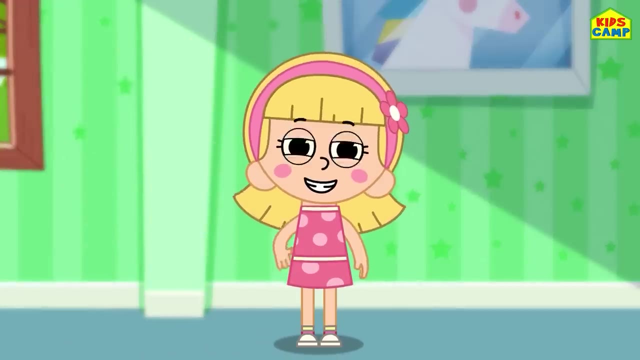 and put it on the shelf. That's right, our room looks clean. Yay, Good job, Eva. Wonderful, Wasn't that fun kids. Bye, Hi friends. I'm Ellie, But I can't find my cat. I don't know where she's gone. Can you help me look for her? 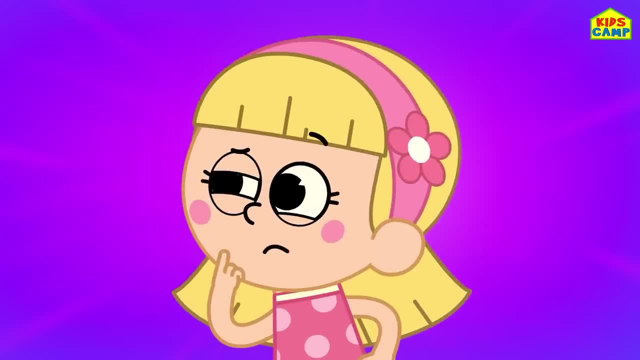 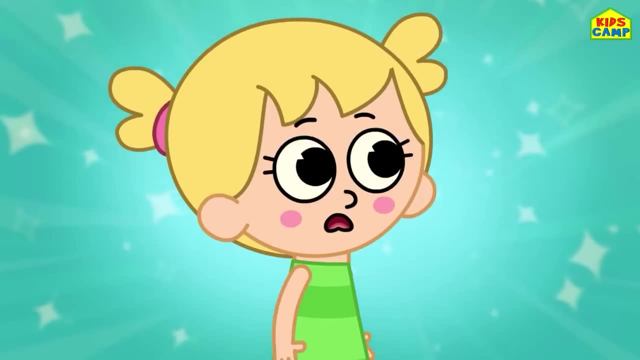 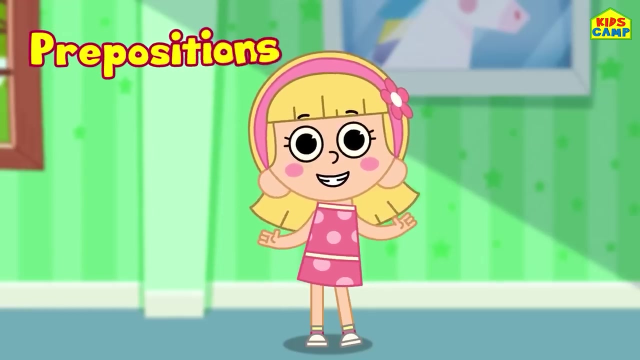 Hi Eva. Where's our cat? That's right, She's in the box. Eva seems to be confused. Don't worry, Today we are going to learn prepositions And how and where to use them. Ready, Let's start. 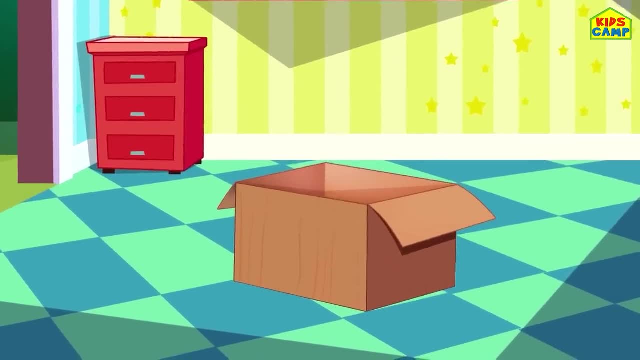 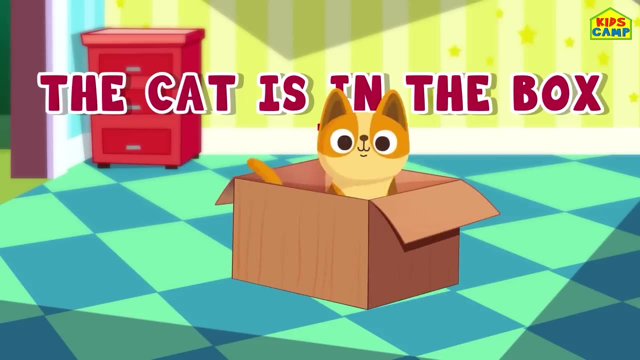 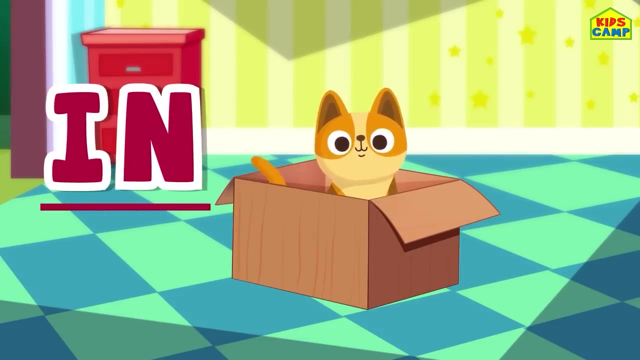 The first preposition is IN. The cat is in the box. Do you see that, Eva? She's in it. IN is the preposition, And THEN is the preposition. This is how we use it To show the position. The next one is ON. 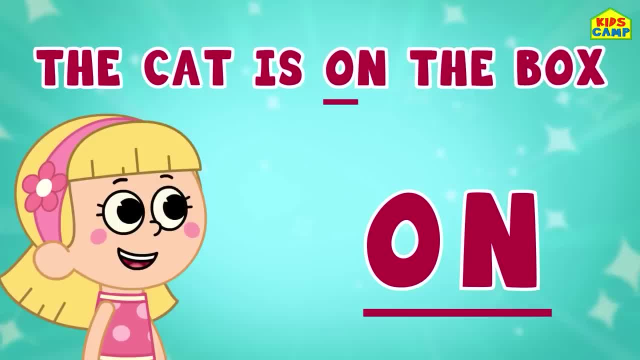 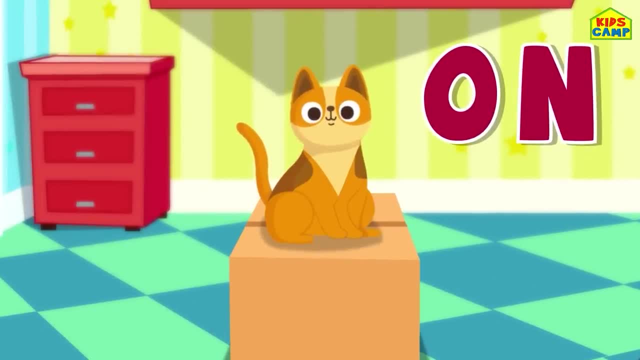 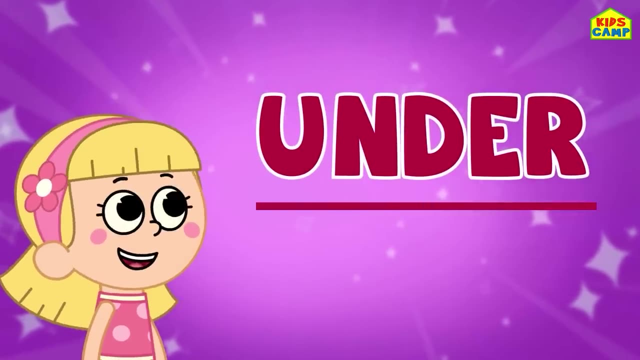 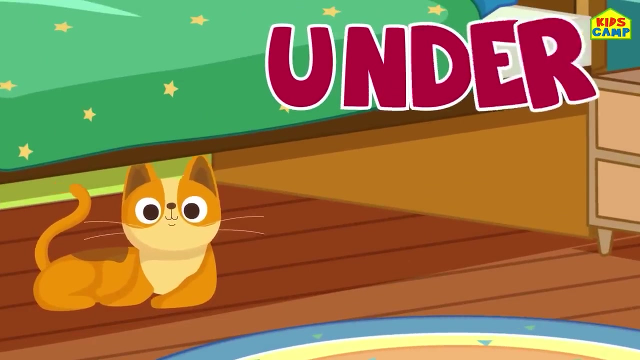 That's right. The cat is on the box. Yay, This is easy, isn't it? This is how we use the preposition ON. Next is UNDER or BENEATH. The cat is under the bed. There she is. We found her. 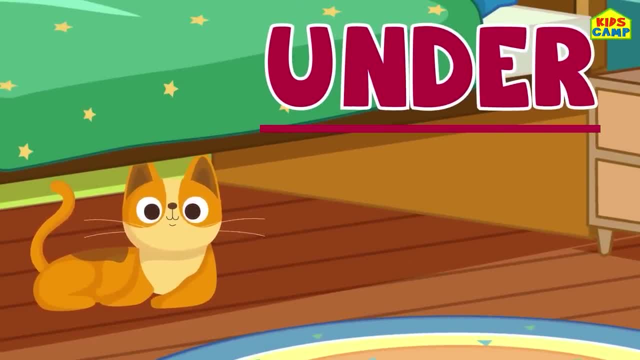 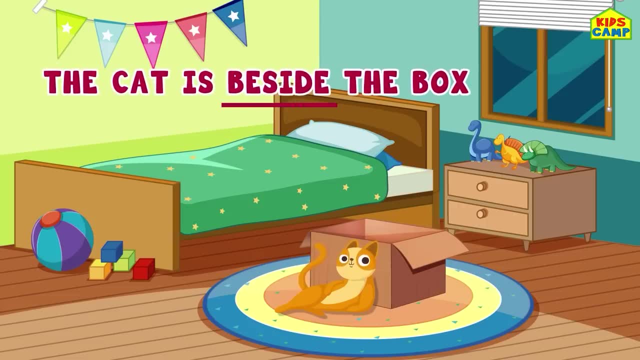 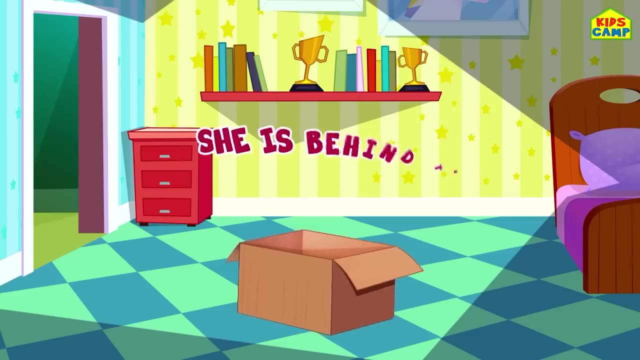 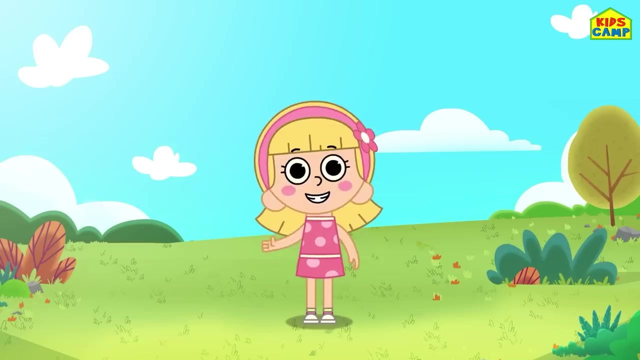 Good job, friends. Where is the cat now? The cat is besides the box. She's beside it Right. Where is the cat now? She is behind the box. There she is. Yay, Yay, Come back for more games and keep watching Kids Cam. 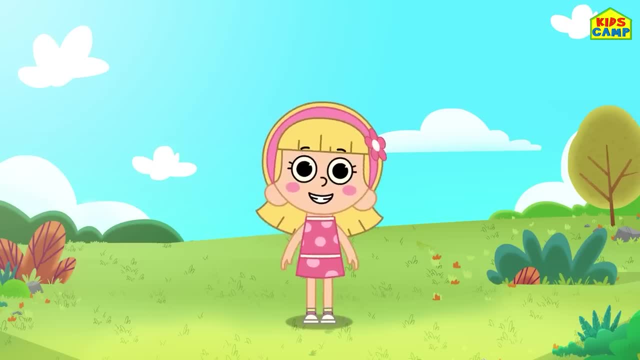 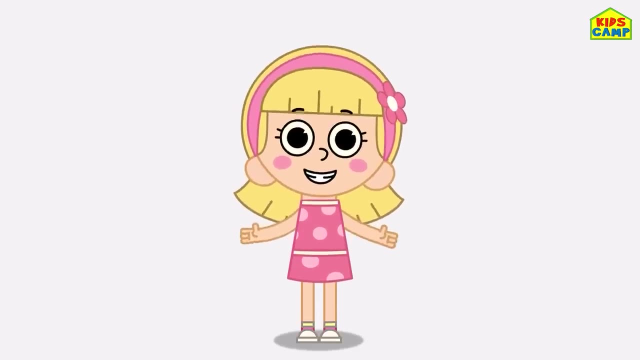 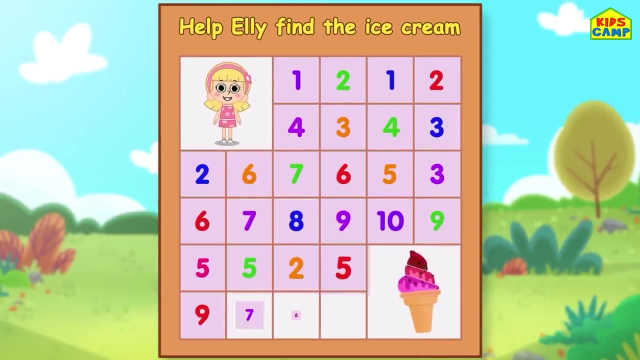 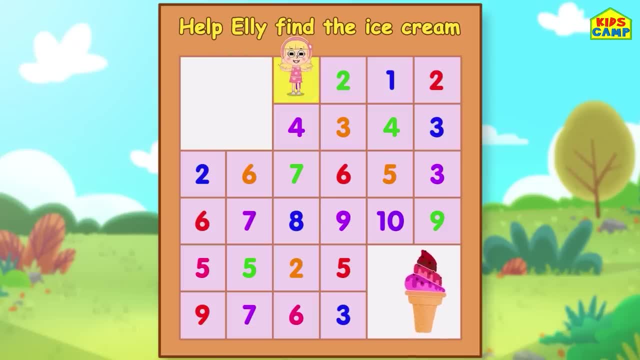 Yes, I'm on number one. Let's go to the next. no Two, Yay, Oh, That's not right. Aha, That's right, That's three. Let's go to the next one, Number four, Yay. 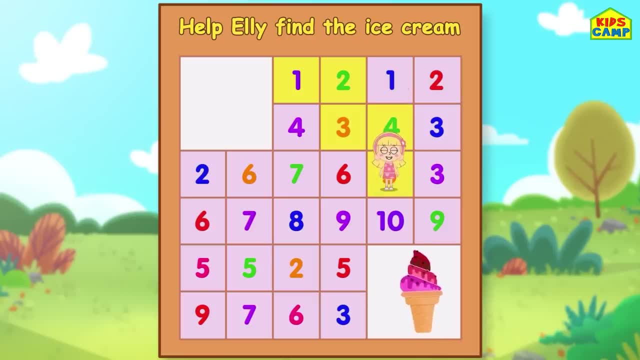 Aha, Number five. Good job, friends. Oops, That's not right. The next number is six, That's right, Wonderful. Next seven, We're almost there. And eight, Yay, Yay, Uh-oh No. 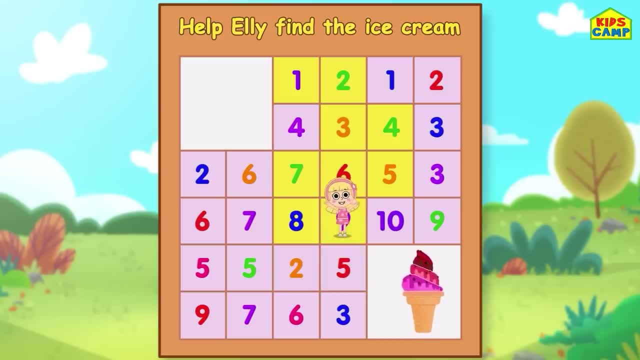 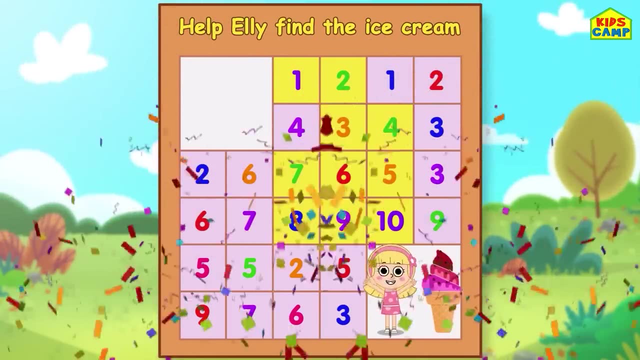 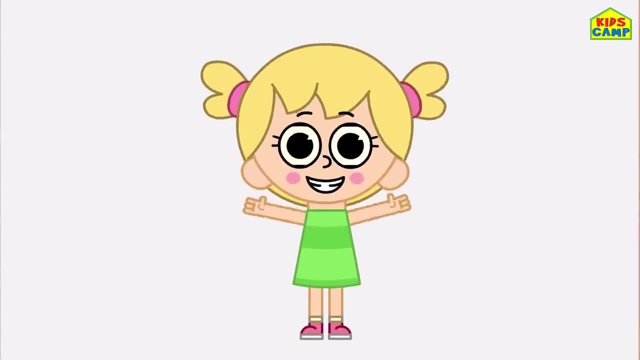 That's right. Nine And ten. Yay, We did it. You helped me reach the ice cream, Thank you. Oh, it's Eva's turn now. Can you help her reach the donuts? Let's get started, Yay. 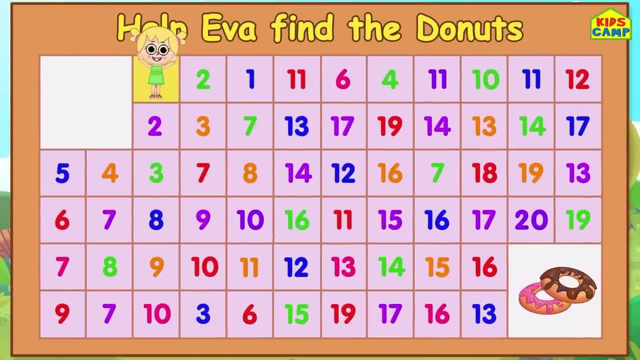 Let's start with number one. One, Two, Three, Good Four, Uh-oh, No, no, no, That's right. Number five: Good Six, Keep going. Seven, Eight, Yay, Oops, That's not right. 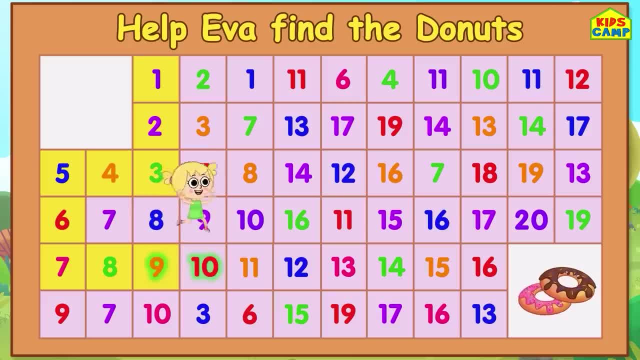 That's right. Nine And Ten And Eleven, And And And And And Eleven. Keep going. Yay, We're on twelve. What comes after twelve? Uh-oh, No, not that one. 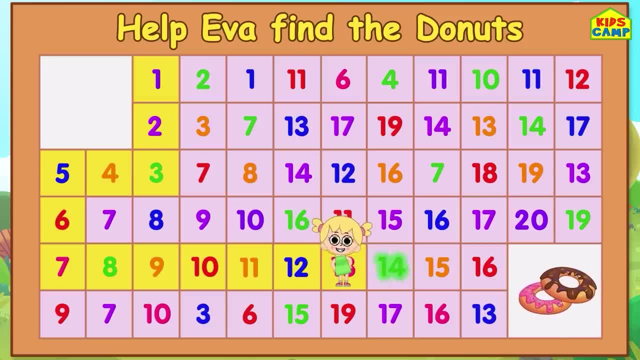 That's right. Thirteen And Fourteen. Next is Fifteen. Wow, Only five more to go Sixteen, That's right. Fifteen And Fourteen, And And, And, And, That's right, Seventeen. 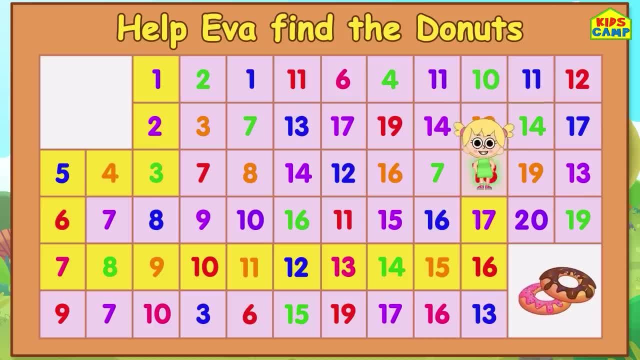 And And. Next is Eighteen, And, And That's right. Nineteen, And, And, And- We're almost there- And And Twenty, That's right, We did it, Woohoo. 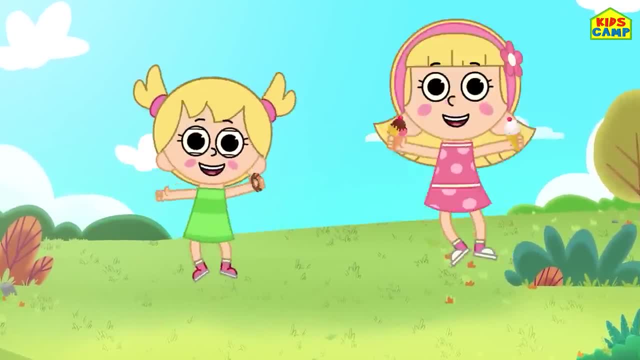 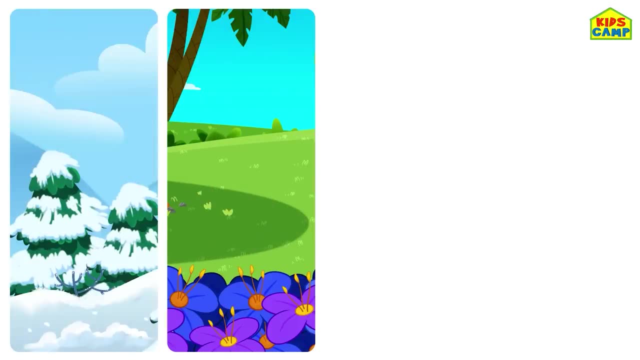 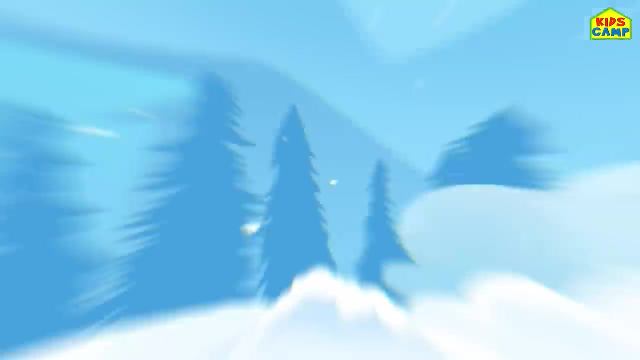 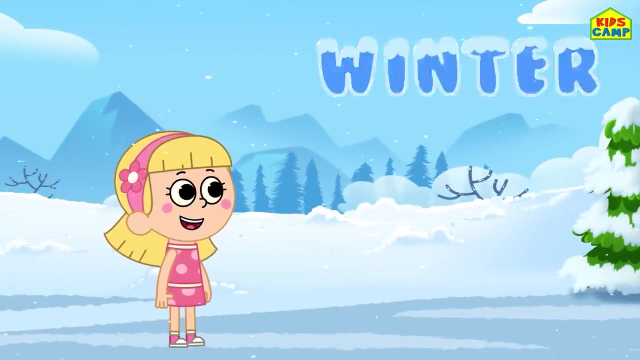 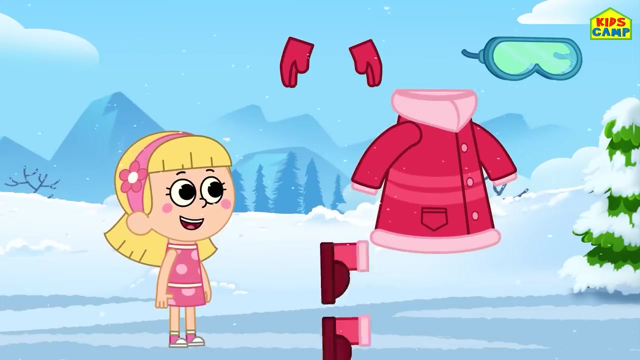 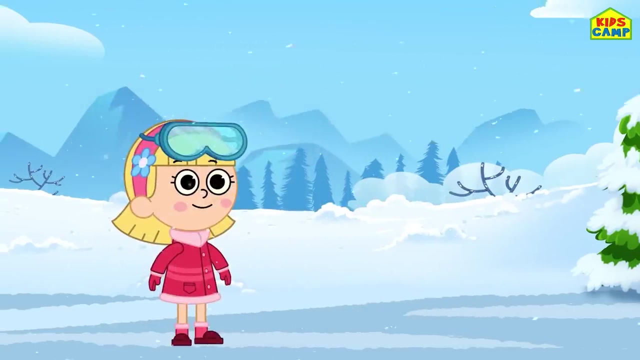 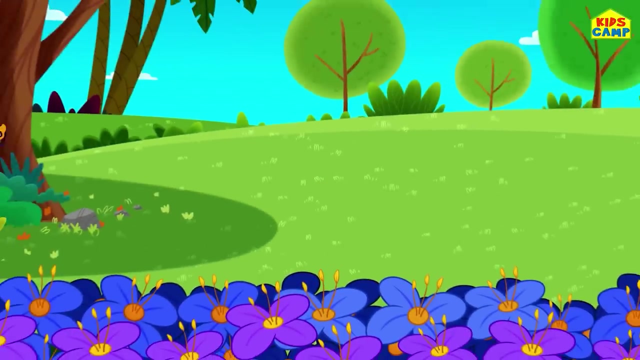 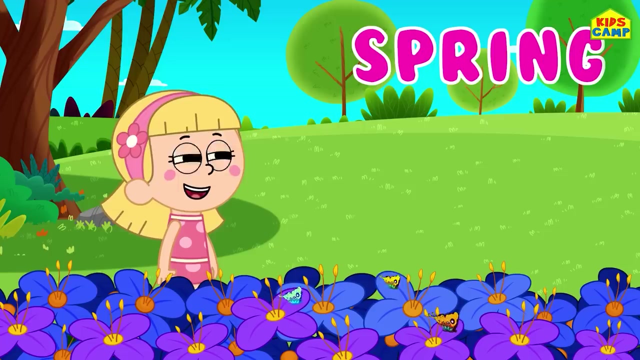 We helped Eva find the doughnuts. Good job, friends. Bye. See you soon, Vogel. usage Seasons with Elli: Snow goggles, Coat, Boots, Yay, Woohoo, Woohoo, What season is this? It's spring. Flower headband. 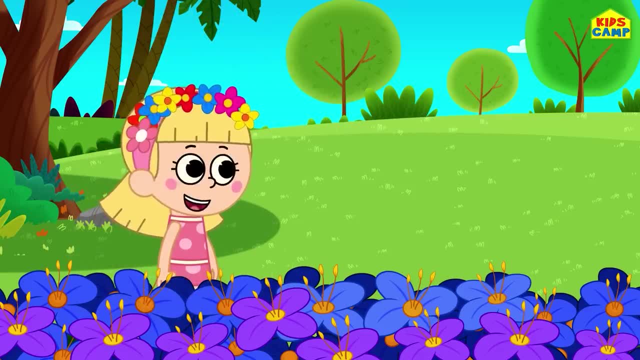 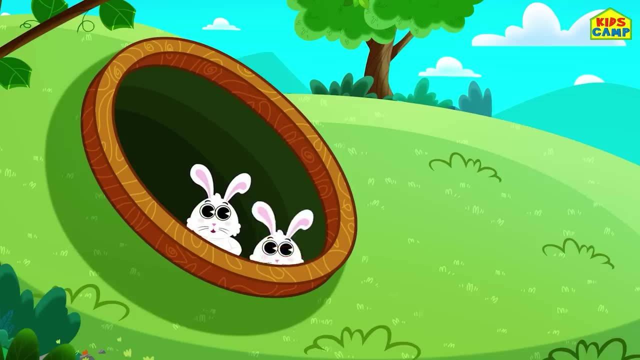 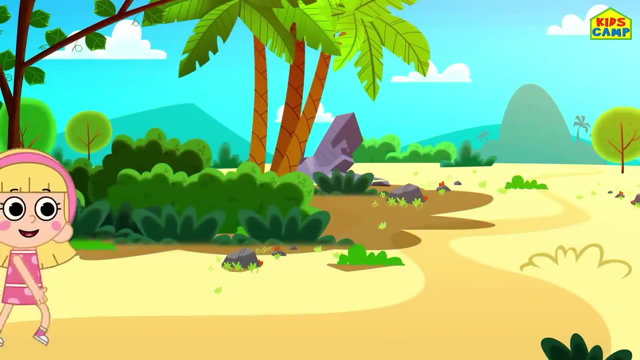 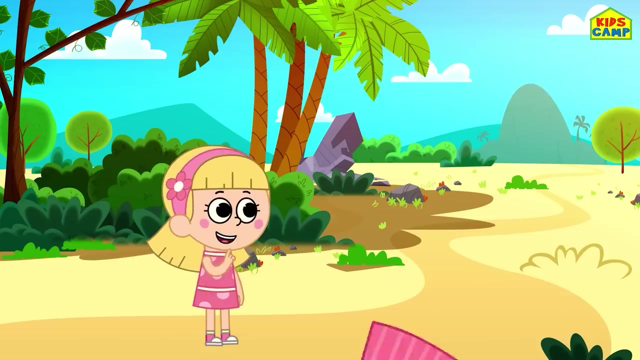 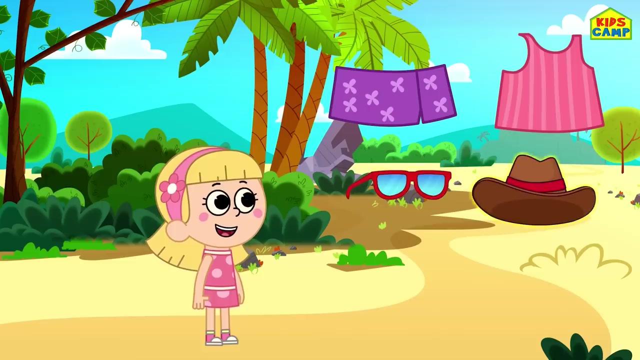 Wow, Look at: the flowers bloom And the birds sing, The bunnies have come out to play And the sun is shining bright. What season is this? It's summer. Swimsuit, Sarong, Sunglasses, Hat- Yay, We're ready to go to the beach. 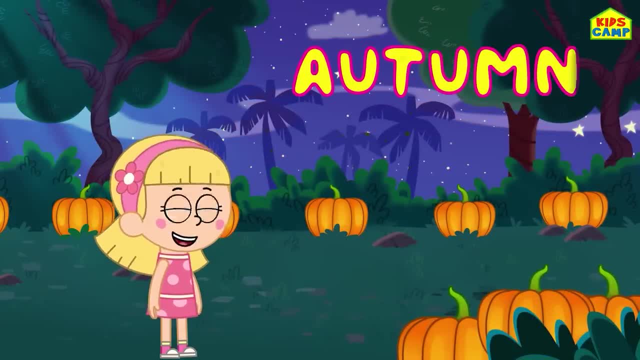 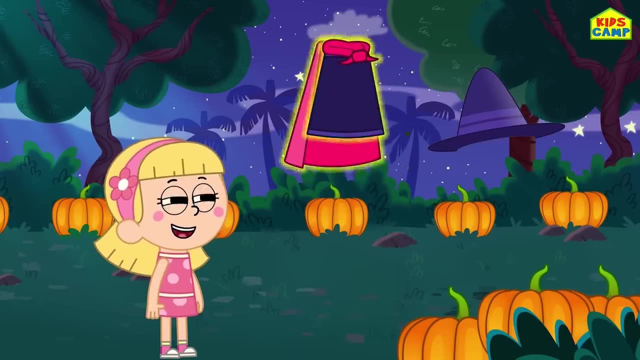 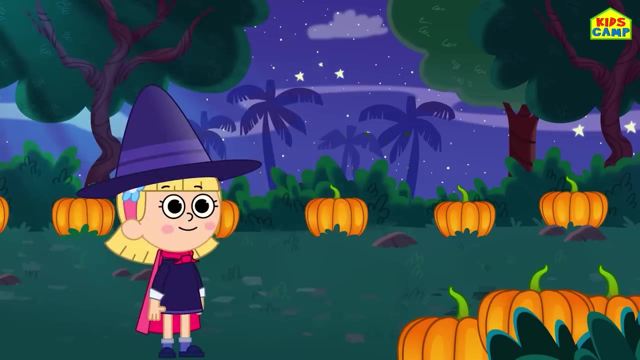 Ooh, It's nearly Halloween. That means it's autumn. A witch's hat, A dresser, A dress with a cloak And witch's shoes- Yay, I'm a witch. Today we learned our seasons: Winter, Spring, Summer And Autumn. 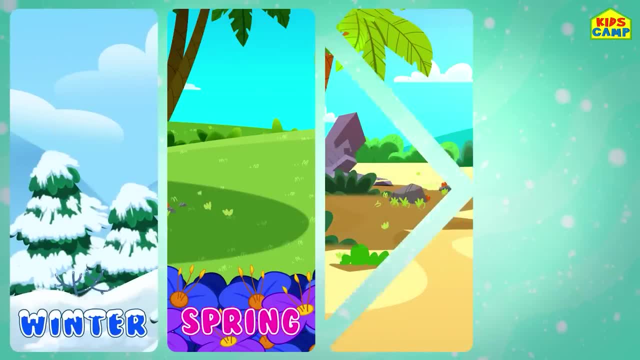 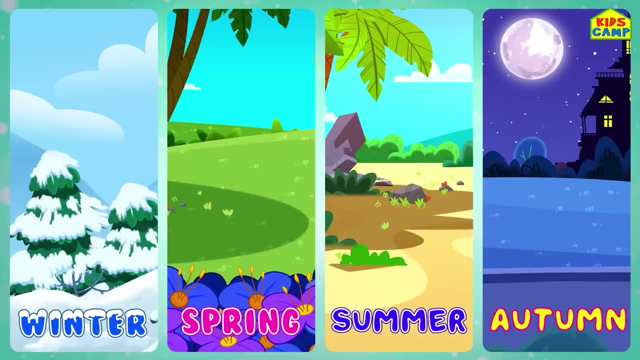 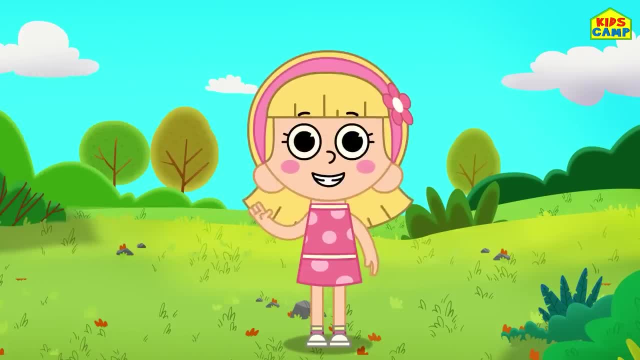 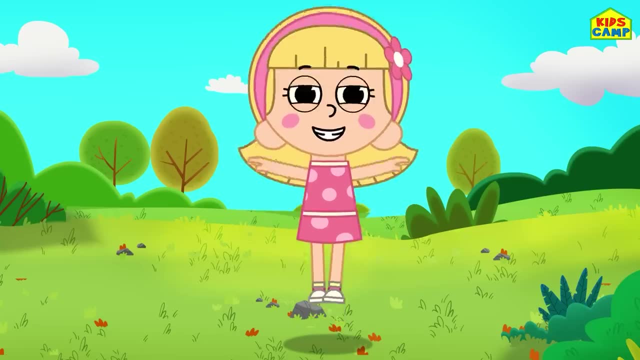 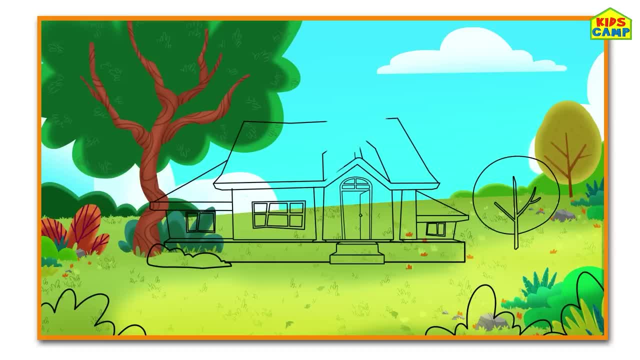 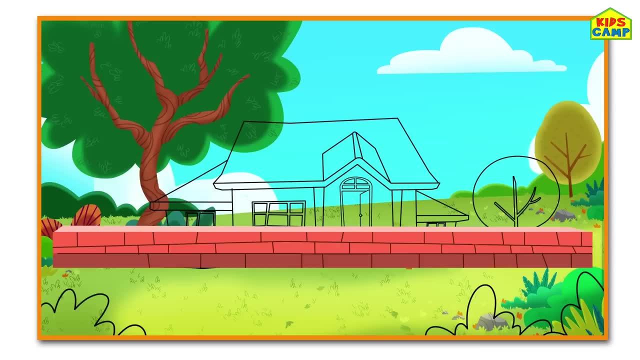 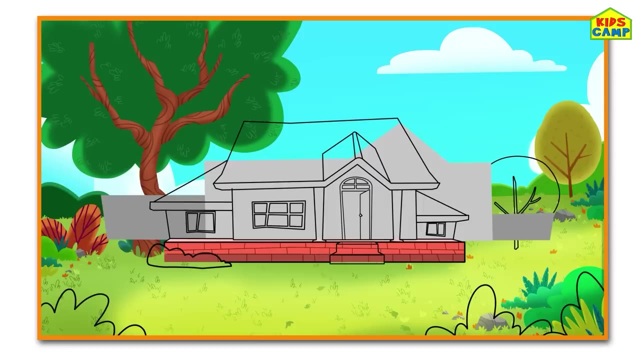 Let's fit the different parts of the house right there. Let's figure out what goes where. First, the foundation, The base. Wow, That was easy. Now let's add the walls. I love Yellow paint on my walls. on my walls, this looks great. next, let's add the roof. 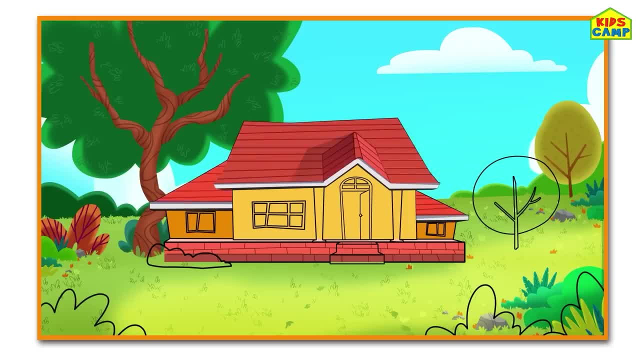 perfect. it's starting to look like a house. what's missing? that's right: a door, yes, and lovely windows to look outside and for sunshine to come in. next we need steps: perfect, and now let's add the pillars. going good, this is such a beautiful house, but what else is missing? let's add color. 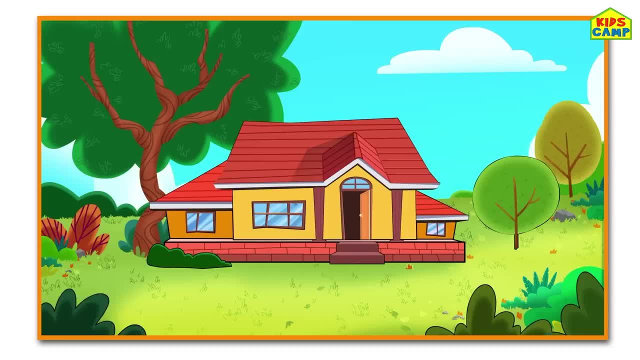 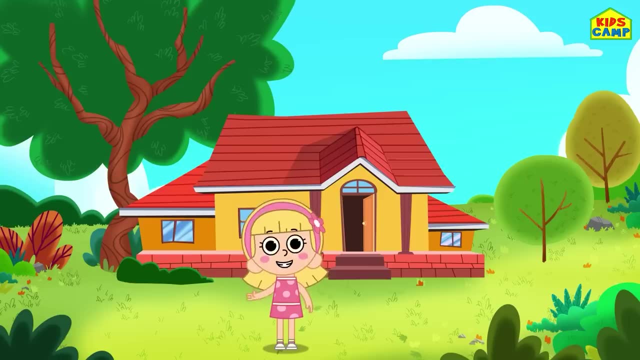 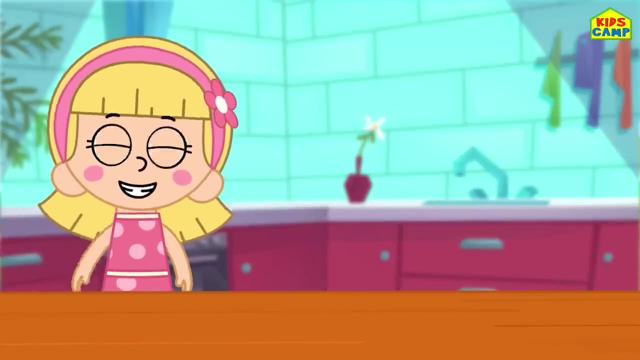 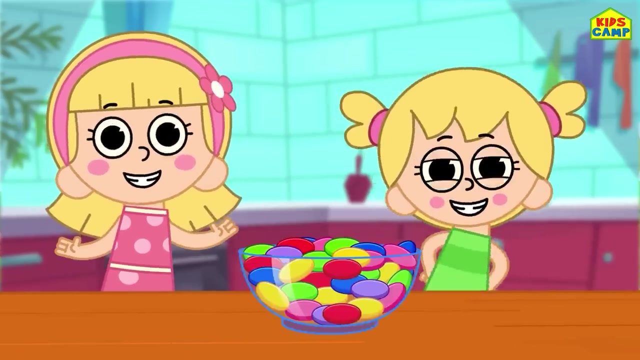 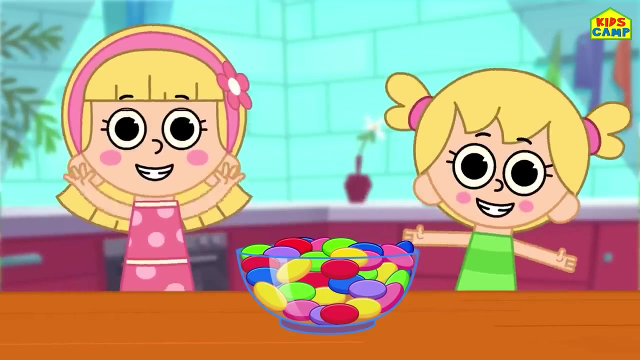 to my garden. wow, it looks beautiful. that's my house. okay, friends, i'm going home. see you, bye, hi, friends, i'm ellie and i love jelly beans, don't you too? that's right, and this is eva. we have to sort the jelly beans by the color, that's easy. 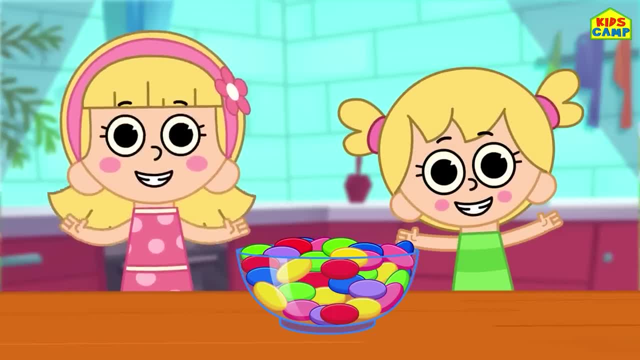 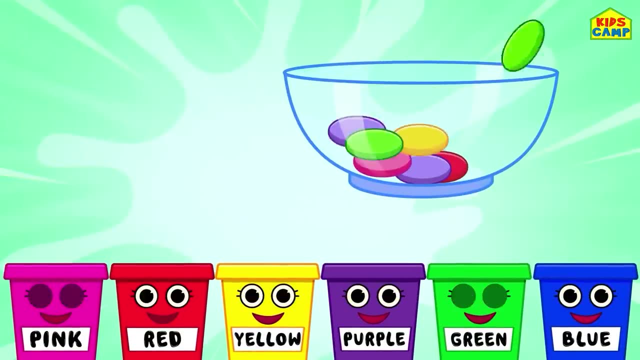 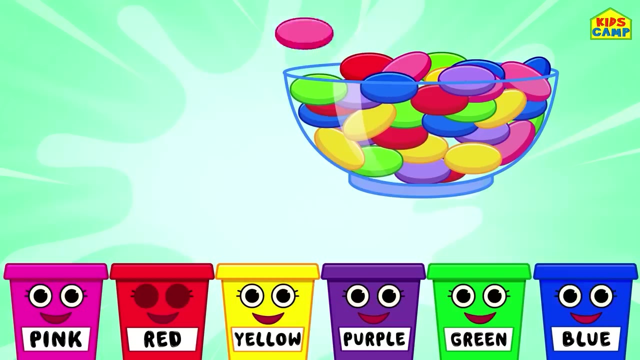 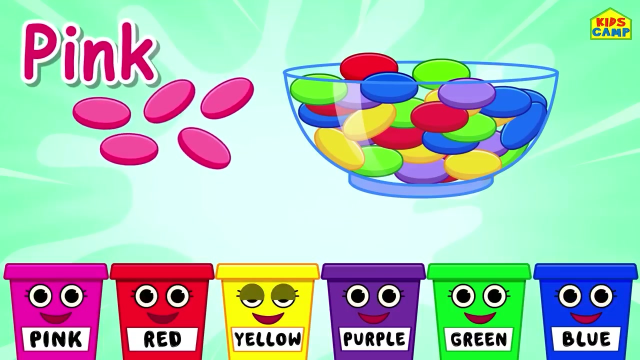 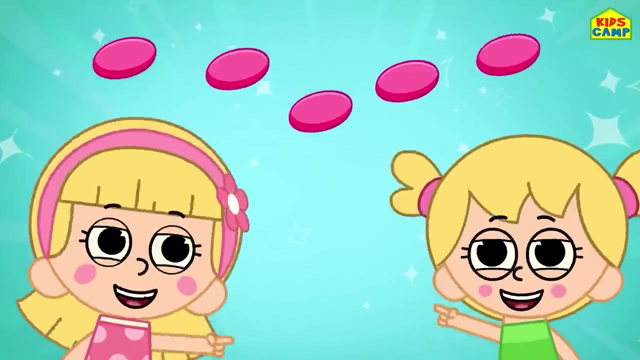 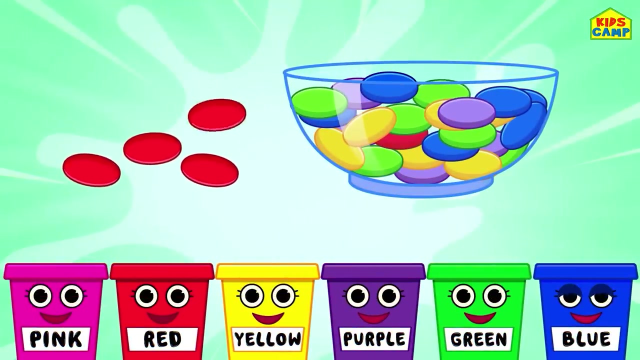 will you help us? let's get started. oh, jelly beans. let's start the pink jelly beans. yummy, into the pink pocket, wonderful, yay. next up is red. let's start the red jelly beans. oh, honey, jelly beans. looks great. let's sort the red jelly beans Into the bucket. 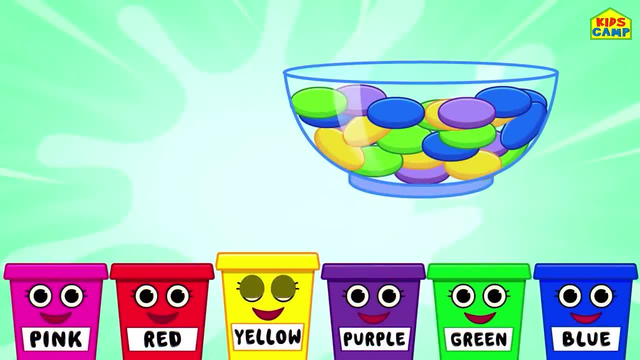 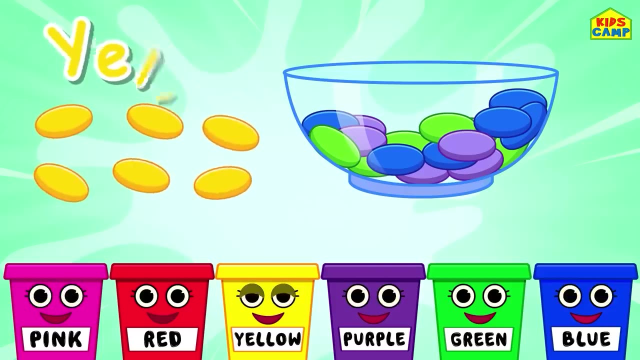 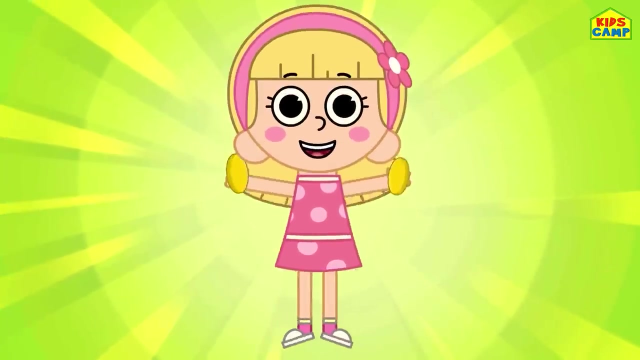 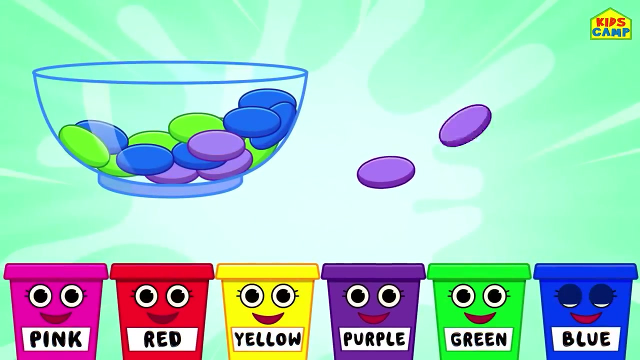 Yummy. Next up is the color yellow: Yummy. Let's sort all the yellow jelly beans That's right Into the bucket. Wonderful, I love yellow. Next is purple. Look for all the purple jelly beans. Yes, That's right. 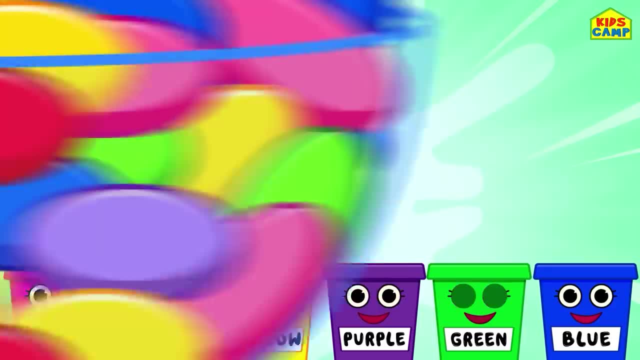 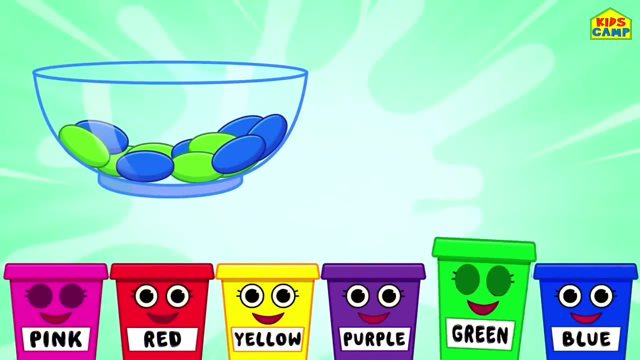 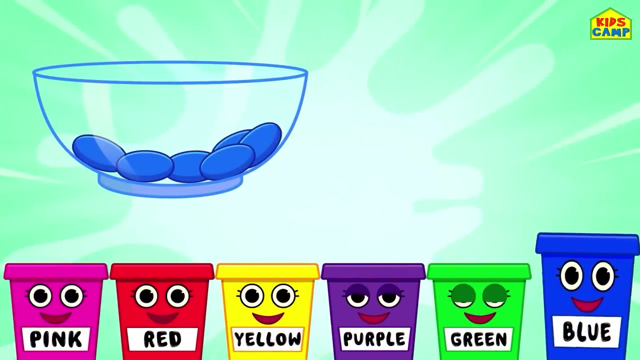 Into the bucket. Great job, friends. Wonderful. We all love jelly beans, don't we? Next is green. Let's sort all the yellow jelly beans, Green jelly beans, Yummy, Into the bucket. Wonderful, Yummy. And the last one is blue. 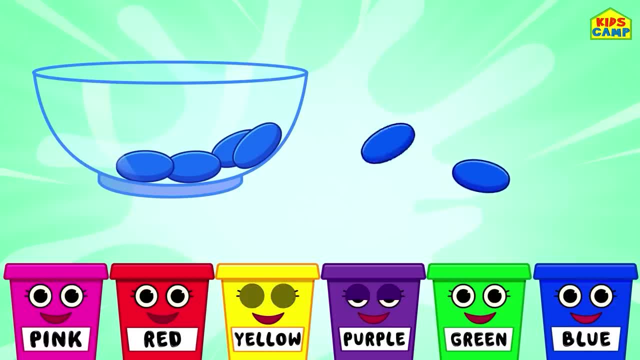 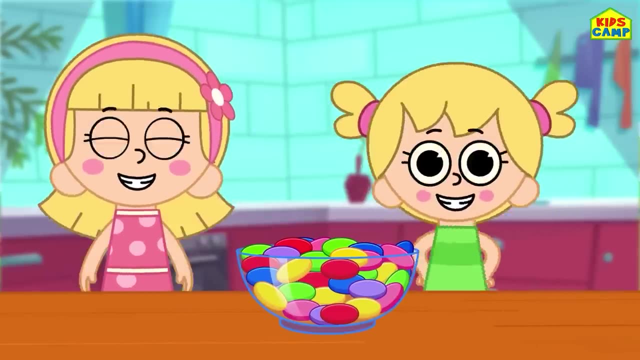 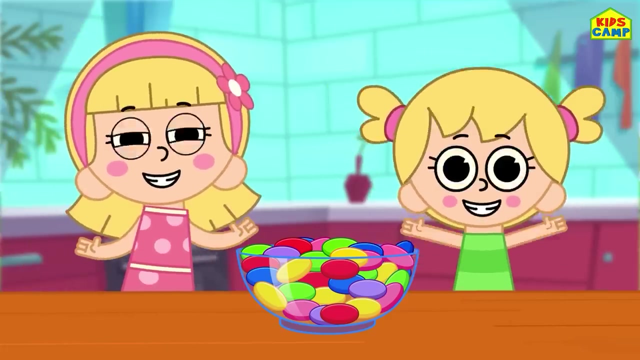 That's right. We have only the blue jelly beans remaining. That's right. right Into the blue bucket And we're done. Good job, friends. That was such a fun time sorting the jelly beans. Come back for more on Kids' Game. See you soon. Bye-bye. 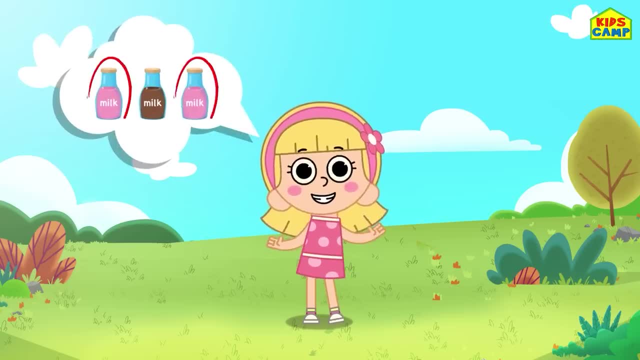 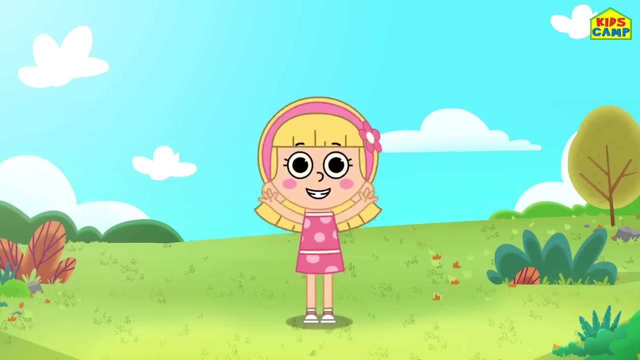 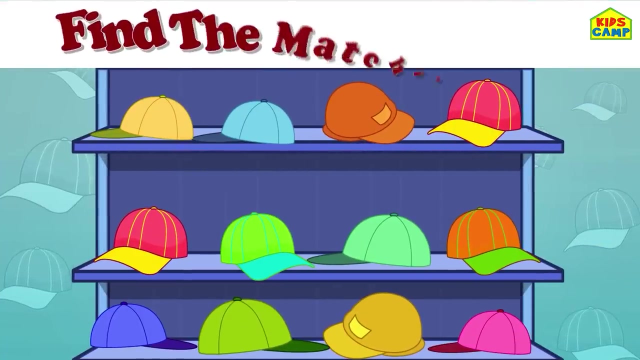 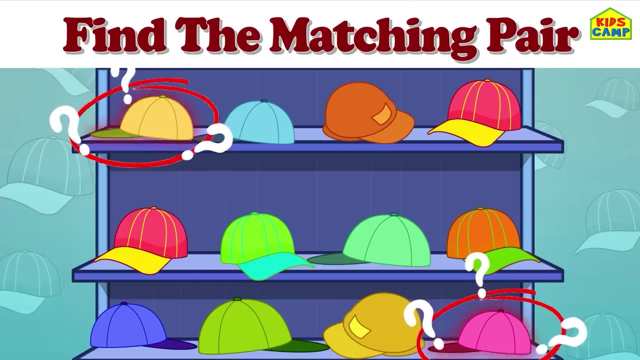 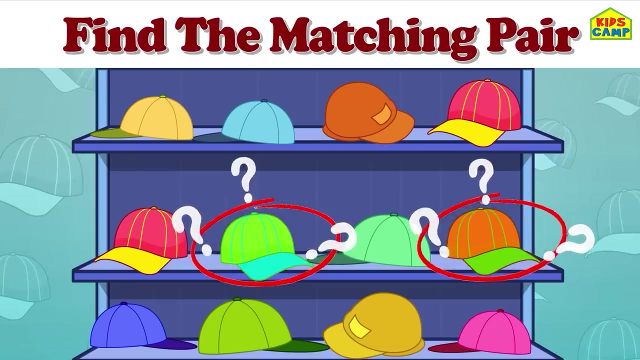 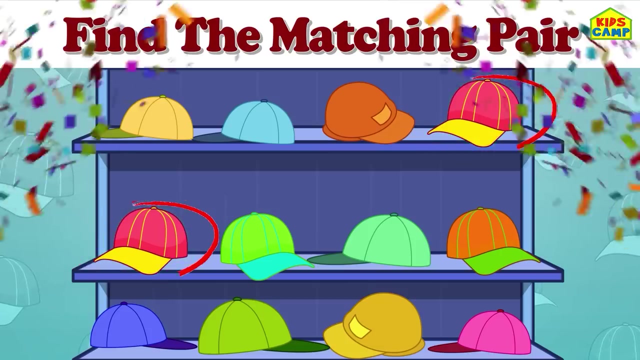 That's right. We have to find two similar objects, and that's the game. That's simple. Ready, Let's get started. Find the matching pair. Can you spot two identical caps? No, they're not identical. No, Yes, Yay, We found them. They're two identical caps. 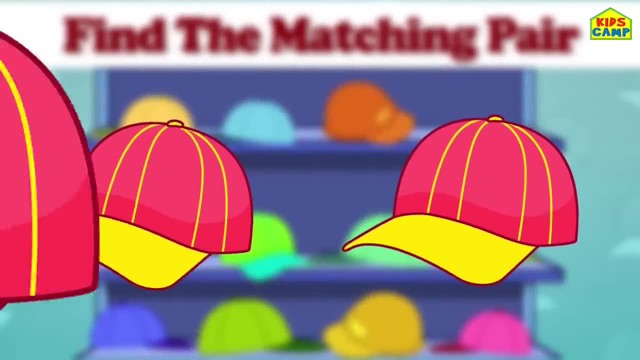 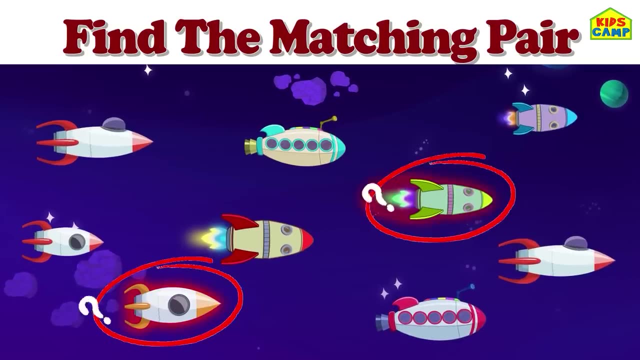 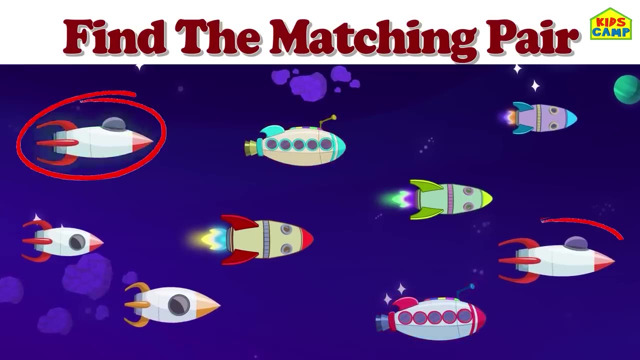 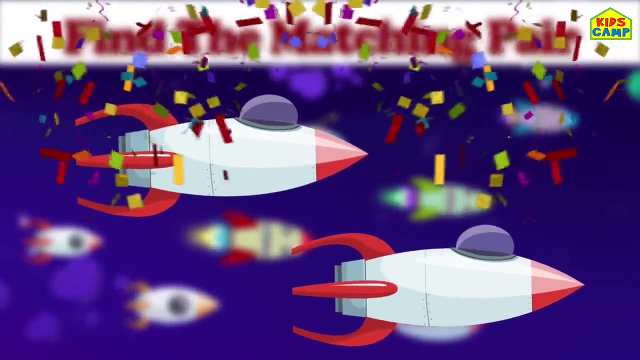 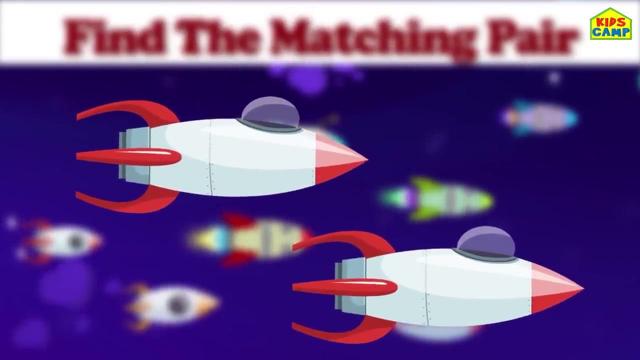 Good job, Let's find another pair. Find the matching rockets, Can you? No, not this one. No, Yes, That's right They match. Perfect, We found them. This was easy. Let's go to the next one. 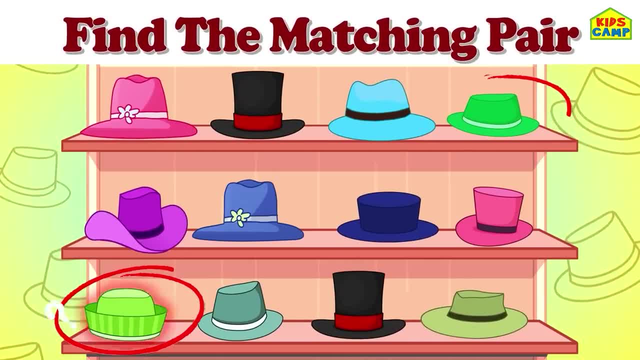 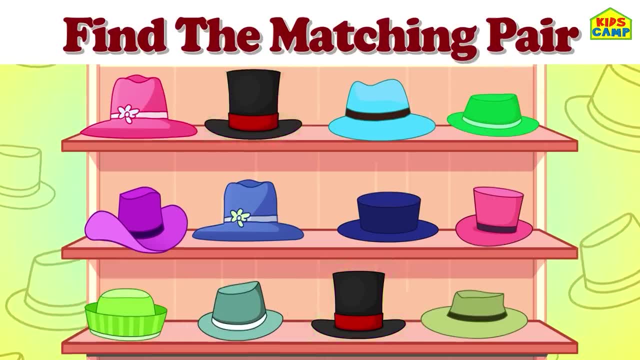 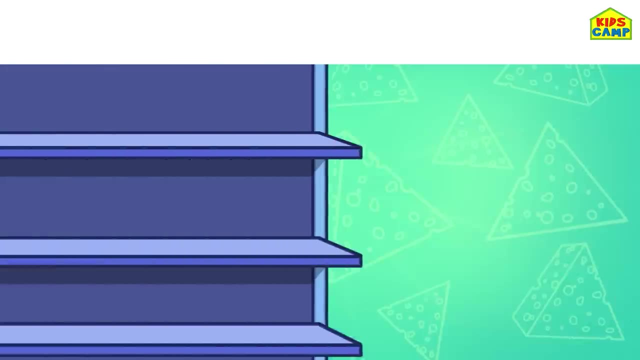 Find the matching hats? No, Yes, We found them, Perfect pair. Good job, friends. Can you find the matching cheese? No, Definitely no, That's right, These match Perfect. Good job. No, No, No. 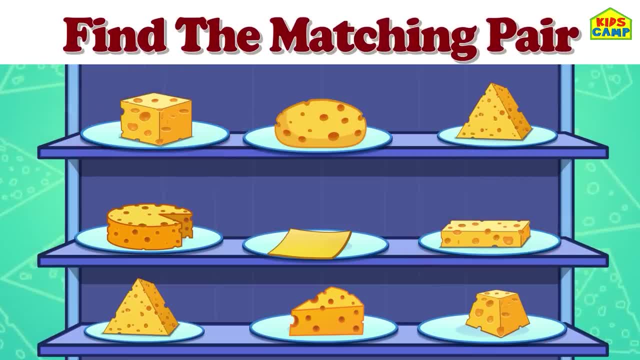 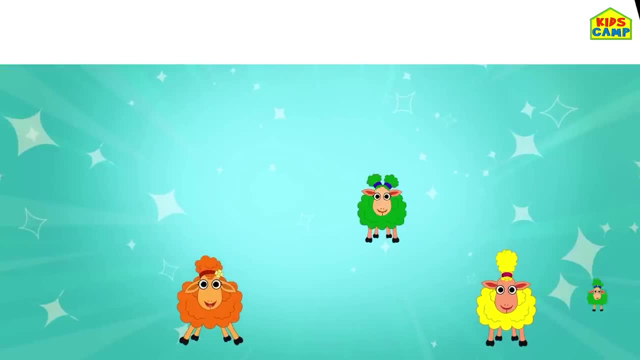 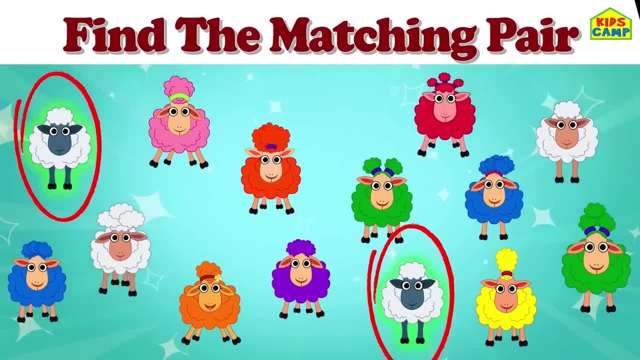 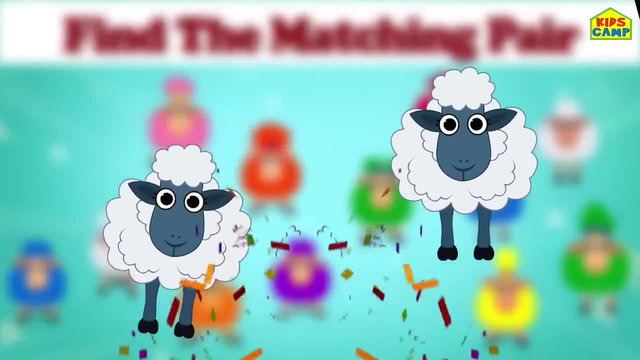 No, They're not identical. Yes, They match. That's right. These sheep match Perfect Perfect. Why does Waree have so many speckles? We can find more if we move the net. Find the matching coolers. 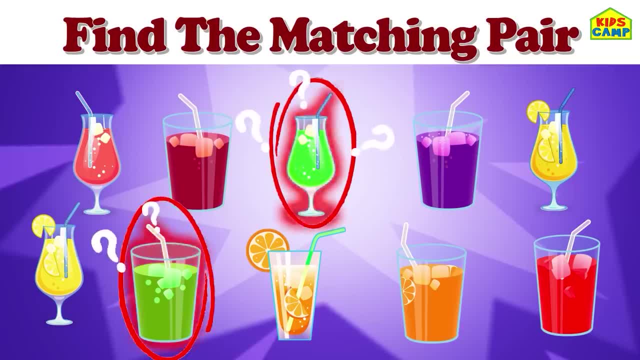 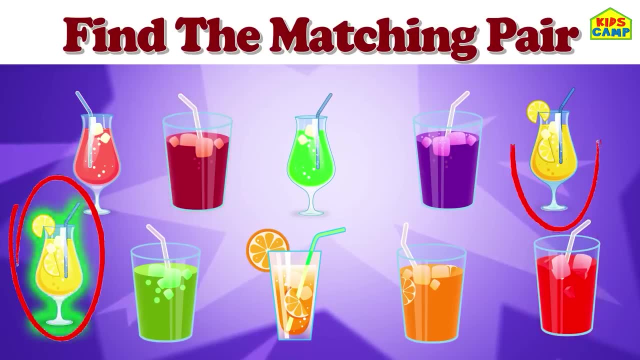 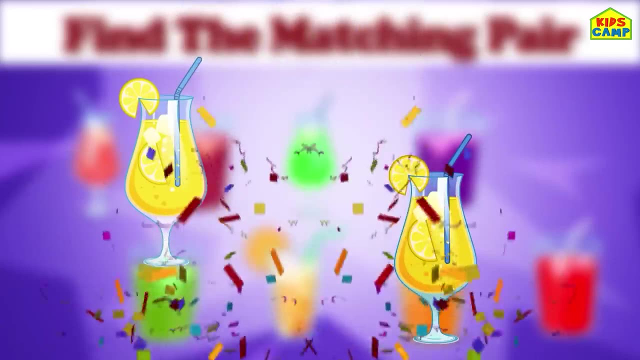 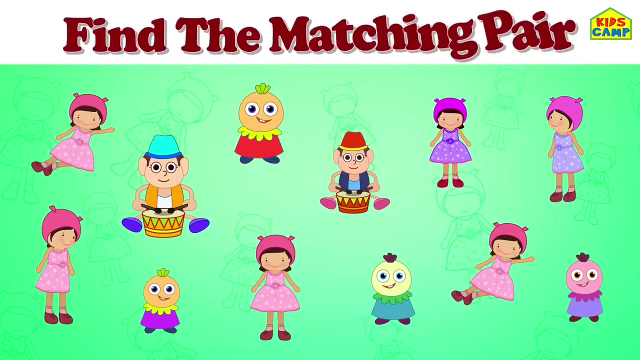 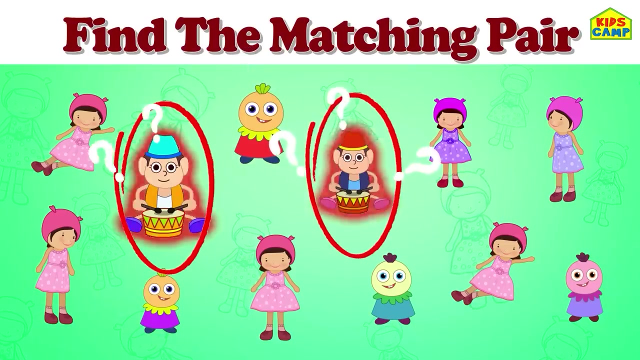 You know what to do If we change new phenol. Do these match? No, Do these match No? Yes, We found the pair. Good job, friends. Find the matching pair. Let's look for one. No, No way. 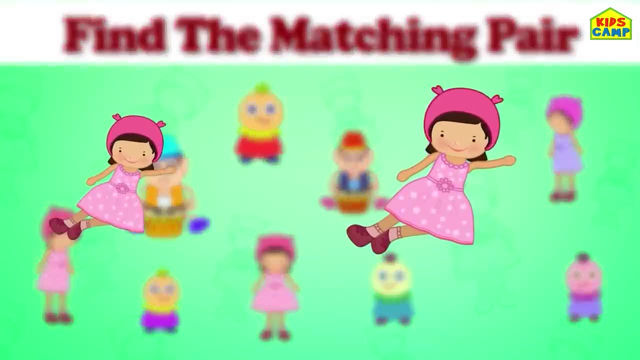 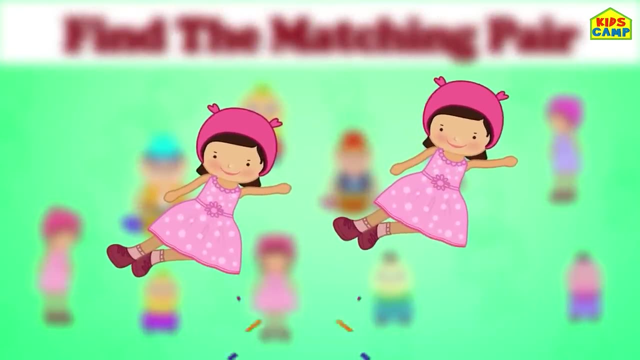 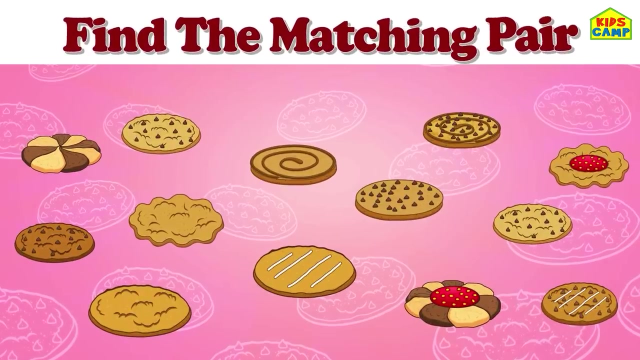 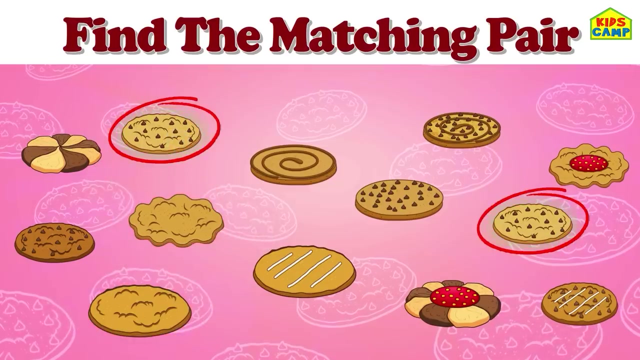 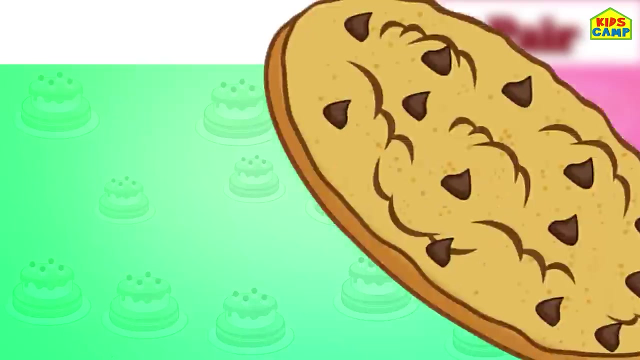 That's right, We found the pair. Yay, Good job. friends, This game is so much fun. Ooh, Cookies. Find the matching pair? No way. Yes, We found them. I love cookies, Yummy. Let's go to the next one. 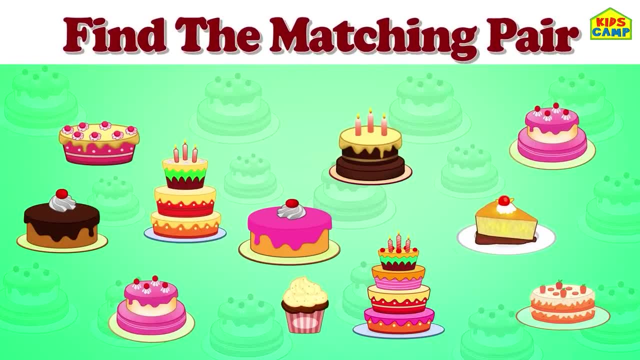 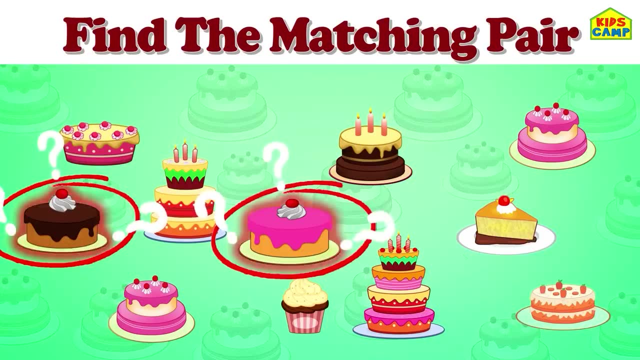 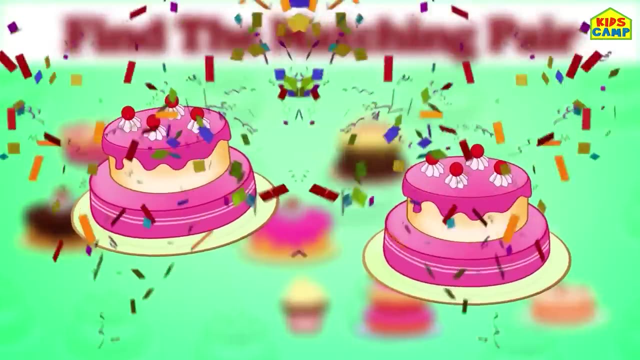 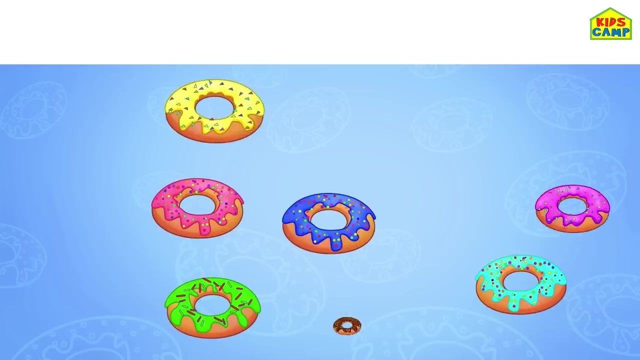 Hmm, Cakes Find the matching pair. No, No, Yes, That's right, The matching pair of cakes. Yummy, Wonderful Ooh Donuts. We found the matching pair. No, No, Yes, We found the matching pair. 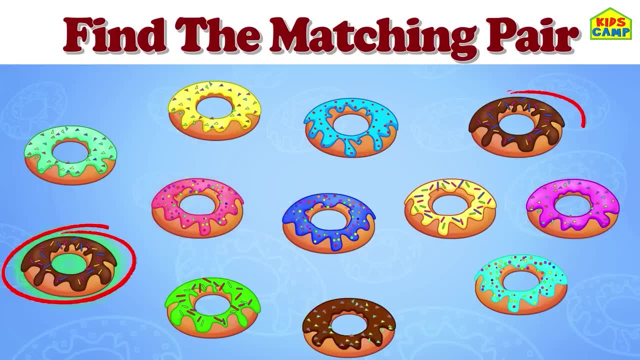 These match. This was such a fun game, friends. Keep watching Kids' Camp. Bye-bye, Hi, friends. I hope you enjoyed this video. If you liked it, please subscribe to our channel And don't forget to like and share it with your friends. 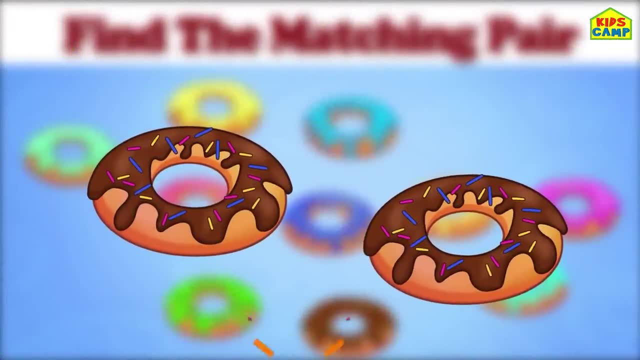 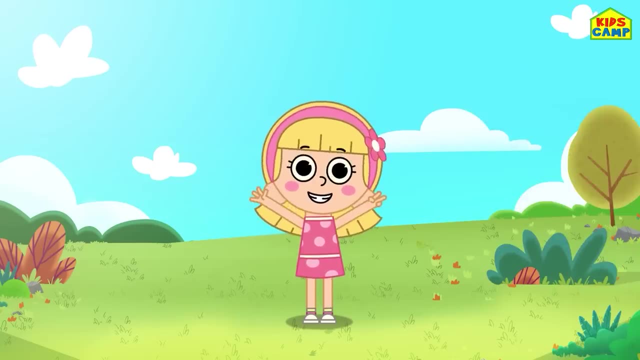 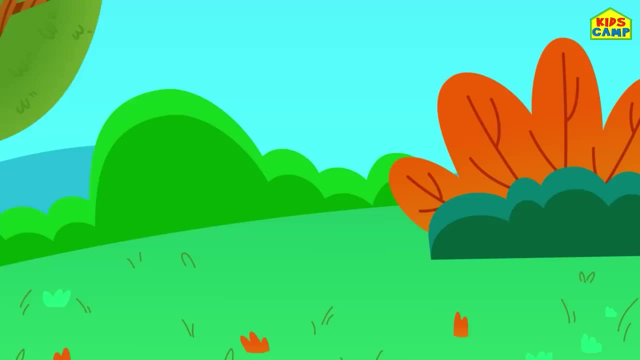 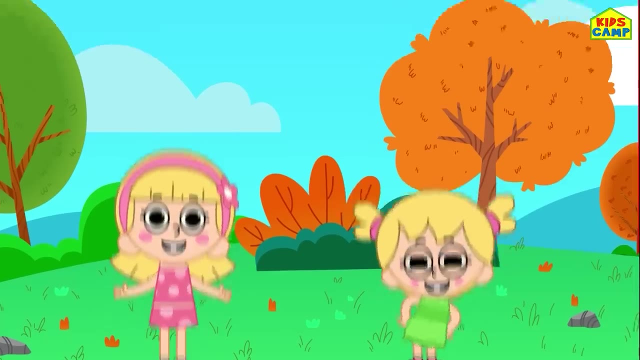 Bye-bye, Bye-bye, Bye-bye, Bye-bye, Bye-bye, Bye-bye, Bye, Bye-bye, Bye-bye, Bye-bye, Bye-bye. Hi friends, I'm Ellie And this is Eva. 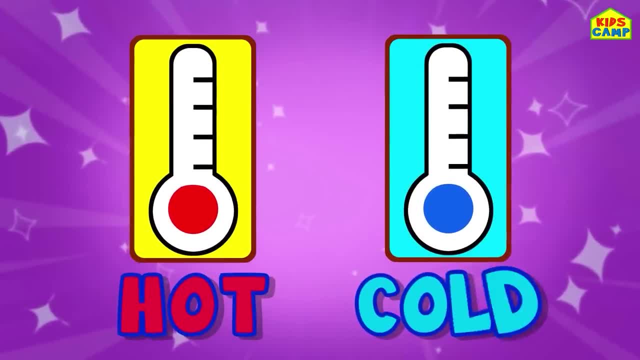 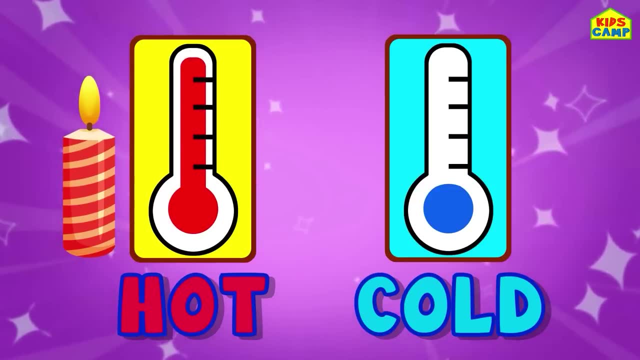 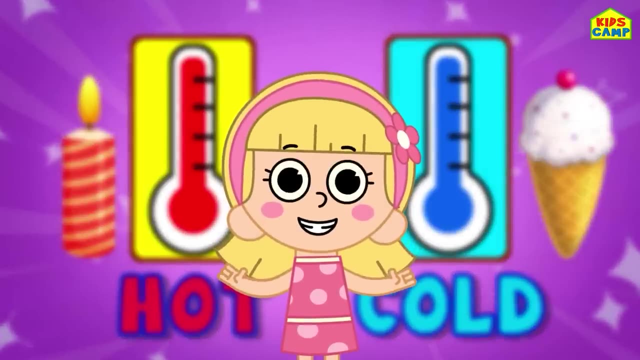 Today we are going to play a fun game of Hot and Cold. That's right. We have to sort according to what is hot and what is cold. For example, a candle is hot, That's right, And an ice-cream is cold. 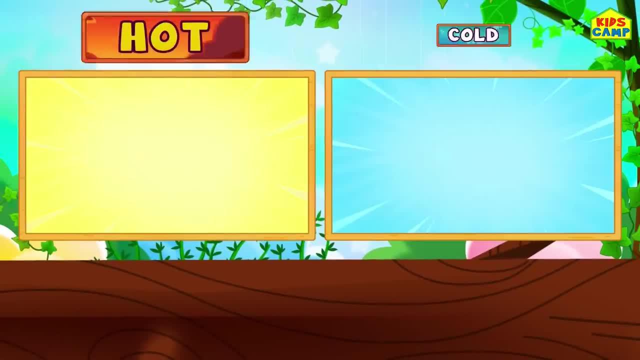 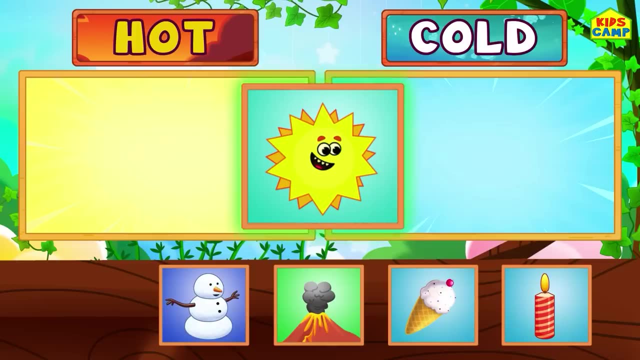 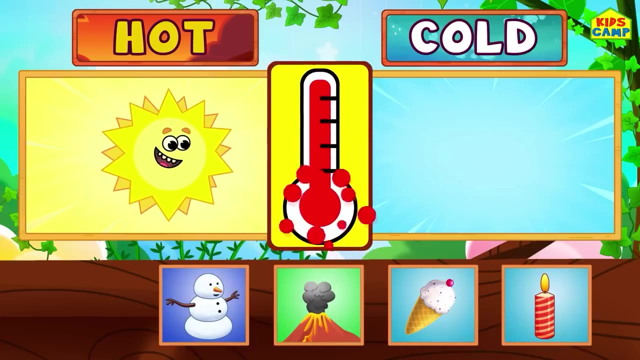 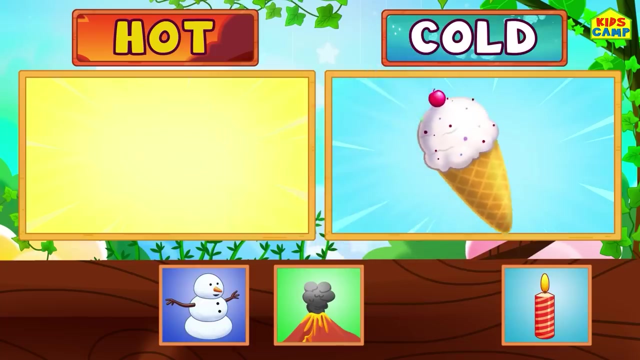 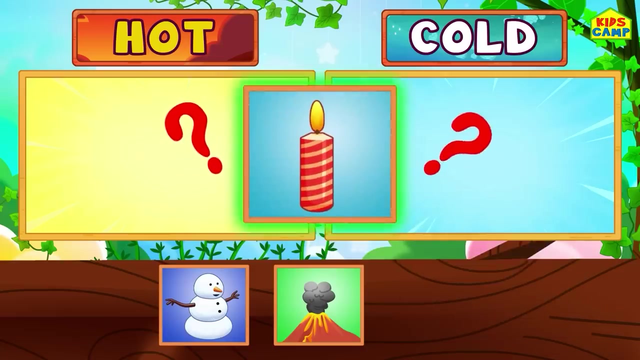 That's right, Wonderful, Easy. Let's get started. Hmm, is sun hot or cold? That's right, Sun is hot, Very, very hot, That's right. And ice cream, It's cold. Yummy A candle- Hot or cold? 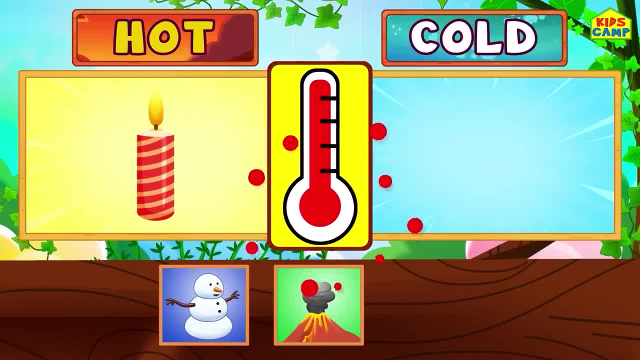 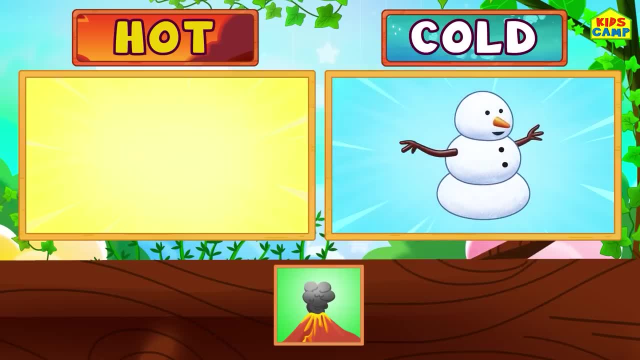 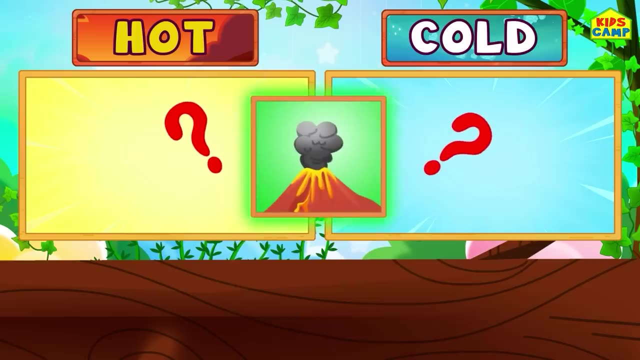 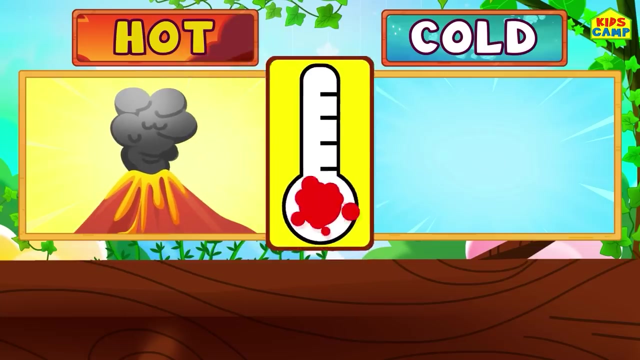 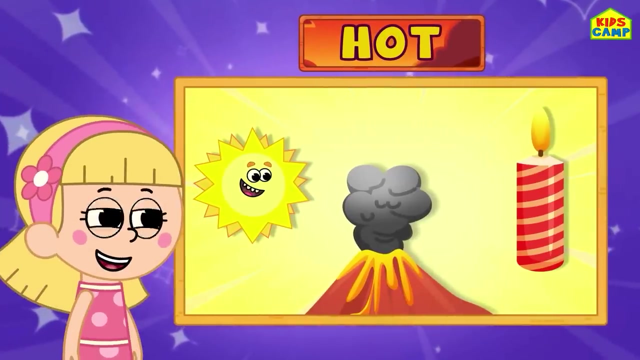 Hot, Good job, That's right. A snowman- Yes. cold, That's right. A volcano- Hot or cold, It's hot, That's right, Very hot, Yay, We found the hot objects: The sun. 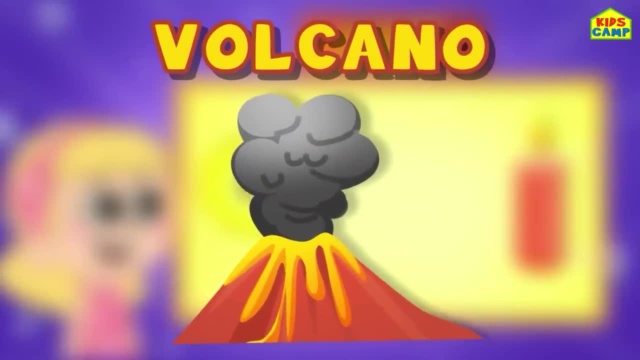 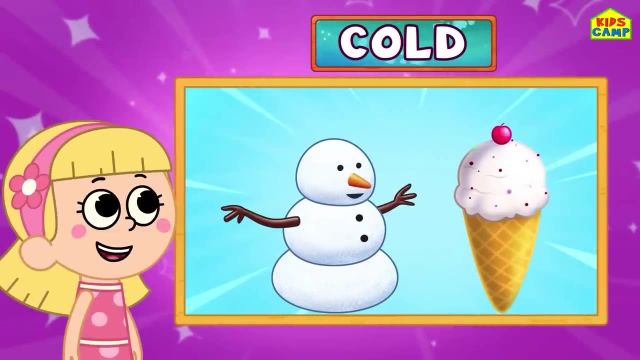 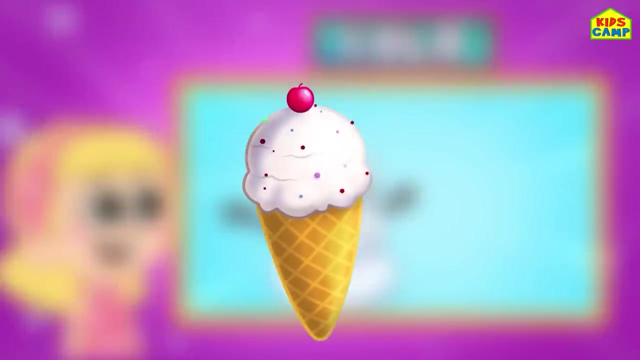 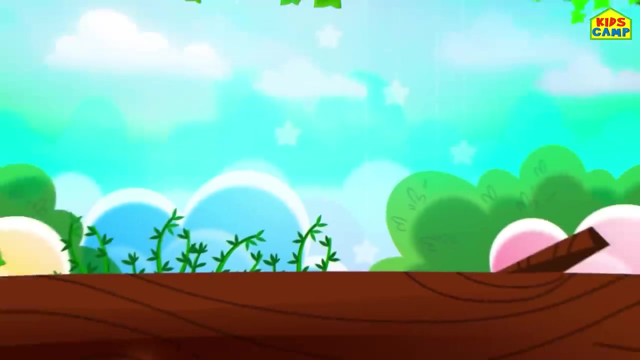 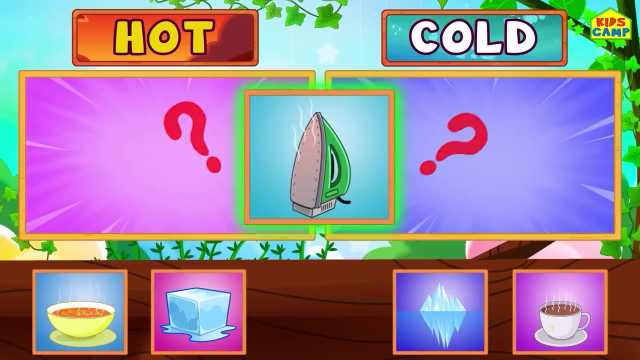 the volcano and the candle, And we found the snowman and the ice cream, All cold, Yay. What's next? This is an easy game: An iron Hot or cold Hot, That's right, An ice cube. 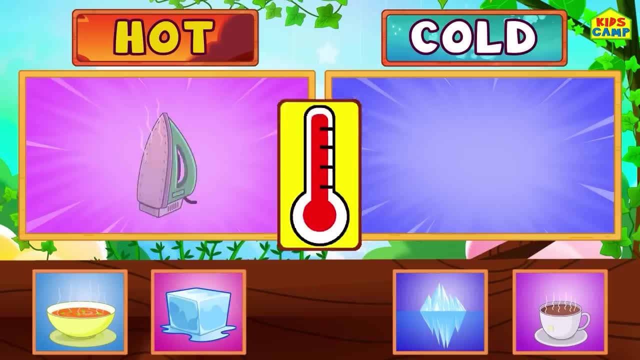 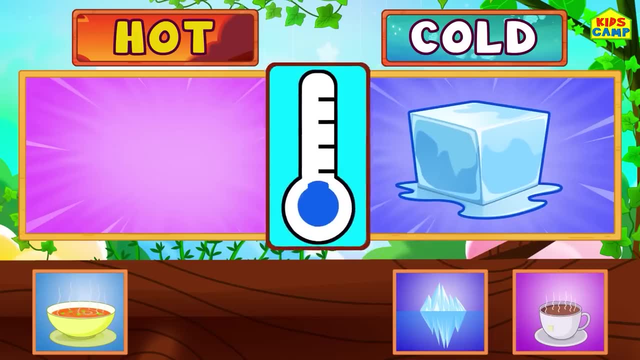 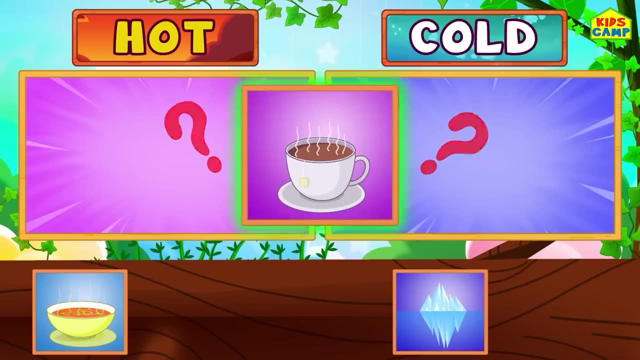 Hmm, cold, Very cold, That's right. Ice cream, That's right, And ice cream, That's right. That's right. A cup of coffee, Hot or cold? Hot, That's right. An iceberg, It's. 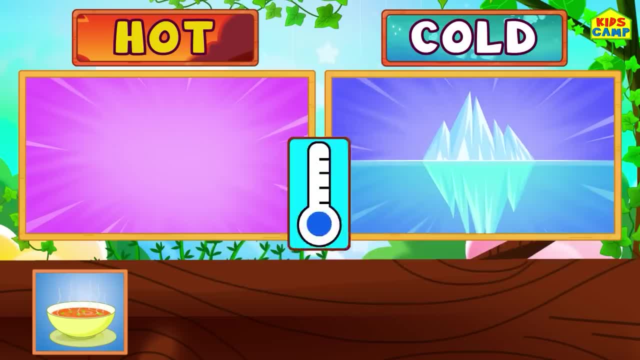 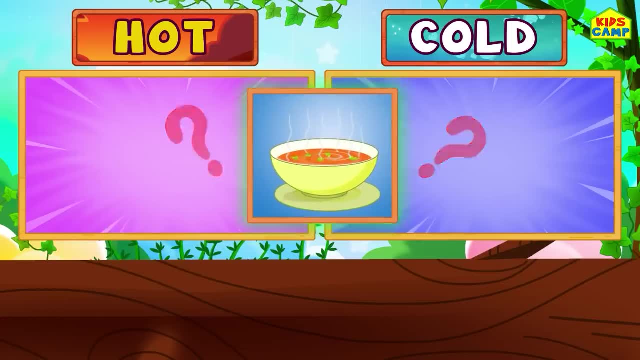 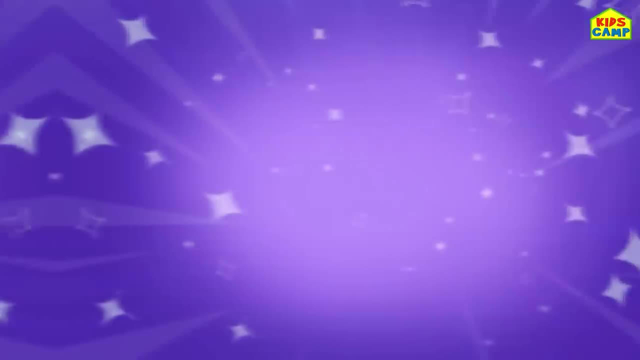 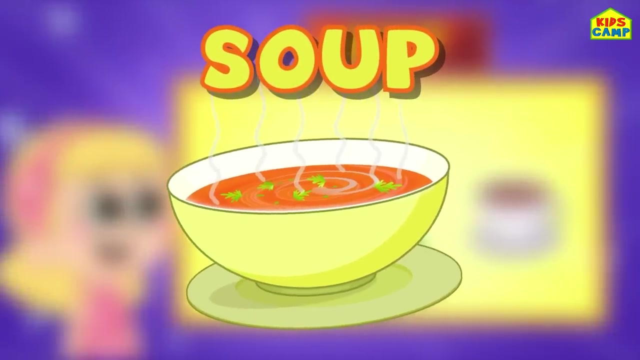 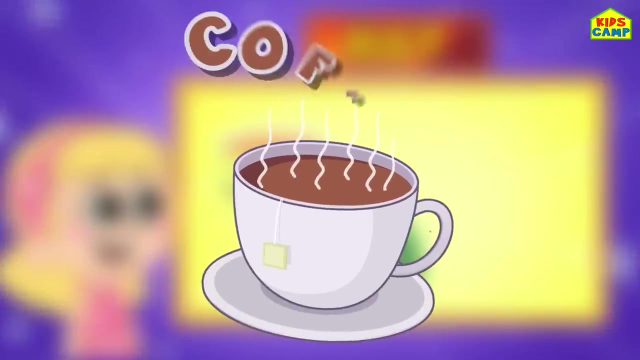 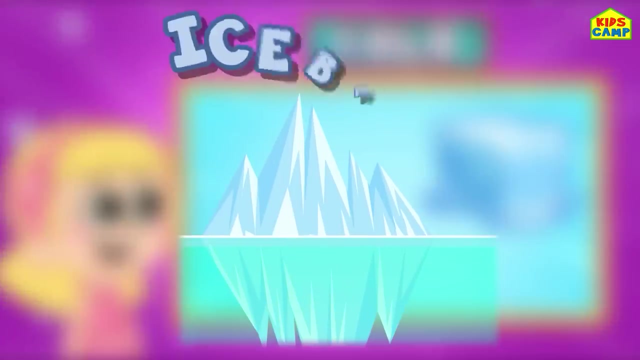 Cold. Good job. A bowl of soup, That's right. Hot, Wonderful. What did we learn? A bowl of soup is hot, An iron is hot And a cup of coffee is hot as well. An iceberg is cold And an ice cube is cold too. 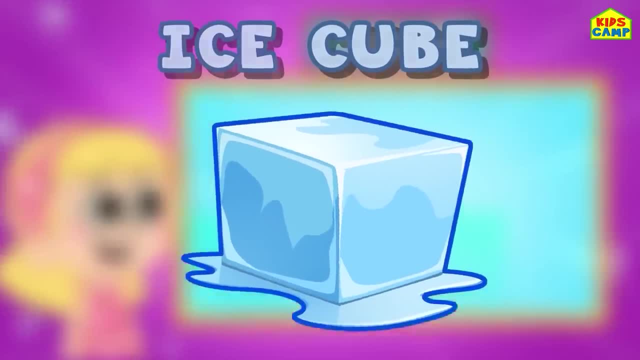 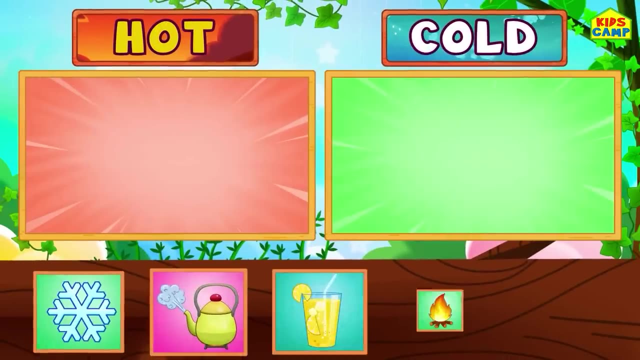 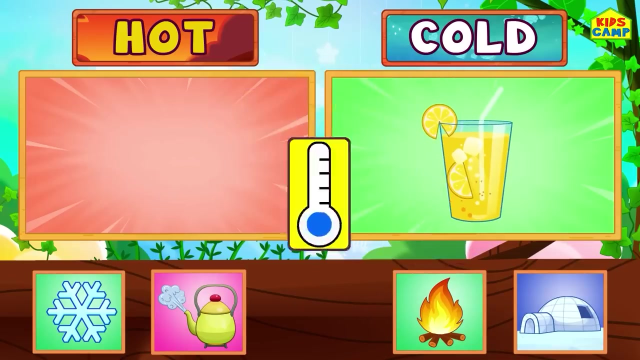 And an ice cube is cold too. And an ice cube is cold too. That's right, Yay. What's next? We're getting good at this game. A lemonade? Hmm, It's cold, Definitely cold. A kettle: 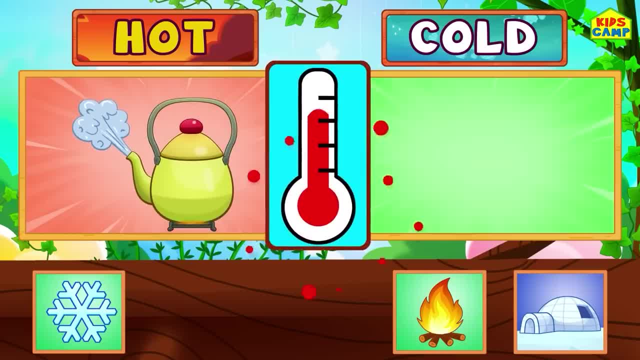 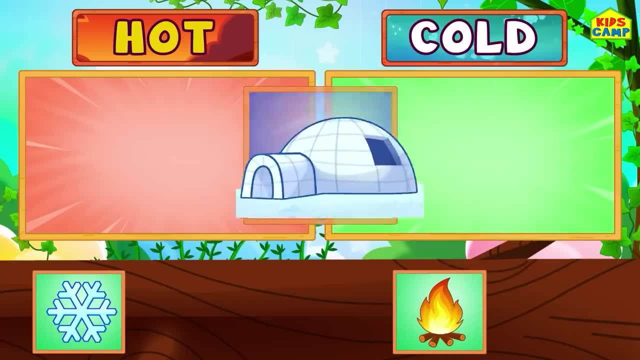 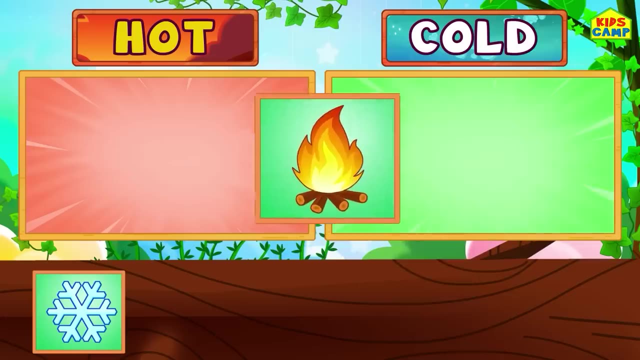 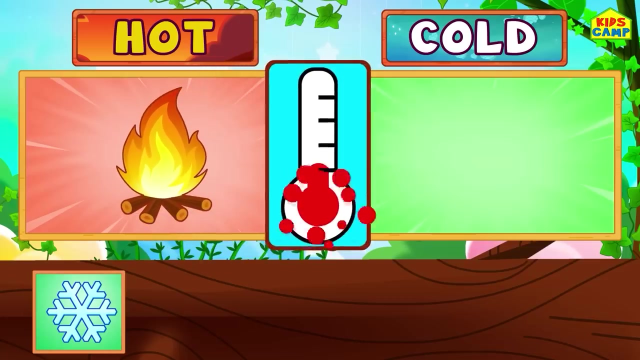 It'shot, That's right. Hot kettle, An igloo, An igloo, That's cold, That's cold, That's cold, Fire, Fire, That's hot, That's hot, Definitely hot. Good job, friends. 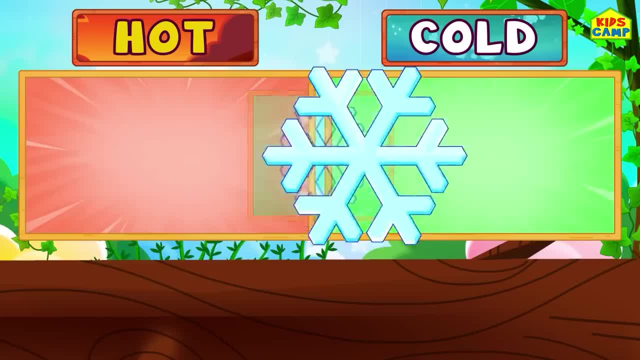 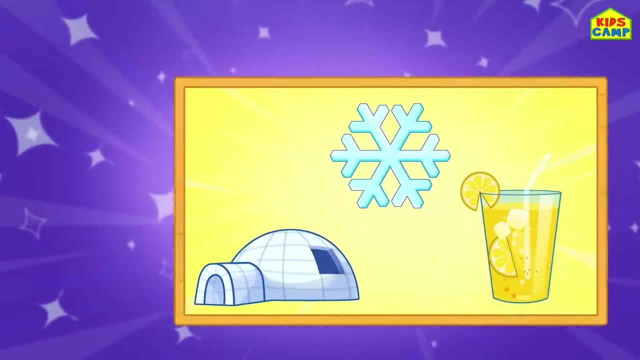 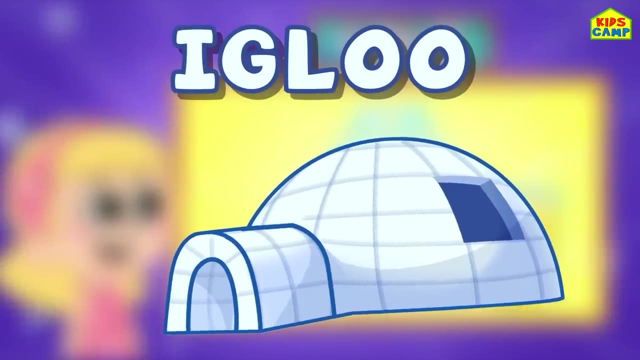 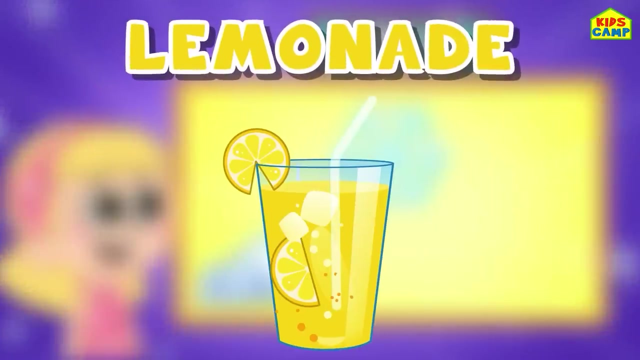 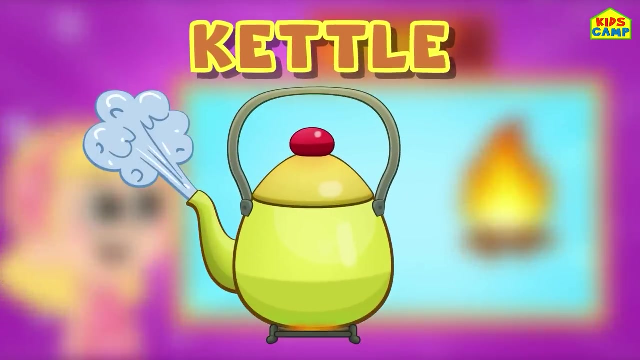 And a snowflake, And a snowflake That's cold, Wonderful, Wonderful. What did we learn? An igloo is cold, A snowflake is cold And a glass of lemonade is definitely cold. A kettle is hot And fire. 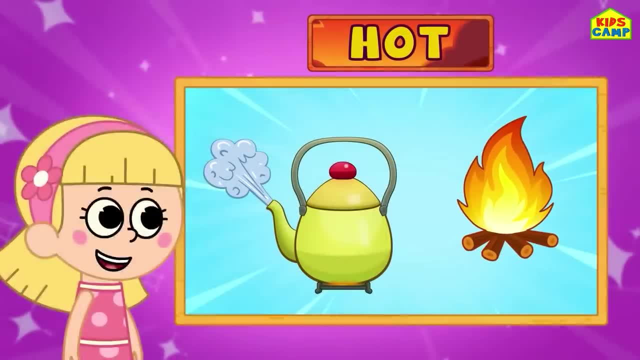 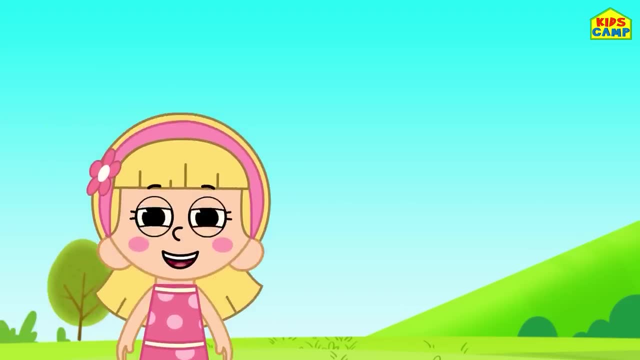 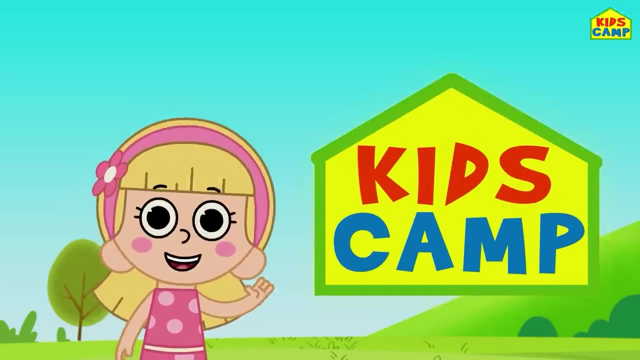 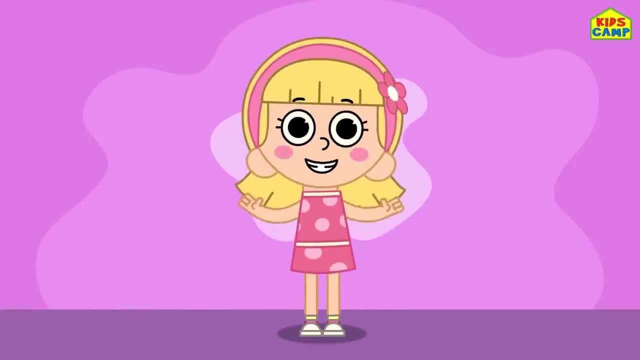 And fire is hot. Wonderful, Yay, This is so much fun learning. Come back for more. Until then, keep watching Kids Camp. Bye, Hi kids. I'm Ellie And today is Eva's birthday. Yay, Will you help me plan a birthday party for her? 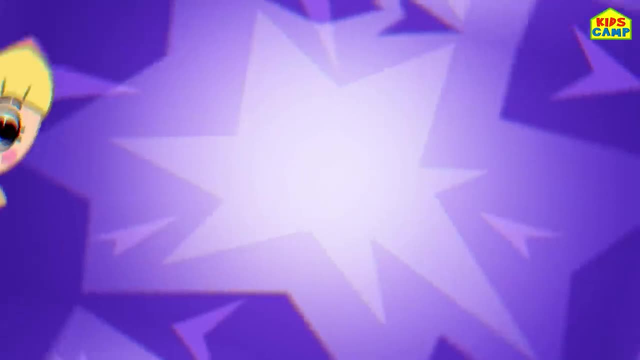 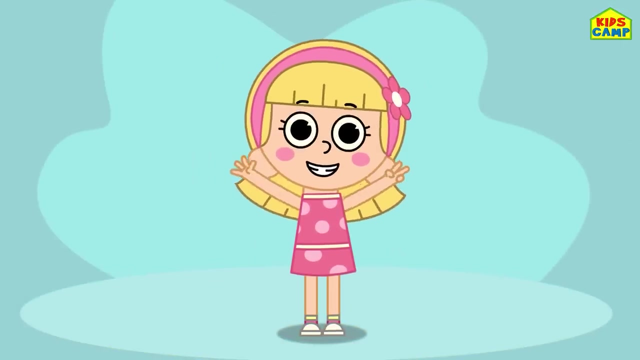 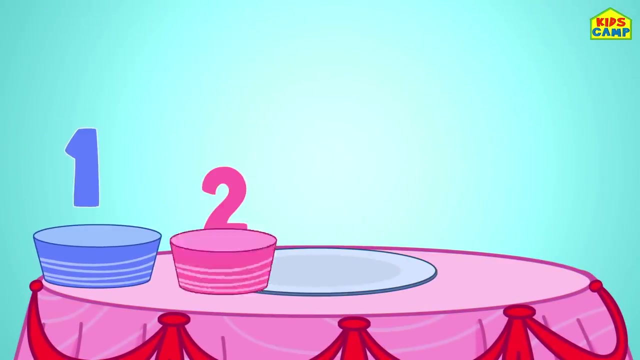 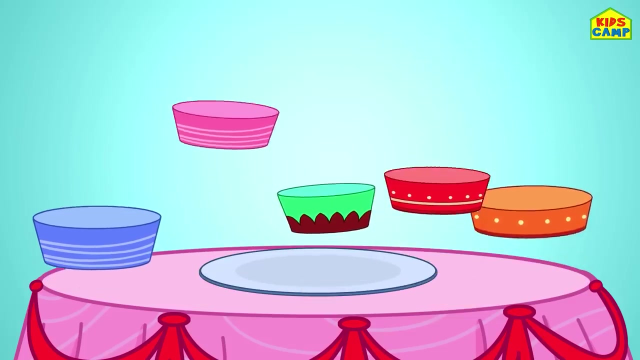 Yes, Let's go First. we'll need a birthday cake. Let's bake one. Hmm, How many layers of sponge do we add to Eva's birthday cake? Let's count One, two, three, four, five, Five layers of cake. 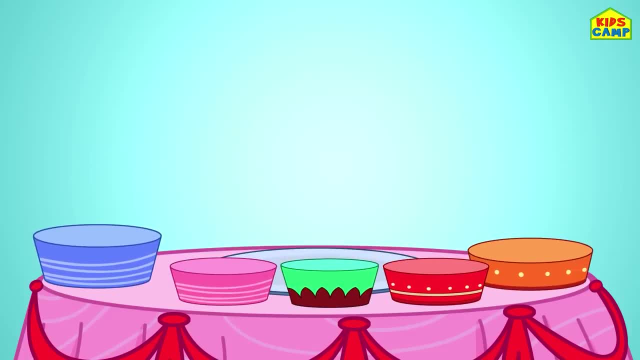 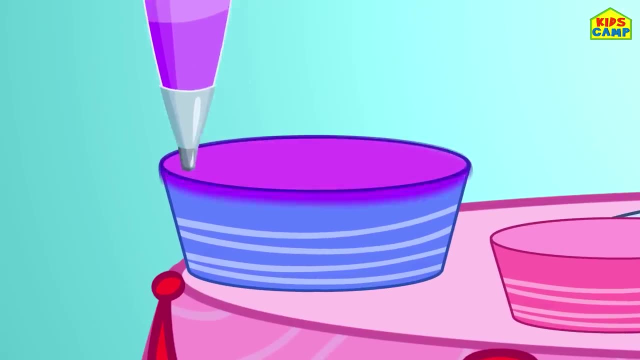 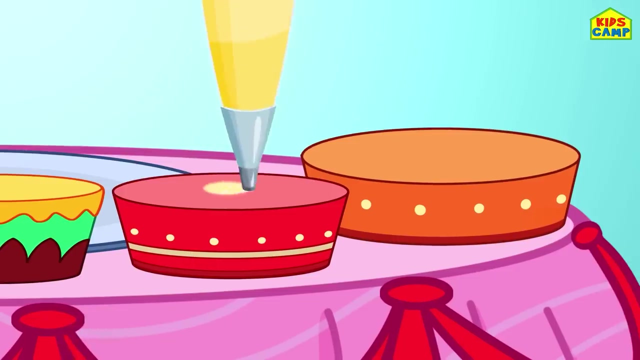 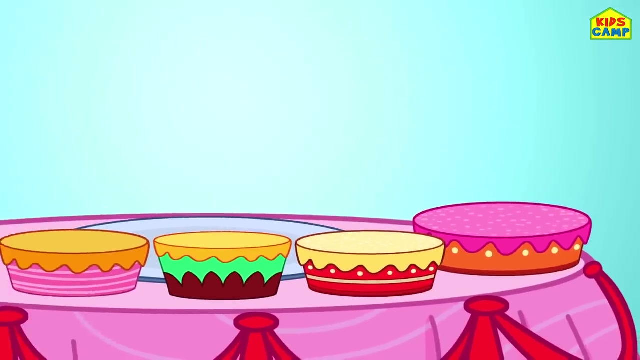 Hmm, What else can we add on the cake? That's right, Icing. Let's add On the first layer, On the second, On the third, On the fourth And the fifth- Woohoo, Five layers of icing. 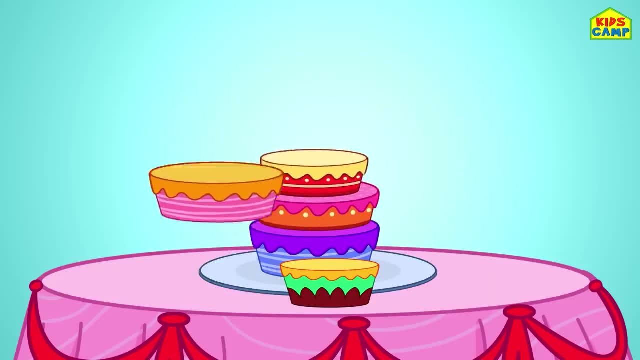 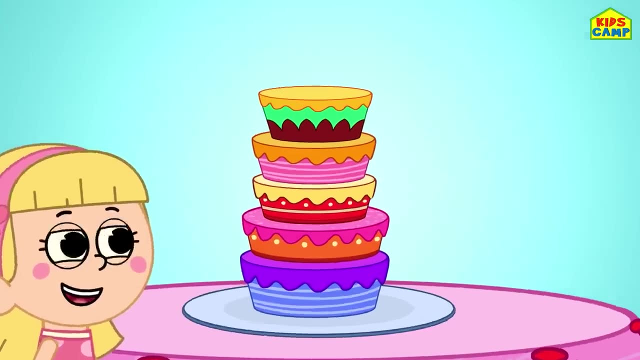 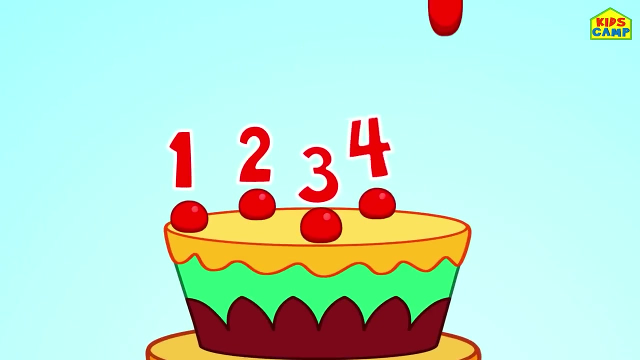 It looks yummy. Wow, Now let's add toppings. Woohoo, Let's add one cherry, two cherries, three cherries, four cherries, five cherries, Yay, Five cherries, Woohoo, Hmm. 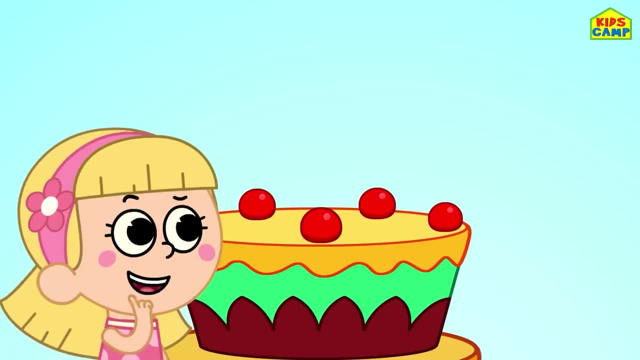 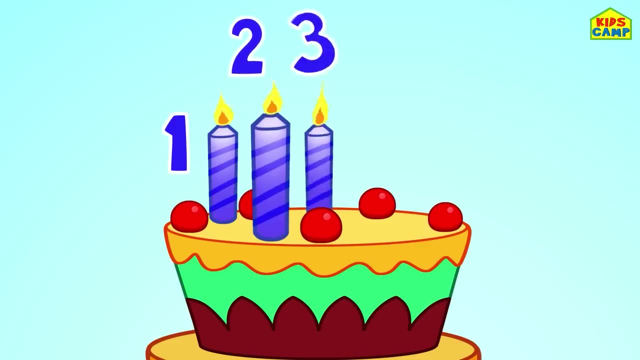 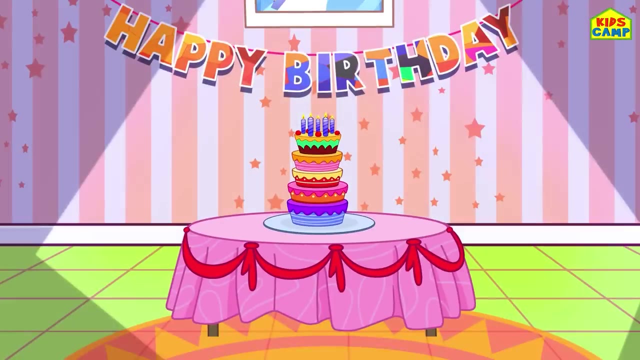 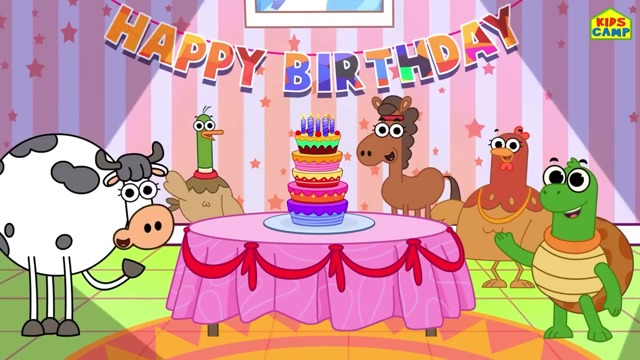 What do you think is missing? Hmm, Candles, That's right, Let's add candles: One candle, two candles, three candles, four candles, five candles. Yay, Wow, Everyone's here. Hi, everyone, We need party hats. 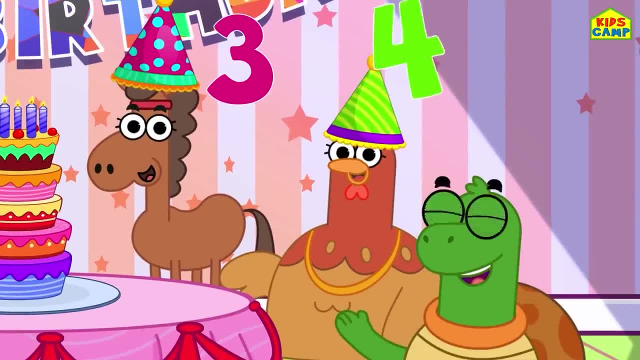 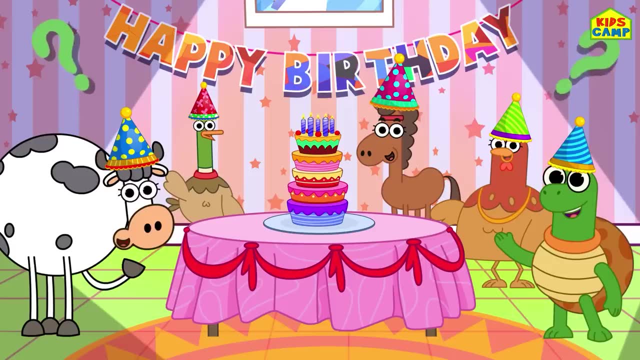 How many party hats do we need? One, Two, Three, Four, Five, Five party hats? Hmm, What else do we need? we need- hmm, something's missing. that's right, we need balloons. one, two, three, four, five, five balloons. this is now starting to look like a birthday party. 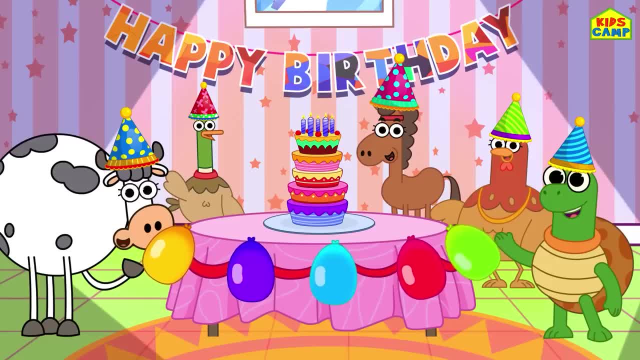 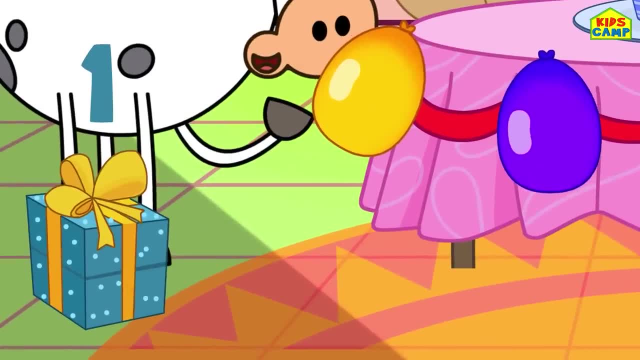 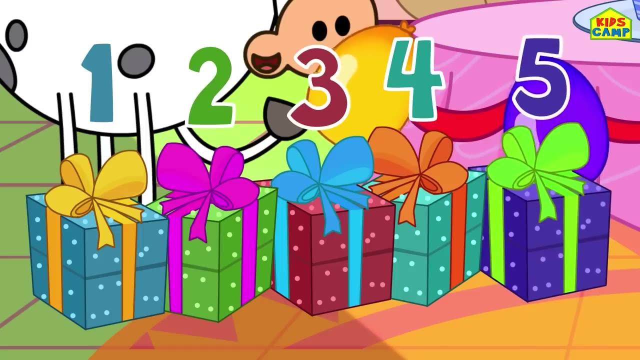 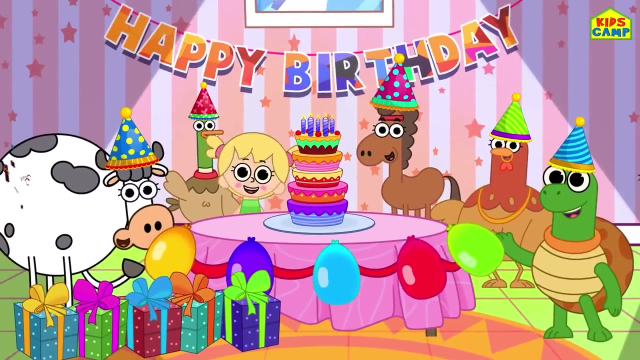 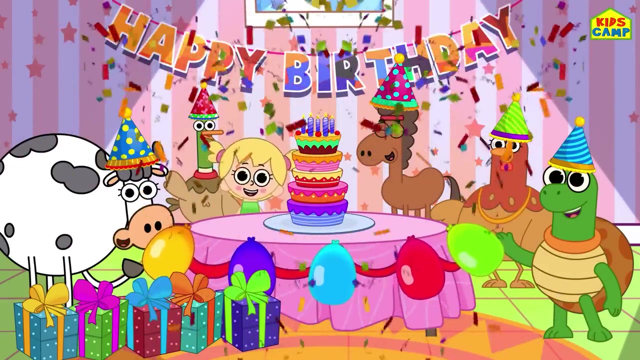 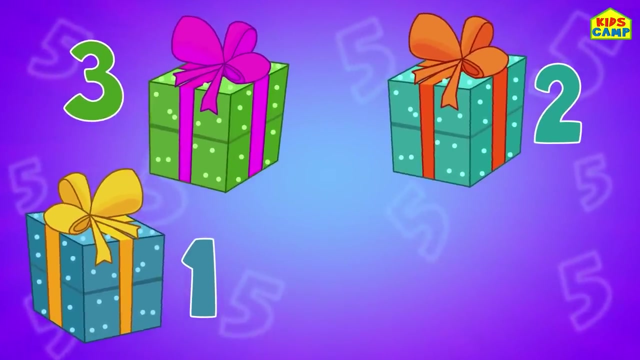 everyone's got presents for eva. let's keep them here and count. here we go: one, two, three, four, five, five presents. let's get this party started. where's eva? there she is surprise. happy birthday eva. this was so much fun, and so is counting. let's do it again: one, two, three, four, five, five presents. 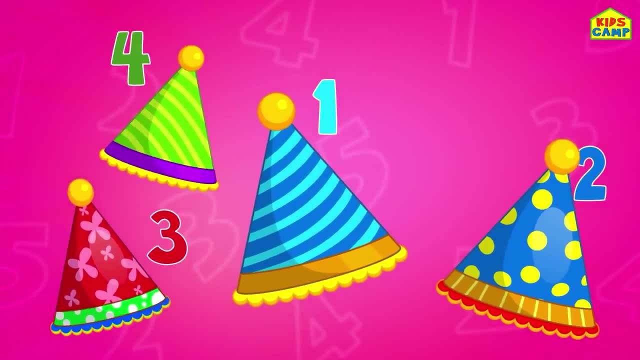 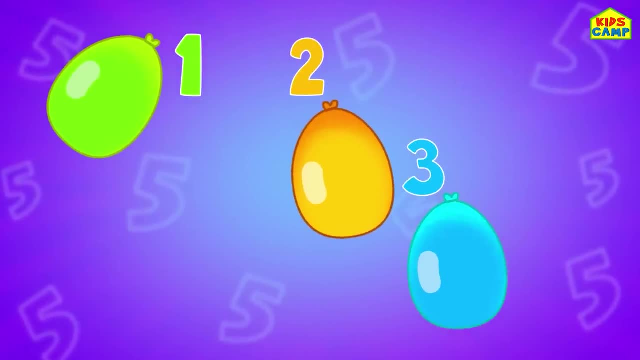 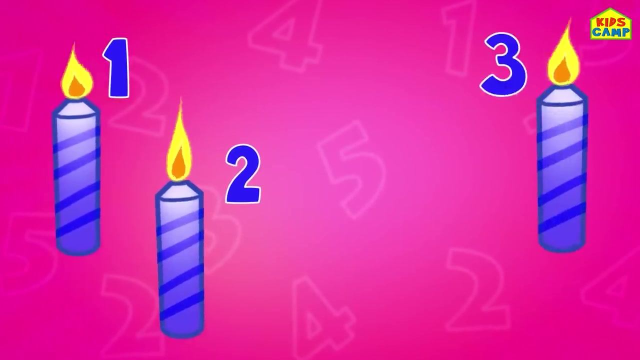 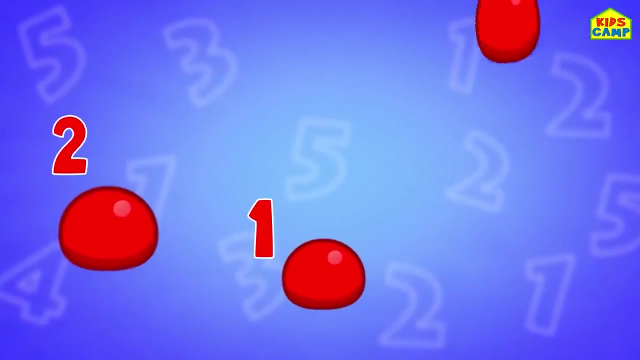 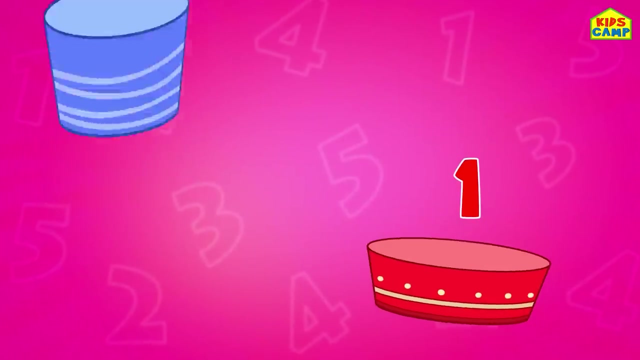 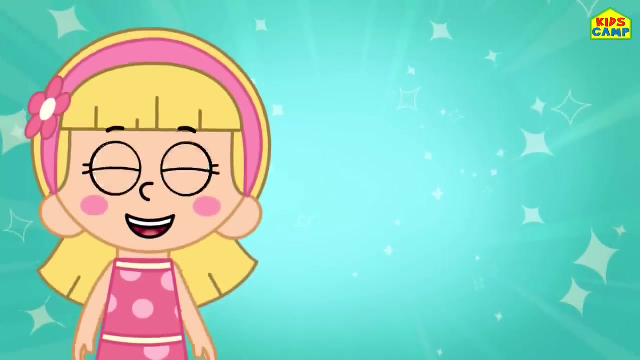 one, two, three, four, five, five. party hats: one, two, three, four, five five. balloons: one, two, three, four, five five. candles: one, two, three, four, five five. cherries: one, two, three, four, five, five layers of cake. this was so much fun. it was the best party ever. bye, bye. 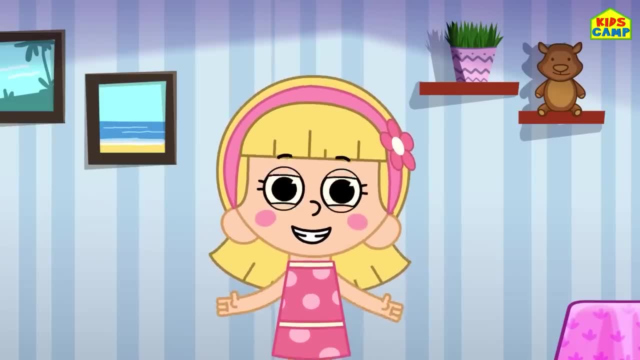 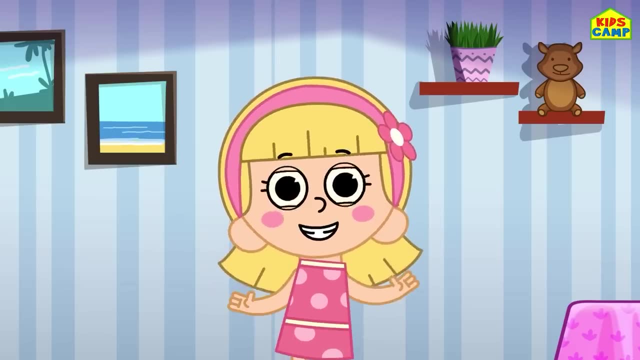 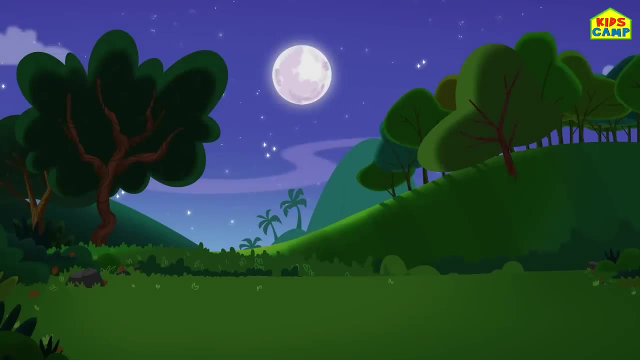 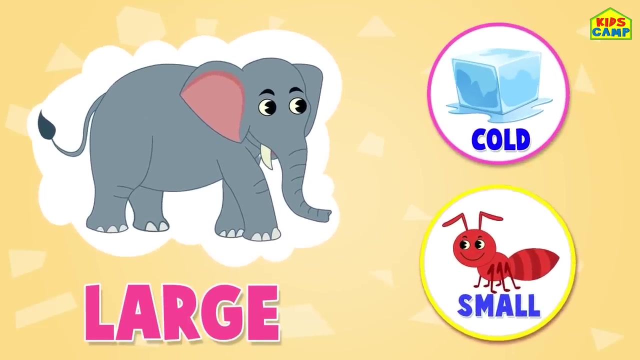 hi, i'm ellie, and today we are going to learn opposites. what is an opposite? an opposite is when two words contradict each other. for example, if it's daytime, the opposite of day is night. right ready, here we go. what is the opposite of large? is it small or cold? 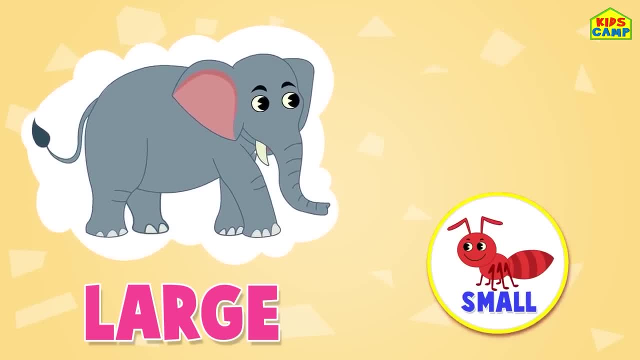 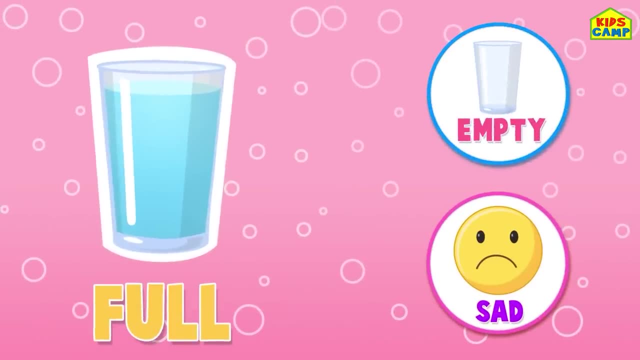 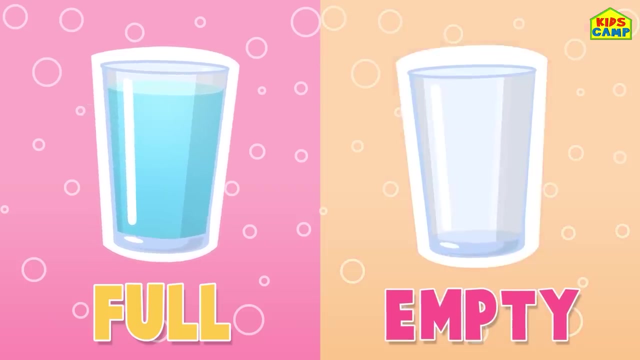 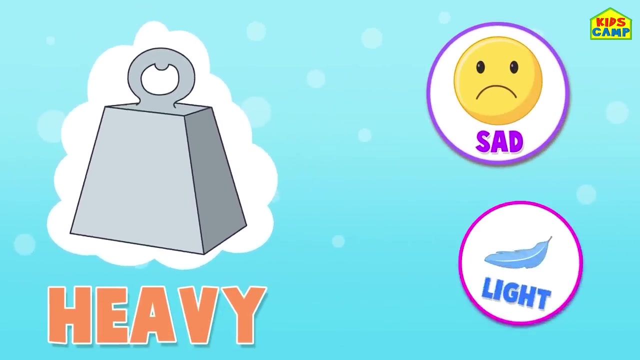 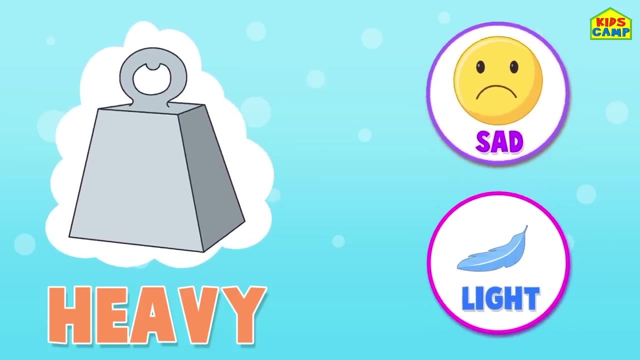 it's small. that's right. the opposite of large is small. what is the opposite of full? is it sad or is it empty? the opposite of full is empty. that's right. what is the opposite of heavy? is it light or sad? it's light. the opposite of heavy is light. 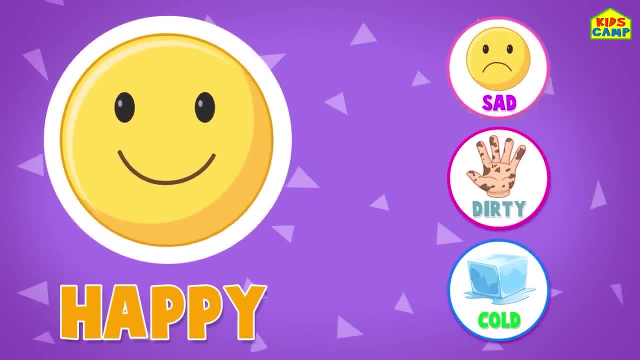 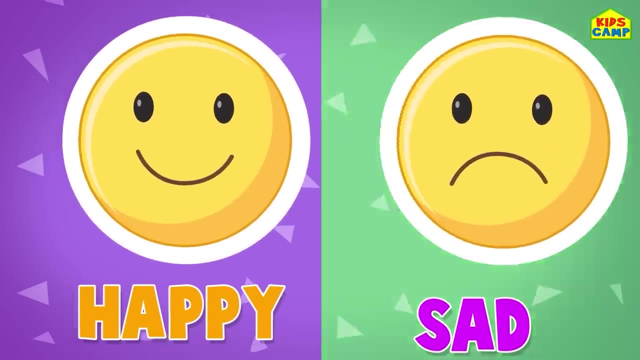 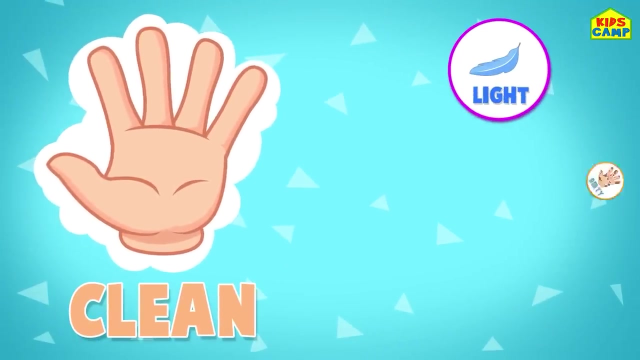 what is the opposite of happy? is it sad, is it dirty or is it cold? it's sad, That's right. The opposite of happy is sad, And I feel happy right now, Yay. What is the opposite of clean? Is it cold, Is it light Or is it dirty? 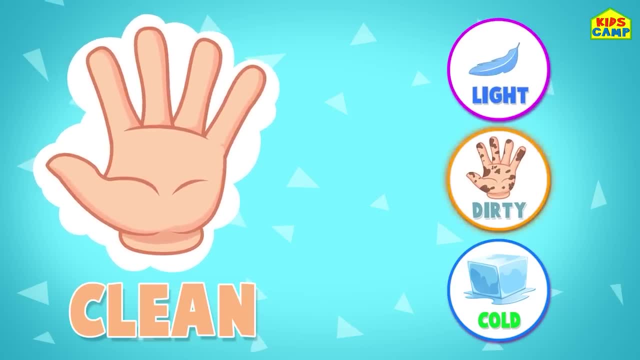 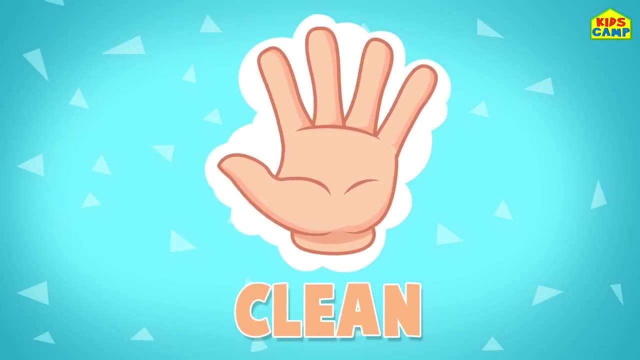 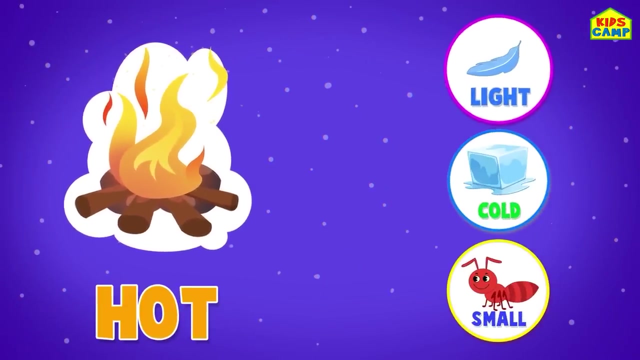 That's right, friends, It's dirty. You should always keep your hands clean and not dirty. What's the opposite of hot? Is it light, Is it small Or is it cold? It's cold, That's right. The opposite of hot is cold. 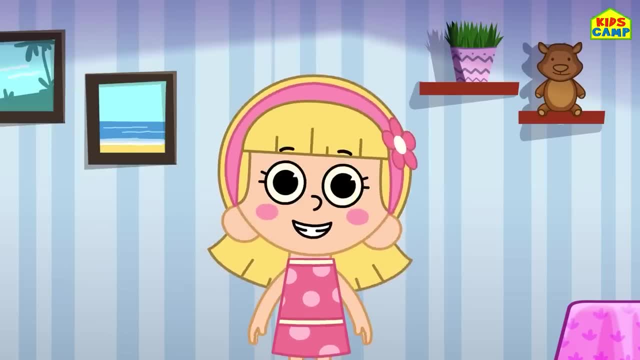 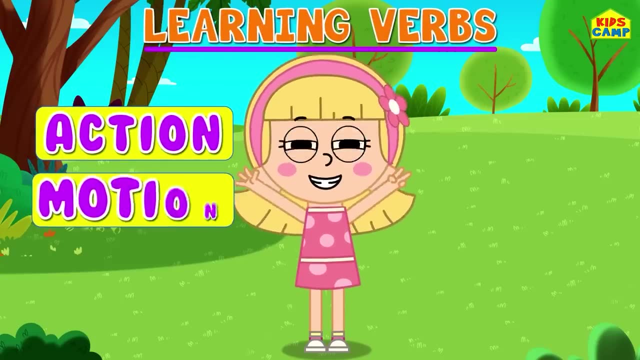 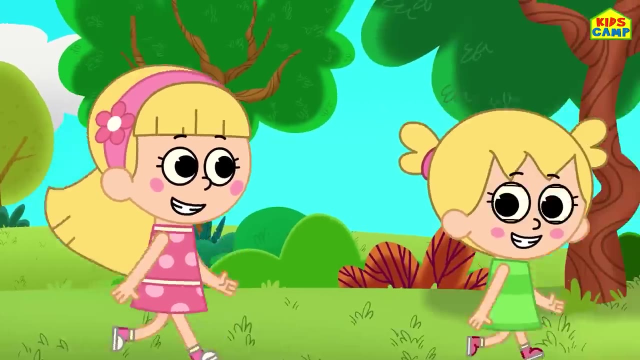 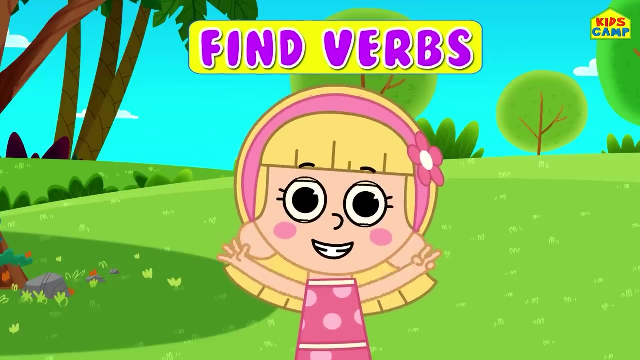 Cool. Good job, friends. Well done Hi. Verbs are words that show action, motion, doing or a state of being. And I am on a playground And I am playing with Eva. What we are going to do today is find verbs. 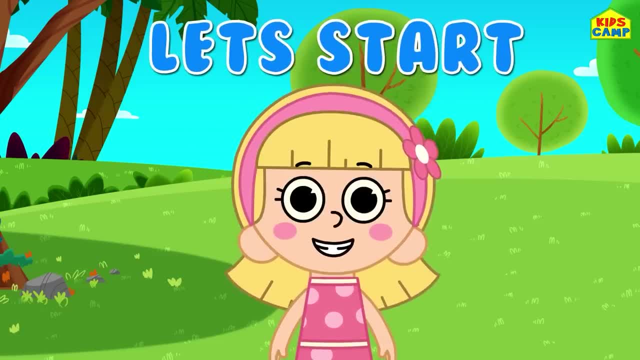 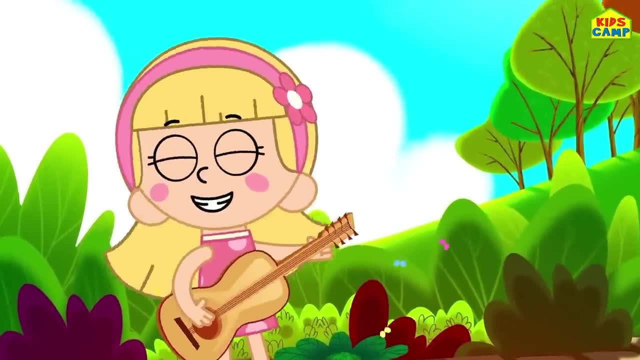 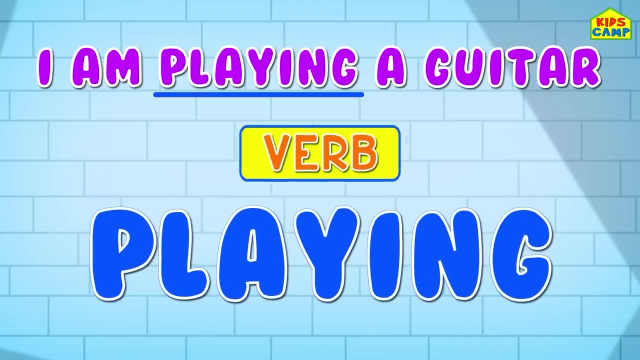 Are you ready? Let's get started right away. We have to look for the verb. Can you find what's the verb in the sentence I am playing? the guitar Playing is the verb here. That's right. What's the activity I am doing here? 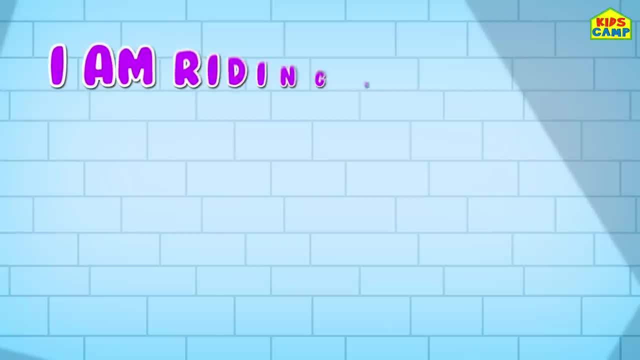 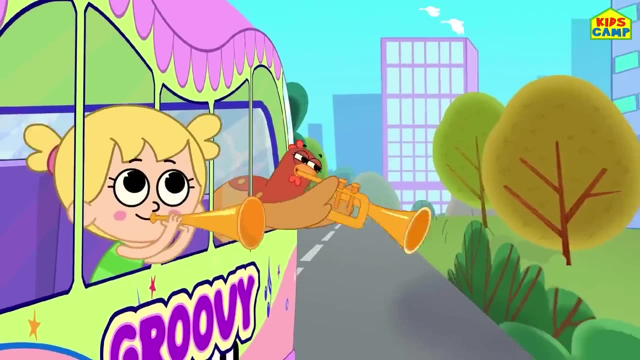 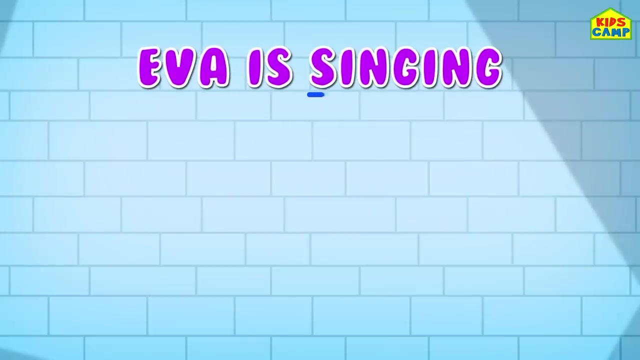 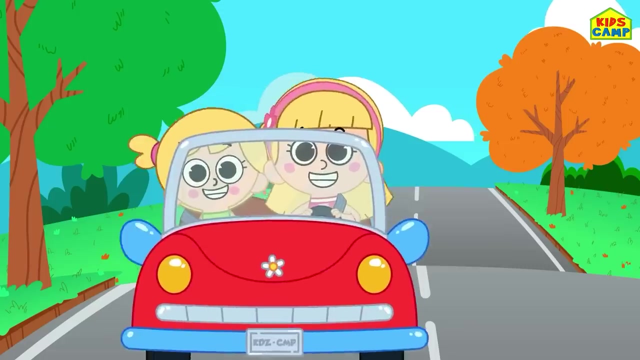 I am riding a bicycle. That's right. Riding is a verb. Woohoo, Look at my little sister, Eva. She loves to sing. That's right, Eva is singing. Singing is the verb here. Good job, friends. Look at me, I am driving. 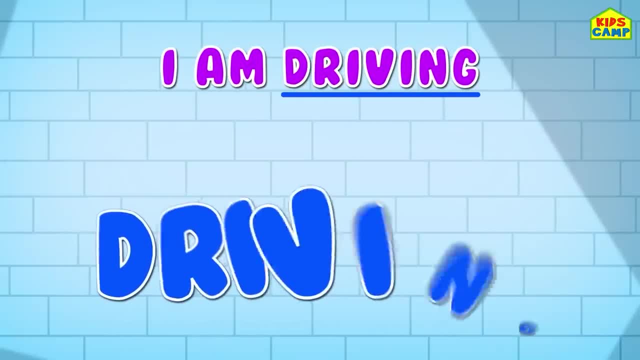 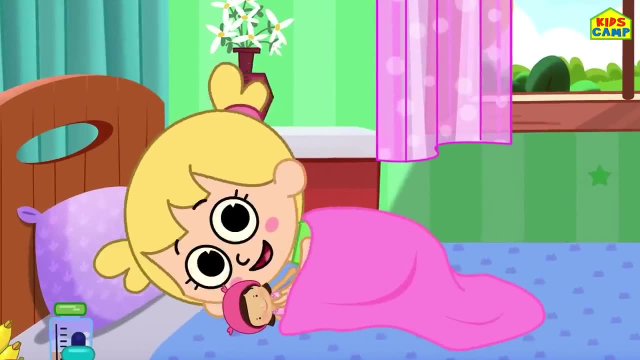 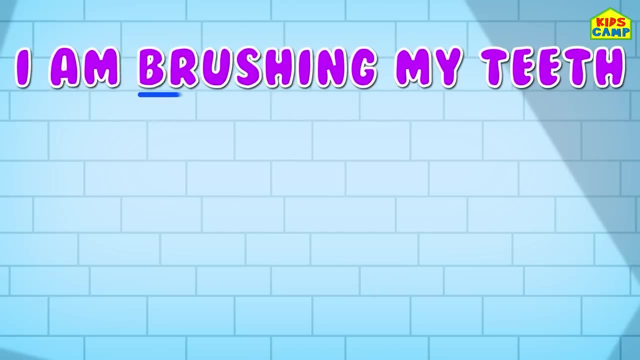 Yay, That's right, Driving is the verb here. And what is it that we do? We do the first thing when we get up in the morning. That's right. We brush our teeth. I am brushing my teeth, Brushing is the verb here. 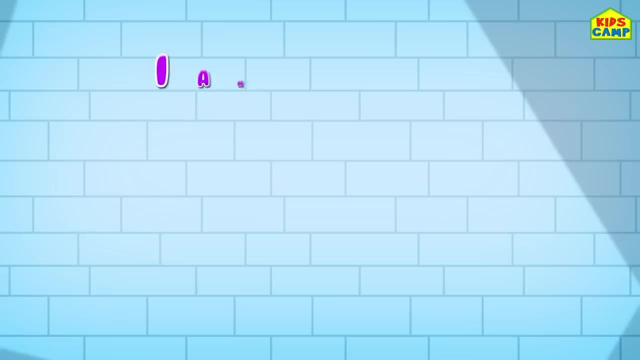 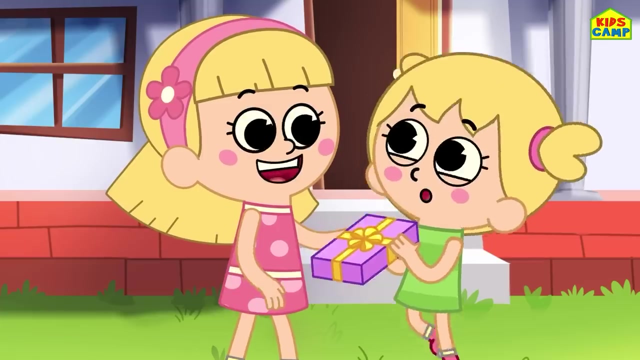 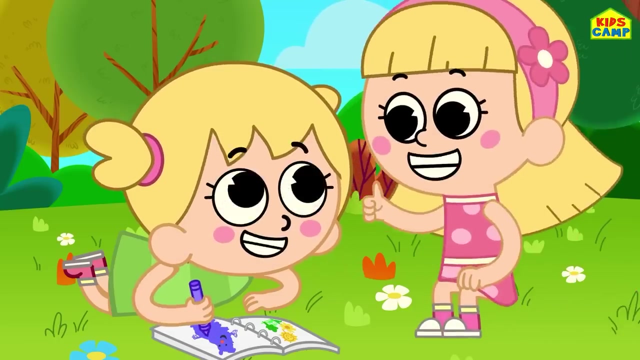 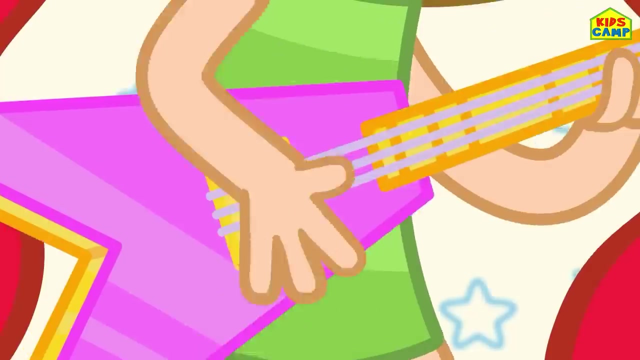 Eva and I love to cook. I am cooking- Cooking is the verb here- And I've got a new box of crayons. I love to use my crayons to draw and color. I am coloring- Coloring is the verb here. Woohoo. 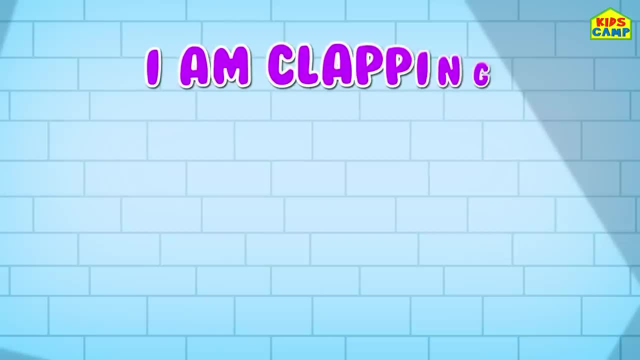 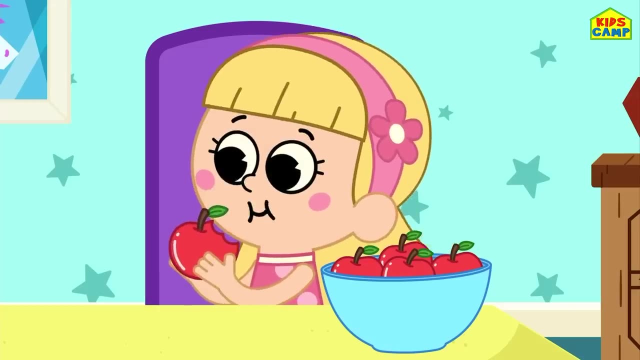 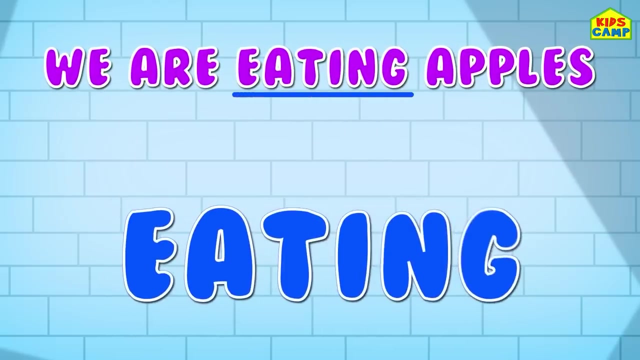 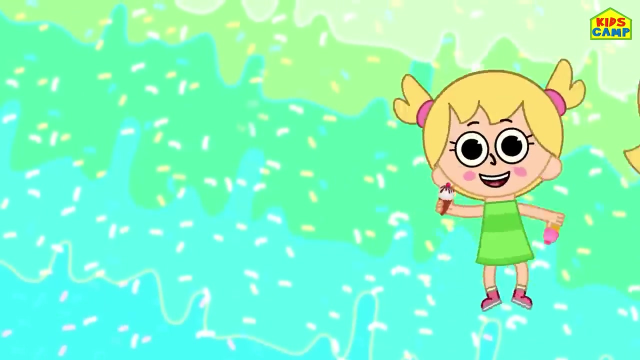 I am clapping, I am clapping. Clapping is the verb here. Woohoo, We are eating apples. We are eating apples. Eating is the verb here. Woohoo, That's right, We are dancing. We are dancing. 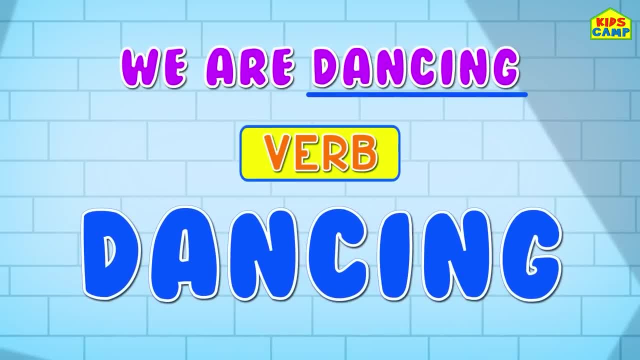 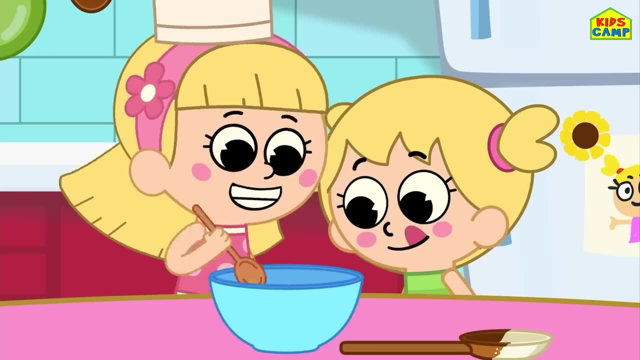 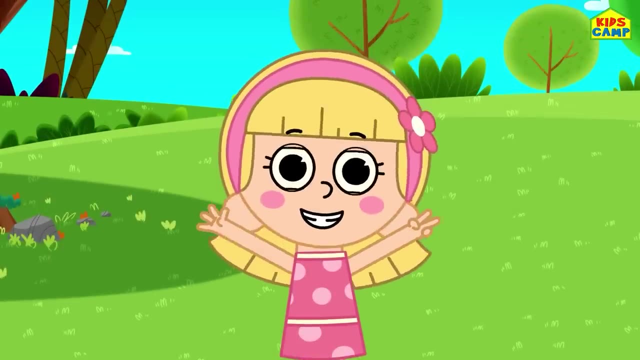 Dancing is the verb here. Wow, This was so much fun. What do you like to do? Do you like to cook, play guitar, paint, sing or ride a bike? Let me know. Until then, keep watching Kids' Camp. 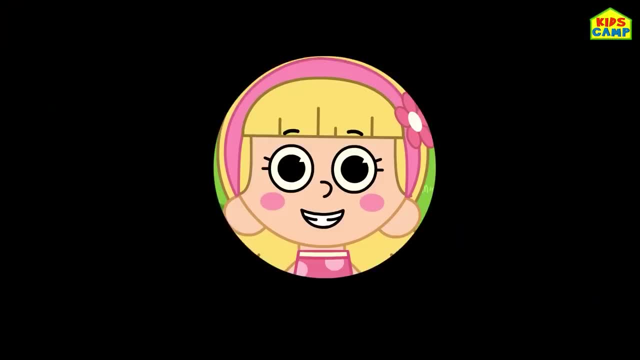 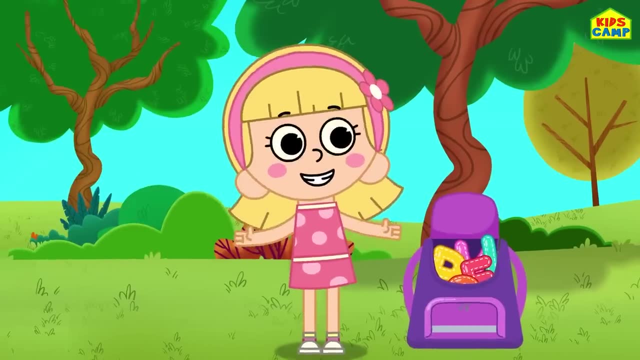 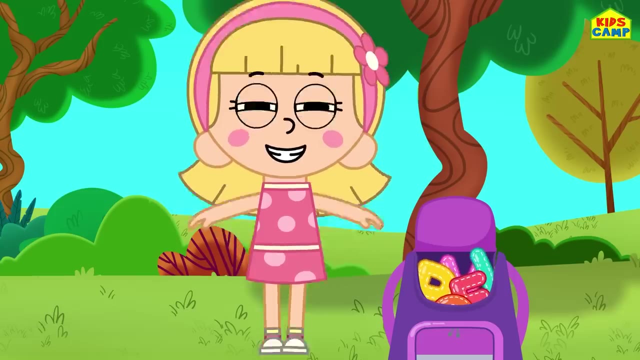 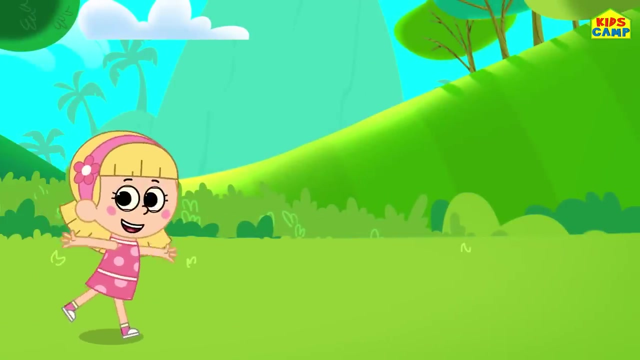 Bye-bye, Hi kids. I am Ellie And I have a bag of alphabets with lots of scrambled and jumbled letters. We have to unscramble them to find the correct word. Fun game- Let's start, Alright. 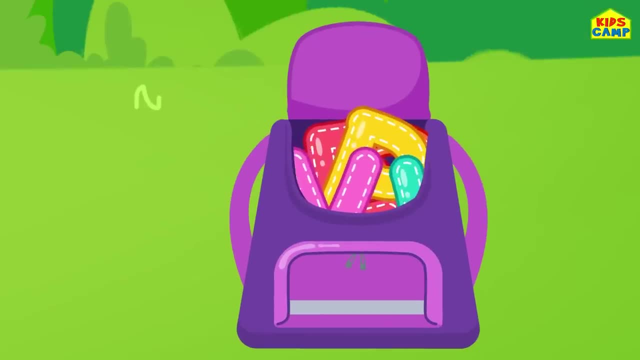 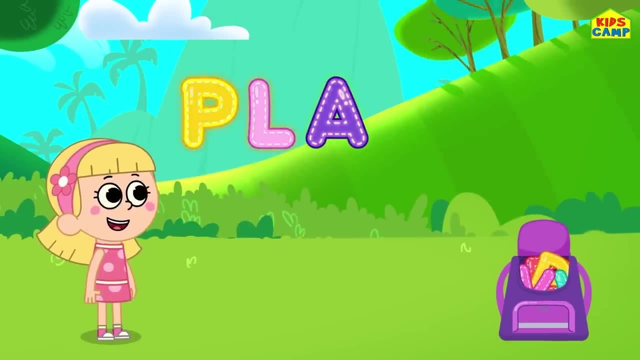 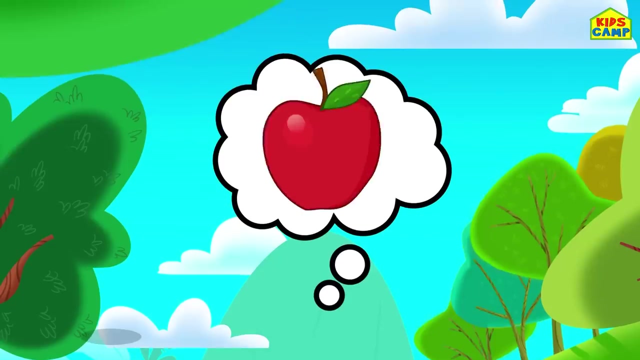 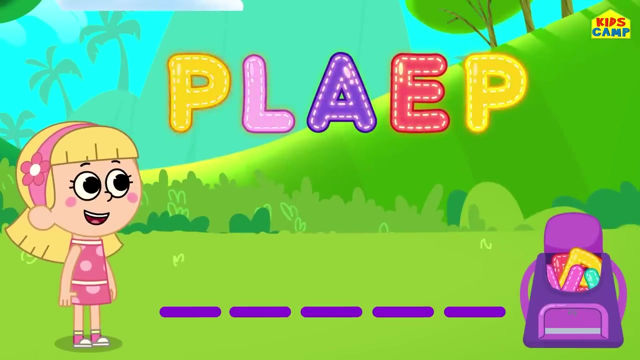 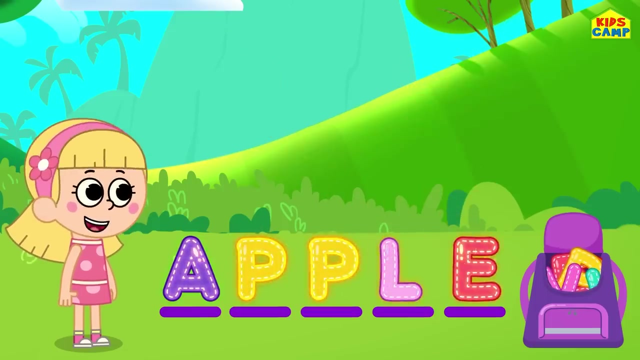 What is this? Hmm, I wonder what it is. Ah, P, L, A, E, P. Hmm, What word could this be? Oh, I know, This is an apple. It starts with the letter A, P, P, L and E. That's right, We got it right, kids. 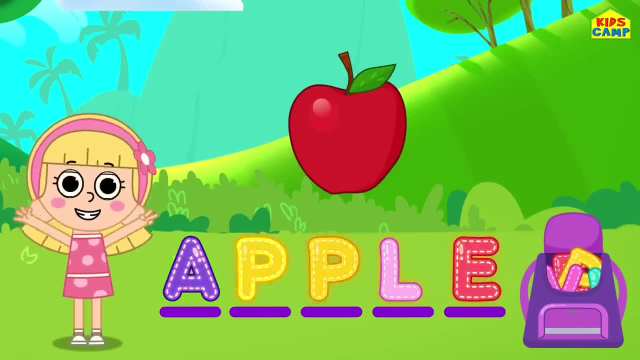 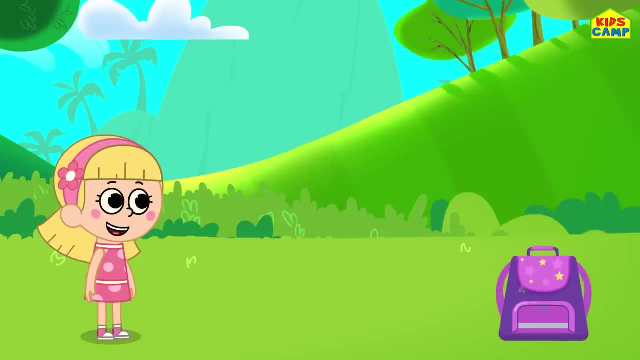 It's an apple. Woohoo, We got the first word correctly. What's next? Hmm, I wonder What could this be? The letter E, A, C and K? Hmm, This looks familiar. That's right, It's a cake. 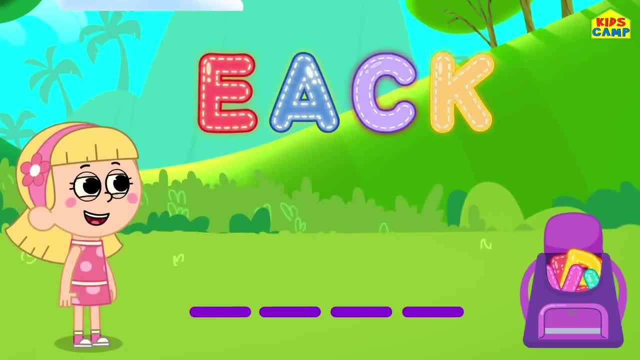 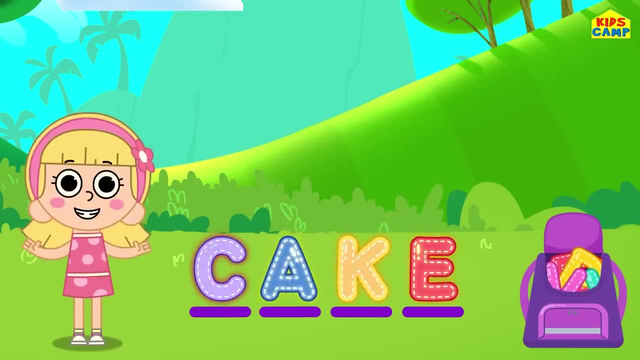 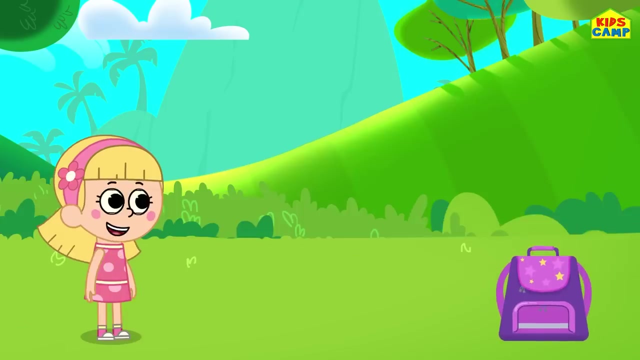 Yes, Yes, I know this one. It starts with the letters C, A, K and E. Yay, We did it again. What's the next word? Any guesses? Hmm, We have the letters U, D, C and K. What is this? 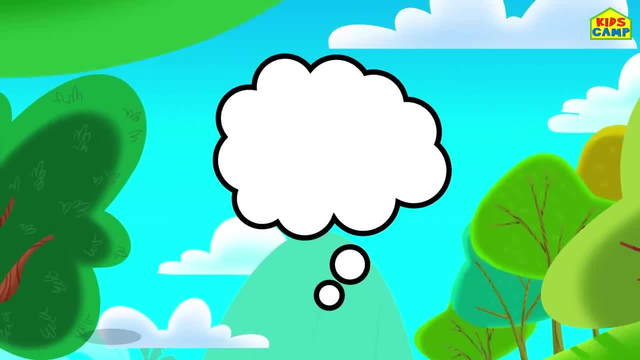 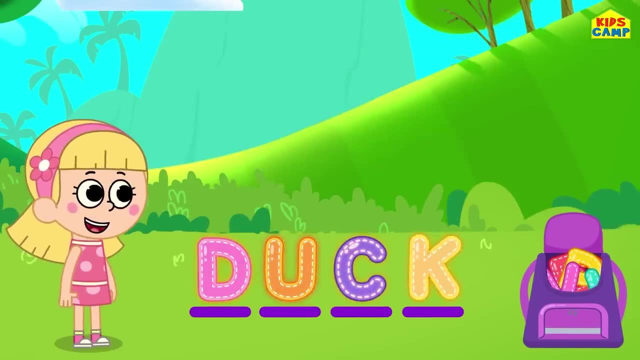 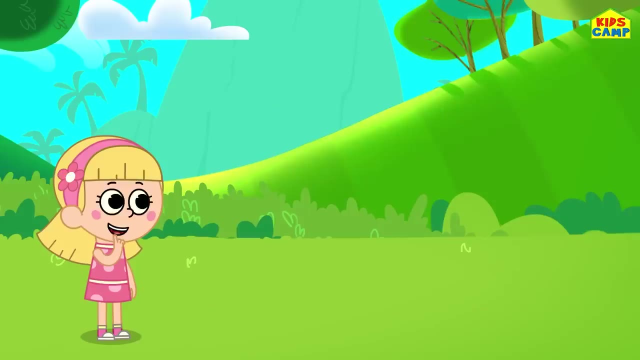 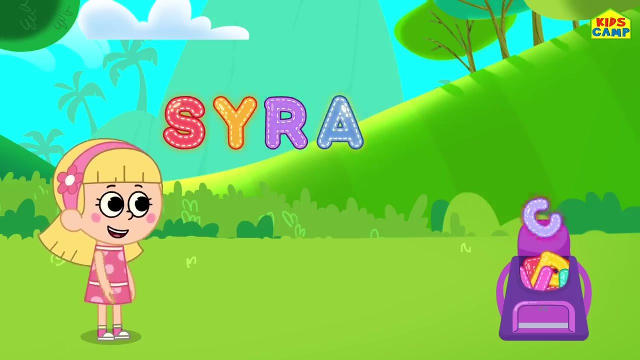 Hmm, It's a duck. It starts with the letter D, U, C and K. Duck Woohoo. Alright, Let's go to the next one. What does my bag of letters have now? The letters S, Y, R, A, C, O and N. 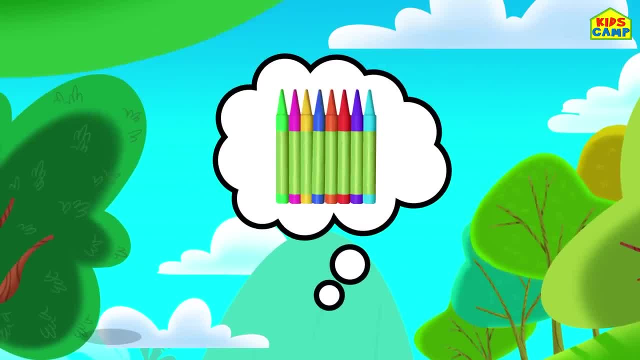 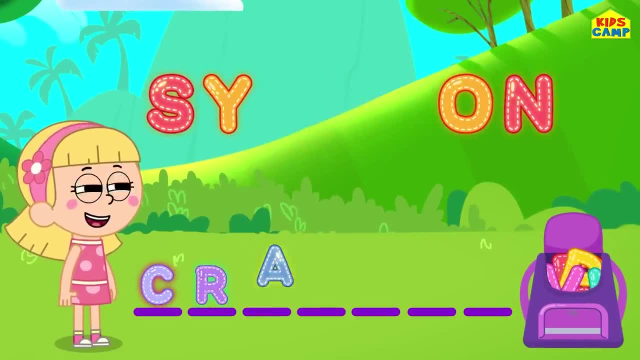 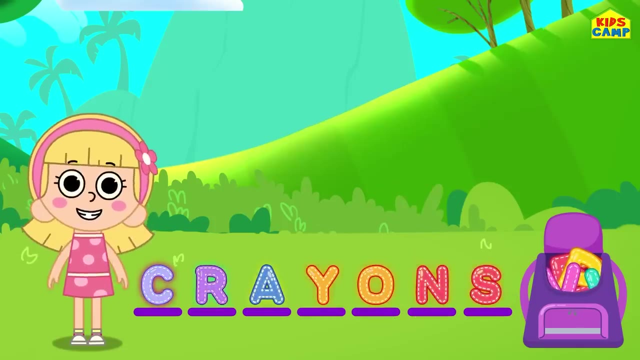 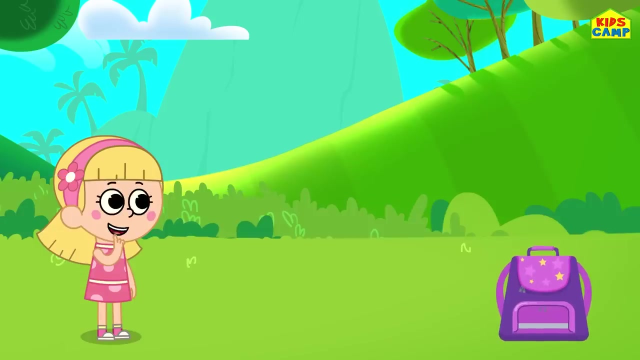 What could this be? These are crayons. That's right, kids, I love crayons. It starts with the letters: C R A Y O N S Crayons. That's right. Woohoo, One more. What will come out of the bag of letters? 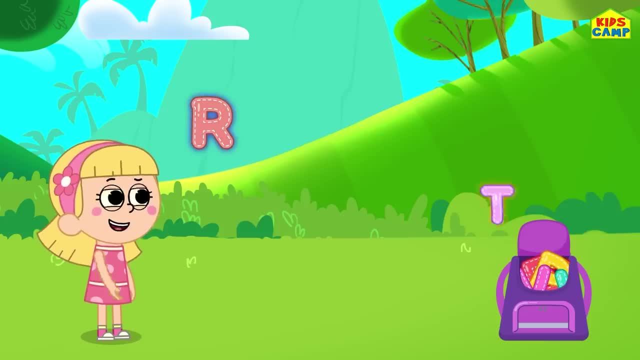 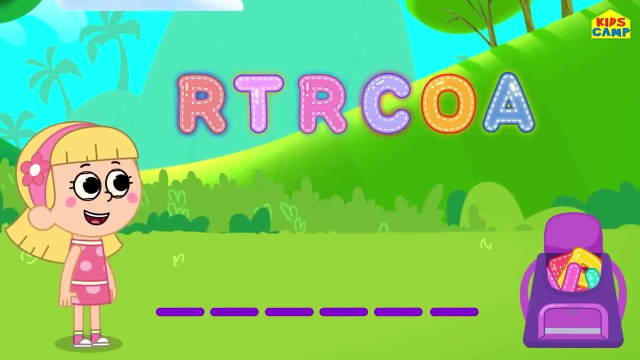 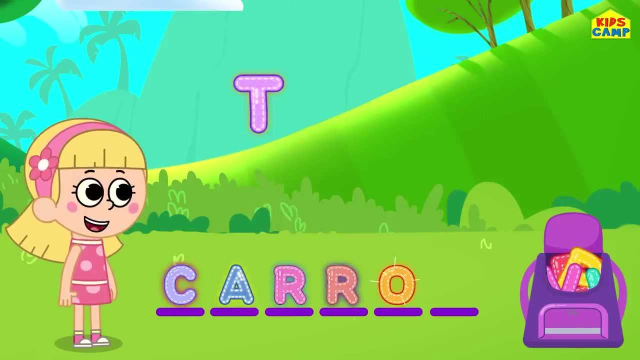 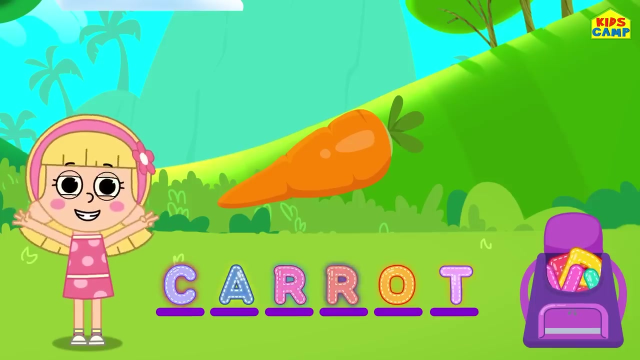 What letters? R, T, R, C, O, A. Hmm, What could this be? It's a carrot, That's right. That starts with the letters C, A, R, R, O and T, That's right, Carrot, Woohoo, Good job kids. 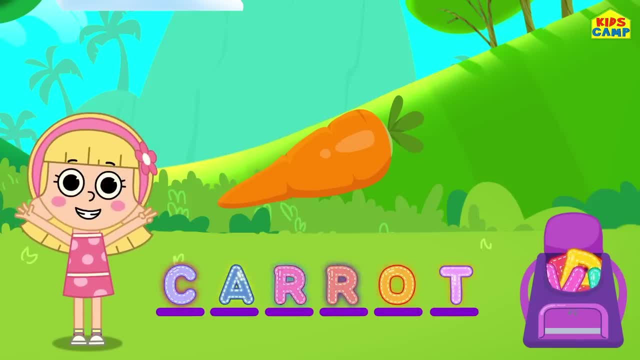 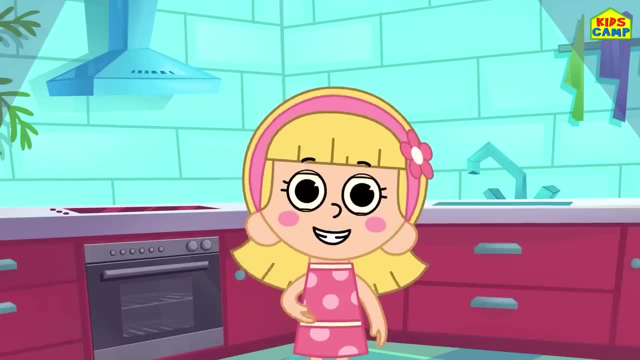 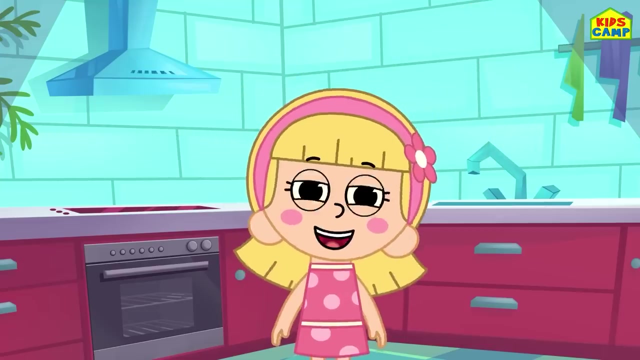 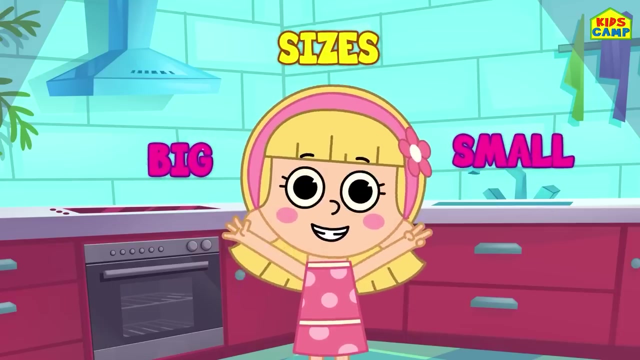 Well done. This was so much fun. Bye, Hi friends. I'm Ellie And I'm making some yummy treats for Eva. Okay, But first we have to sort them according to their sizes: Ready, Big or small. Will you help me, friends? 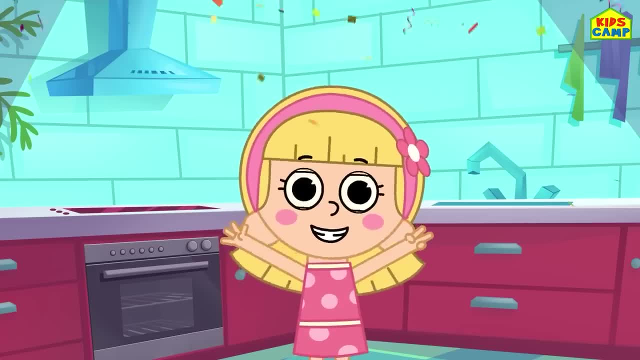 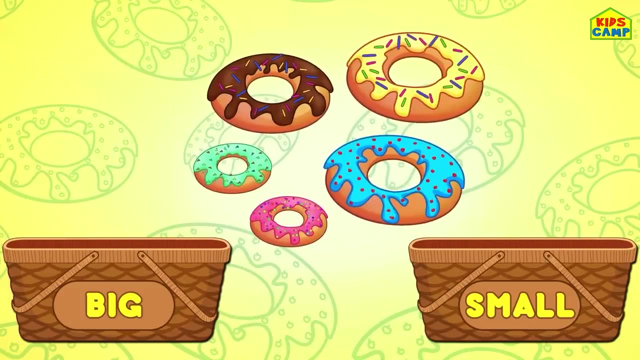 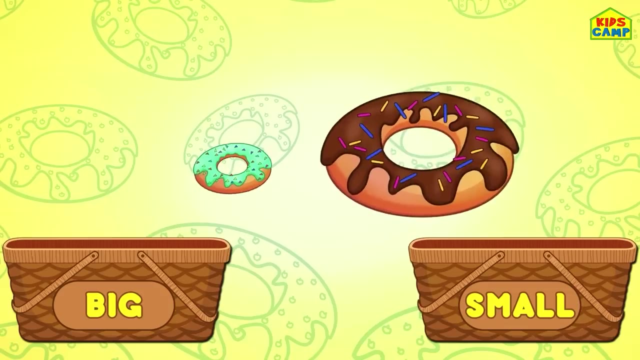 Yes, Then let's get started Right away. Wow Donuts- Yummy, I love them. Let's sort them according to their sizes. This chocolate donut looks bigger than this one, That's right. The bigger donut goes into the basket labeled big. 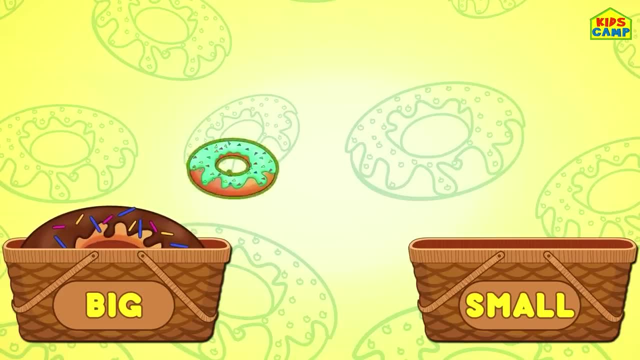 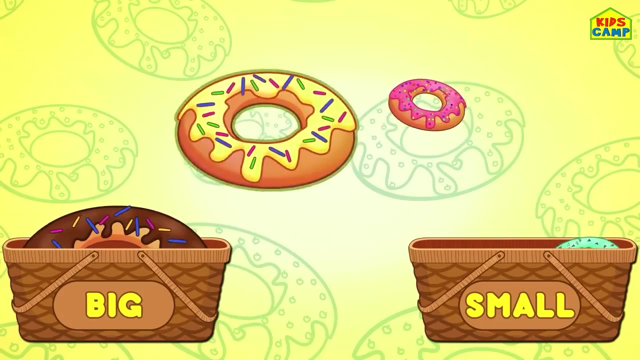 That's right. And the small donut goes into the basket labeled small. Yay, Yay, Let's compare these two. The pink donut is smaller than the yellow donut, That's right. The smaller one goes into the small basket. 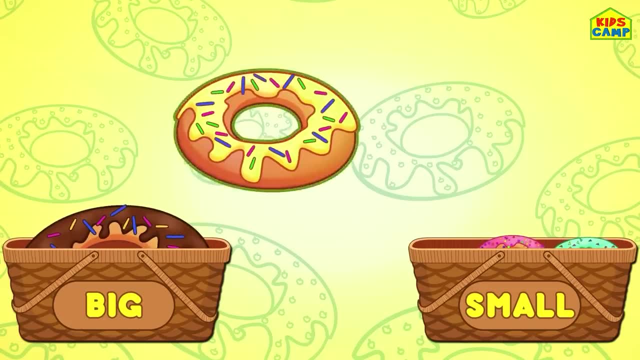 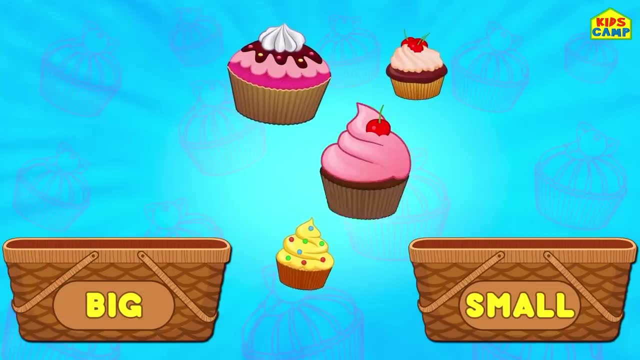 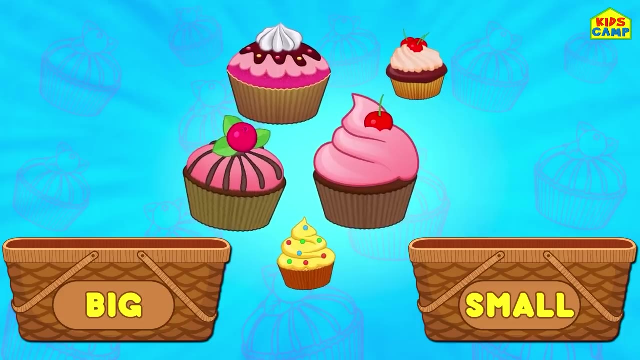 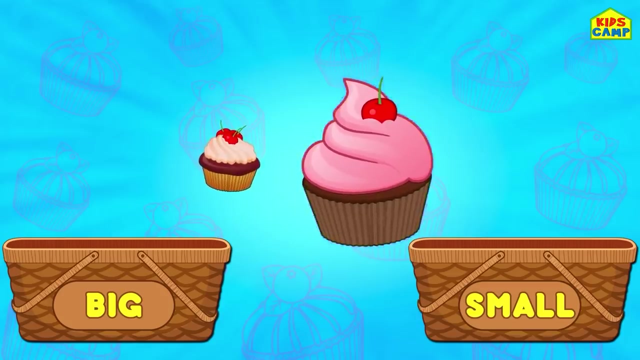 And the bigger donut goes into the big basket. That's right. I see a lot of cupcakes. Wow, Let's sort them according to their sizes. The pink cupcake is bigger than the other cupcake. The big pink cupcake goes into the big basket. 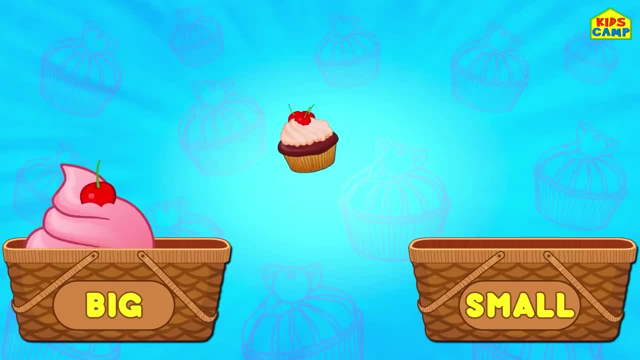 And the smaller one goes into the small basket. Wow, Ooh, More cupcakes. Let's compare these: The pink cupcake is bigger, The yellow cupcake is smaller, The yellow cupcake goes into the small basket And the big one goes into the big basket. 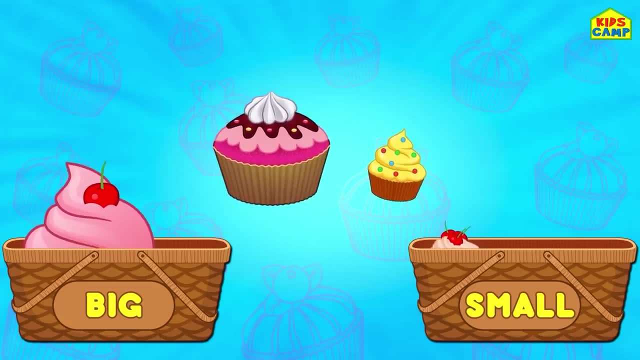 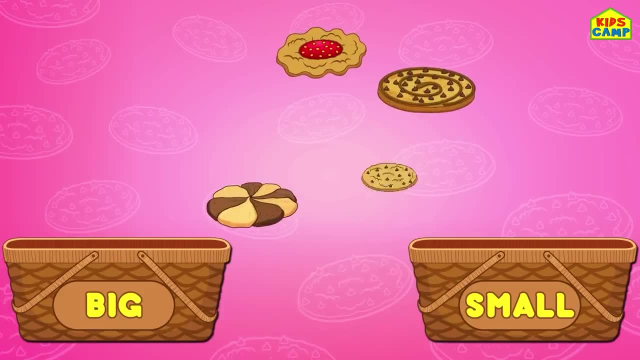 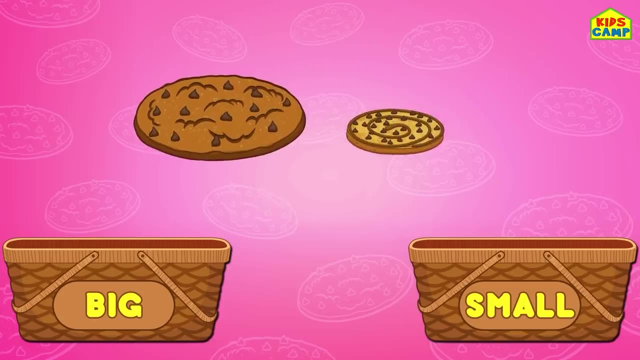 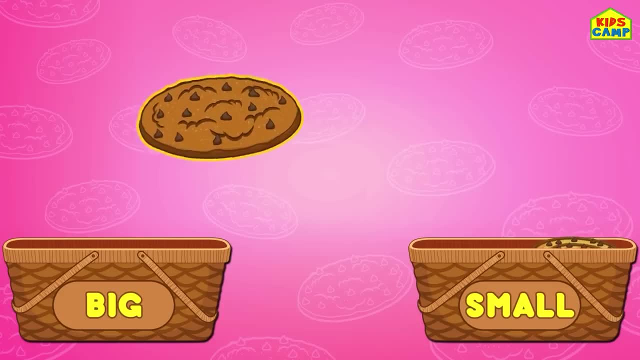 And the bigger cookie goes into the big basket. That's right. Yay, Yay, Yay, Yay, Yay. This smaller cookie goes into the small basket And this big one goes into the big basket. Yay. 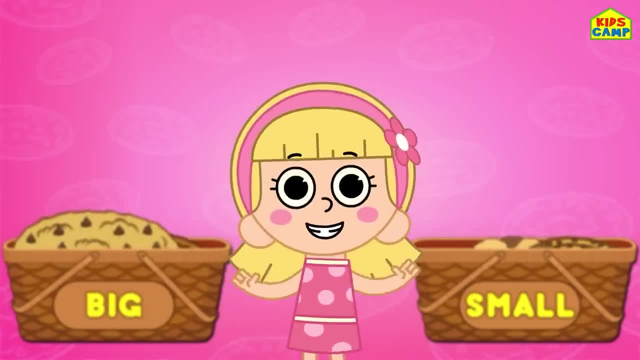 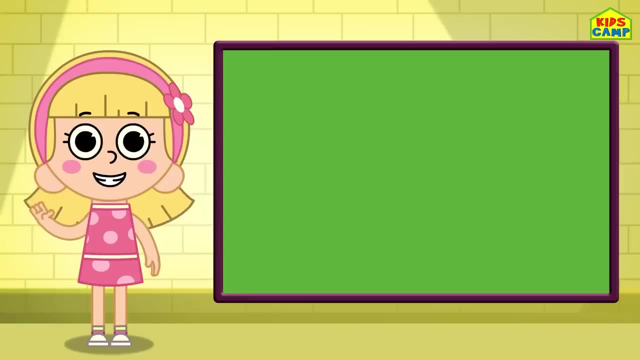 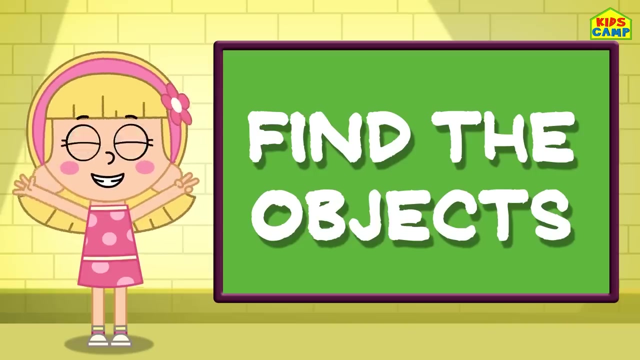 Yay, Wow. We sorted all these treats according to their sizes. Good job everyone. Hi kids, I'm Ellie and today we are going to play Find the Objects. That's right, Let's get started. Let's find the bat and the teddy Ready. 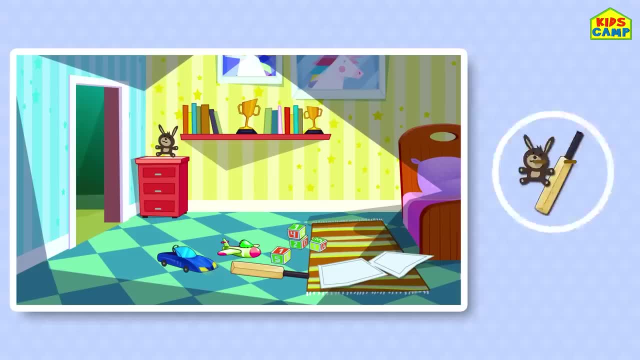 Here we go. Can you find the bat and the teddy? Where could it be? Can you see the bat and the teddy anywhere? Keep looking Time's up. Aha, There it is. We found the bat and the teddy. 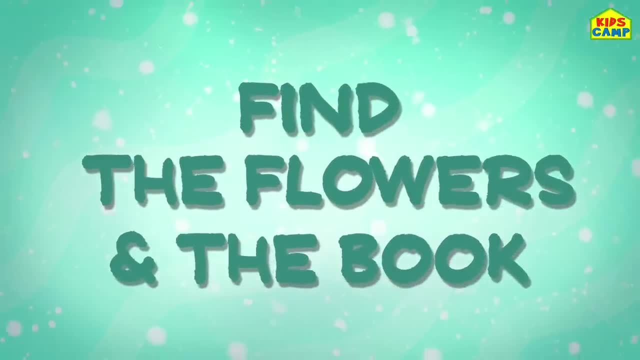 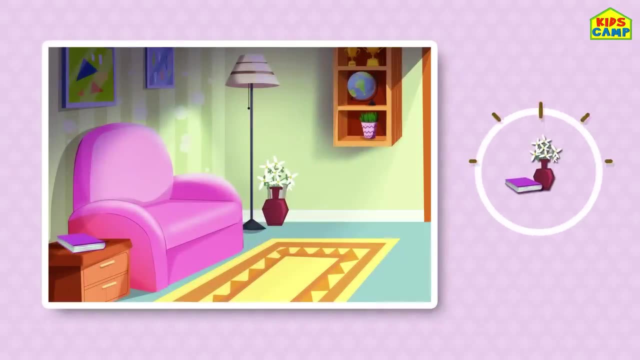 Find the flowers and the book. Let's look for it. Can you spot the flowers and the book? Where could it be? Where could it be? Not on the sofa? Where is it? Keep looking. Time's up- There it is. 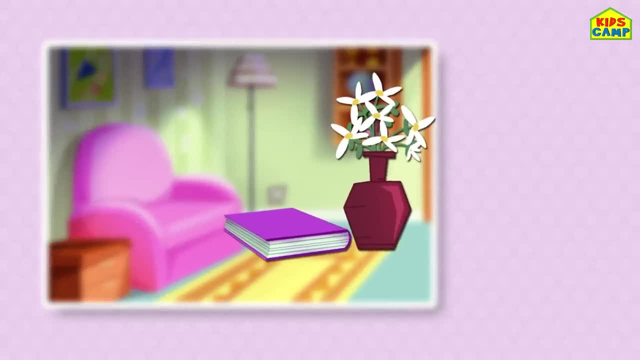 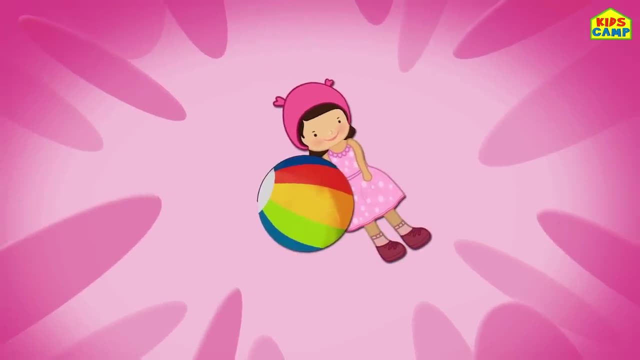 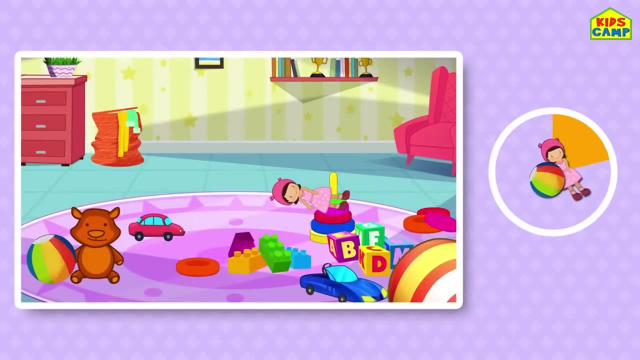 We found the flowers and the book. Find the ball and the pink doll Ready. Can you spot the doll and the ball? Where could it be? Where could it be? Hmmm, Keep looking. Our time's almost up, Time's up. Did you find it? 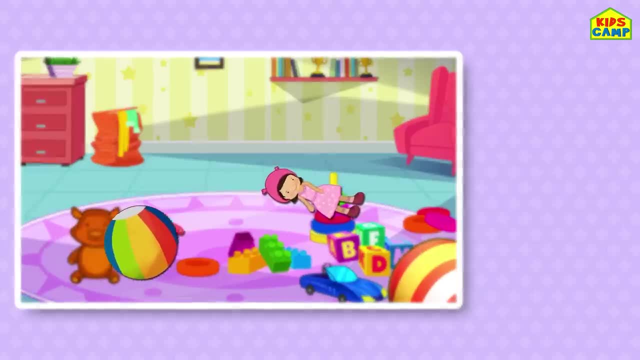 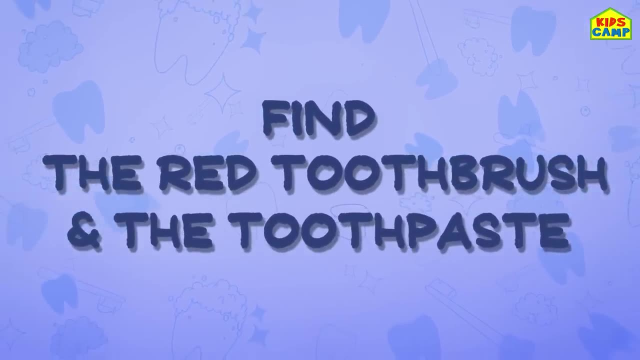 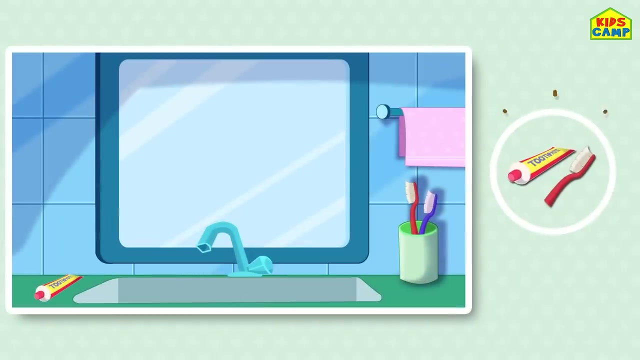 Yes, There it is. We found the ball and the pink doll. Yay, Find the red toothbrush and the toothpaste. Ready kids Look for it. Can you spot the red toothbrush and the toothpaste? This one is easy. Keep looking. Time's up. 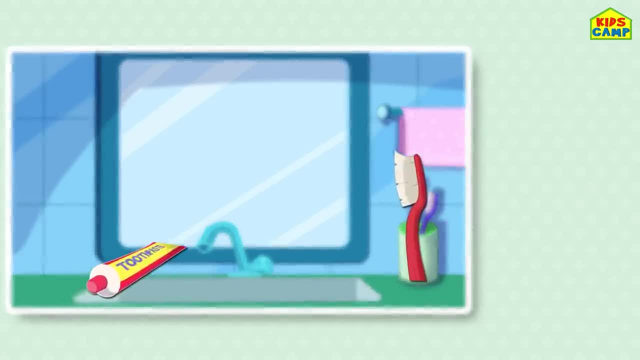 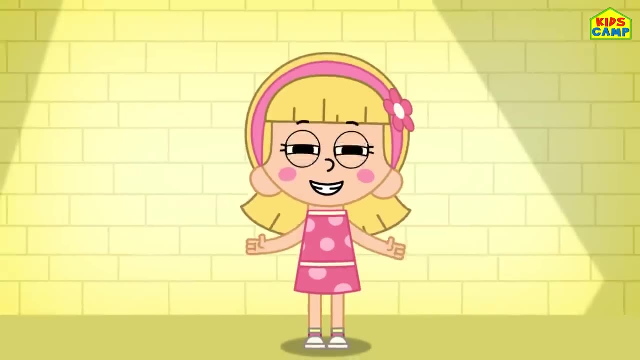 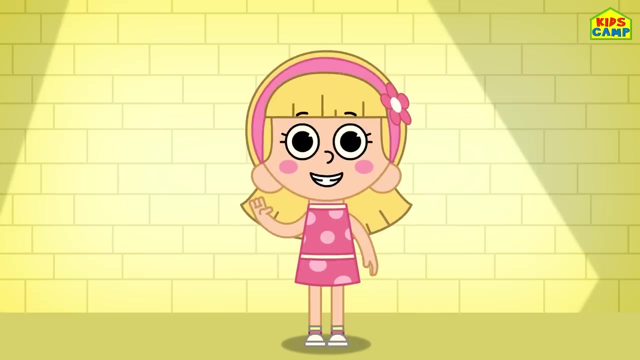 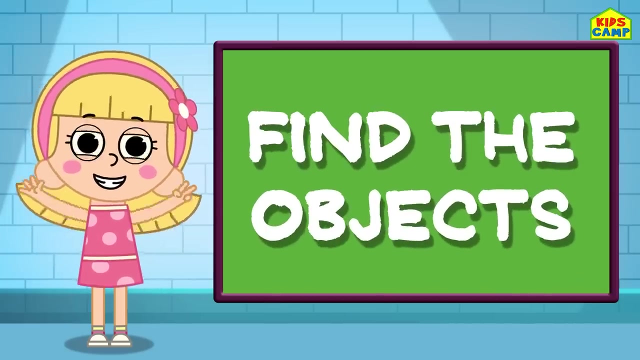 Woohoo, You did find it There. it is The red toothbrush and the toothpaste. This was so much fun, kids. We found all the objects. See you soon. Hi, kids, I'm Ellie And today we are going to play Find the Objects. 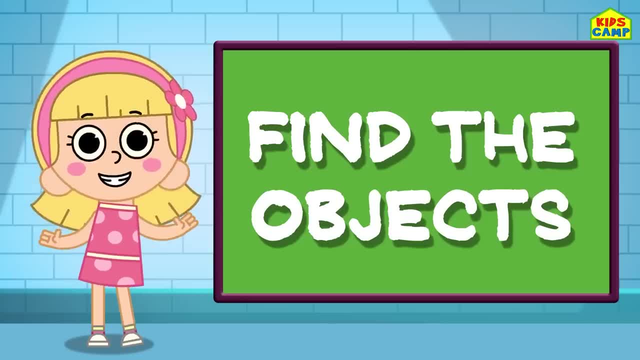 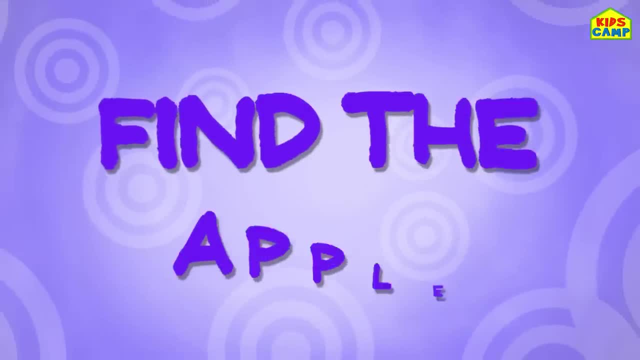 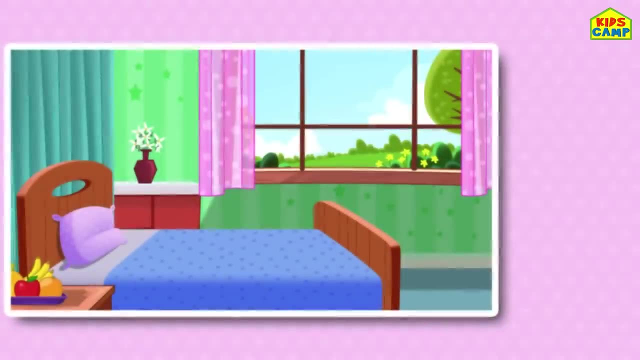 Yay, Ready, Let's get started. Find the apple. Hmm, that's easy. Let's look for the apple. Where's the apple? Is it on the bed? No, Where is it? Keep looking Time's up. Did you spot the apple? 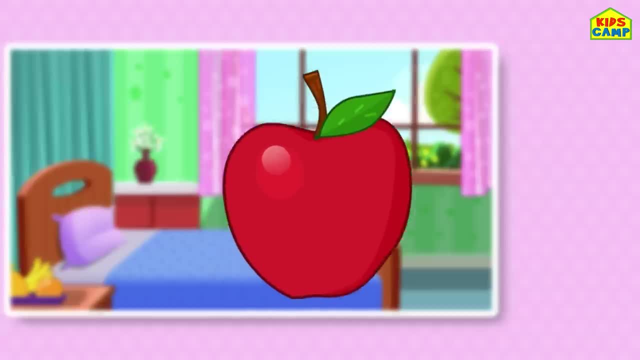 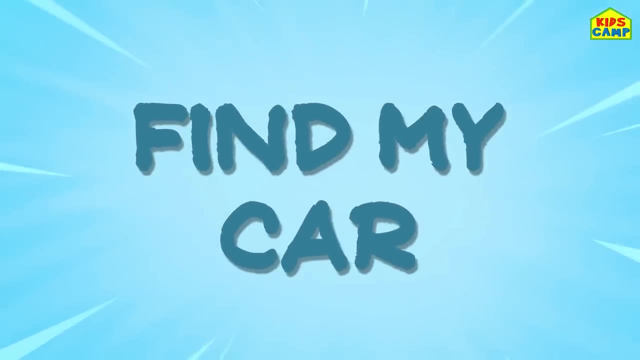 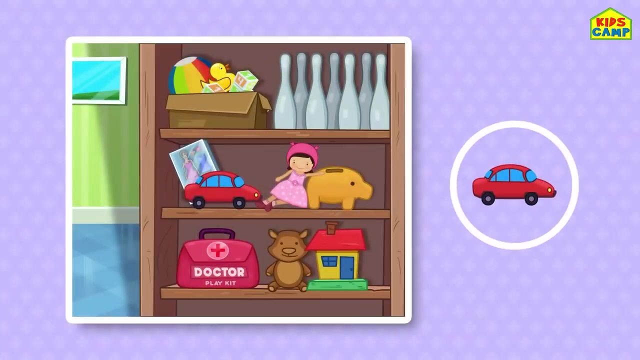 Yes, There, it is. Good job, kids. We found it. Find my car. We have to look for my red car. Can you spot it? Hmm, where is it? There's so many toys on the shelf. Uh-oh, Time's up. 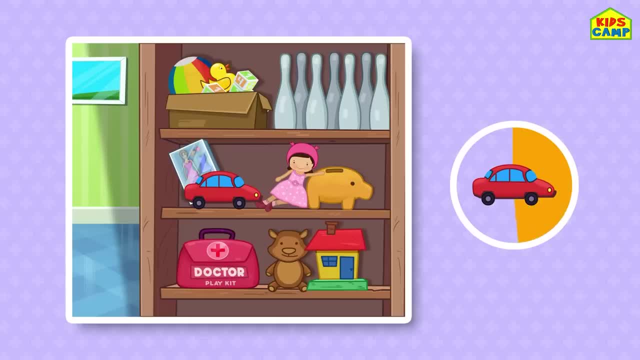 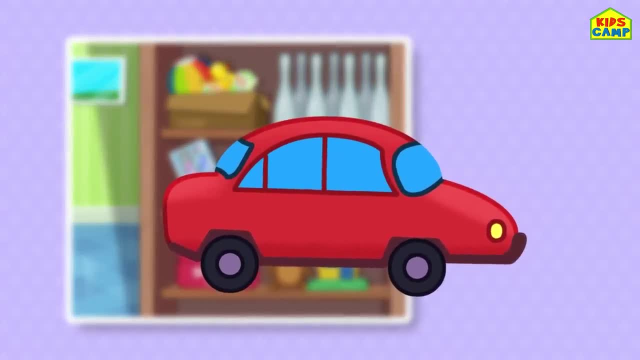 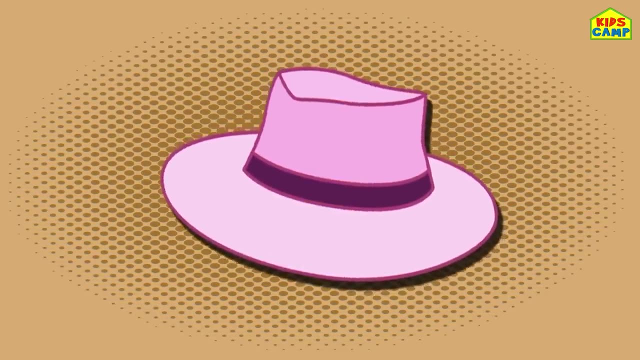 That's where it is. That's my red car. Vroom, vroom. Find my hat, My pink colored hat, My pink colored hat. Can you look for my hat? Can you look for my hat? Oh my, There are so many hats. 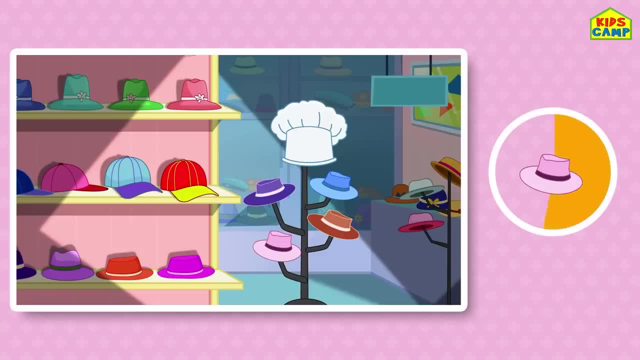 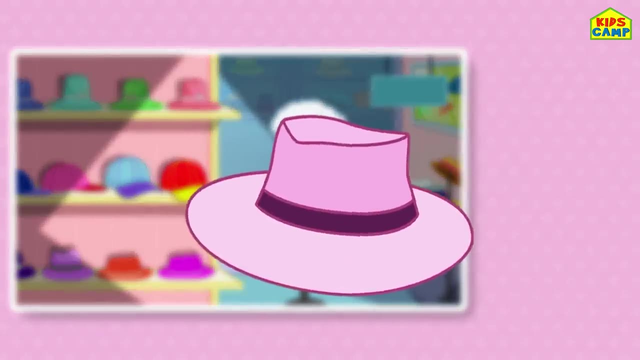 Can you spot the right one? Can you spot the right one? Come on, Come on. Time's up, Time's up. Yes, That's the one, Yes, That's the one. Good job, kids, You found it. 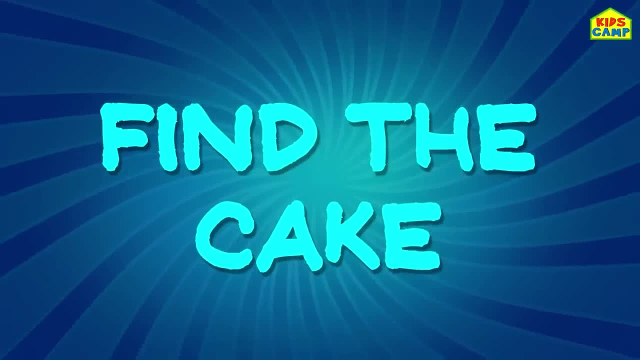 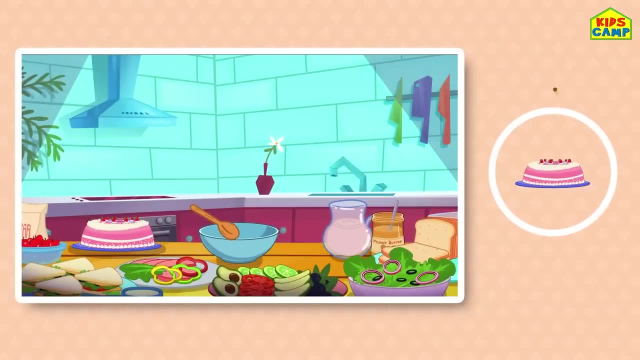 Woohoo, Find the cake. Find the cake. Delicious, Let's look for the cake. Let's look for the cake. Wow, There is so much food on the table. Wow, There is so much food on the table. Can you look for the cake? 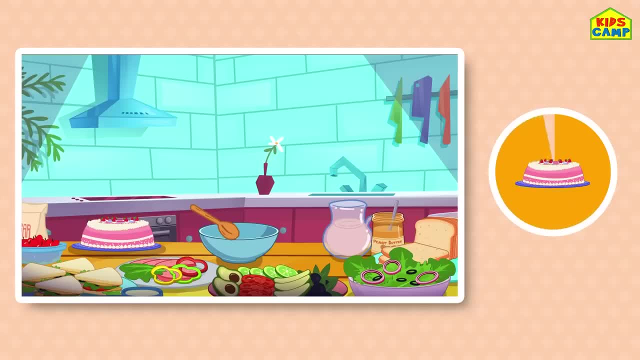 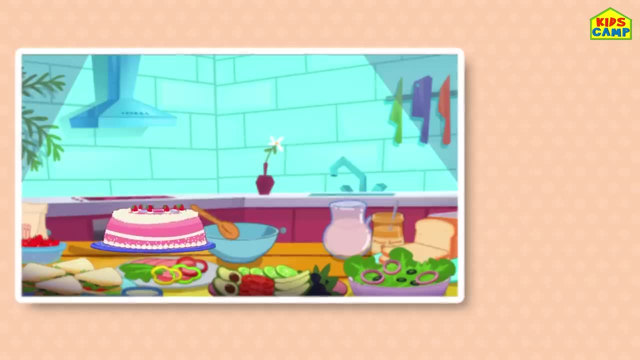 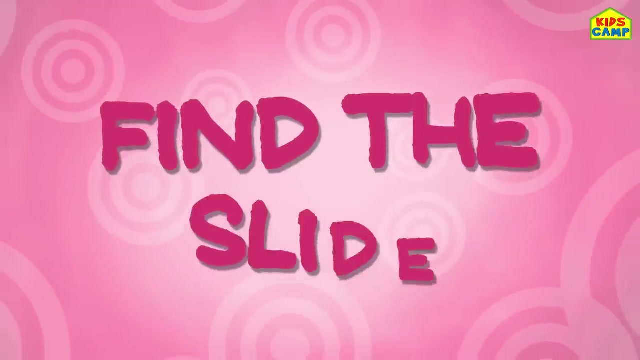 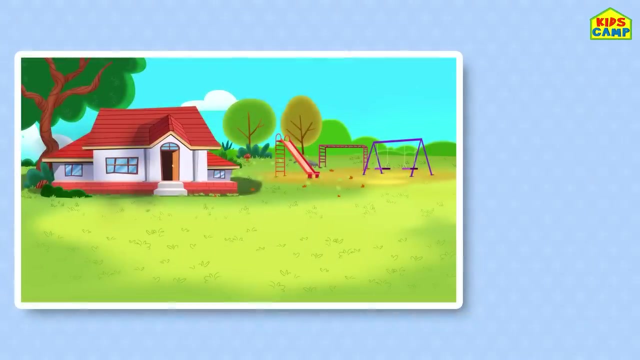 Where's the cake? Time's up, Time's up, That's right. There it is. You found the cake Looks delicious. Find the slide. Wow, I love the slides. Where's the slide? Can you spot it? Can you spot it? 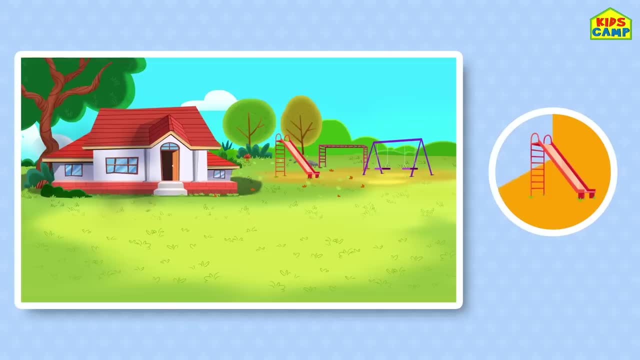 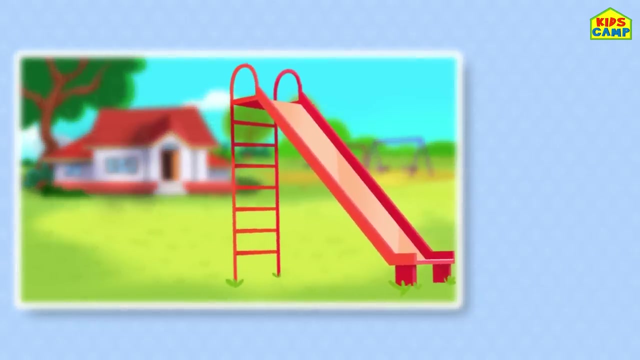 Keep looking. Time's almost up. Time's almost up, Uh-oh, Time's up. Uh-oh, Time's up. Yes, That's right, We found the slide. Woohoo, Good job, We had so much fun. 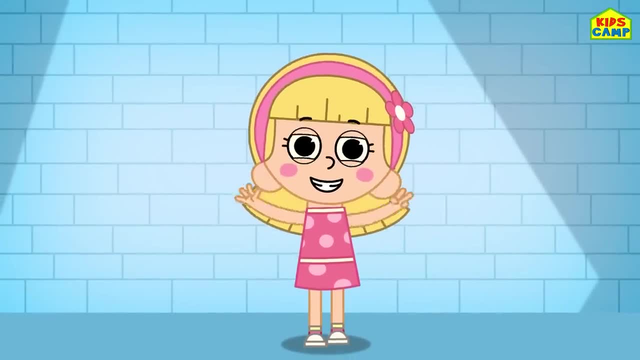 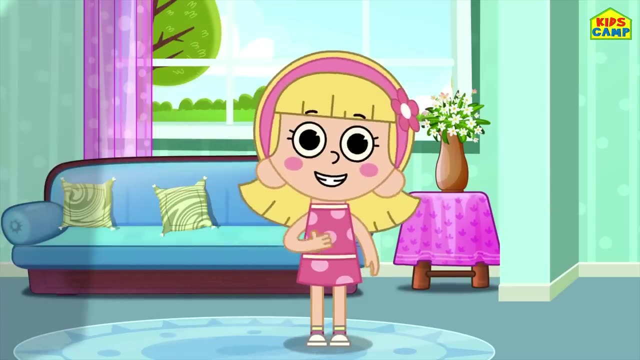 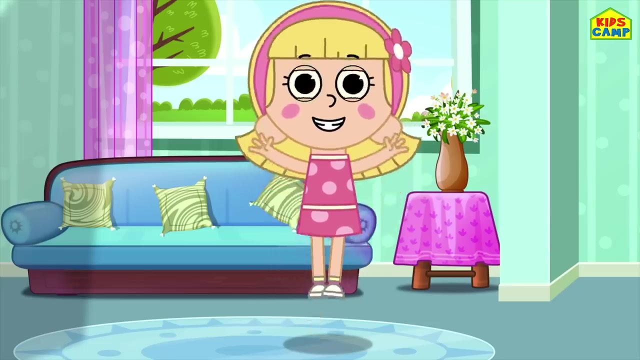 finding the objects. See you soon. Bye-bye, Hi kids. I'm Ellie And today we are going to play with puzzles. Don't we all love puzzles? That's right, Let's start. Ooh, That's a car. 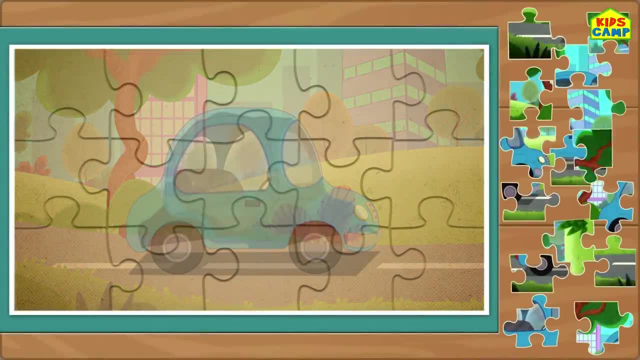 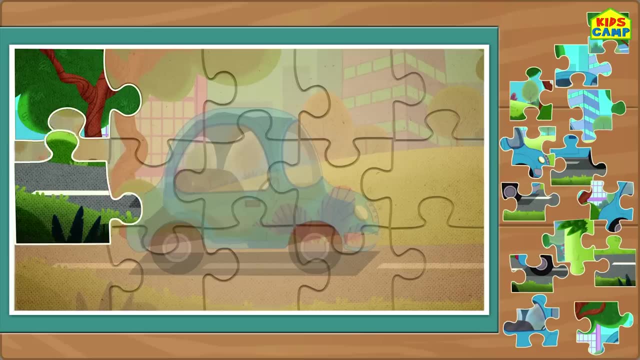 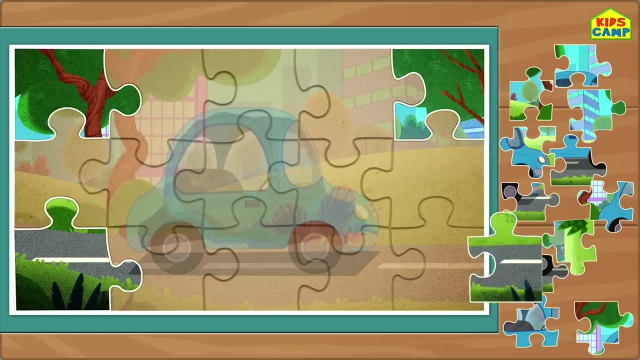 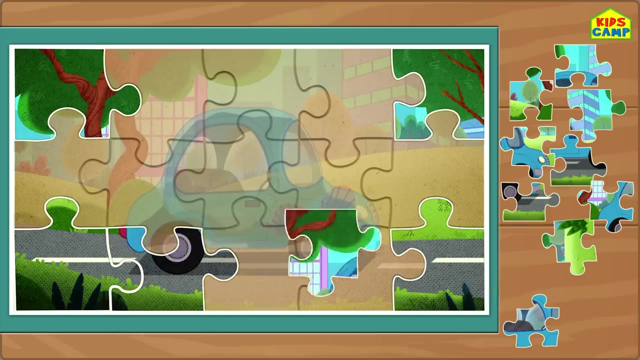 Let's put all the pieces together. Let's start with the corners. Let's start with the corners. That's right. It goes right there. That's right. Perfect, We got all the four corners. No, That goes up there. 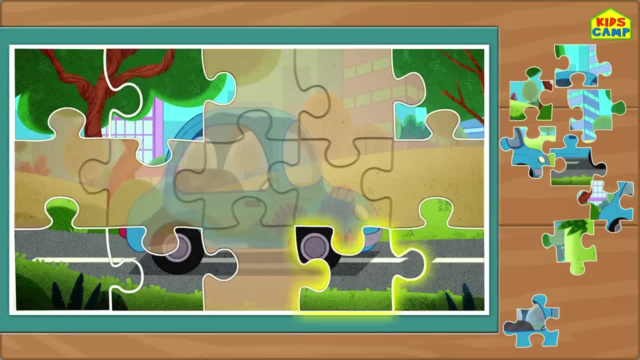 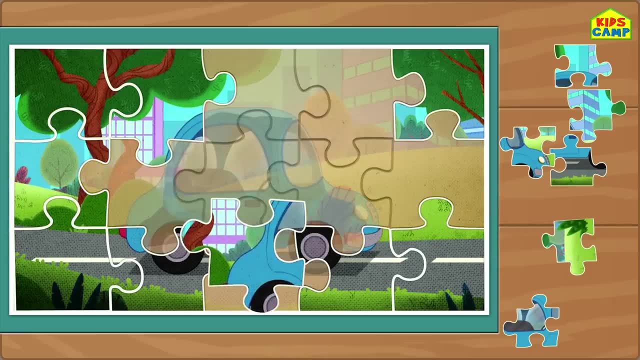 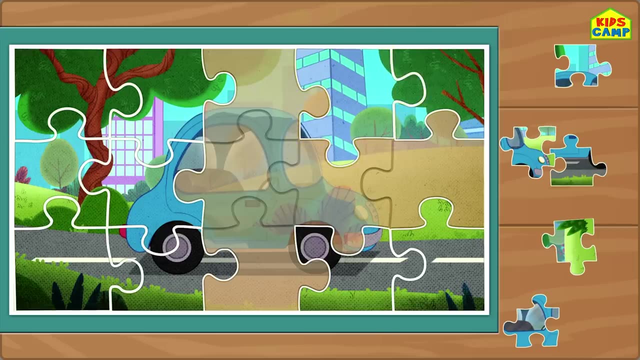 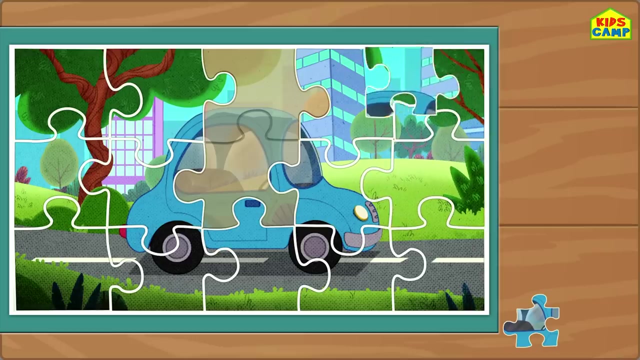 That's right. Another wheel, Perfect, Great, Uh-oh, That's right. Wow, Wow, So much fun. I like puzzles, Don't you? No, No, That doesn't seem right Now. it is Perfect. 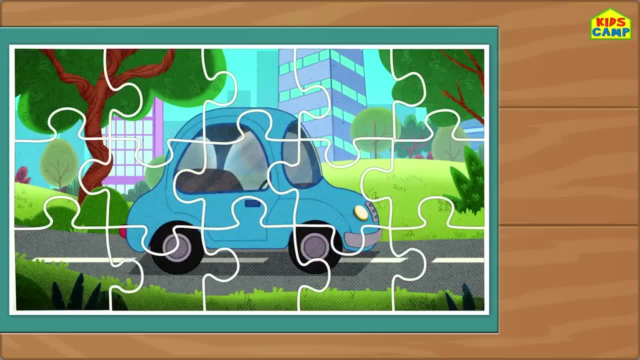 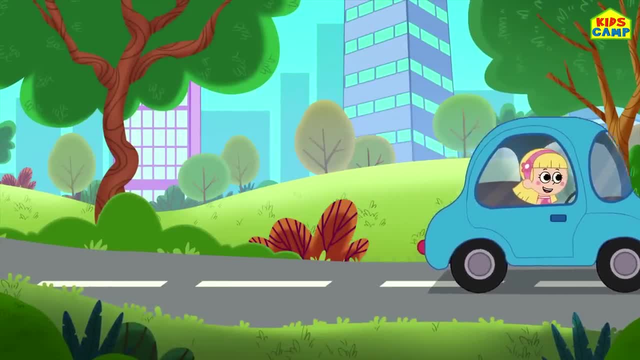 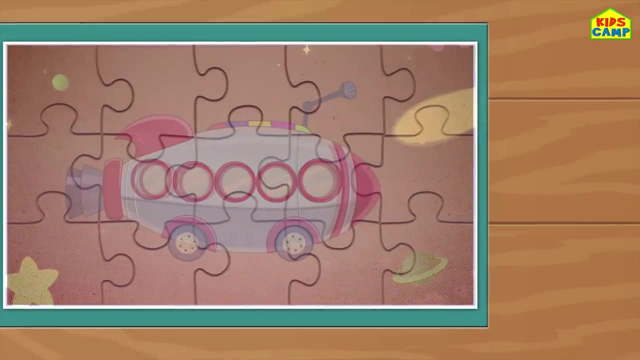 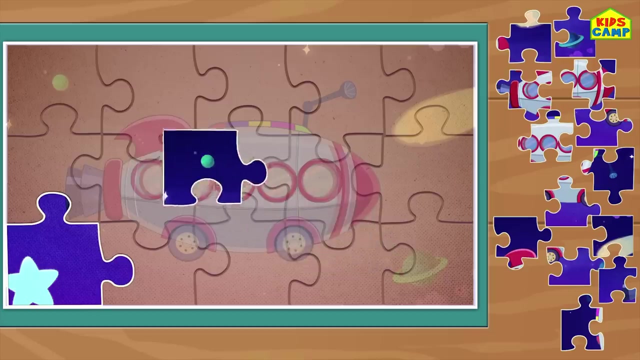 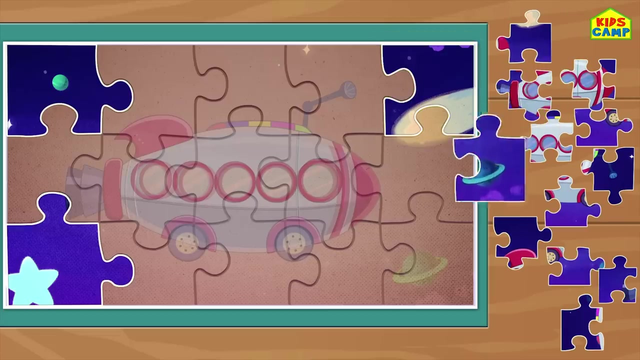 And the last piece: Woohoo, We did it. kids, There goes my car Vroom, Vroom And A spaceship. Let's start with the corners. That's right. Yay, We got all the four corners. 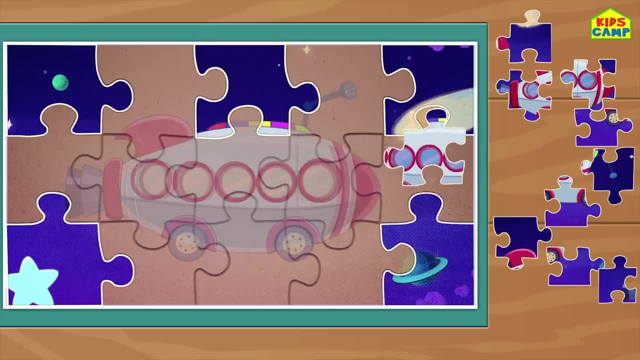 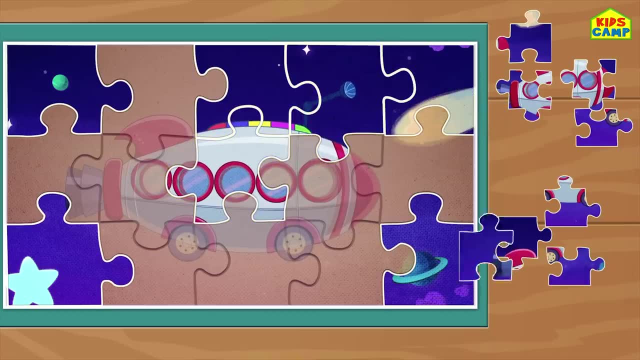 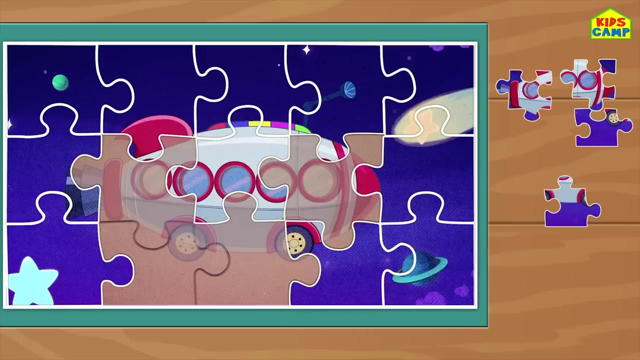 Uh-oh, Yes, Wow, The windows Perfect. Woohoo, Woohoo, Woohoo, That's right, That's right, We're almost done. We're almost done. Just a few more to go. Just a few more to go. 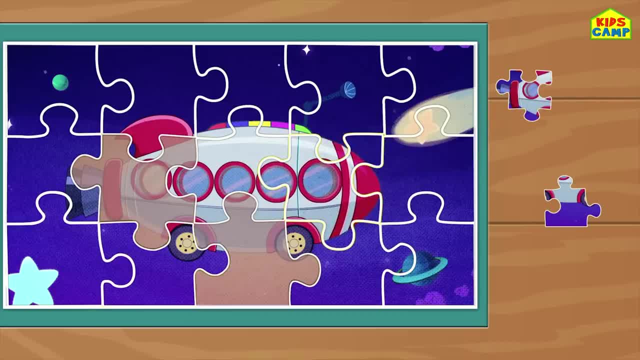 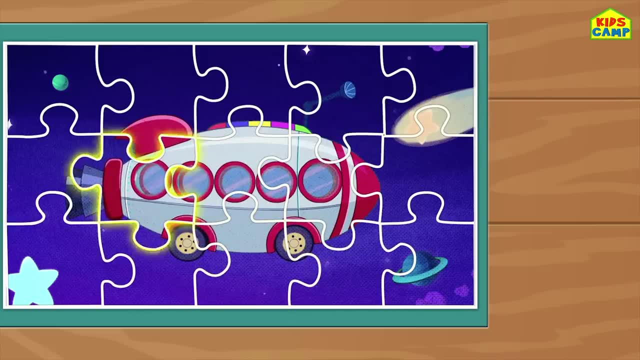 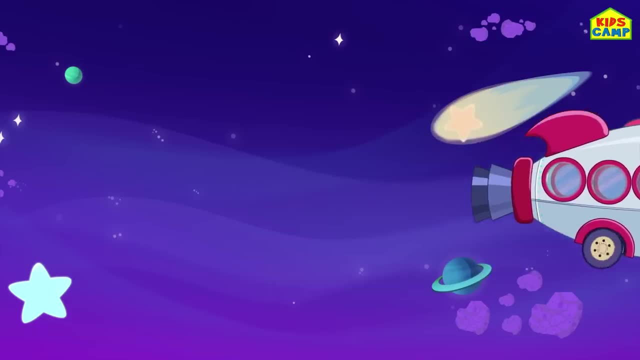 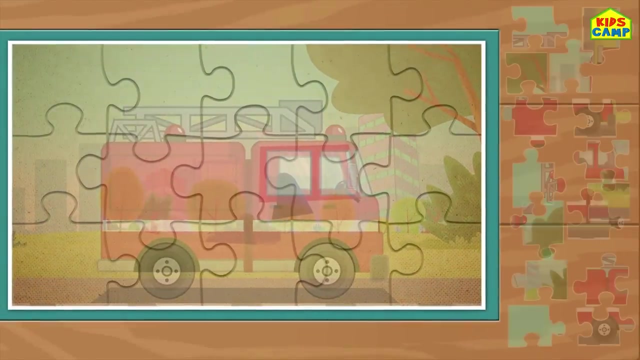 Perfect. A few more pieces. Wow, This looks so good. And the last piece: Our spaceship is completed. Our spaceship is completed And here I go: Woohoo, A fire truck, A fire truck. Once again, let's start with the four corners. 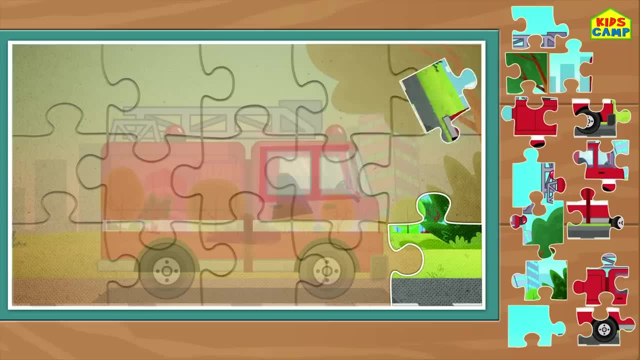 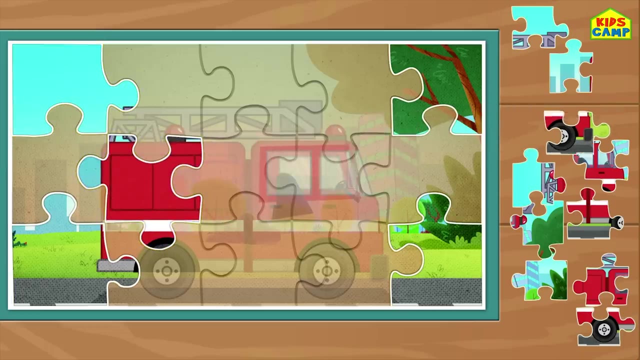 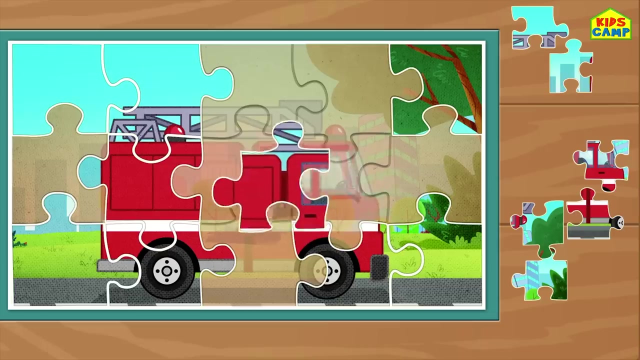 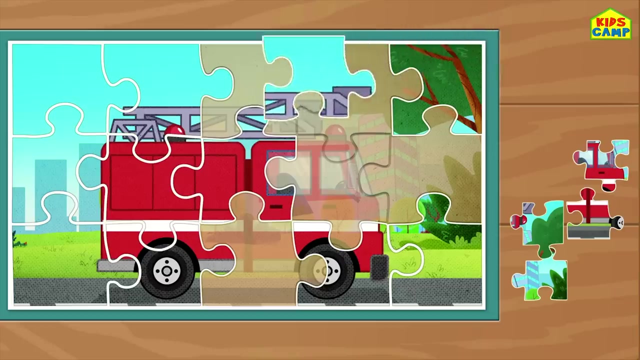 Let's start with the four corners. Let's start with the four corners. What a complete λ? Damn girl. Wow, you're so good, It look perfect. Wow, we almost got it. A few more pieces, That fits correctly. 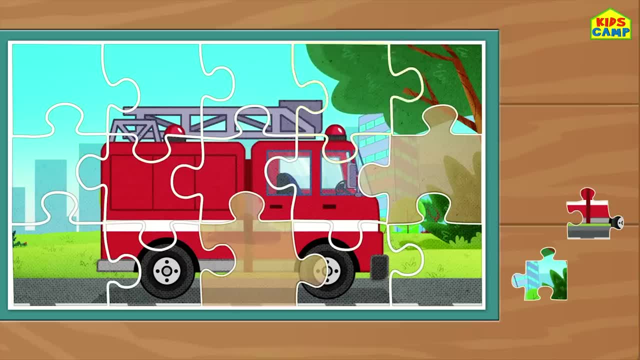 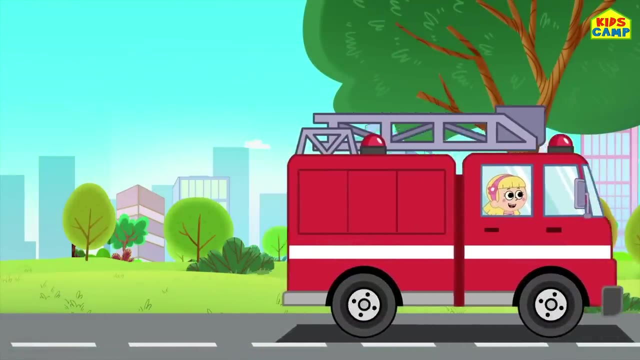 Oh, we gotta spin that around. Perfect, And the last piece. We did it. Our firetruck is ready to go. Wow, Yay, This was so much fun solving puzzles. See you soon. Hi, I'm Ely. 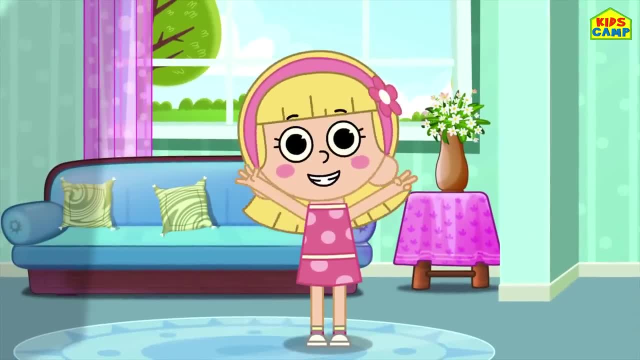 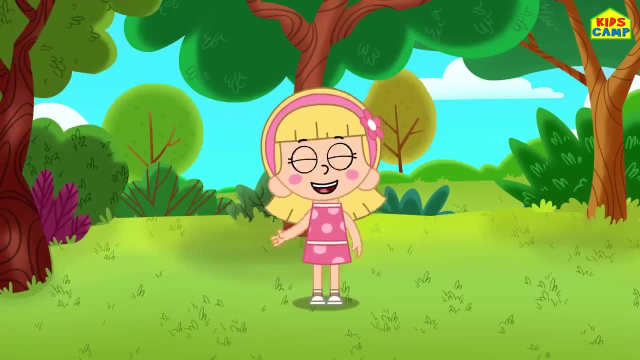 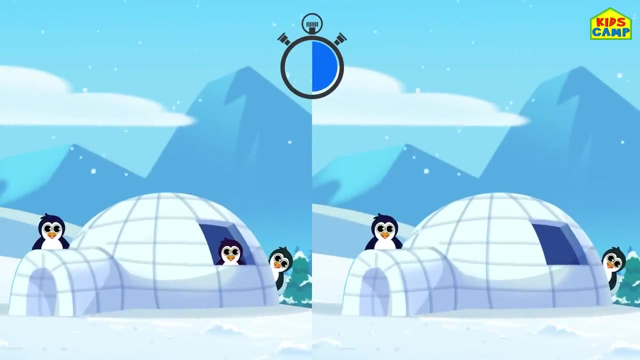 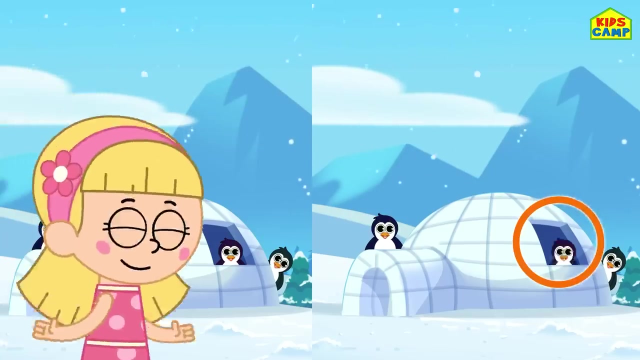 And we are going to play a fun game. We have to spot the differences And this is going to be such a fun game. Ready, Let's start. Can you spot the difference? Time's up, That's right. Next one: 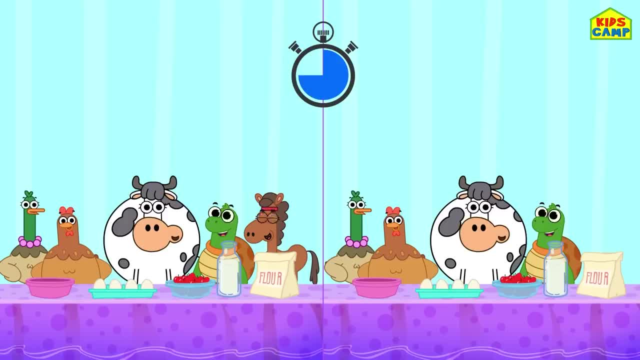 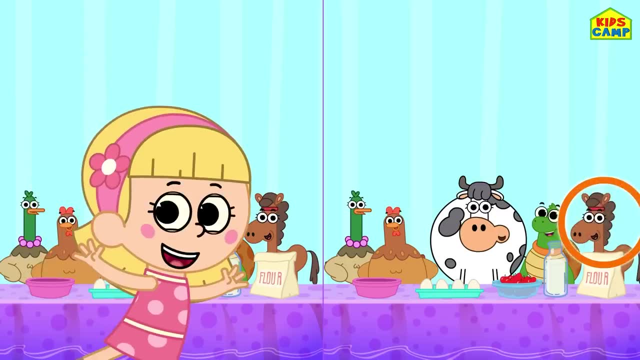 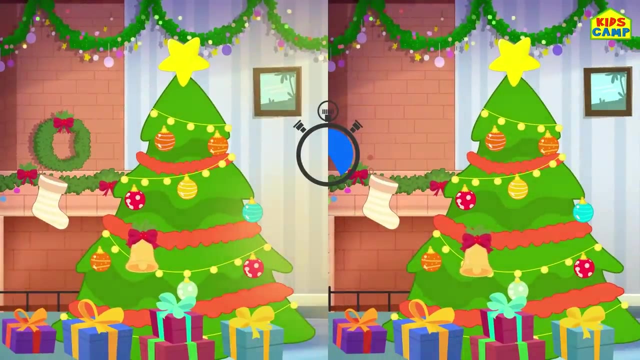 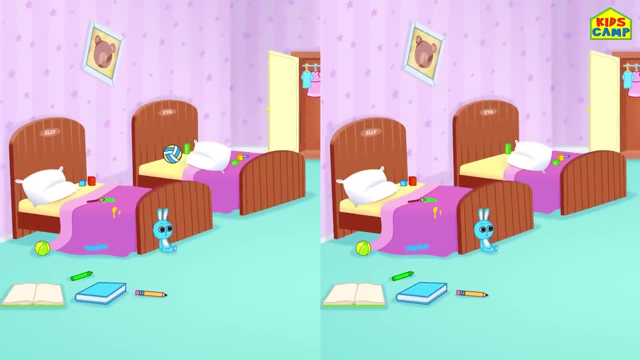 Can you spot the difference? Time's up, That's right. Can you spot the difference? Keep looking Time's up, That's right. Next one: Can you spot the difference? Keep trying Time's up, That's right. 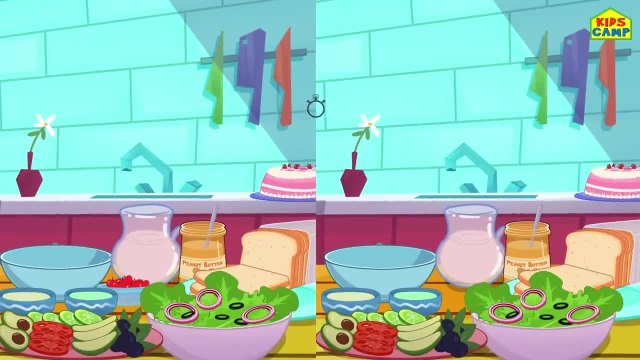 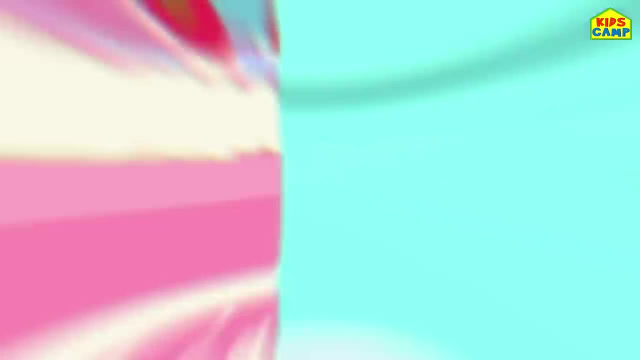 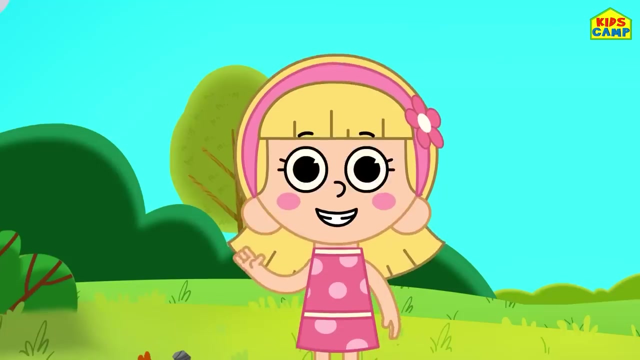 Next one. Can you spot the difference? Keep trying Time's up. Woohoo, You guys did it. Yay, This was so much fun. Bye-bye, Bye-bye. Hi friends, I'm Ellie and I've learned some new words. 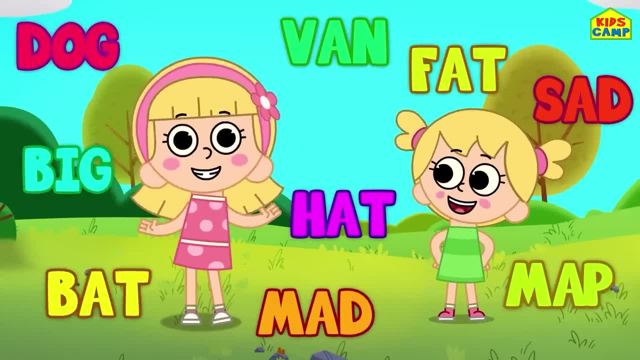 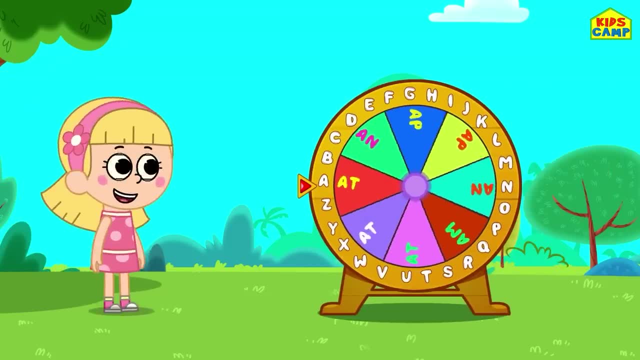 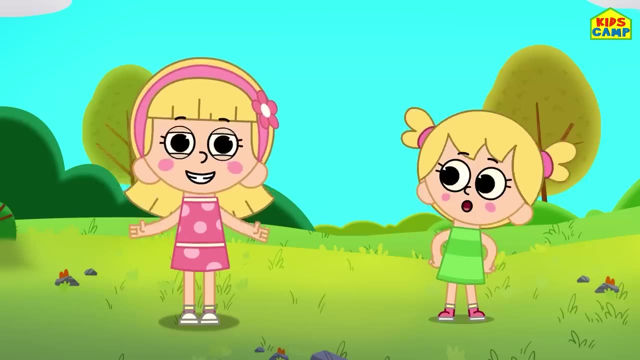 That's right. Do you also want to learn with me? Yes, Let's get started. This is the word wheel. We have to spin the wheel and match the letter to make the correct word, And we also have clues. This is going to be so much fun. 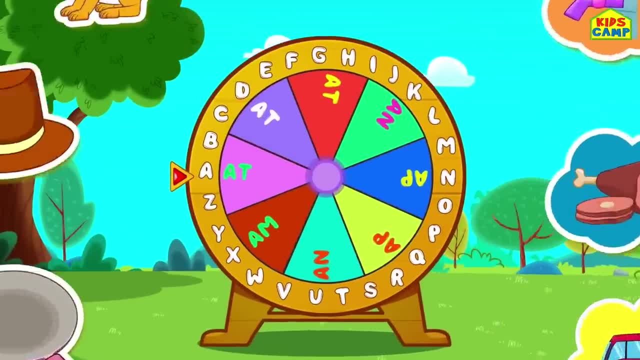 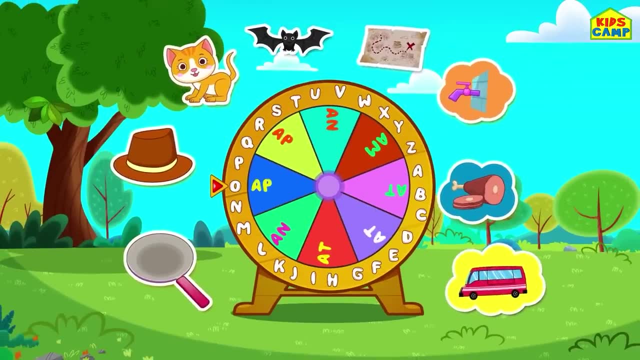 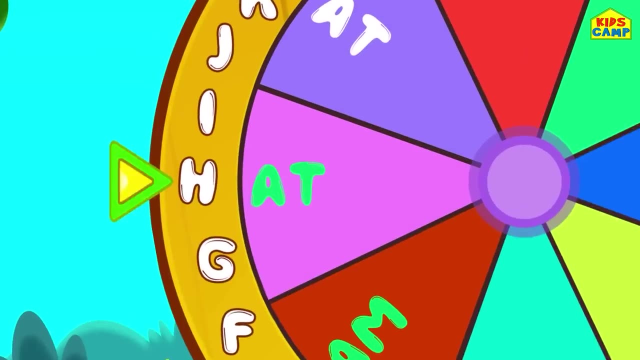 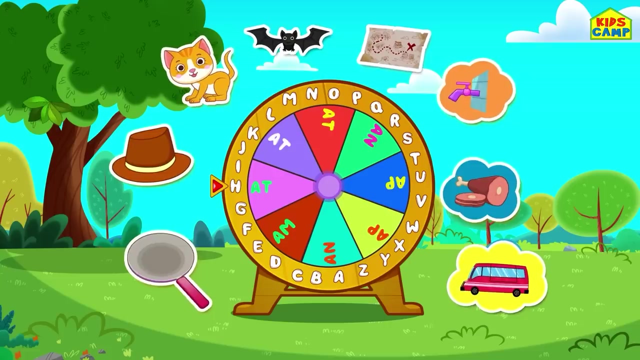 Let's get started. Let's spin the wheel. Woo-hoo, Is that a word? No, Let's keep spinning. Is that a word? H-A-T hat, That's right, That's how you spell a hat. We found the first word. 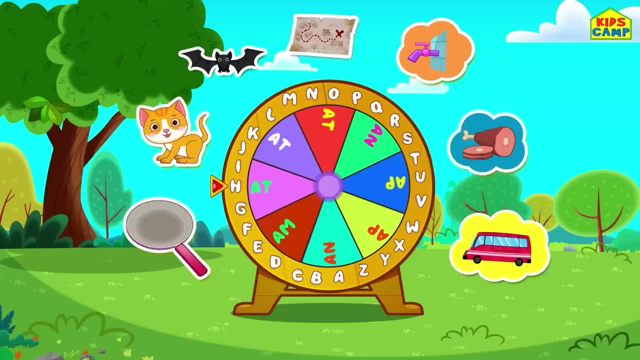 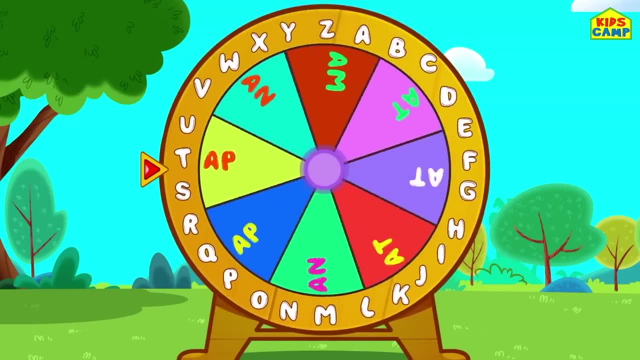 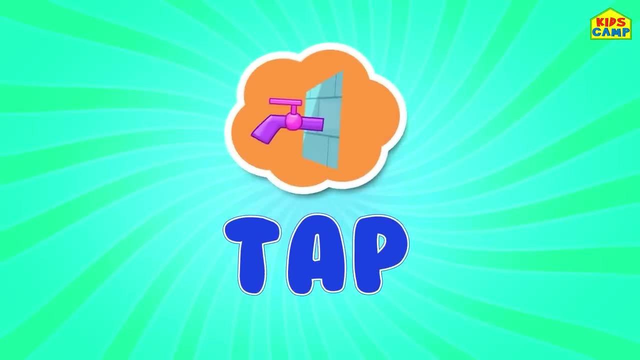 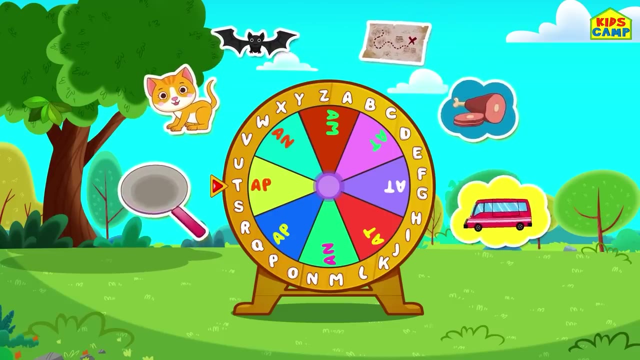 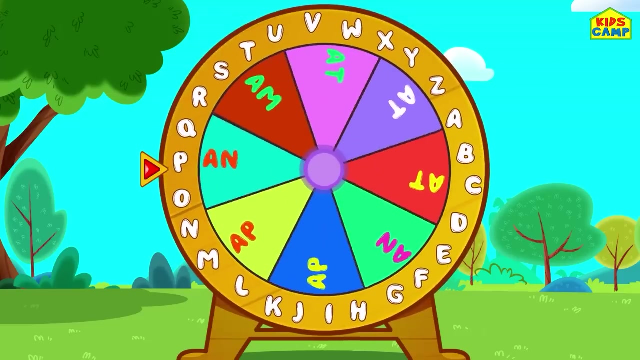 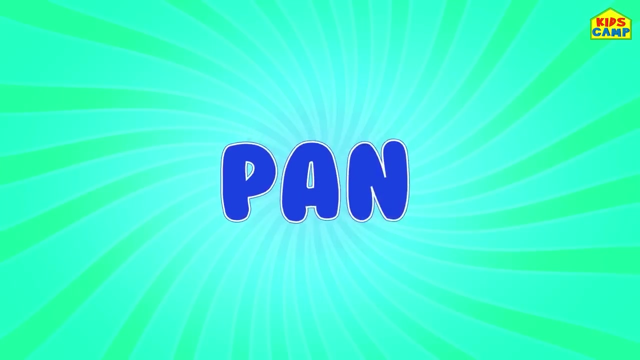 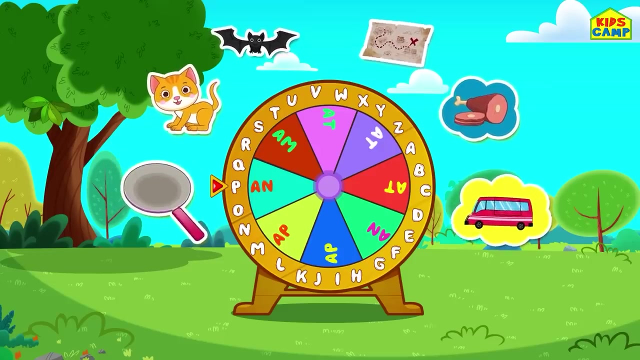 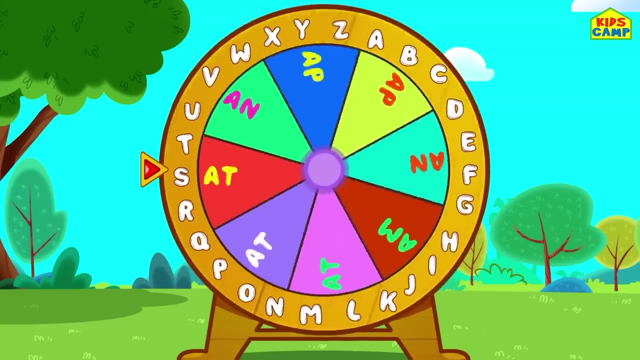 That's right, That's a word. A tap, Wonderful, We found one more. Let's look for some more. Keep spinning Woo-hoo, Is that a word? P-A-N Pan- Yes, that's a word. Wow, We found another one. What's next? Let's keep spinning. Yay, Is that a word? 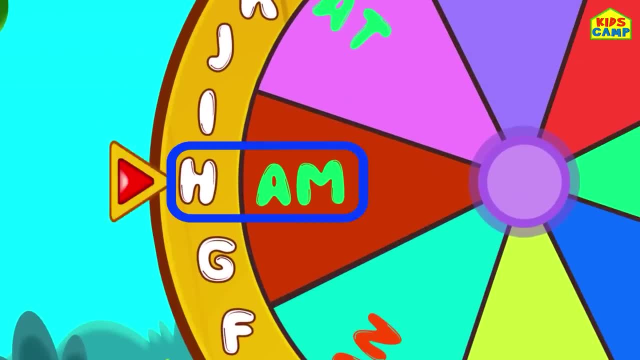 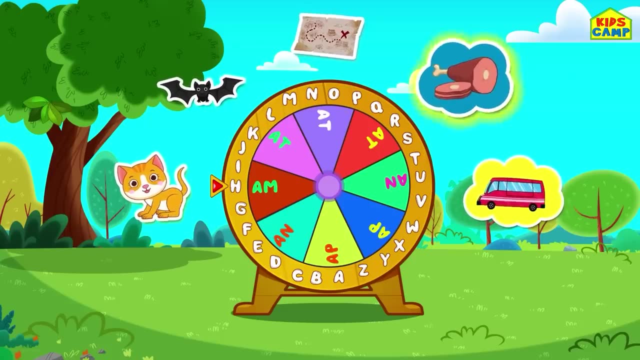 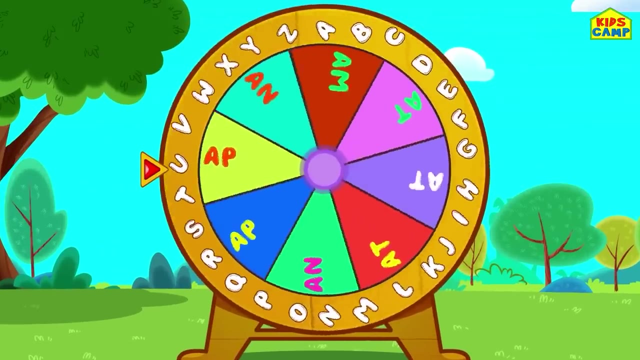 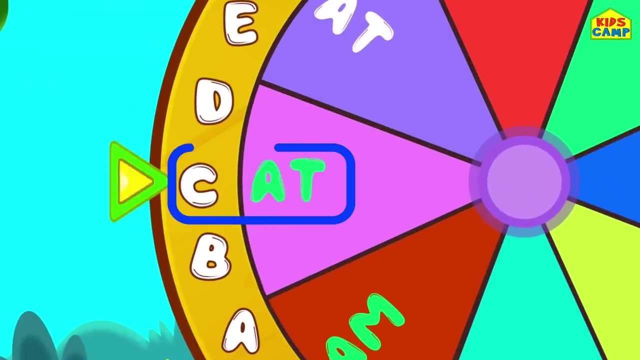 H-A-M. Ham, That's right, that's a word. Yummy, We found another one. Let's find some more friends. Let's spin the wheel. C-A-T. That's a word. Cat Woohoo. 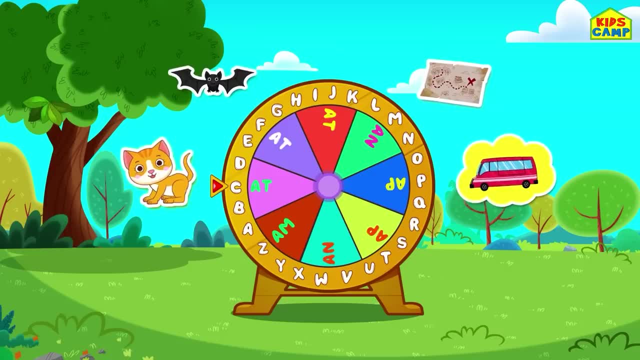 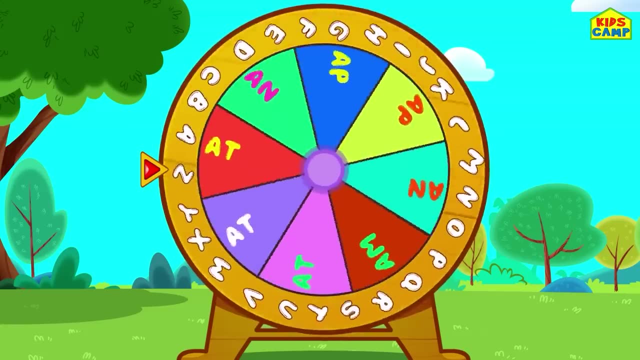 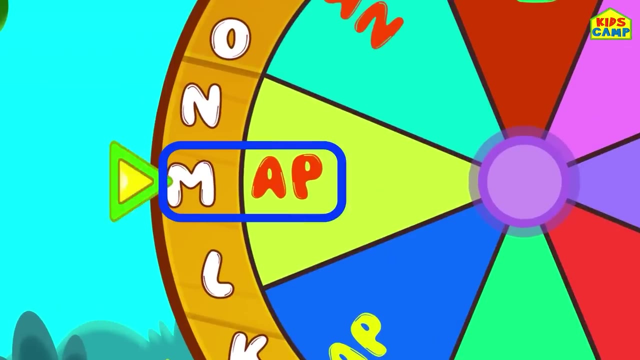 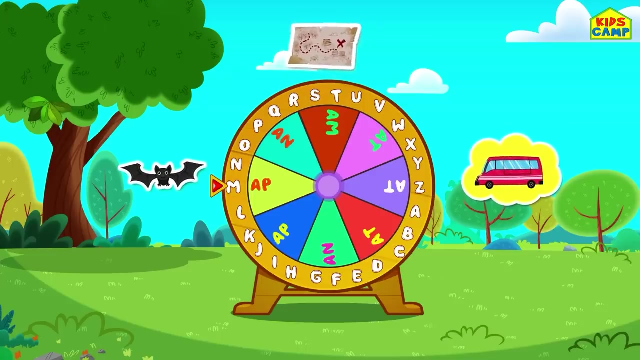 What's next? Let's spin the wheel again. Word wheel Keep spinning. Uh-huh. We found another word: M-A-P, Map. That's right. Map is a word. We found the word map. Good job, friends. 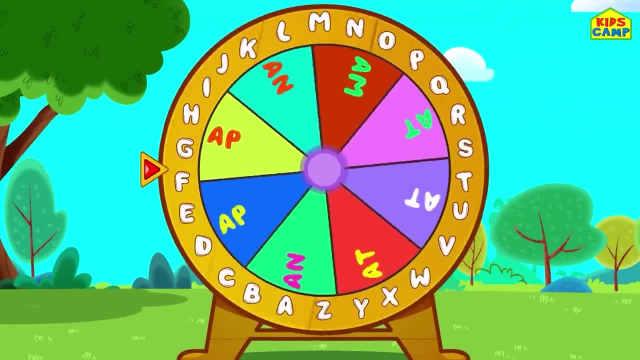 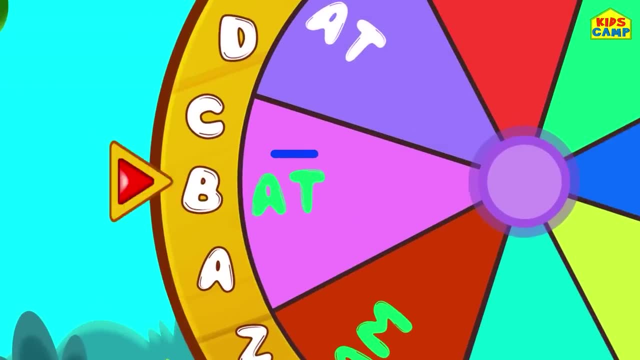 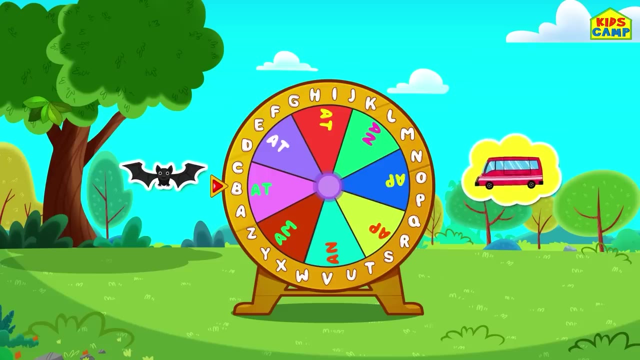 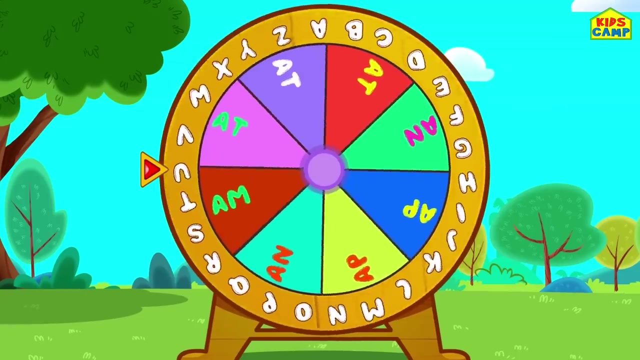 Let's keep spinning the wheel. What's next? What's next? That's a bat, B-A-T bat. That's right. We found another word: A bat. Good job, What's the last word? Let's keep spinning the wheel. 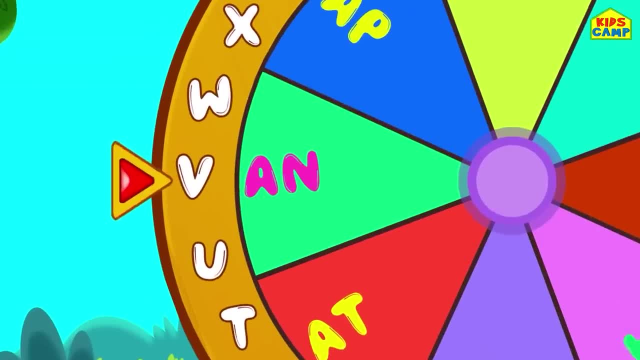 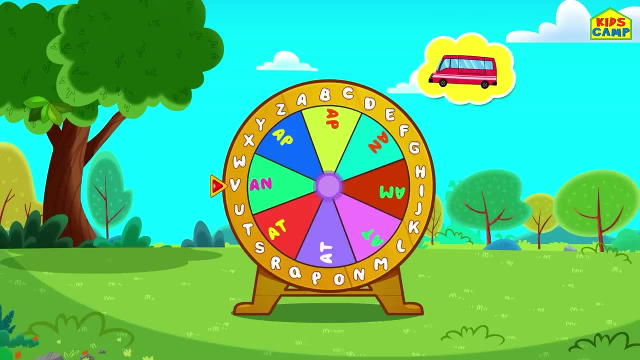 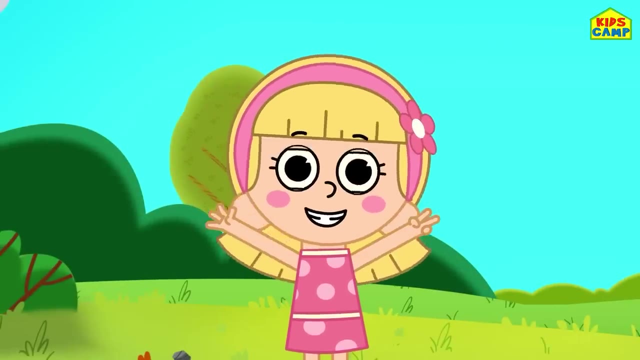 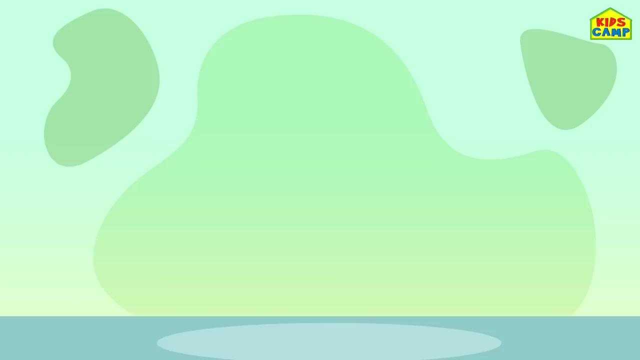 It is a van C-A-T. What's next? That's right, We got all the words. We had lots of fun today. Yay, We learned some new words today. Bye, Hi kids. I'm Ellie And I'm going to put up some pictures in Eva's bedroom. 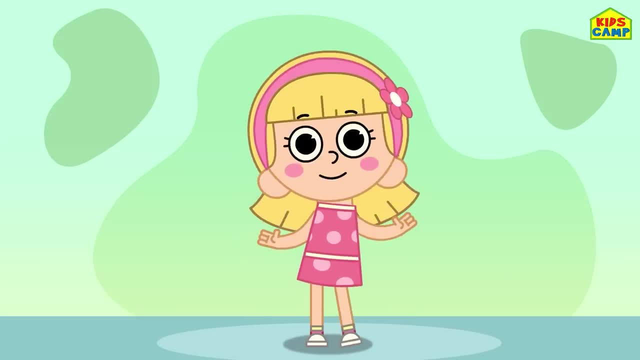 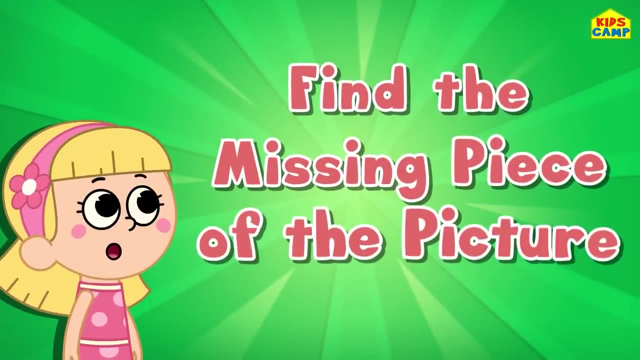 But there's just one tiny problem. There seems to be a missing piece in each picture. Can you help me find it? Woohoo, Let's get started. This is going to be a fun game. Let's find the missing piece. 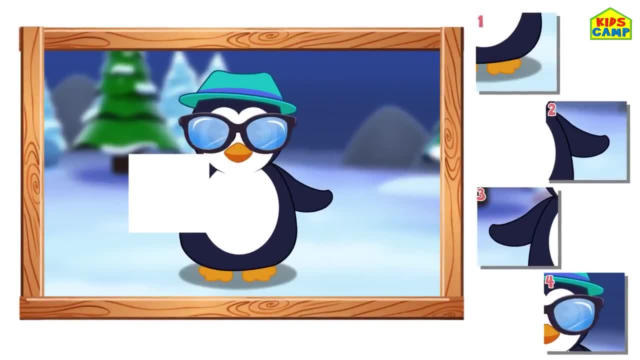 Hmm, Do you know which one is the right piece? Let's try. Let's try. Is number 2 the right piece? No, it isn't. Is number 1 the right piece? Uh-oh, It isn't. Is number 4 the right piece? 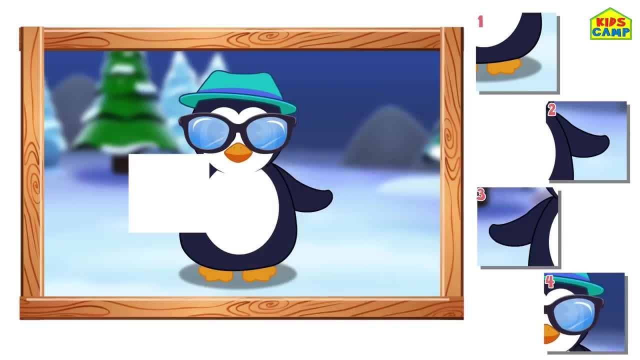 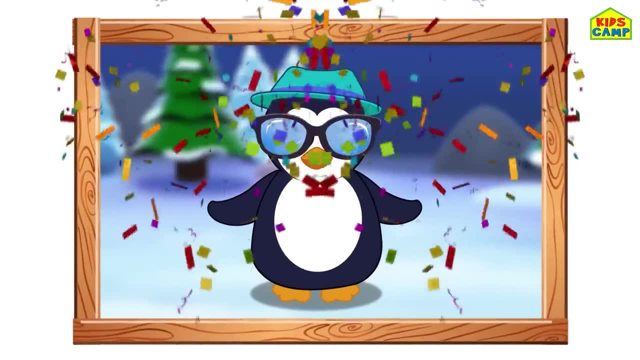 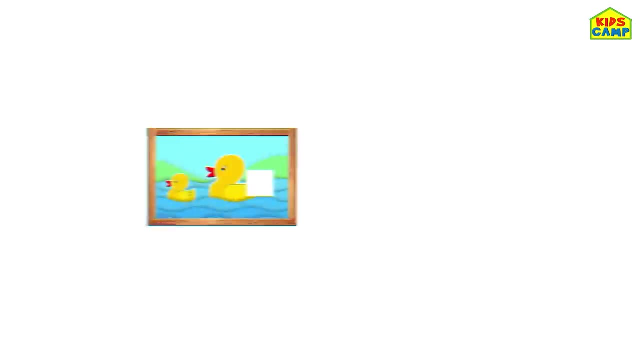 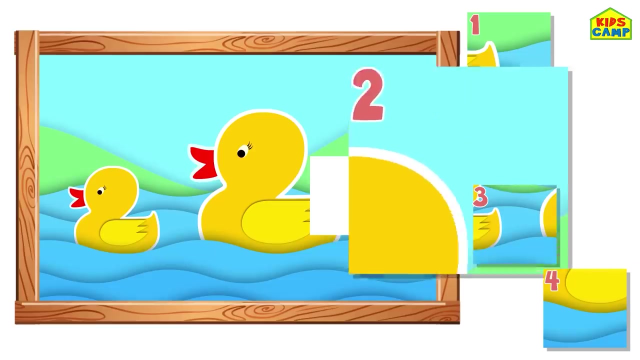 No, Hmm, Let's try number 3!. Yes, We got the right one. Woohoo, Good job, kids. Let's move to the next one. What is missing from here? Let's try number 2!. No, Let's try number 4!. 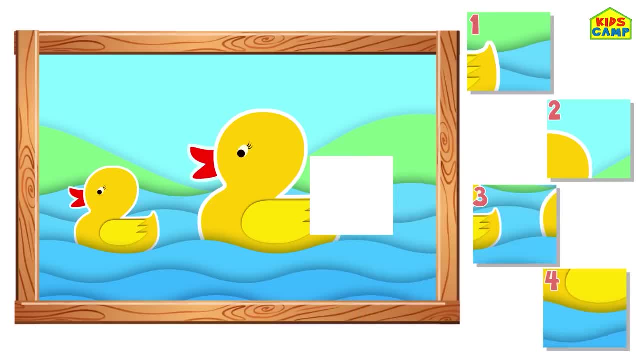 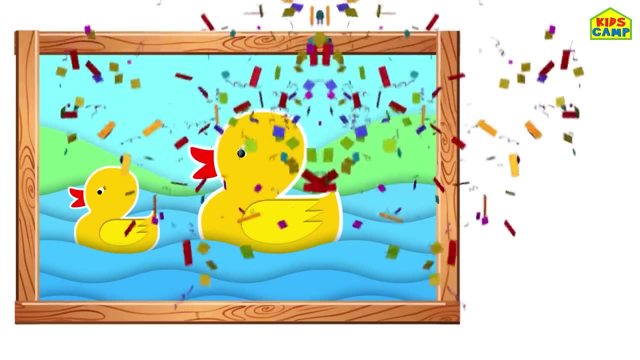 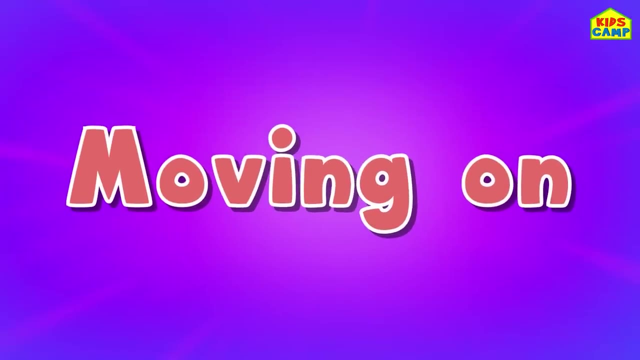 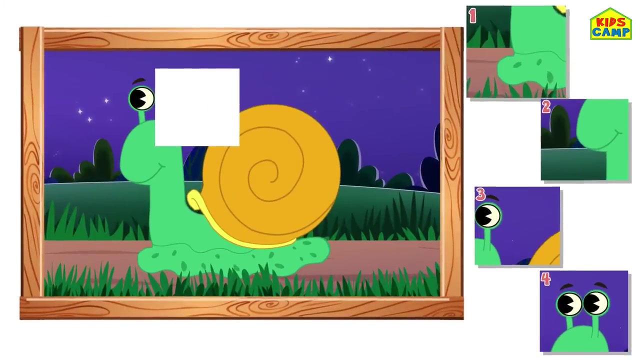 No, no, Let's try number 1!. Yay, That fits right, We got it. Woohoo Moving on. Hmm, What's missing here? Let's find out. Let's try number 2! No, That doesn't fit right. 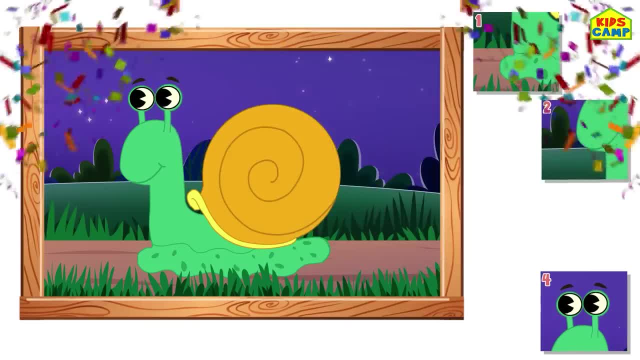 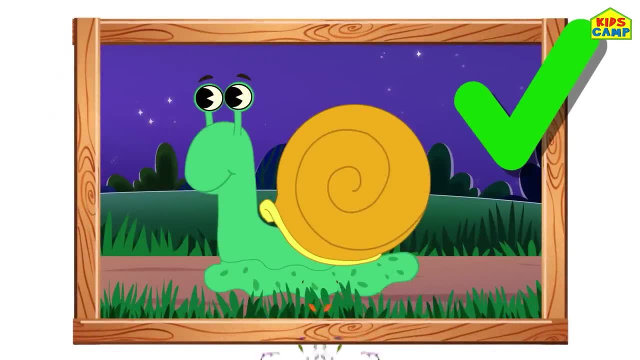 Let's try number 3!. Wow, We did it. We got that one right, Ready to go up on the wall Moving on. Hmm, What's missing here? Let's try number 1! No, That doesn't seem right. 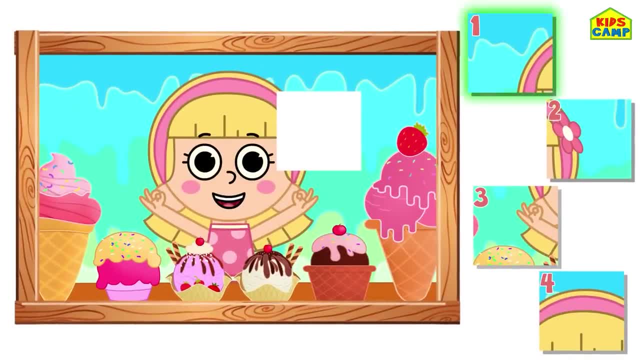 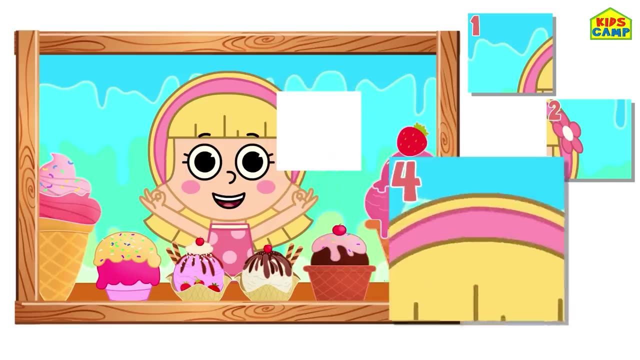 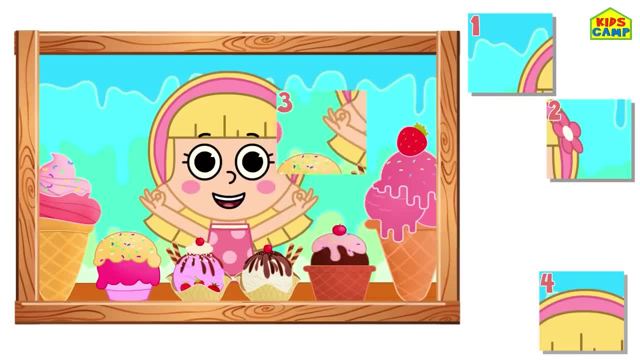 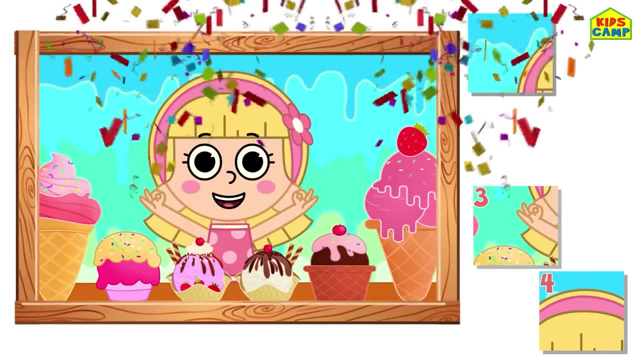 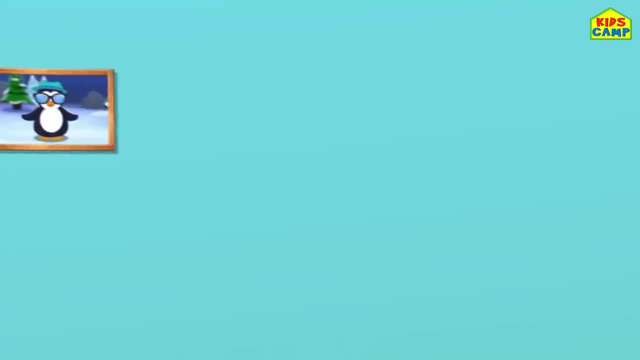 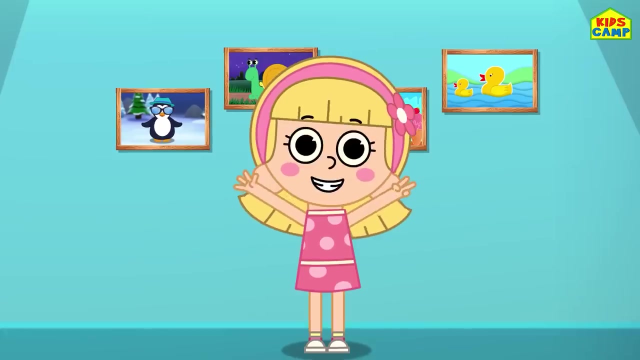 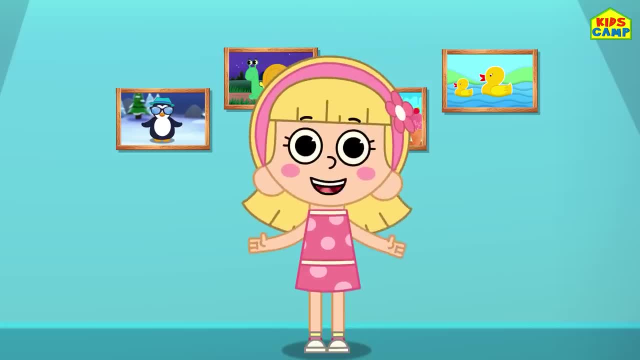 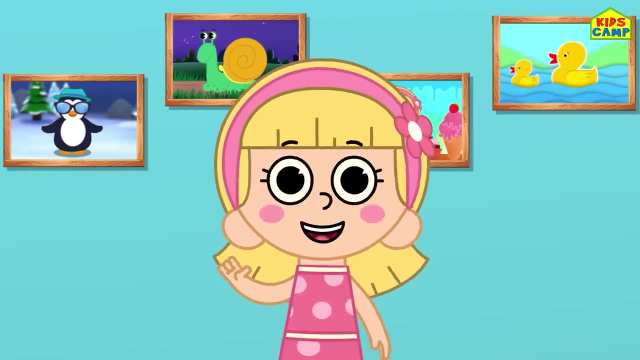 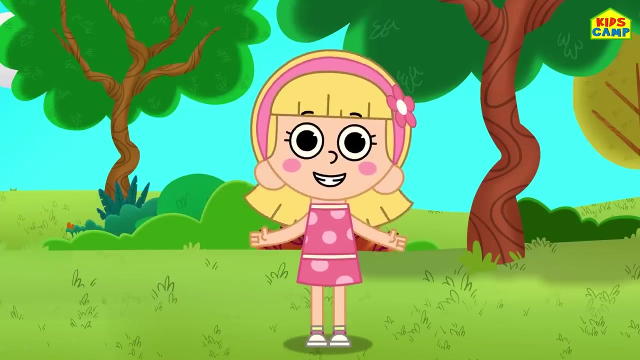 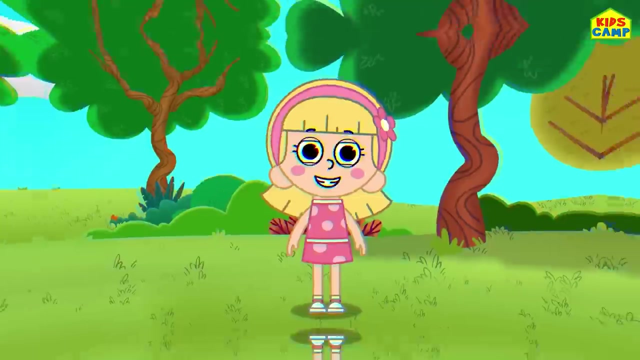 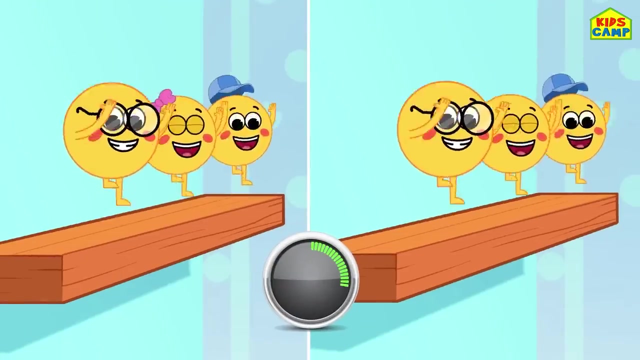 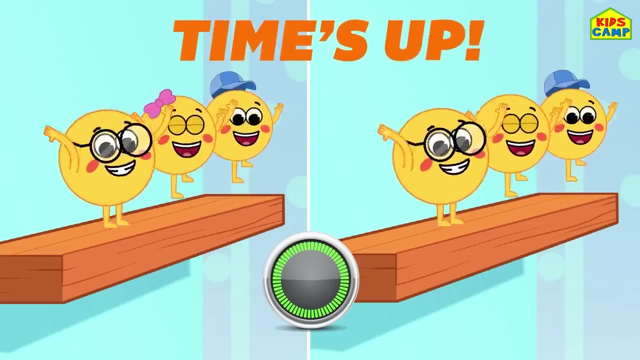 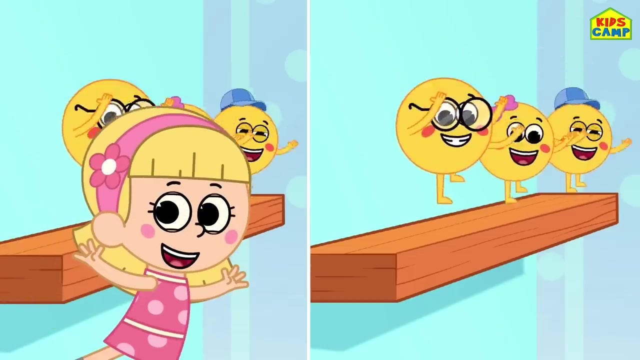 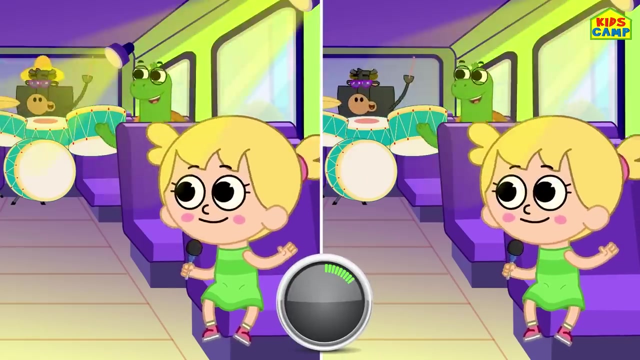 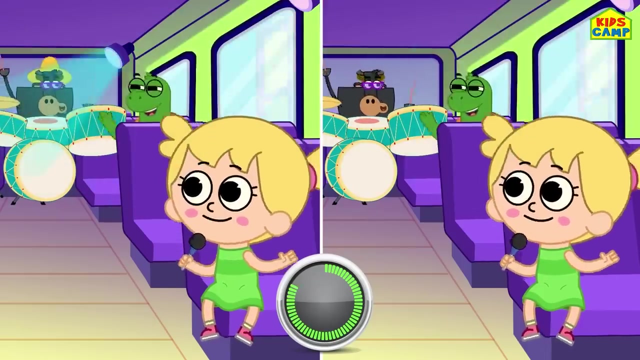 No, No, No, No, No, No. Eiffel pot. We've solved the pop time And will start the real test tomorrow. Bye, bye, Bye, Let's go to the next one. Can you spot the differences? 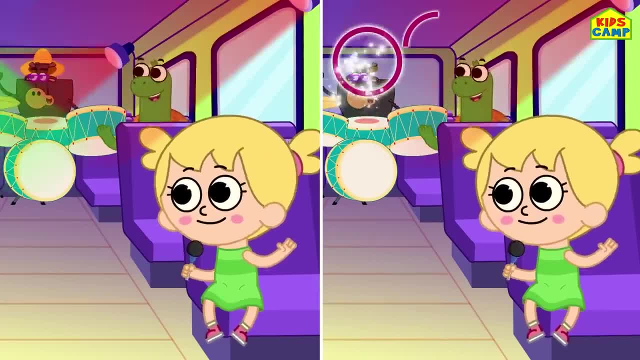 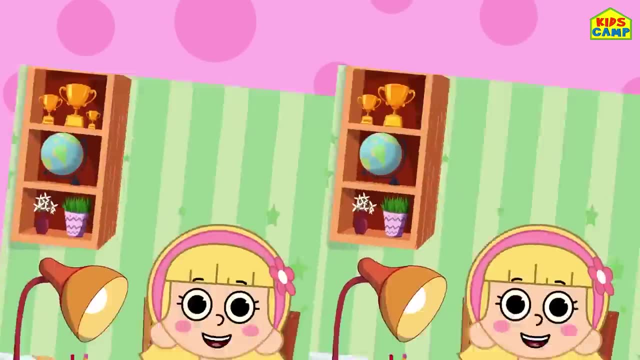 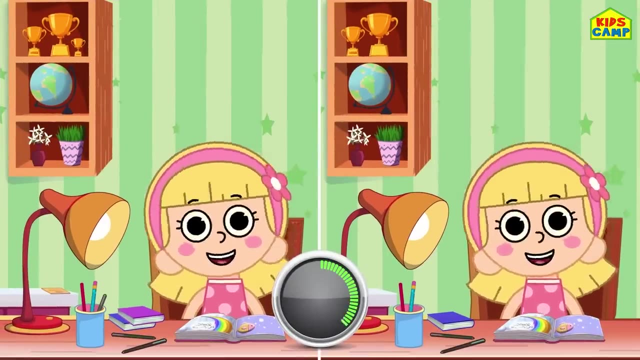 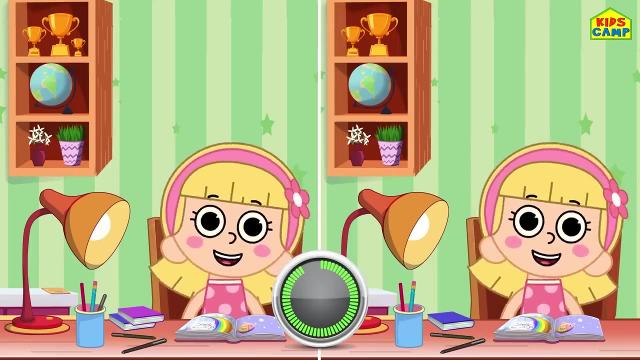 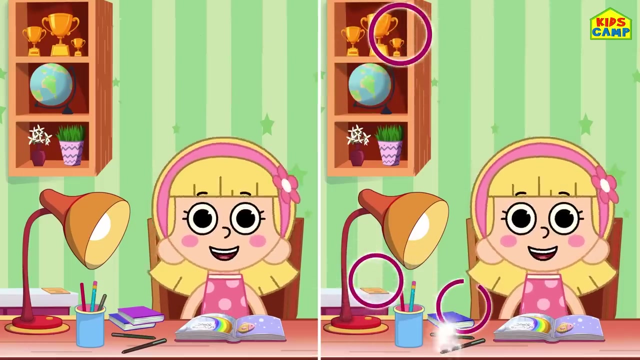 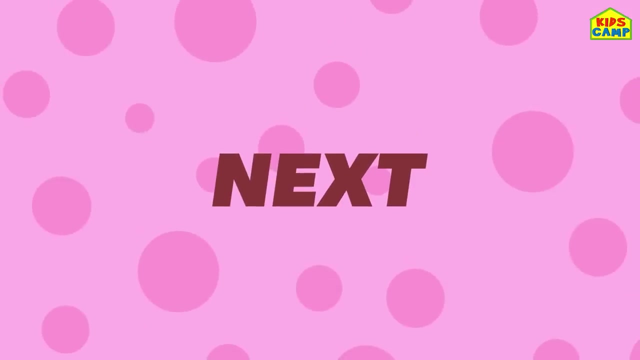 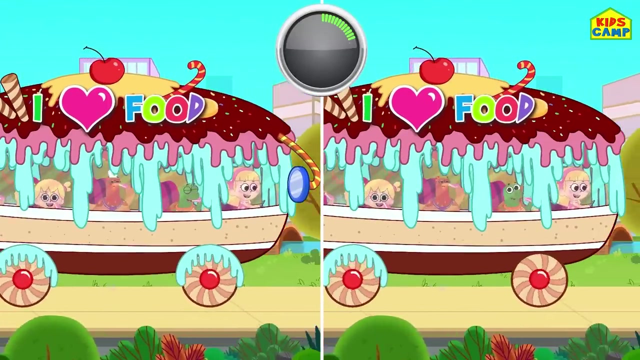 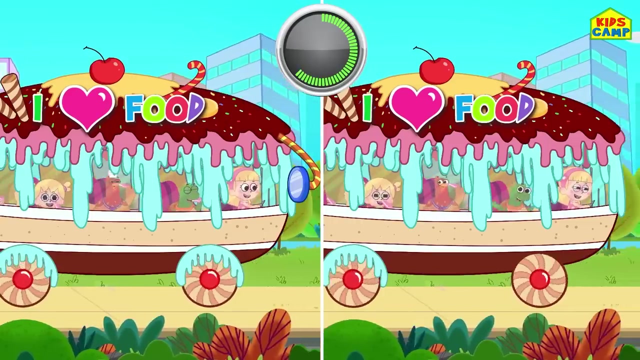 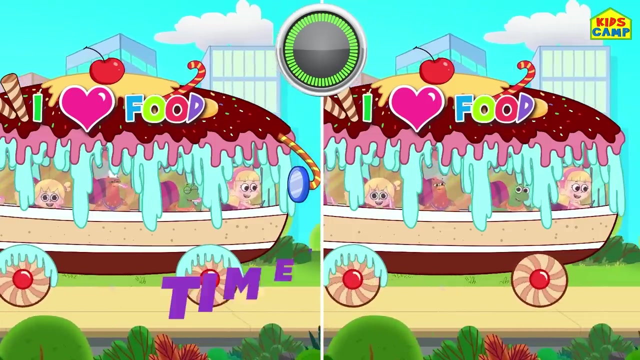 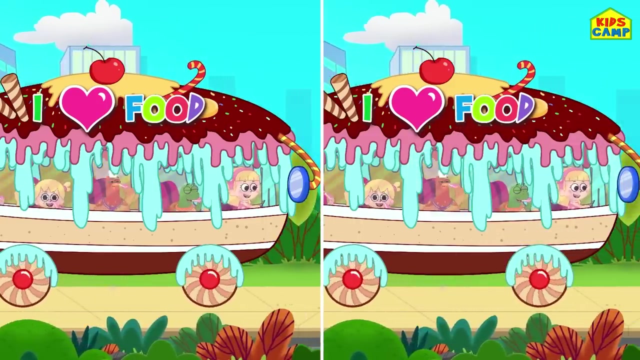 Let's do the next one. Can you spot the differences? Time's up, That's right, You got it. Next one: Can you spot the differences? Keep trying, Time's up, You got it. Good job, kids. This was so much fun. 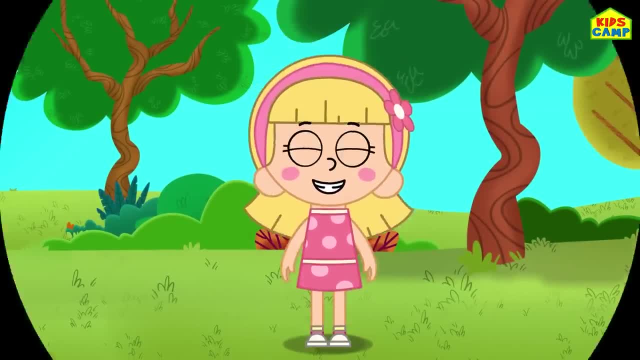 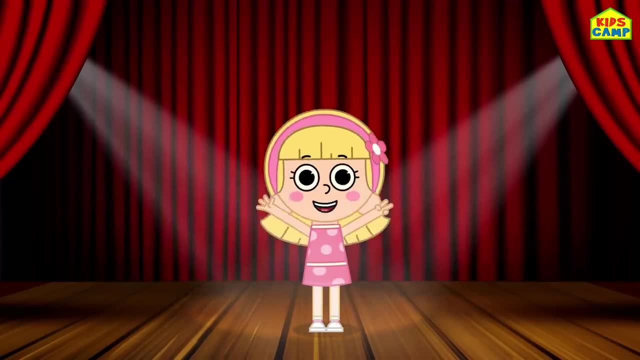 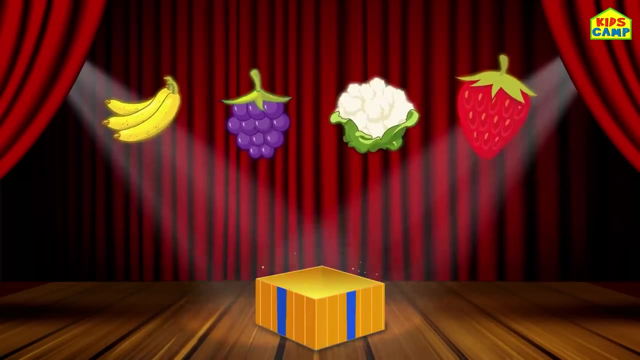 Keep watching Kids Camp. Bye-bye, Hi, I'm Ellie and we are going to spot the odd one out. Ready kids, Let's go Spot the odd one out. Hmmm, Is this a fruit? Yes, Is this a fruit. 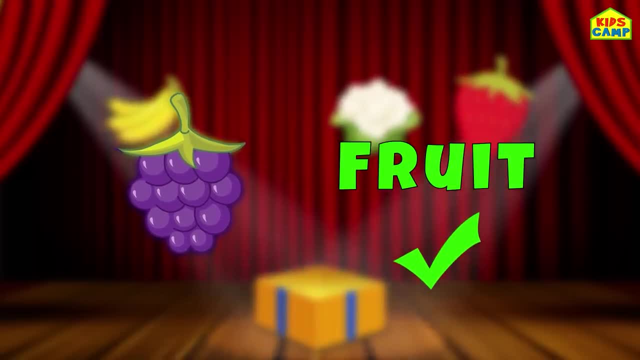 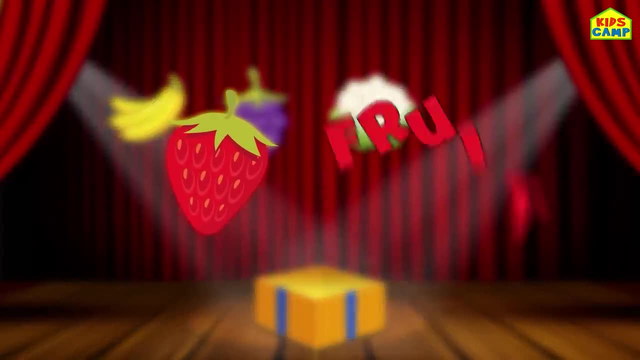 Yes, Is this a fruit? No, Is this a fruit? Yes, Here we go. This is the odd one out. We got the odd one out. Now what? What's this? Is this a fruit? Yes, It's a fruit. 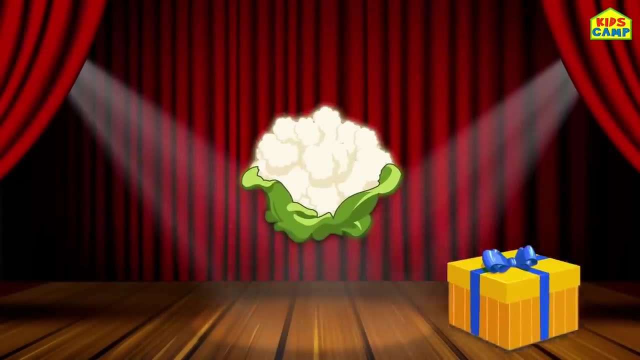 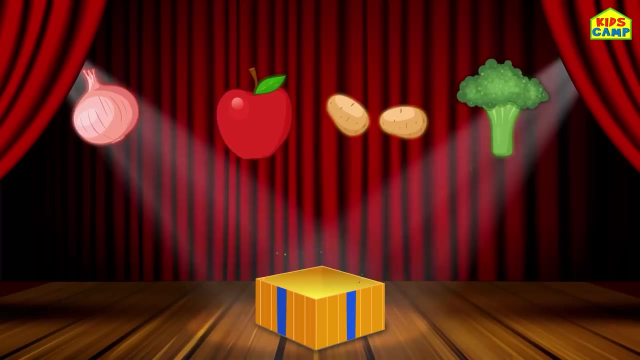 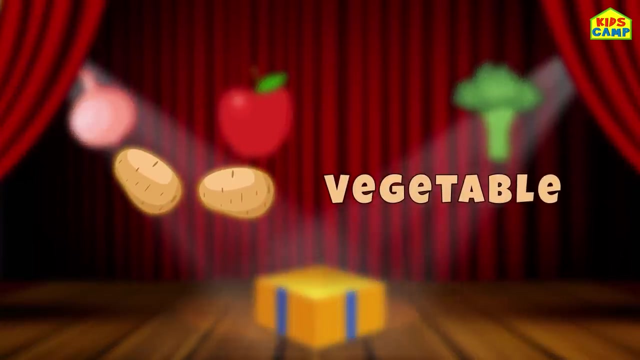 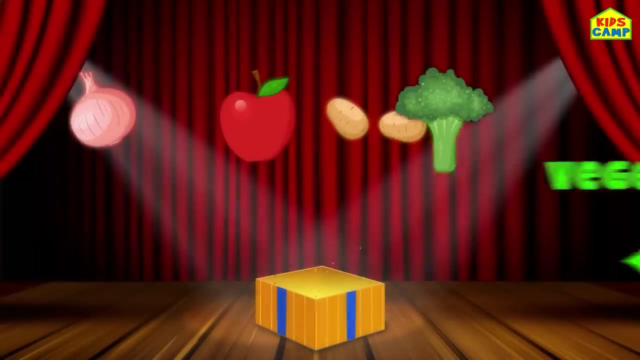 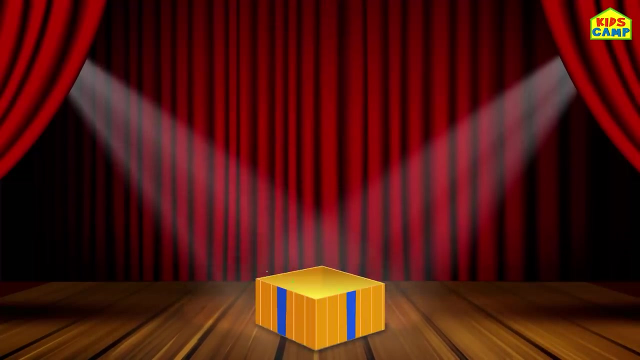 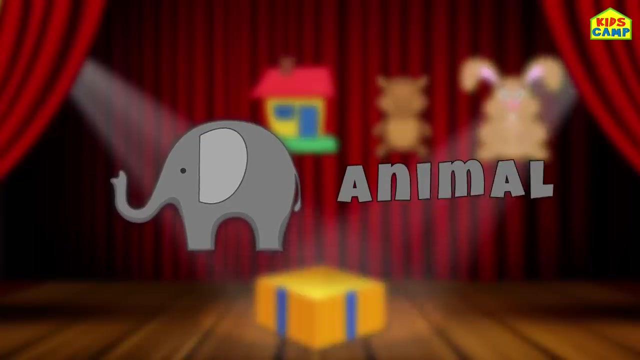 What? What fruit? It's a fruit. What fruit, What fruit out? Is this a vegetable? Yes, Is this a vegetable? No, Is this a vegetable? Yes, Is this a vegetable? Yes, Yay, We spotted the odd one out. What next? Is this an animal? Yes, it is. Is this? 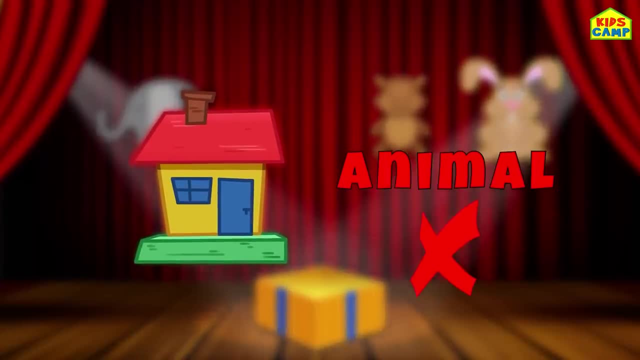 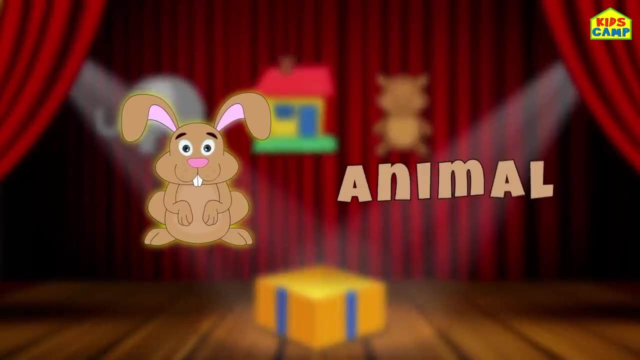 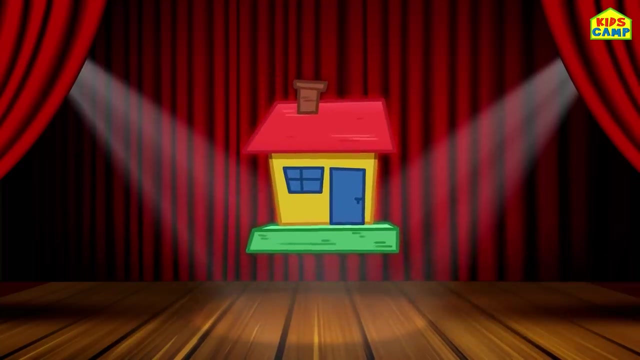 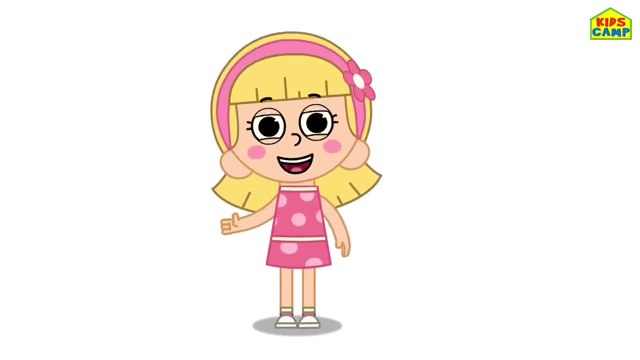 an animal? No, Is this an animal? Yes, yes. Is this an animal? No, Is this a vegetable? Yes, it is. We spotted the odd one out there as well. Good job, kids. Hi, I'm Ellie Well. 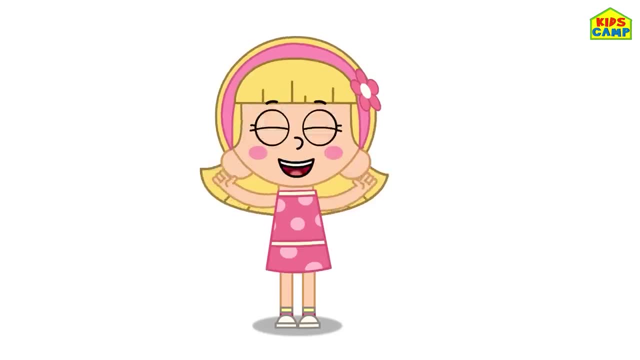 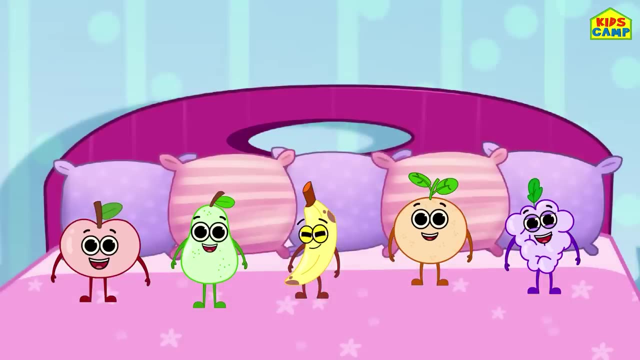 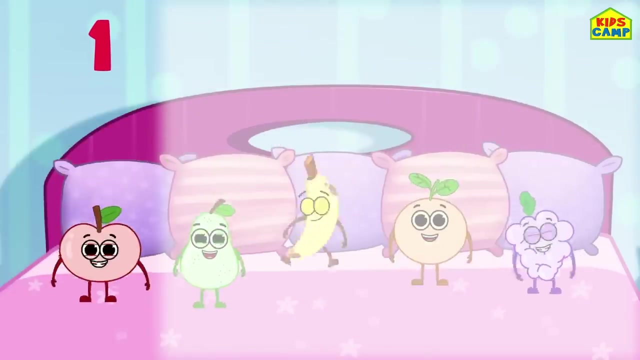 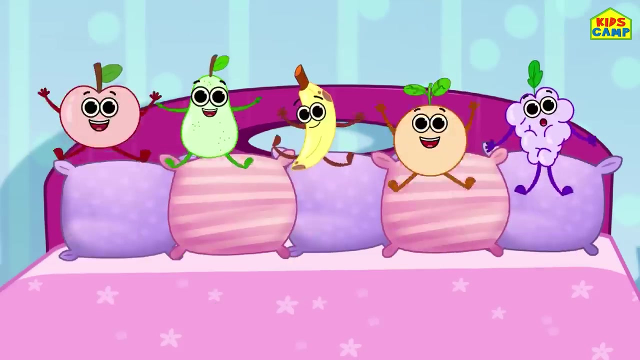 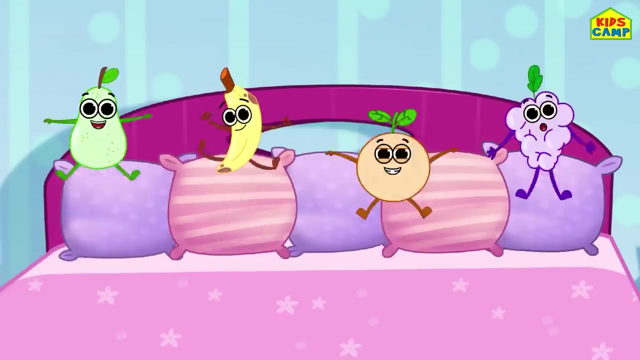 hello boys and girls. Today we are going to learn how to do simple math Subtraction. That's right, We have five fruits. Look at them jumping on the bed, So cute. One, two, three, four, five, Wow, Five fruits. Oops, one of them fell down. Ooh, how many. 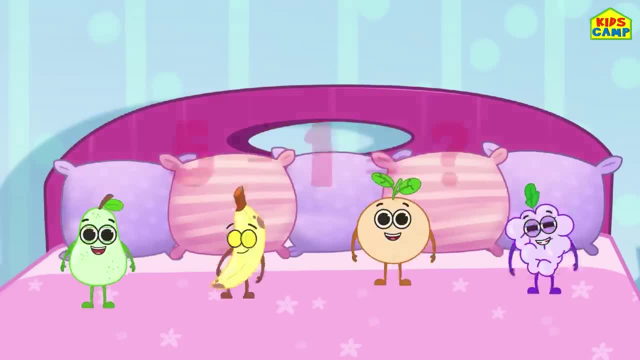 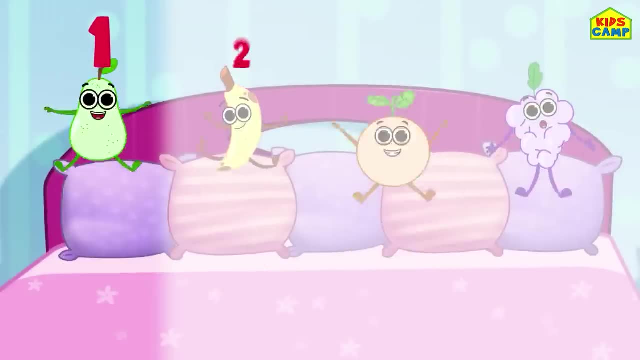 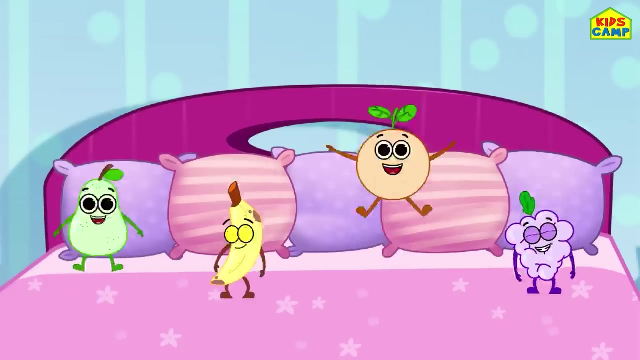 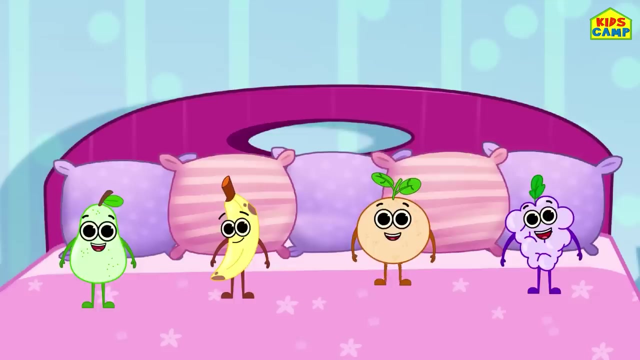 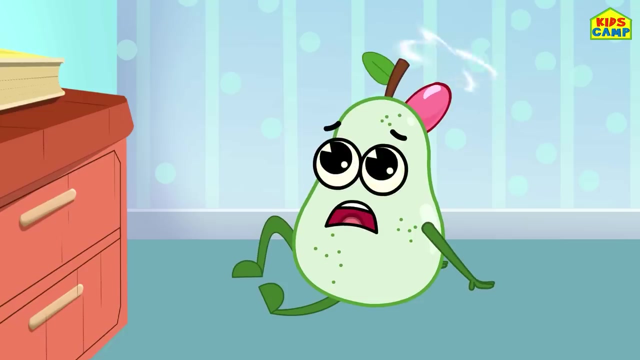 fruits do we have on the bed now? Five minus one is We have one, two, three, four, five, Four. We have four fruits jumping on the bed. That's right. Five minus one is four. We have four fruits jumping on the bed. Oops, one fell off. Oh, How many fruits do we have? 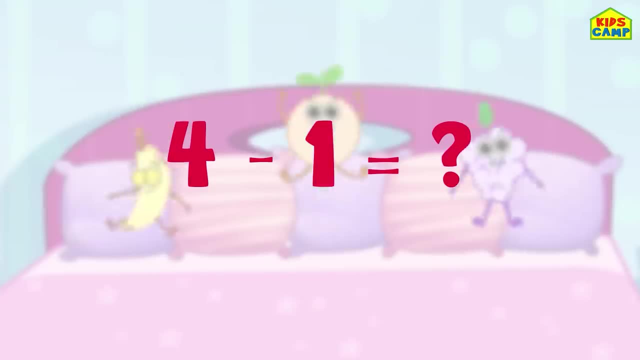 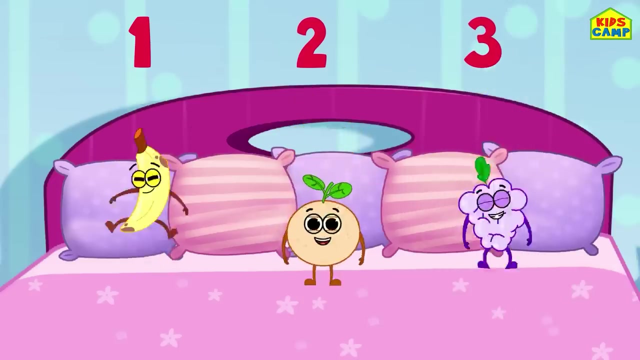 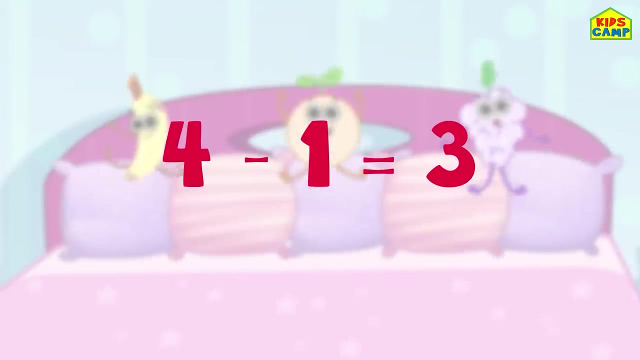 jumping on the bed. now, Four minus one is: Is it two, Is it three? Is it four? Is it four? Is it one, Is it two Or is it three? No, our boy are jumping off the bed, losing what they have lost. We have three fruits, We have four fruits. Four minus one, Oh we. 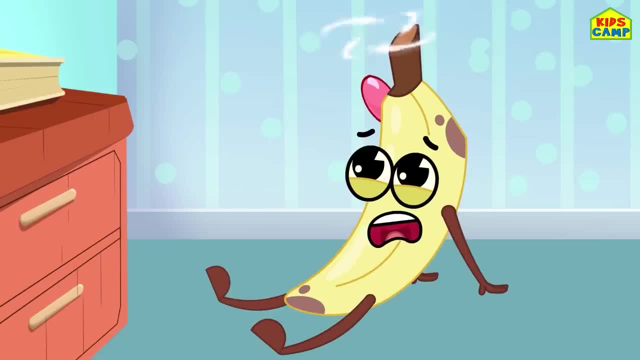 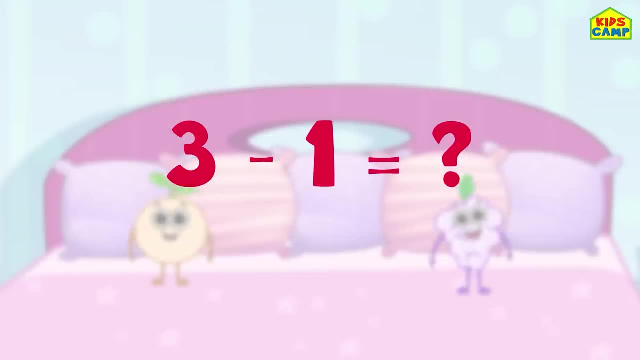 have two. Three fruits don't count. Yeah, Okay, having four fruits means we have five fruits, And will we hunt these ones down? Nope, Of course not. Then we need to find them. single 3 minus 1 is: is it 1, is it 2 or is it 3?? 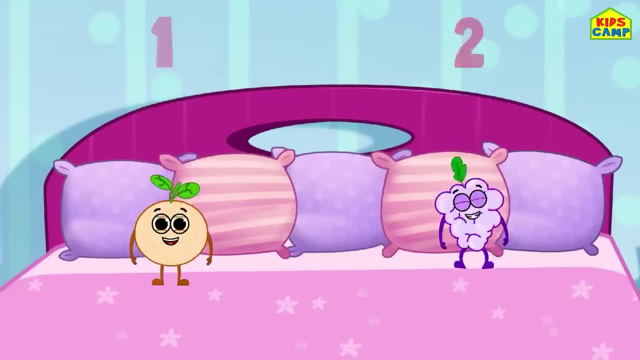 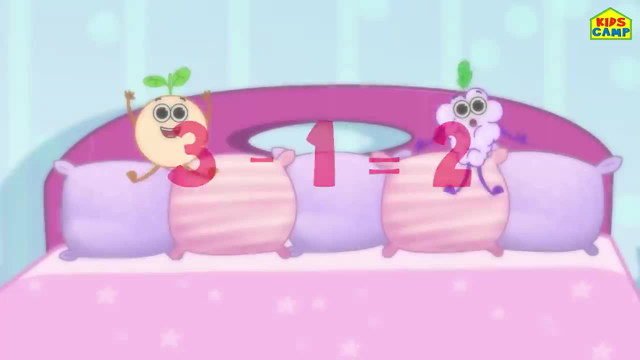 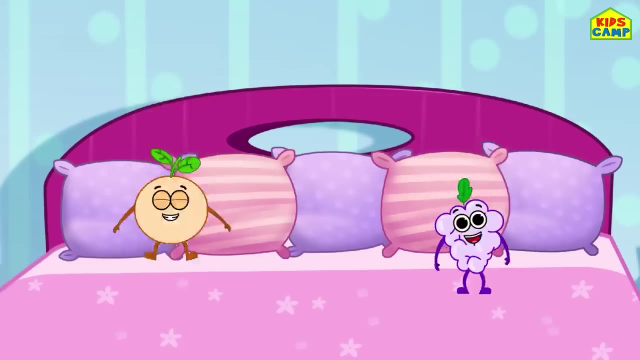 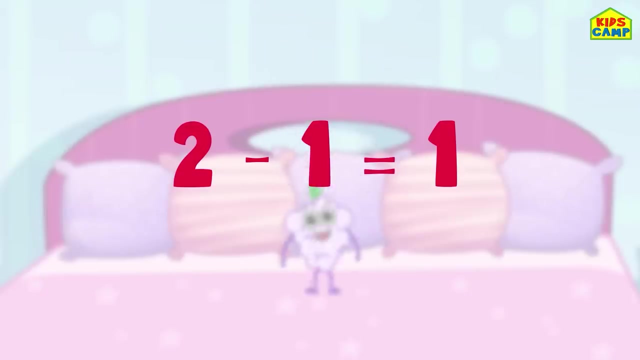 1,2. We have two fruits jumping on the bed. 3 minus 1 is 2.. Wow, One more fell off. Ouch, How many left on the bed? 2 minus 1 is 1.. Let's put it on the table. 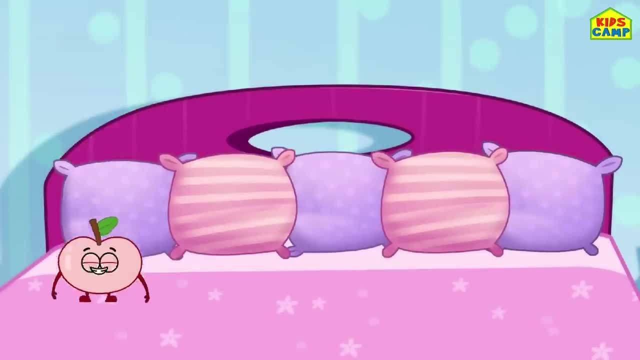 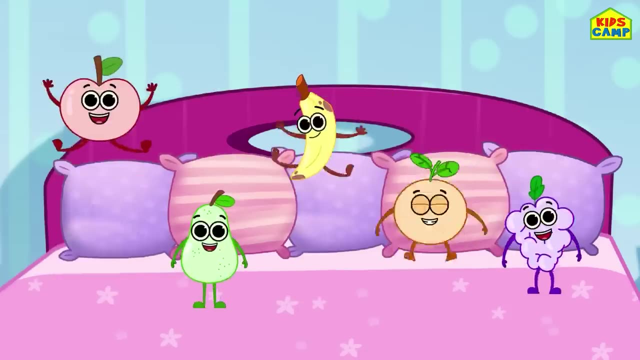 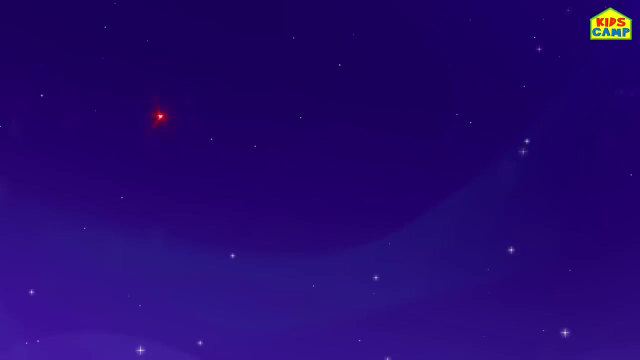 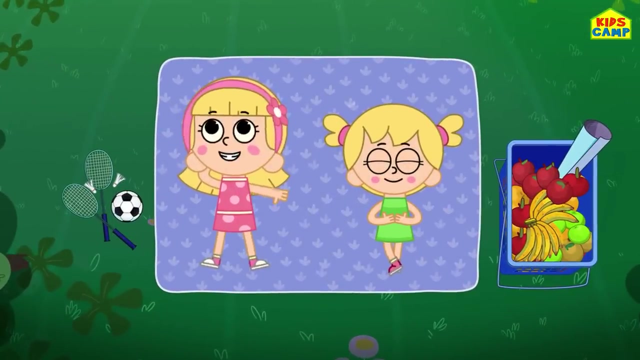 And put all the fruits back on the bed. Yay, We did it. Good job, kids. Bye, Look, Eva. Twinkle twinkle little star. Twinkle twinkle little star. Twinkle twinkle little star. 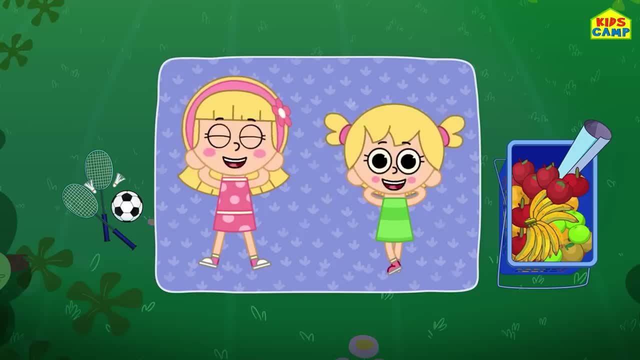 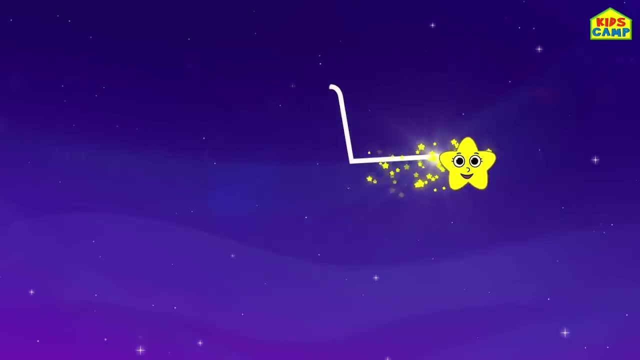 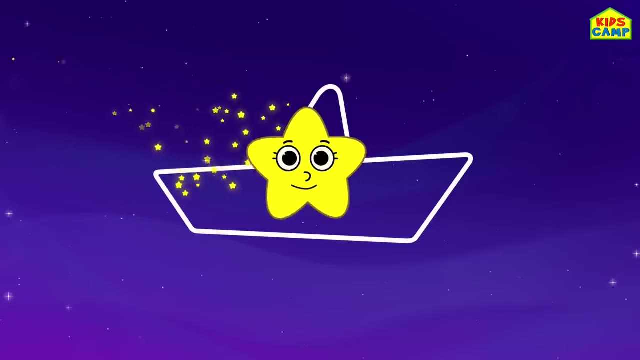 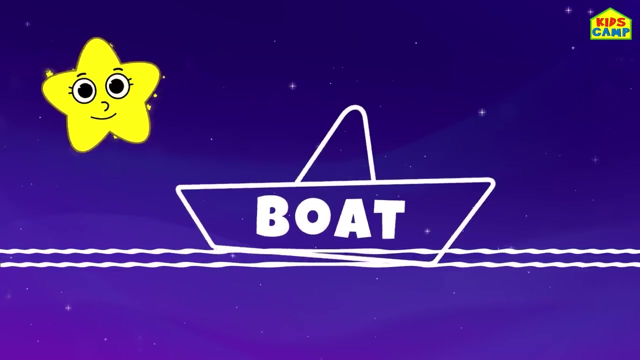 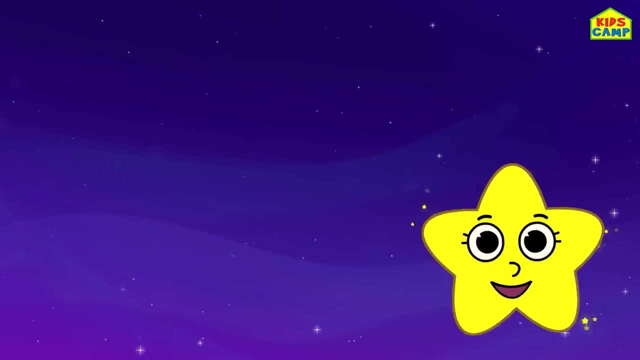 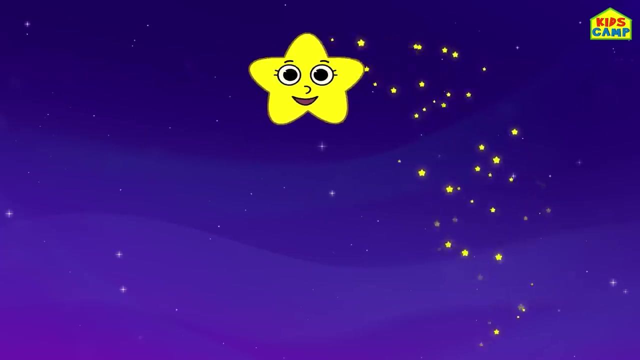 Tell me what vehicle you are. Wow, This is so exciting. Woohoo. What is that? I think it's a boat. The boat sails in the vast ocean. What is that? I think it's a boat. Twinkle, twinkle, little star. Tell me what vehicle you are. 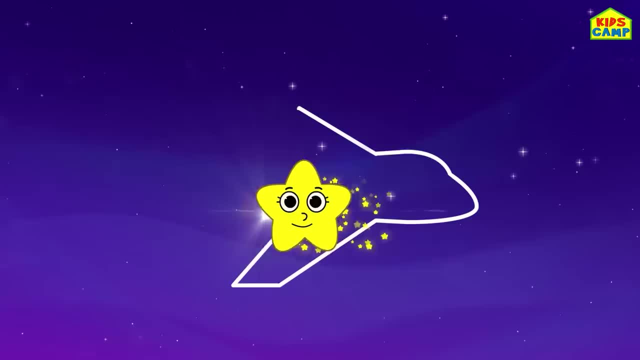 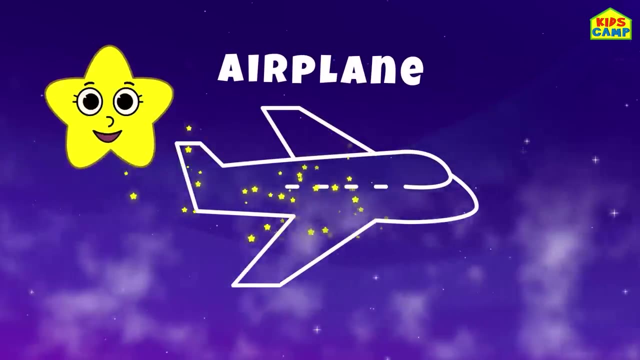 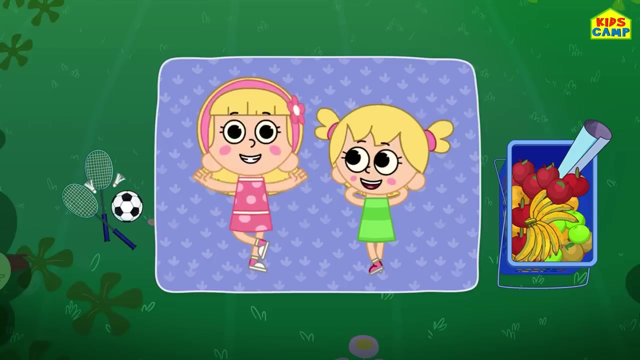 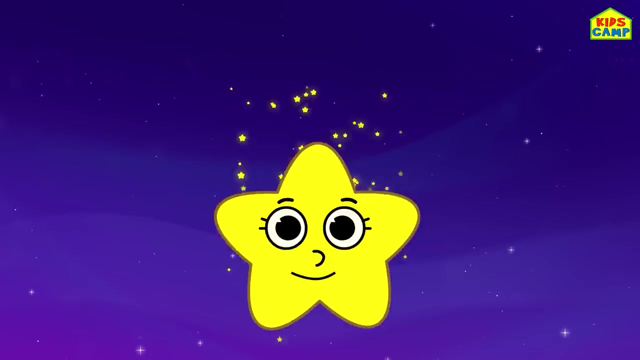 Here comes another one. Wow, Look, it's an airplane. An airplane flies high in the sky and can take us anywhere in the world. Wow, We're getting good at this Twinkle, twinkle little star. Tell me what vehicle you are. 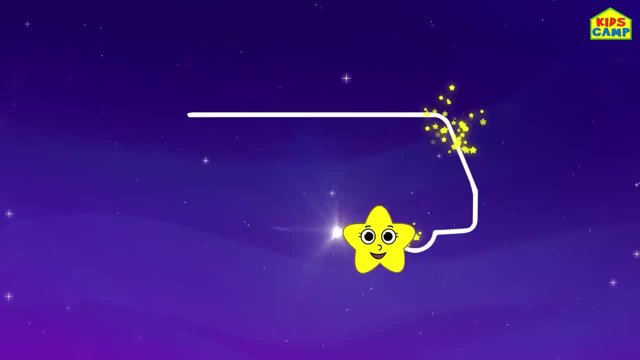 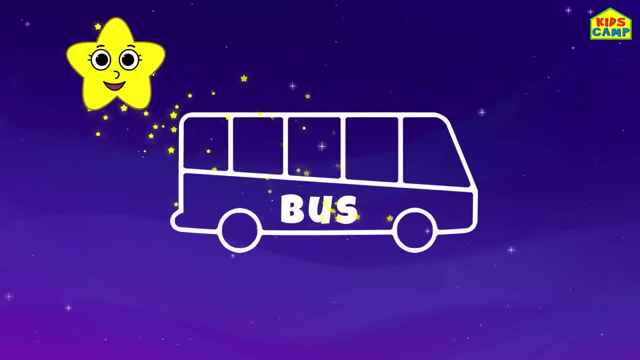 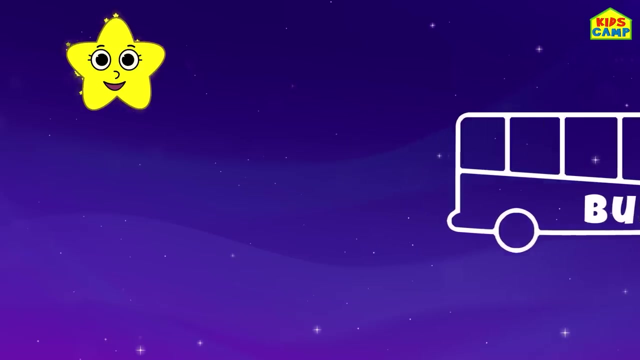 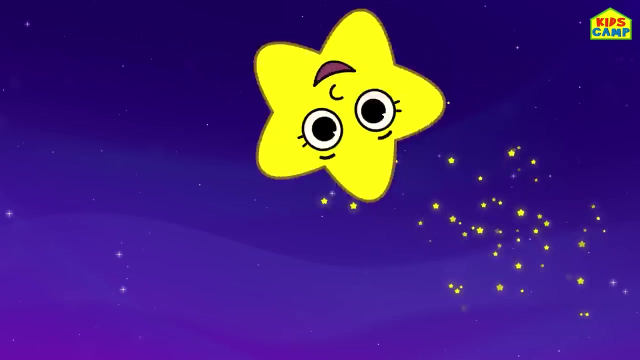 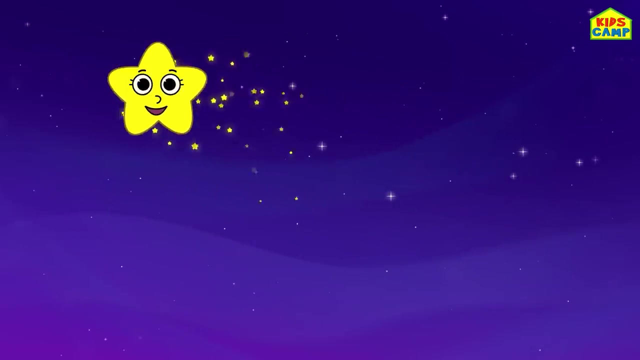 Look, look, One more. It's a bus. You're right, Ellie. We go to school in the bus. It's so much fun. Yay, Twinkle, twinkle little star, Tell me what vehicle you are. Here comes another one. 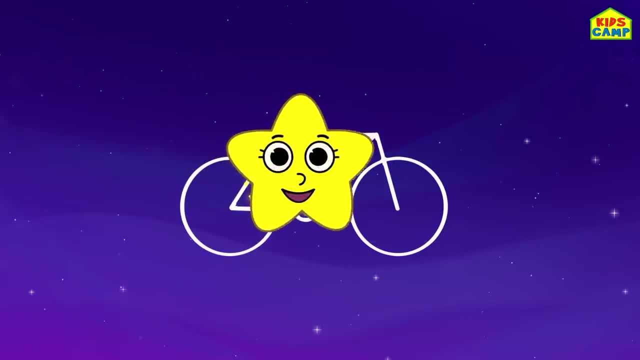 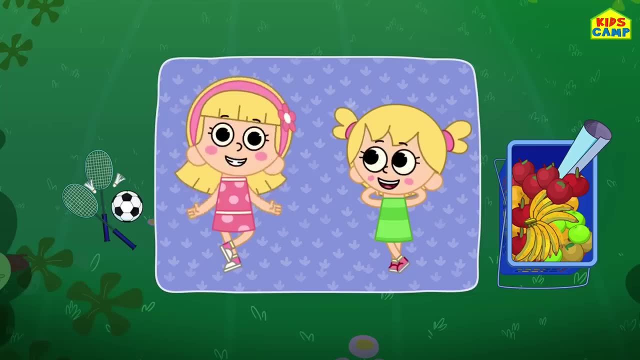 Hey Look One more. Is that a bicycle? Yes, yes, I love cycling. It also keeps us fit and healthy. Yay, We did it. We had so much fun learning vehicles. Goodbye, Woohoo, Hi friends. 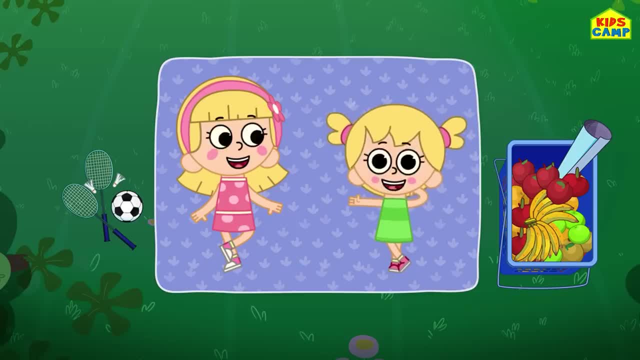 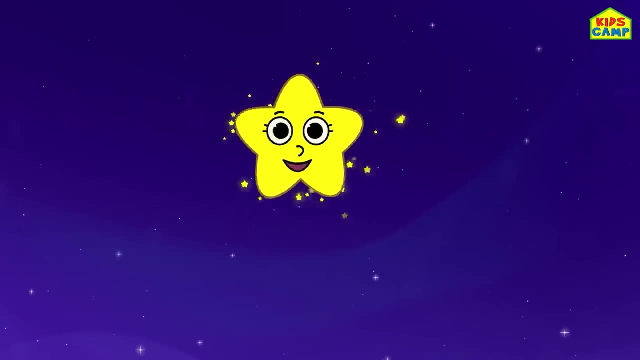 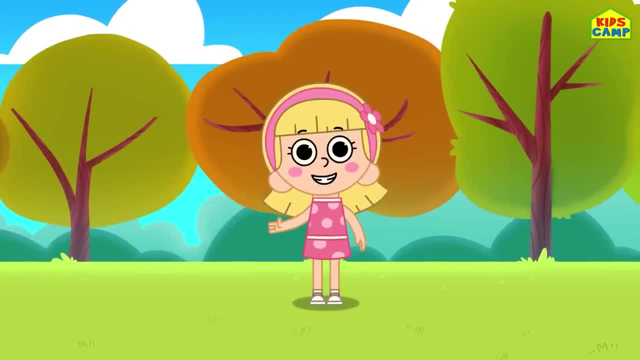 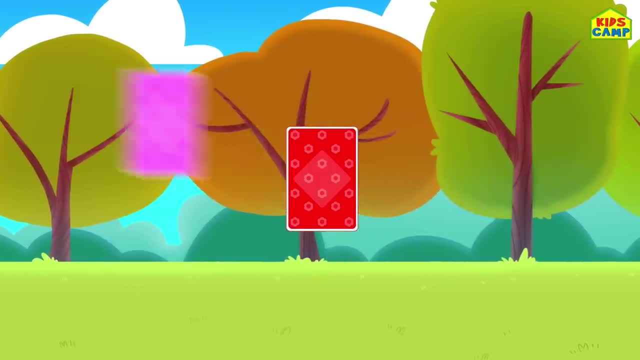 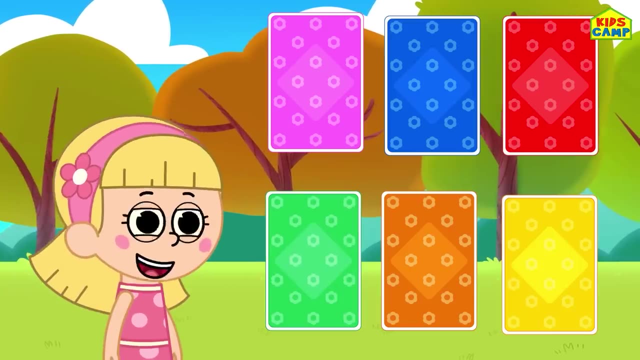 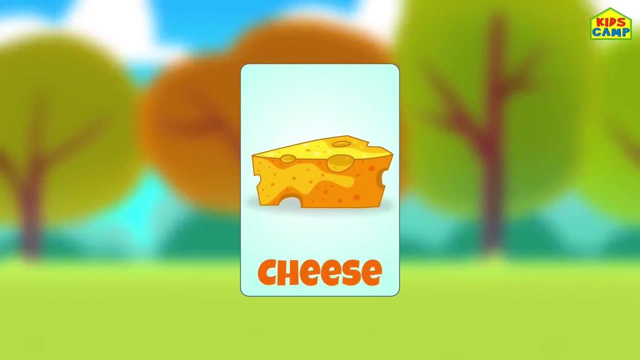 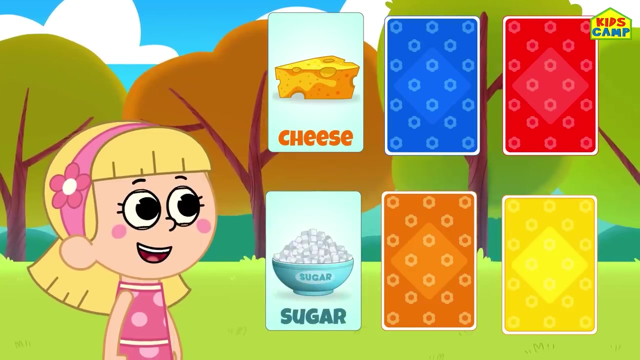 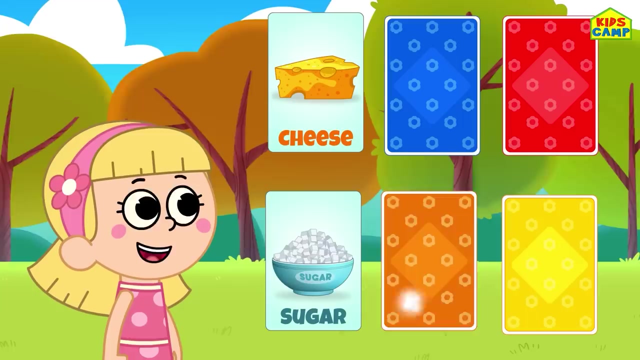 Oh, What is this? It's cheese. We need to find what cheese is made of. Uh, Oh, What is this? Sugar? Is cheese made from sugar? No, I don't think so. Let's flip another card. Hmm, it's milk.